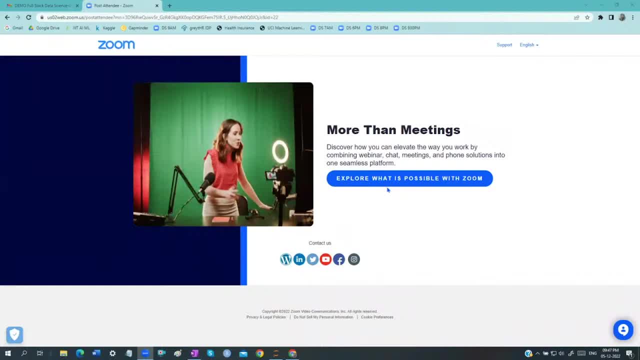 Like I think so many people are there, actually guys. Manohar, yeah, Just give me a minute. So, yeah, right, Okay, guys, So guys. I can see some more people has been joined as a today's class. Today I think you have been joined as a demo class, actually guys. But 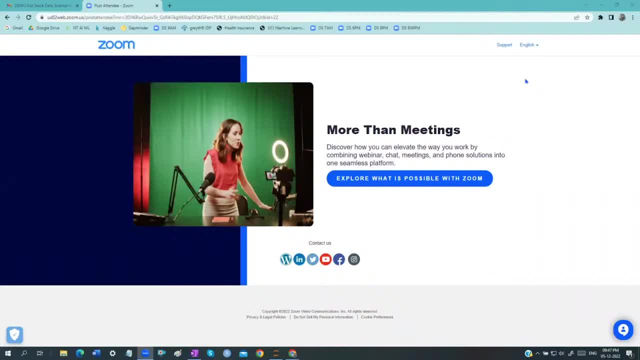 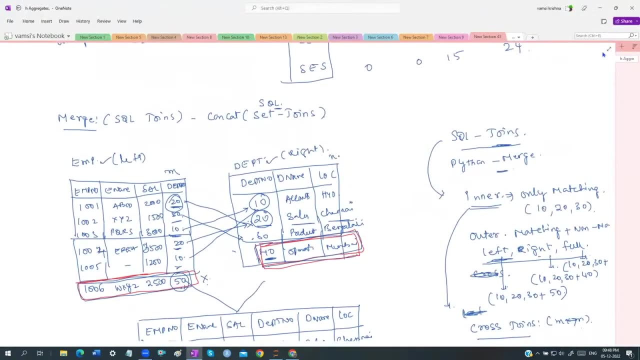 let me tell you what has been happened, guys. So in the last week only we have been started this session. Last week means it is almost two weeks, actually, guys. One week is just a demo sessions, actually, guys. So it is hardly two weeks it has been got happened, Just we have been started with. 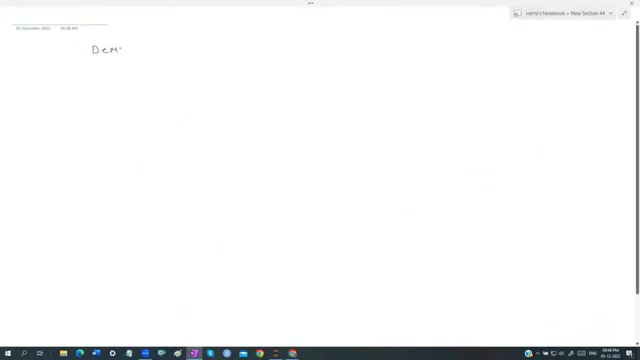 some first week We have been taken a demo session. actually, Demo means like: what is data science, what is machine learning? These are the some of the things, What I have been got discussed about that. So that has been happened for one week. One week means it is. 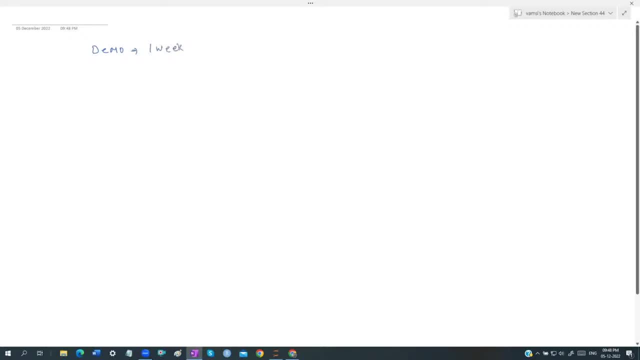 not too much time actually, guys. Just hardly 45 minutes, 50 minutes class only. I can see that actually we have been taken. So in second week I have been started with the basics of Python. We have been got started actually, guys. So this has been happened for some. another one week It has. 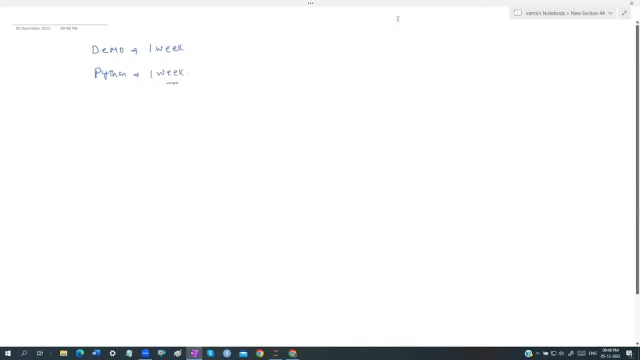 been got happened, But I can see some more guys has been joined now, So don't worry guys, I am going to take some backup session actually. So I think I can say somewhere around 7 to 8 people has been joined for the today's class. I can see your names, like some names, I can see who has been joined. 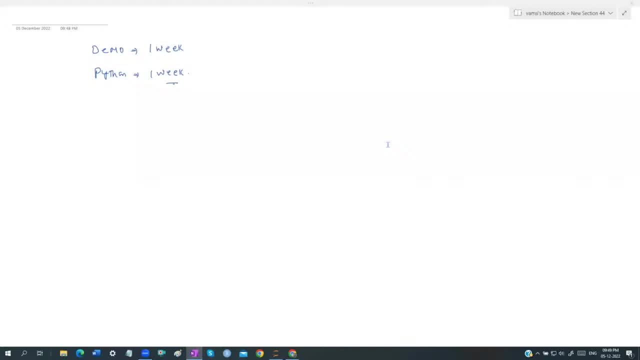 for the today's class. Somebody has been joined in the previous sessions only, But a very few people. 7 or 8 people has been already joined. They have been already registered for the course. I can see another 7 to 8 people. I can see it actually, guys. So don't worry, guys, because I thought that maybe 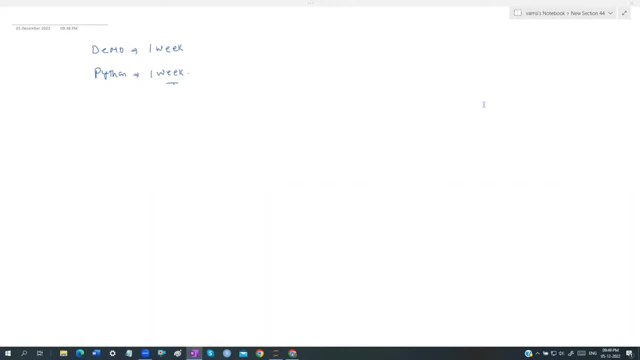 one or two people may join, But I am going to take some backup session actually, So I think I can see I have seen a little bit more people has been joined, So don't worry, guys. who has been joined for the today's class? So don't worry about that, because I didn't expect that these many guys will. 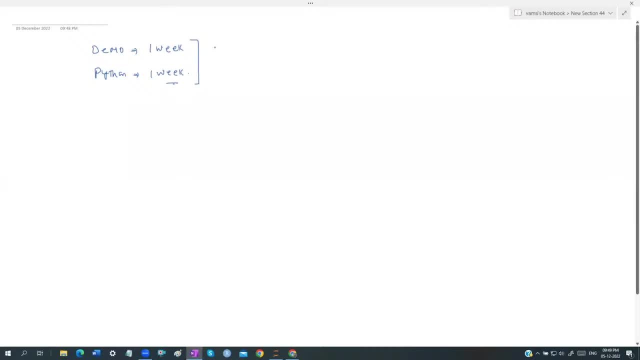 join. I expected that there may be some regular students. There are 7 or 8 students has been already registered. I expected that maybe somewhere around 3 to 4 people, But I can see somewhere around more than 8 people. 8 participants are there. who has been joined for the today's class? 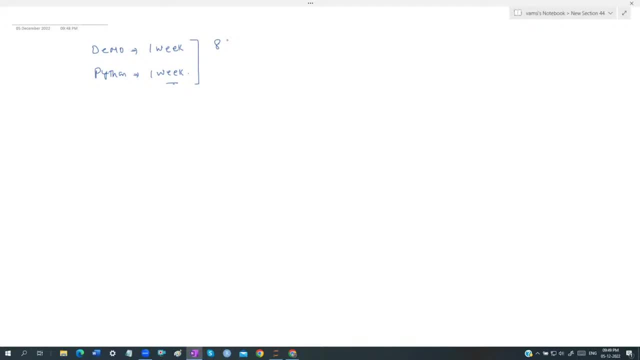 Because what has been happened. don't worry about that. It's only basic things. If you are already having some core concepts of Python, it's a very simple topics only which you can understand them. Don't worry, I am going to take the backup session. guys, If you really feel that there is actually I 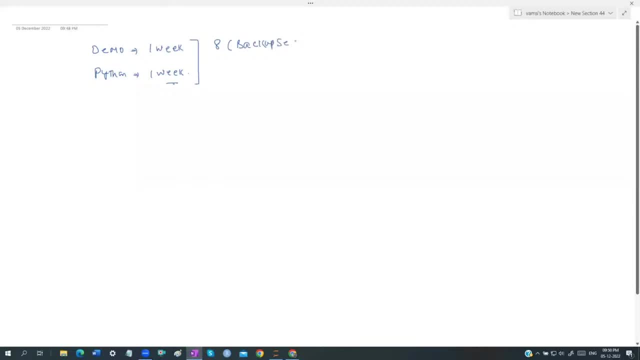 can give you a recorded session actually So I can take some kind of a backup sessions. I can take it actually. But just give me one or two days of time. I will arrange the backup sessions actually, guys. Okay, So don't worry about the completed. 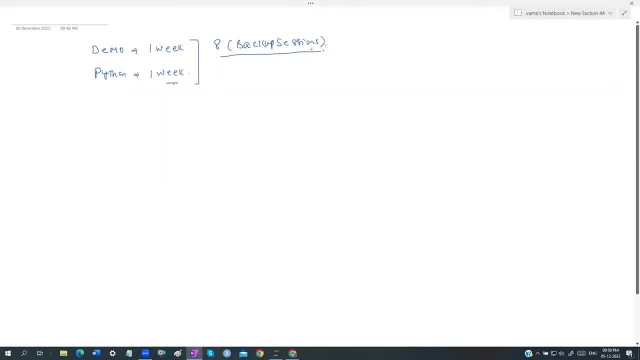 What has been already done. It's only basics and only some part of introduction Only. we have been got started, So in first week only thing is like what is data science? like what is machine learning, what we can do it in machine learning. It's only just an introduction part, Actually actual. 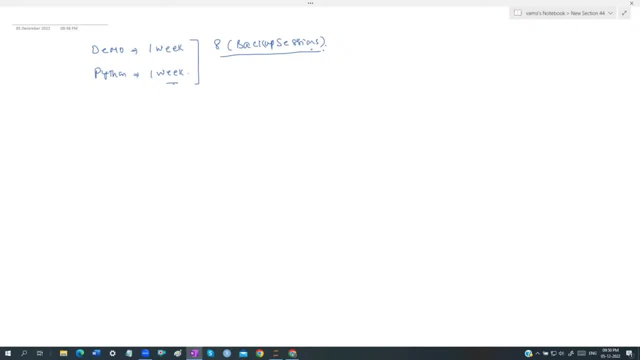 discussions will be there and actual explanations will be there whenever we start with our regular classes of machine learning, So that you can just go through the recorded videos and you can go through them. and coming to the python also, guys, we are still in the basic concepts only, so don't 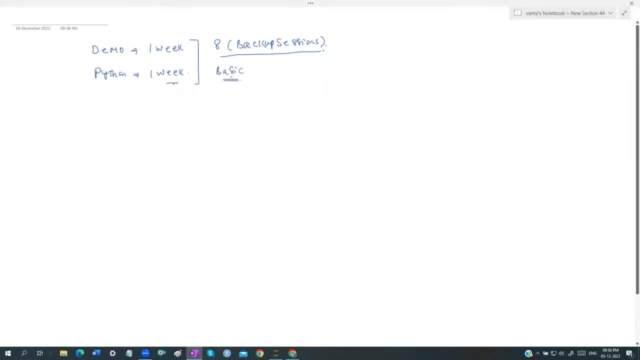 worry within just two or three classes? hardly. whatever the basics i have been about discussed is hardly three, four days concepts, only guys, not more than that. so what is my suggestion for the guys who has been joined for the two days classes? again, i cannot start from the 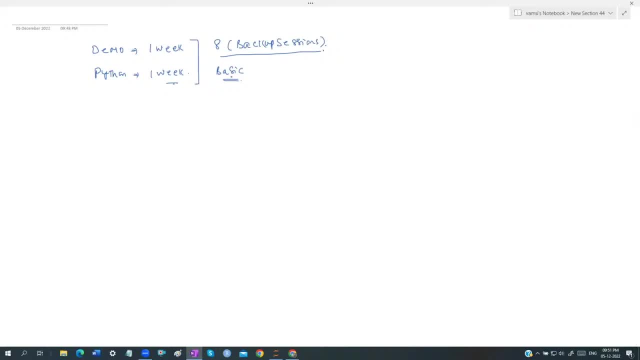 introduction part in the today's class. because i don't have a plan. i don't have a plan. i will arrange the backup sessions, guys. so whatever the classes you have been got missed i am going to discuss as part of that particular backup session, guys. okay, i'll plan it, i am. 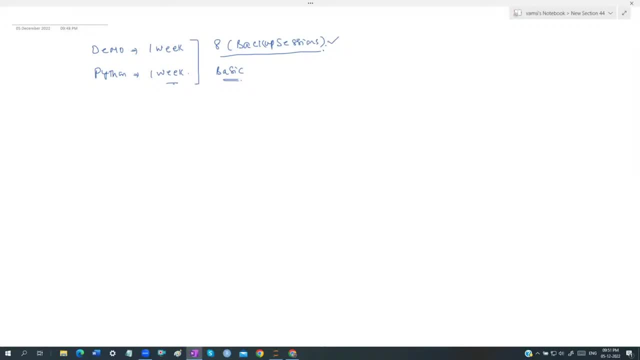 going to plan those particular sessions and my team will intimate you about those particular sessions, maybe by the end of the week or maybe some friday, saturday, sunday even. i'll take a sunday session and i'll take some kind of a backups and i'm going to make you understand. 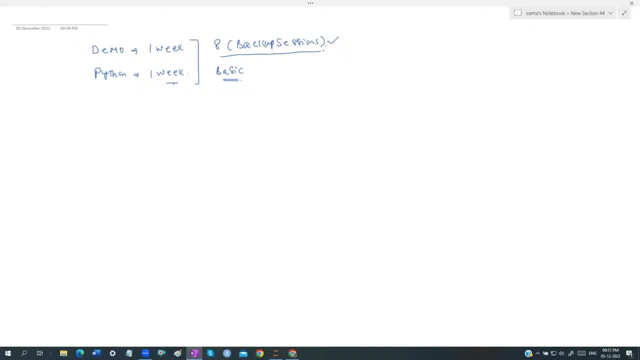 whatever the missing classes are there. so we have not yet started with any machine learning concept. we have didn't started anything about data science classes, actually guys, actual classes. we have been not started about that, so don't worry about the classes. i just started with some introduction part of the data science and we have started with the one week of python. 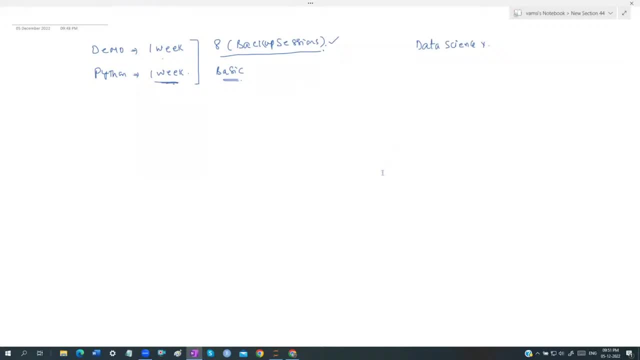 classes only. we have been got discussed. yeah, i'll, i'll, i'll add them, we'll. we know everybody's been about that. we'll have all that information. i'm going to do that, actually, guys. okay, fine, so don't worry about that. no, no, it's no worries, don't worry about this, guys. my backend team. 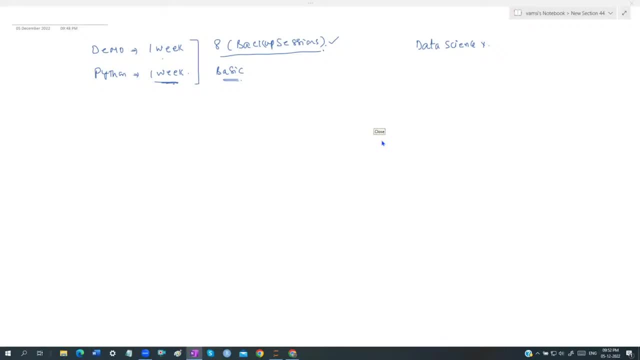 will have all your details and they will take care about that. okay, i'll add up everything, so no worries if you come to find any more. names are available now. as i said, it would be just a proszę dot com at the finish of this video, because they are now on the heaven. 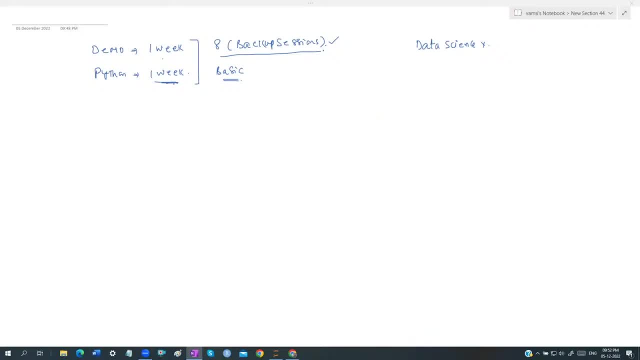 even coming up with more related video. all the details are available in the description of this three radiation channel at the end of this video. we have an entire training schedule for you guys from from tel Sap drill buddies here from sur find this method. go to our website, patrick kenney. 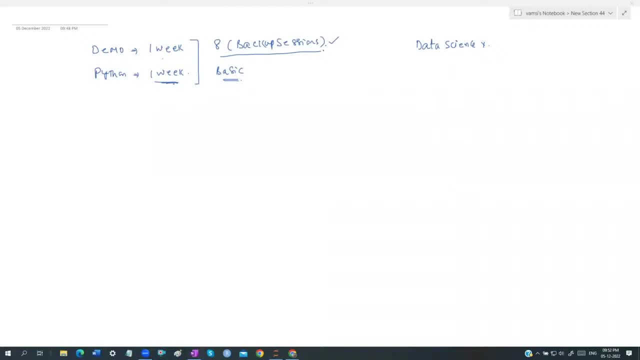 don't know what is the reason. it may be a short intimation or something like that. very few guys has been joined and we expected that more people will be joining, uh, as part of the registration. but i can see. but today we have a good number, actually, guys, so 20 people, i think, 20 participants. 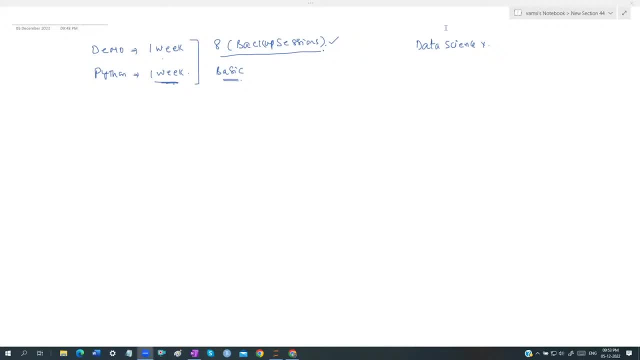 are there now. including me and my back-end team, it is 17 candidates will be there. sufficient guys. 20, 21, 22, 25 people will be there. so don't worry about the data science classes, guys, because everybody is having an interest like they. we don't want to study with the python, so what, what? 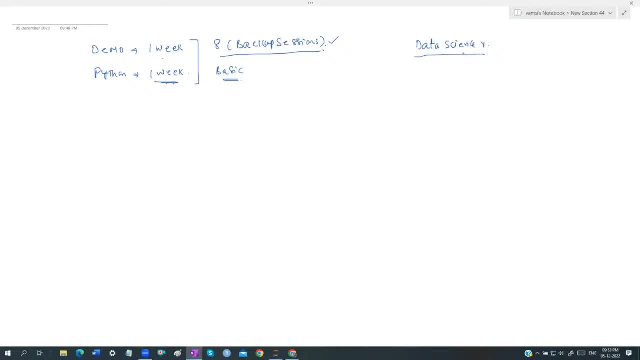 we are going to learn as part of the data science. what are the techniques, what are the technologies we are going to learn? i'll arrange a backup session, guys, don't worry, just give me one or two days of time. i'll take a backup session. so today, don't worry, even if you are not familiar with the 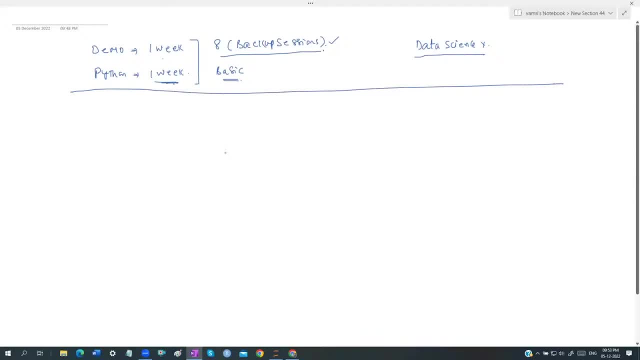 concepts, whatever i'm talking today. don't worry about that. just go through the class. it is only just like a why do you? why, basically, demonstration is required. guys like to know what is our plan like, what is our schedules, like, how we are planning the schedules or how my lectures are there. uh, is my? is i'm teaching in a proper way? 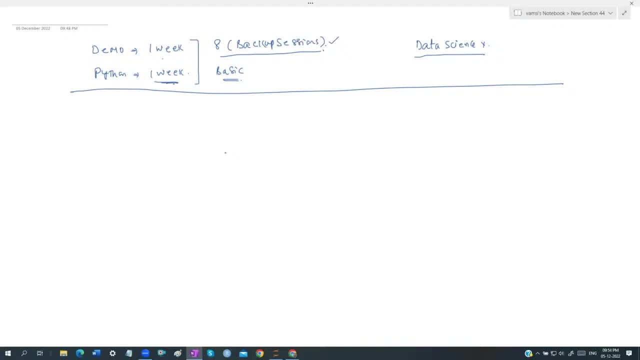 or not? so how is my explanations? uh, can you catch up my accent, or not? so to get some idea about that, we'll attend the demo classes, right? so after that you will plan it, whether you want to join my class or some other x batch or y batch. you want to join it actually, so, being i cannot directly. 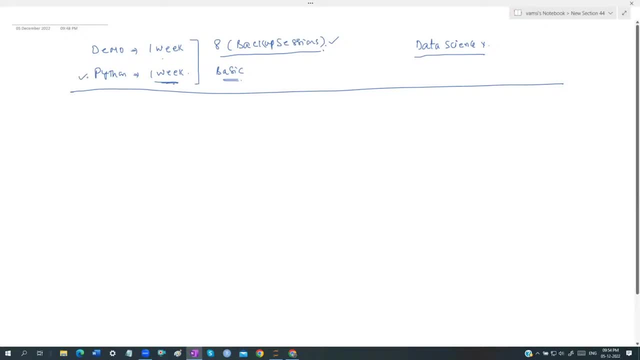 do this? i don't have any plan for that. actually, let us happen today and tomorrow will just happen. we'll just plan for the, as usually with the python classes guys, maybe today, tomorrow and day after tomorrow. as of my plan, if the same numbers are there- monday, tuesday, wednesday will cover them. 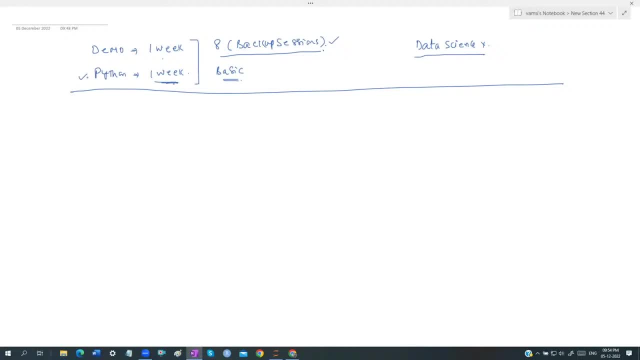 and i'll break the batch. and thursday, friday, saturday and sunday: i'll take the backup sessions. i'll cover all the things actually, guys. okay, and being it is already a late night batch, i cannot extend the batch more and more. that is one, so we'll try to. we'll try to just make up the backup sessions so that everybody will be on the. 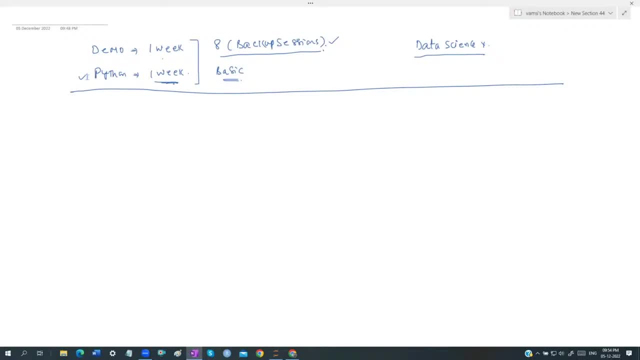 same page, but today everybody is not on the same page. some of them are in advanced level, some of them are going to be in the beginning levels. actually, if you are already having the concepts of python, guys, you can handle that. we can just understand the concept. what i'm talking about. 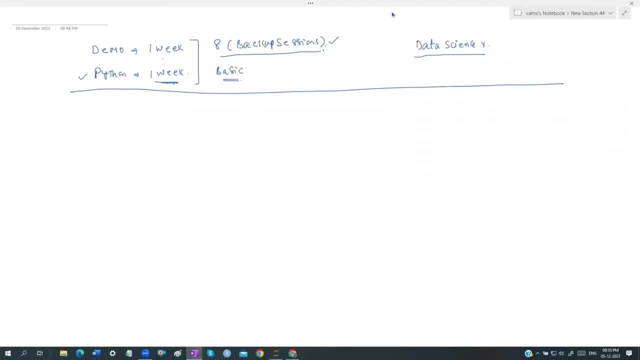 okay. so guys don't worry. who has been joined for the today's class? so please give me just one or two days of time, because the batch was already started. you may be having a little bit lagging, is you? so don't worry, i'll take up the backup sessions and cover all that particular whatever. 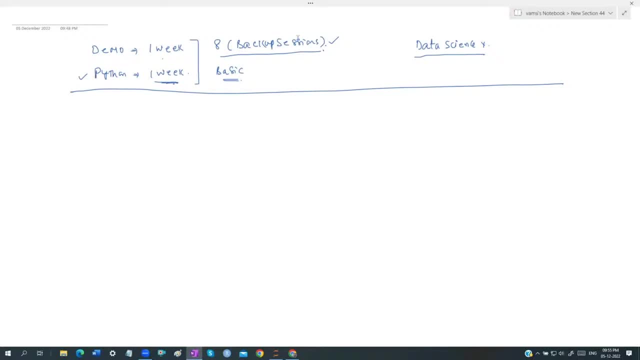 the message topics. are there guys? okay, i'll give you five, ten minutes uh time. i'll give you, guys, at the end of the class so that we can have some discussions. we'll have a discussion, guys. okay, right guys? uh, hope all of you understood what i have been explained, guys. 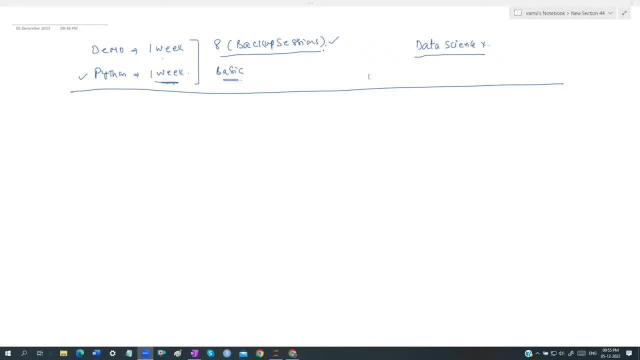 fine, guys, so you can use a chat panel. guys, try to answer it, just try to make it interactive. just answer it as s or no so that i can know, like, what you are feeling, uh, regarding my discussions. actually, okay, so shall i continue, guys? shall i continue with the regular class guys? right, i'll, i'll continue with the regular class guys. 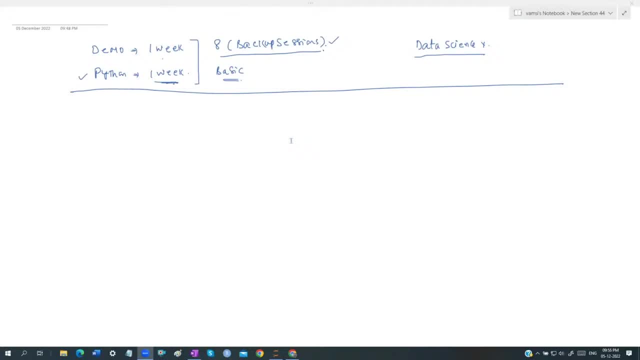 maybe some of you will already have an ideas about that. if you're already having a python, you don't find any difficulties. okay, fine. so, guys, we have been started with. uh, currently, our discussion is on the a python concept which is going to be in python. we have something called as: 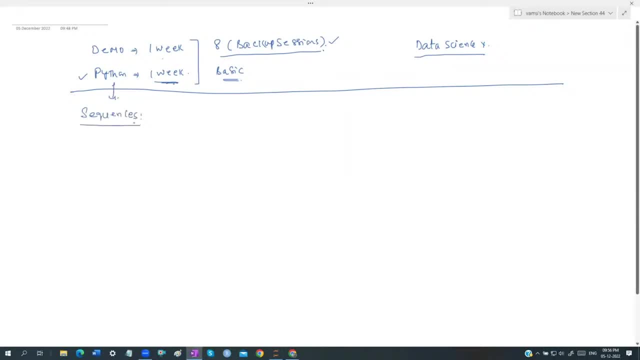 normally, if you have an idea about a programming languages, so it's not a python class. actually, guys, we are learning python for implementation of the data science concepts. so some little bit core python is required, guys. two weeks python is going to be required. the two weeks python is only what. 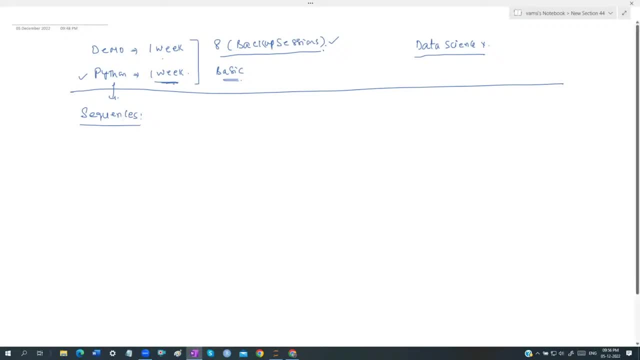 i am trying to discuss it here, actually, guys. okay, so in python we have some concept called as in sequences, actually, guys, some kind of a data structures which are basically to store multiple values. actually, like, we have something called as ld's, we are having something like a tuples, we have a set objects and we are having something called. 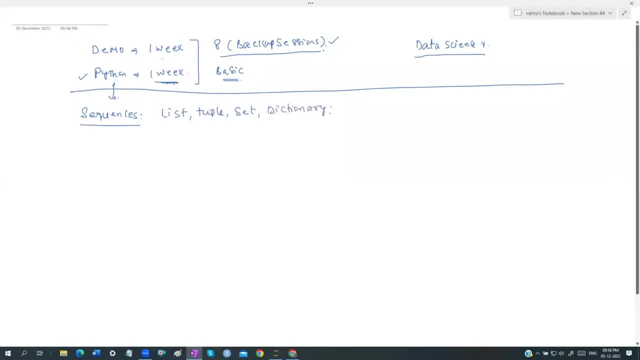 as an a dictionary objects. actually, guys, these are the four basic data structures which we use it in python currently. we have started with the list concept. actually, guys, what is a list? actually, a list is going to be nothing, but it is a collection of some which is going to be some. 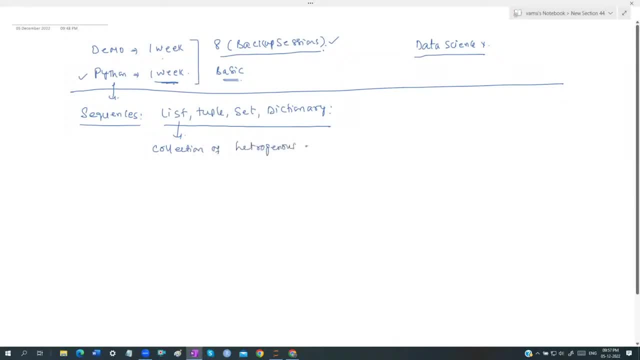 kind of an heterogeneous elements. actually, it is not just a single value. actually, guys, it can store elements. those elements can be it. it can be of a different, different data types, heterogeneous. how do you create a list? actually, guys, list is created just by enclosing within a square brackets. 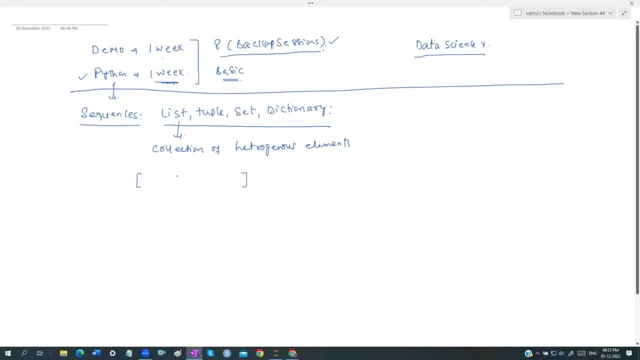 like in other languages. you need not to write something like list, integer, float, okay, string. we need not to write it. actually, guys, simply, we are going to put some kind of a square brackets actually. yeah, yeah, i'm discussing. i'm discussing it actually it's nice. just i'm giving some 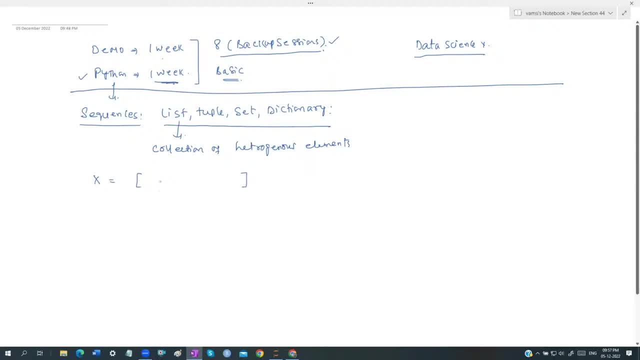 idea about what the what has been happened actually. so list is going to be nothing but a collection of some heterogeneous elements. what we are going to be having actually, i guess an integer and we have a float, we can have a string, we can have a bull, etc. etc. we can have it actually. yes, so this is: how do you create a list? 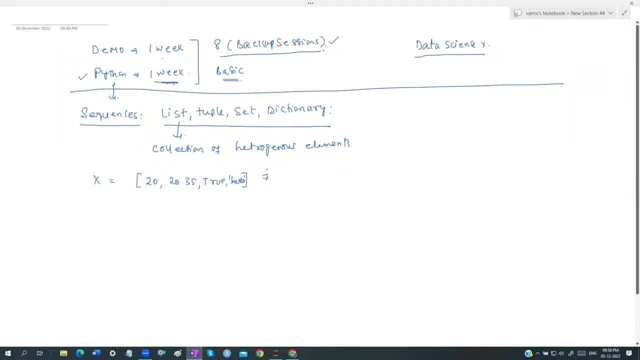 to manage this list, actually to manage the list. what is the meaning of managing off list? actually, guys, we can add some elements, we can remove the elements, we can modify the means, so we have to require some kind of a methods that are required, actually, guys. so very simple. 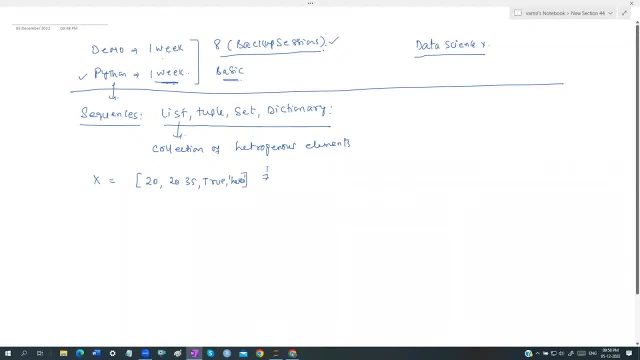 guys, i have discussed only four methods as of now. i discussed only four methods actually, guys. so if you are already having an idea about object oriented guys, well and good. who has already having the idea about object oriented? even if you do not have any idea, just understand them. 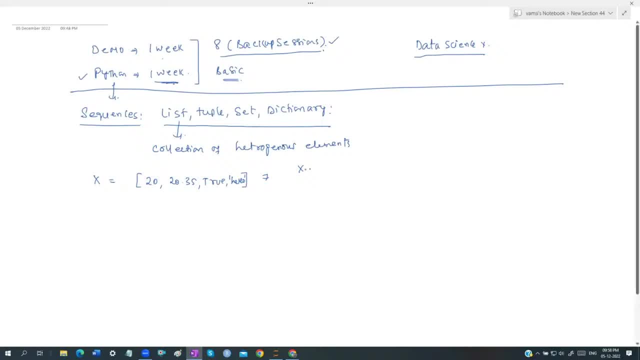 i am going to discuss about those particular applications later. actually, guys. so i have been got discussed about what is a method? actually, guess, method is nothing but just a function which is used to do some management or a manipulation with that list. actually, guys. so, for example, if x is a nothing but a list, so this is going to be nothing but a list actually. 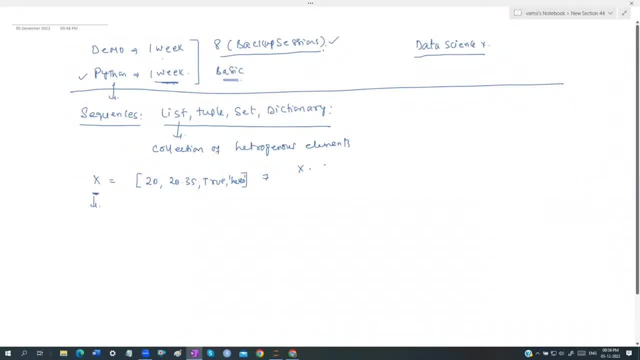 guess i am going to use a method associated with the list actually, which is going to be nothing, but i can say x, dot, clear. actually, yes, what is this clear is going to do? it is going to clear all the elements from the list. actually, yes, there are going to be clearing all the elements from the list total, the total list. 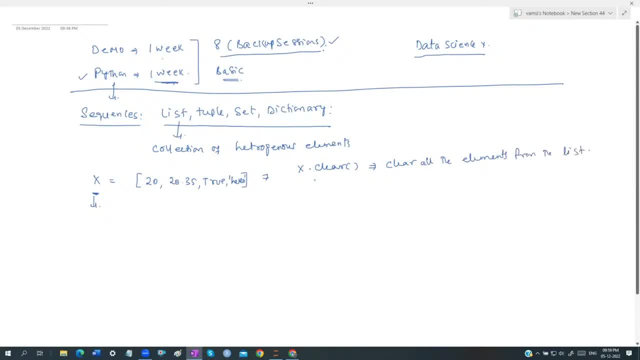 is going to be gets cleared. actually, guys, that is nothing but what we call it as a clear method, and, apart from that, i have been discussed about a method called as a count. you have to give some input value. whatever the value we have been given, it will gives you the count, the occurrence, how, 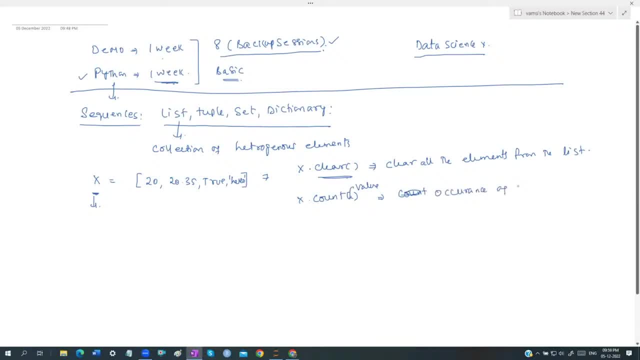 many times that particular value has been got. occurrence, actually guys, the occurrence of the value in the list. so at least i'll expect guys like who has been joining for the data science, at least they will have some basic knowledge of programming concept. so at least i expect that at least we have some 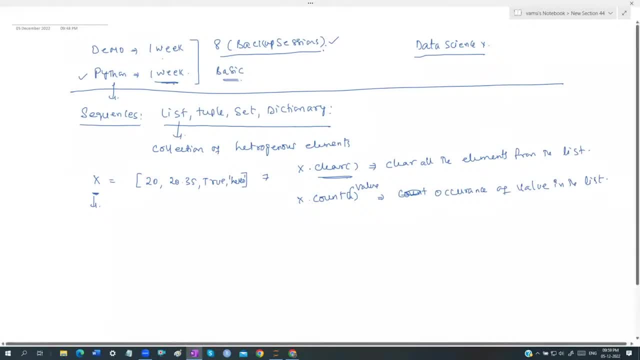 minimal knowledge of programming, so that it's a person who is completely without having any knowledge on computers. they don't prefer to learn a data science, actually, because data science is completely a little bit higher level concepts, actually same as it is. i have been told about a method called as a pop method. actually, guys, 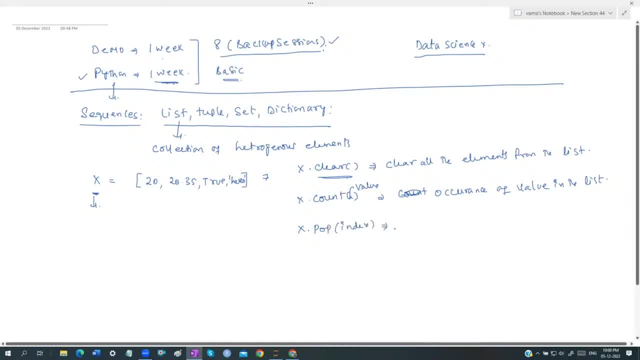 pop is going to be nothing. but what it is going to do is it is going to remove the element at the given index. normally, like other languages, index start from 0 to n, from the left to 2 right. don't worry guys, it is also from right to left also, we can talk about them, don't worry about that. 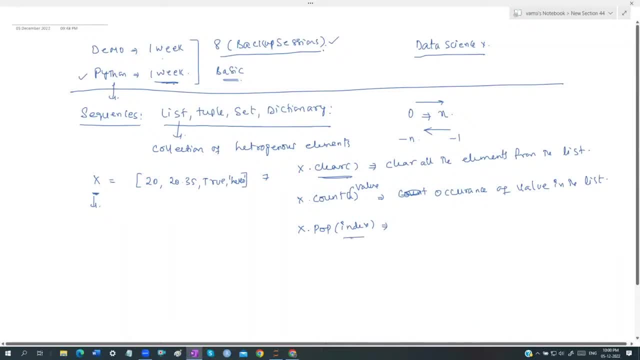 right to left index also, we can define it. actually, guys, it is indexed based. it is going to remove the element actually. yes, it removes the element at the given index, actually at the given index it is going to give. removes the element actually, guys. and then we have been got discussed about x, dot remove, i'll. 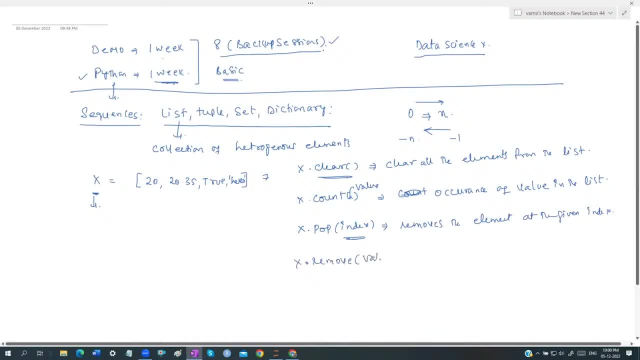 just show you once. i quickly i'll show you guys. after that you can understand the things. it is going to be value based. removes the given value. actually, guys given value from that particular list. if the value is available from the multiple um, it's going to be available for multiple times. 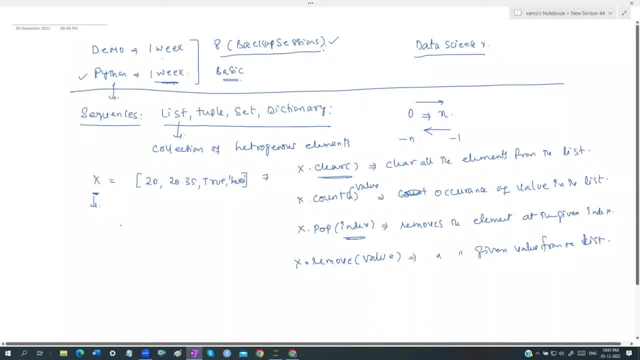 only the first occurrence will be removed. actually, guys, for example, if i have x is equivalent to: we have 20, we have a 10, we have a 20, again a 10, again a 20, again a 10, some 30, 40, we have it actually. 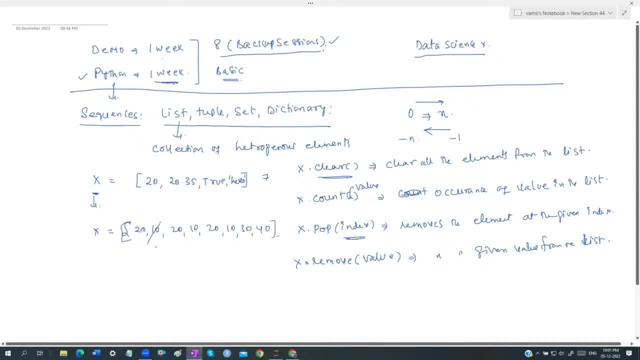 if i said, remove 10, only this 10 will be removed, but not all the 10s. only the first occurrence will be removed. actually, guys, we are completely in the beginning. concepts only, guys. i didn't started with any complicated work. actually, we didn't started with any main work. also, 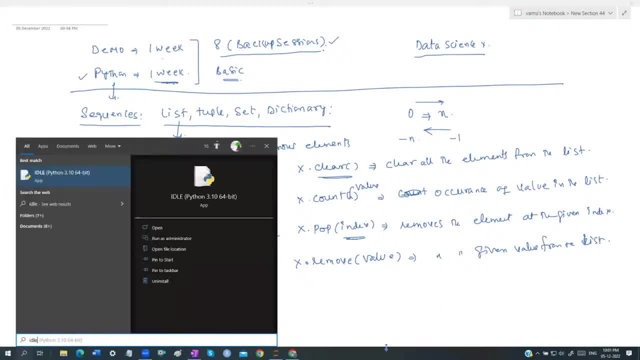 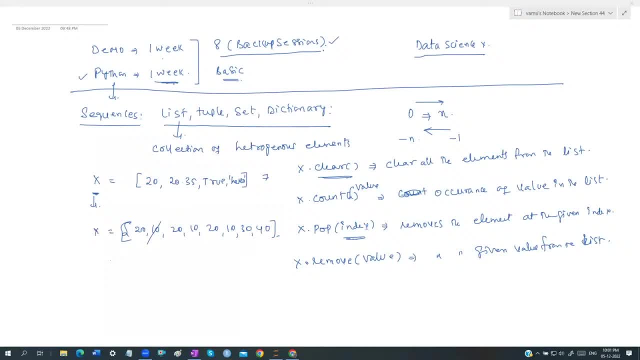 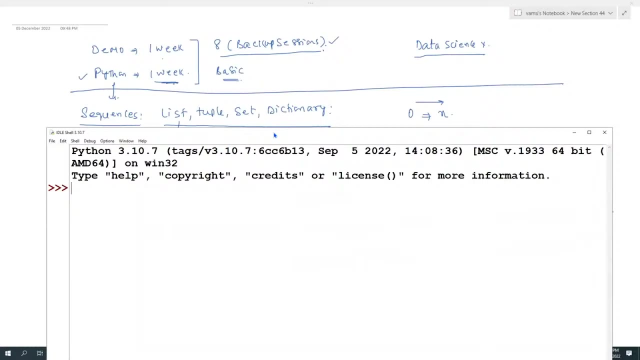 so this is going to be a simple installation of python installation. i'll show you later the backup sessions, i'll arrange the backup sessions and i will explain it. actually, guys, i'll arrange the backup session, guys, as soon as possible, don't worry about that. okay, so fine. so this is going to be what i am going to call it as an ideal. actually, guys, i'll 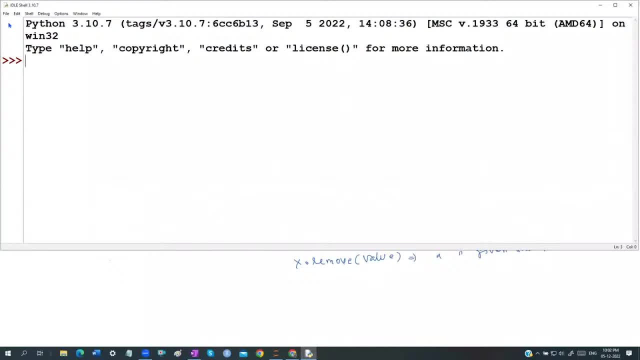 tell you about more, about the ideal which comes along with the python installation only which i have done: the python installation, along with the python installation, only i have got this particular ideal. actually, guys, you can see a prompt like this. actually, guys, we can see a pretty xc is. 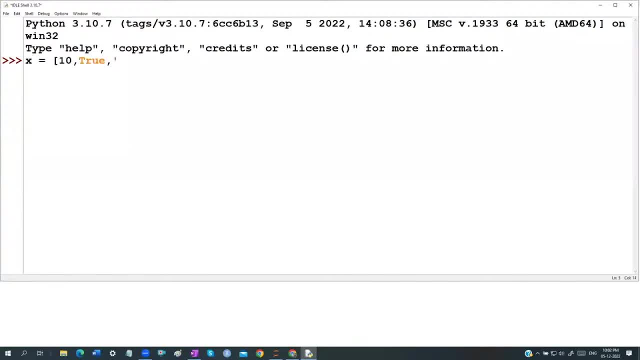 equivalent to nothing but 10, which is a true, i said, which is an hello, and which is going to be something like n 20.45. actually, guys, it's a list. actually, guys, i'll tell you all the things. guys, don't worry. just it's very simple, simple topics, only, guys. i didn't started with any complicated. 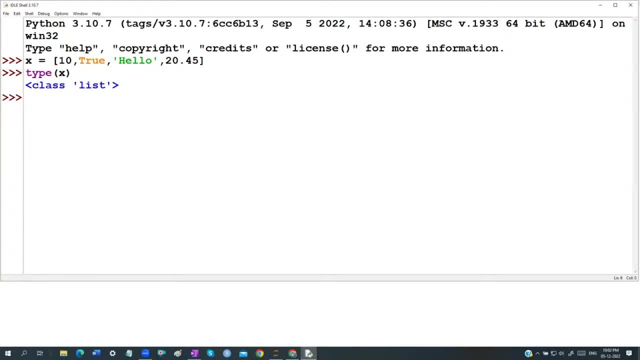 topics actually. so in like in other programming languages, we don't require any declaration part in python because python is a dynamically type of language. guys like other programming languages, you don't declare in other languages, we'll declare it. no, guys like which is going to be something like an 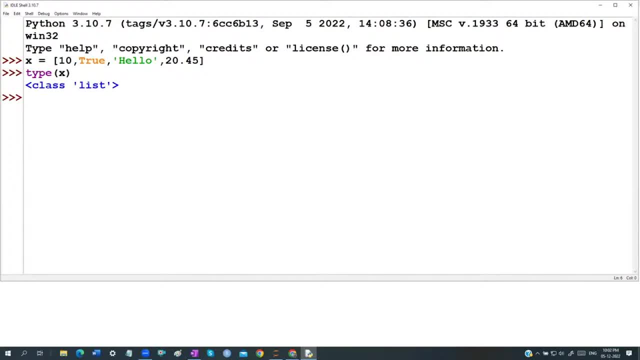 it's an integer, it's a float, it is going to be a bool. we'll do it. no, guys, in python, we don't do it. actually, guys, i'll tell you guys, it's one of the feature of python, which is going to be what we are going to call it as n. it's a python is going to be a dynamically type of language actually. 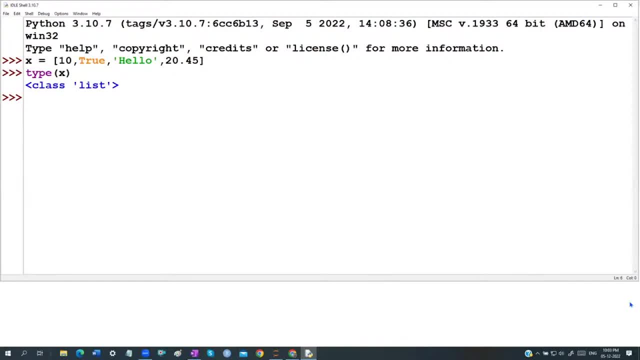 guys, python is a dynamically type of language which is going to be nothing, but no declaration is required. no declaration is required. actually, guys, like other languages, even i can work with integers, i can work with strings, i can work with bools, i can work with, actually guys. x is equal to. i said hello. 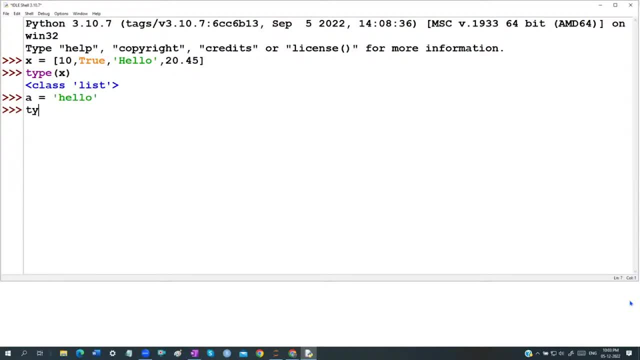 x is equivalent to hello. actually, guys, if i said what is going to be type of the a, type is the function which will tell you like what type of data type it is going to be. there got the point. so here you can also ask: what is the length? also, if i say length of the a, it will tell you like how. 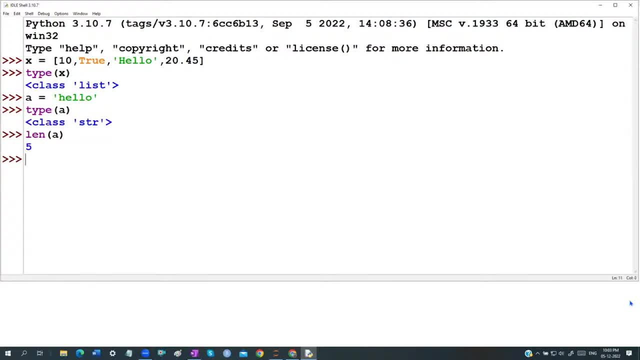 many characters are there. hello is a collection of characters. uh, string. string is a collection of characters length of x. we can say it actually. yes, it is four. so if i want, i can print the value of x. actually, guys, don't expect that like a programming language. we do it actually, yes, not. 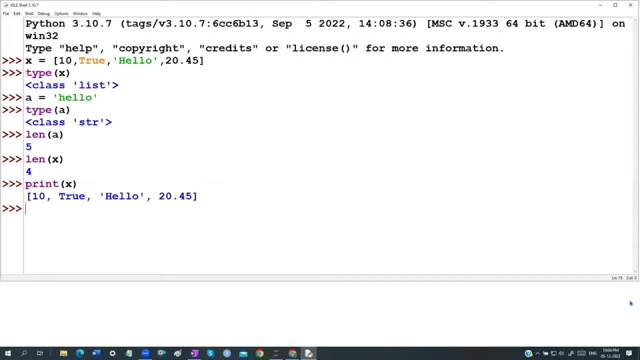 like a programming language. so don't expect, like c, c plus plus java, we are going to write a dot c file. save the file main method. come up with a dot c file. save the file main method. come up with a dot c file. compile the program. save the x. run the program. we don't do it actually, guys. simply it is going to be. 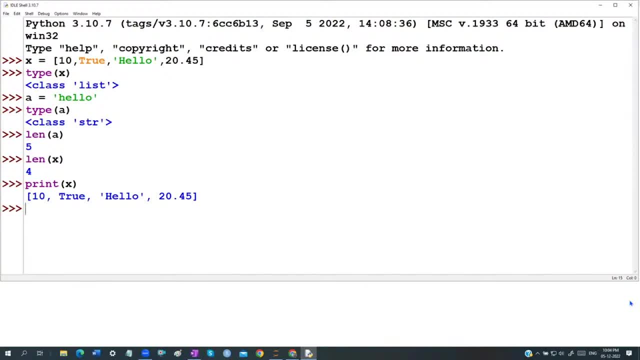 x and print x actually over. you can see it, actually, guys. so if you want to remove the elements, let me count it. actually, guys. how many times 10 was there? you can see the count. actually, guys. it was there for one time x dot count of 100. it is going to be there for zero time. these are methods, actually, guys. 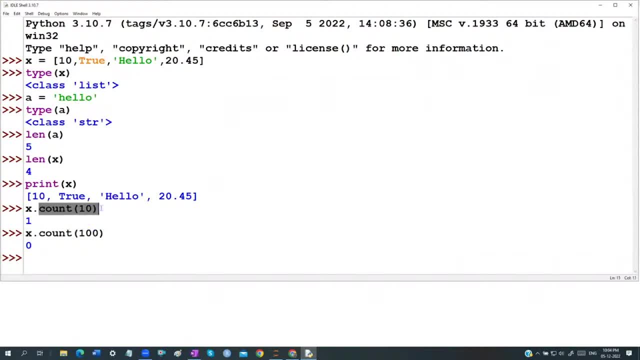 these are what we call it as methods. so the guys who are already having the idea about object about this. even if you do not have the idea, don't worry guys, i'll explain. i'll take a backup session so i'll complete off that x dot count of 100. actually guess 100 is not there so we can see. 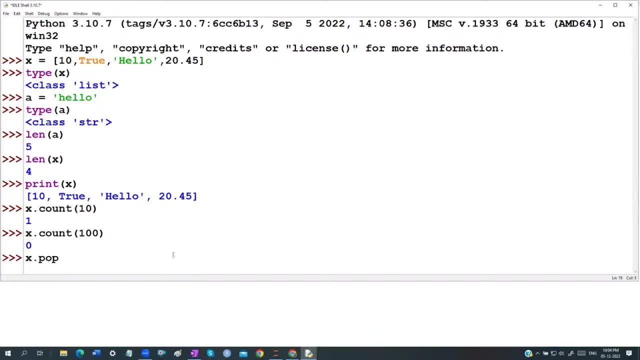 the zero value. i want to remove the elements. actually guys. x dot pop pop is basically based on the indexed base. removing actually guys index base means which one? zero, one, two, three. like this, we can specify that zero, one, two, three. even we can write in reverse order: actually guys, this is. 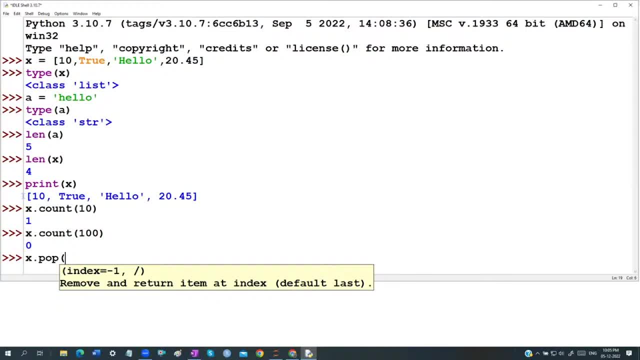 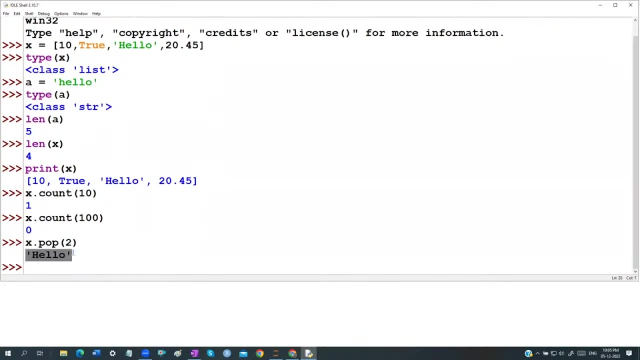 minus one minus two, minus three minus four. it is from left to right, right to left. index. is there? if i said x dot pop of two, actually, guys, the second element will be remote. second index: zero one, two, hello will be removed. actually, guys, it will tell you, like, what value has been removed. also, it is going to tell you: don't think that it. 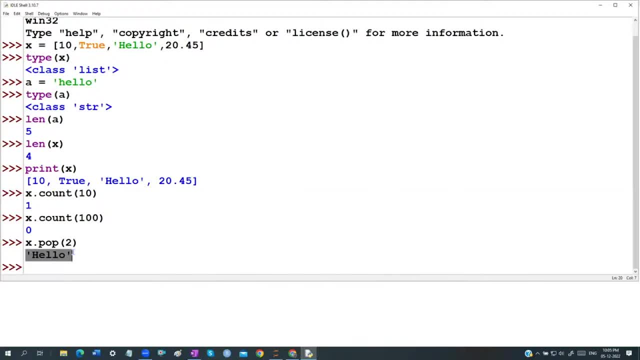 is only returning the date. actually, guys, that particular 22, the element that 2 has been removed and written the value actually. so now, if you can see x, you don't see the hello. actually, guys, previously, the length of the x is going to be. the length of the x is going to be. the length of the x is going to be. 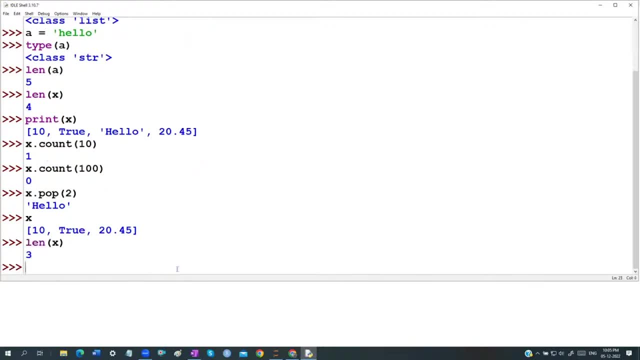 four. but now i can say length of the x is equal to three actually guys. why? because you can see one element has been got removed. so pop is basically on the index. if i don't specify which value we have to remove, it automatically removes the last element. actually guys it automatically. 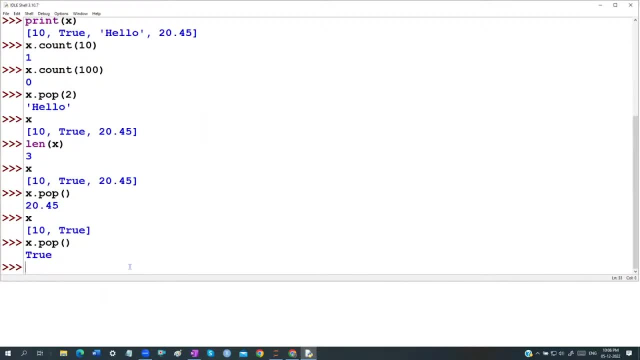 removes the last element. x dot pop: it removes the last element. actually, that is going to be what we are talking about: the pop method. once again, i will create it: 10, 20, 10, which is 30, 20 again at 10, 20 again at 20, 30, whatever you want, we can give it actually no worries. now i can say: 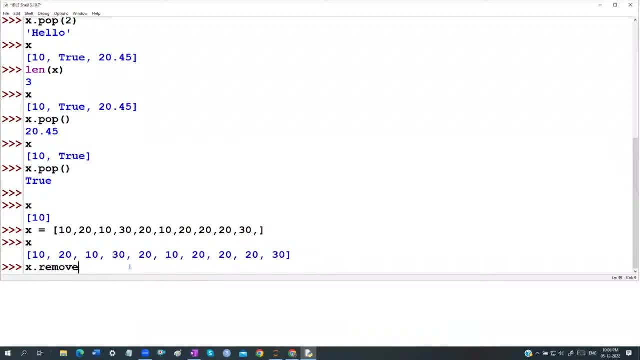 x dot which is going to be remove. remove is not based on the index guys, it is completely based on the value. if i say remove of one, you will get an error actually why? because one was not in the list. index pop will can do that actually, but remove can't do that because remove is value. 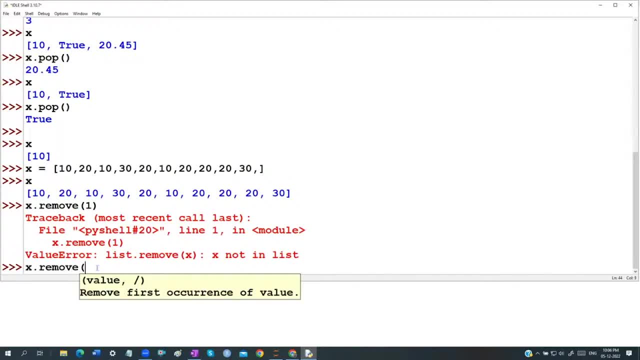 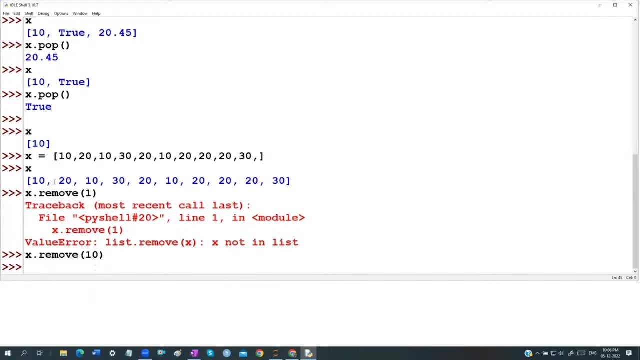 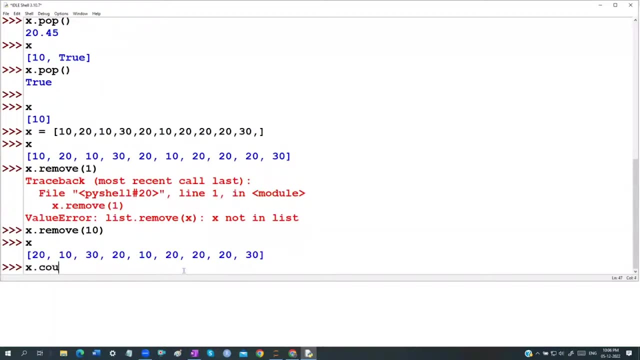 based. actually, guys x dot. i said remove off, which is going to be 10, only the first occurrence of the removed. it won't remove all the tens. one, two, three tens are there. so out of the three tens, one ten has been got removed. now, if you want, we can count it. actually, guys x dot. count of 10. 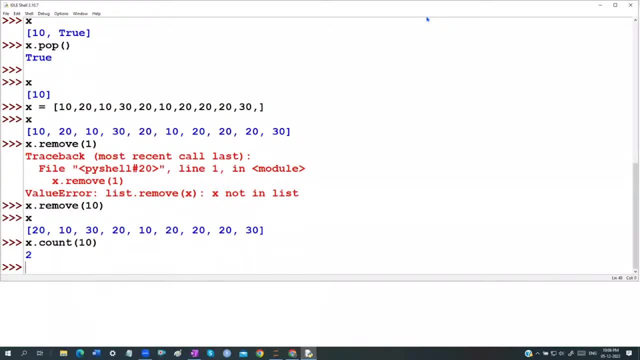 we can see the result is going to be two is the result what we can see? it actually okay, so something like that. we can see that. so these are the four methods i have been got discussed actually on saturday. uh, very few guys has been joined, only three people has been joined. 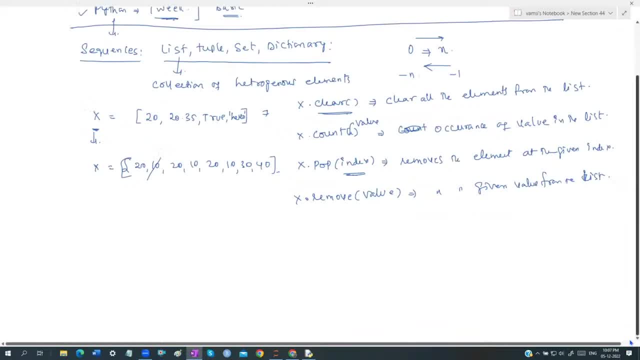 and what i thought is it may be an important, uh um class. so i didn't taken the class on the saturday, i cancelled the session, but for next week i don't do it. actually, guys, actually some of the guys said that, sir, let us give the recording. 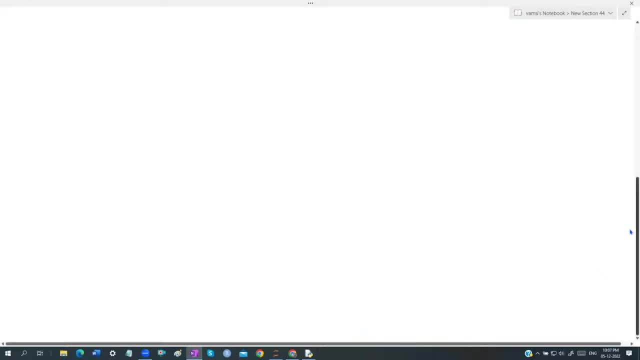 session for them. but i have been excused, actually because it's an introduction classes, no beginning classes. if you miss the classes, you may not understand the topic. that's why this week i have been given the excuse. guys, from next week, uh, even if the if the number of attendance is going to be, 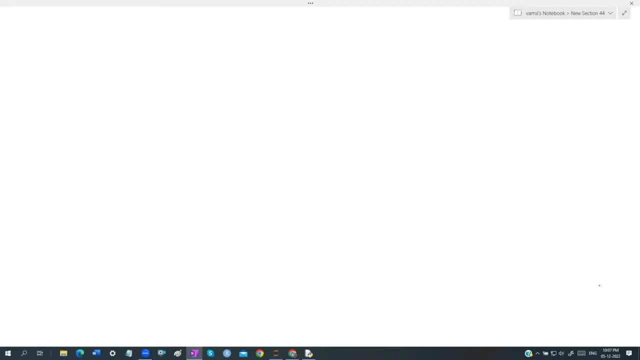 very low also we'll. we'll take up the class and those recording sessions will be very low also. we can. we can take it and we can understand the recordings actually. so on saturday we didn't take in the class due to some less participations are there. so today we'll continue with the same class. 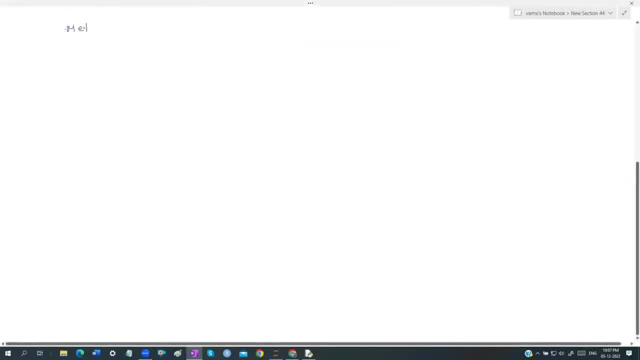 actually, guys, so totally how many methods we have been got discussed. guys, we have been learned about four methods. one is going to be nothing, but i i discussed about a clear. the second one is going to be nothing, but we discussed about a count and we discussed about a pop method and we have been 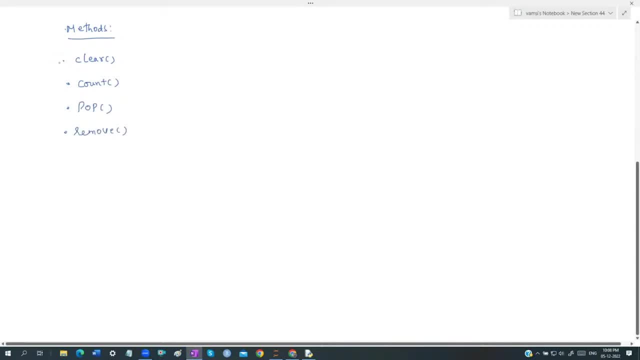 discussed about a remove method. actually clear, pop and remove almost all. all the three are using for the same purpose. actually, we are used for removing the element from the list. clear will removes all the elements. pop is going to remove the given index. pop will remove the element from the given index. 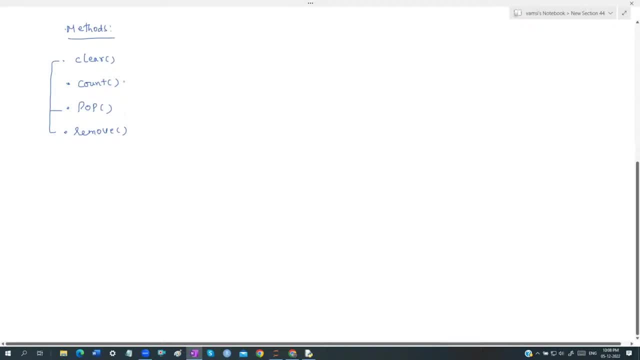 remove is going to be removes the first occurrence of the given value. count is not doing any removing or adding. it is going to be completely only for counting, actually guys. so today i'll tell you about another three more methods. actually total 11 methods. are there actually guys? list is associated with 11 methods, as i told you, except copy, copy. i'm not going to. 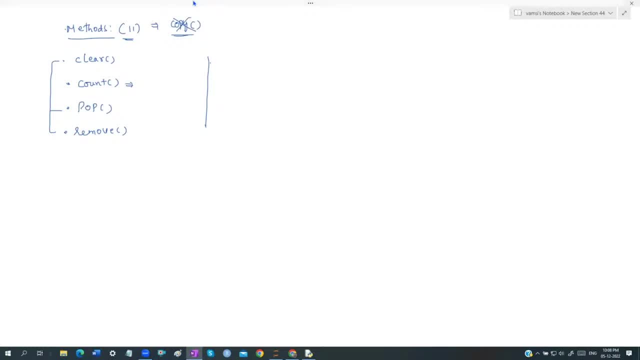 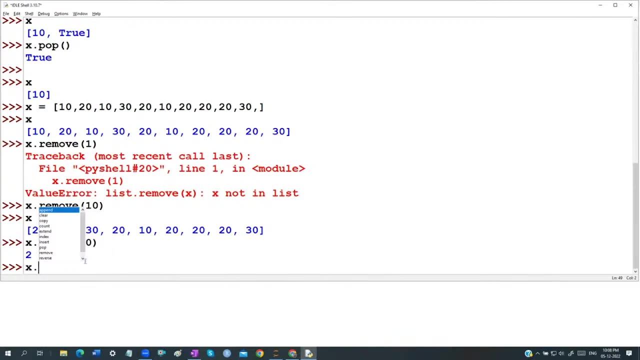 discuss now. copy is a method you need, not to. i told you nothing to hide from ugr s. i can't hide anything from ugrs because you can see it actually. yes, can you see x dot? when i said x dot, automatically all of them will pop up. actually, yes, all of them will automatically pop up. i don't do. anything. actually, guys, if you want i can, i can zoom. no to zoom in or down that my this is, and then when i know normally don't see that so i don't have to focus too hard on one of them, but you can, yeah, if you don't customize. we are going to look at like this: is the open high spec bySimple matrix like this, all right, and here you'll see that scd 30 is not. 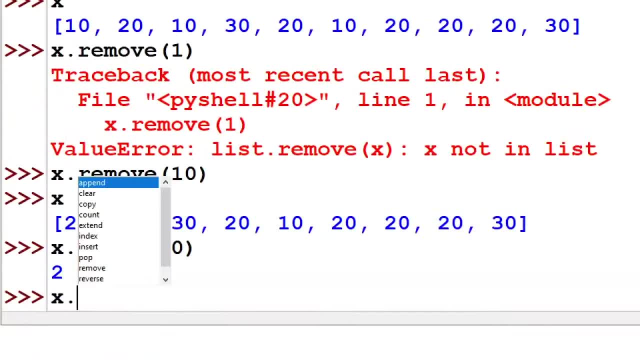 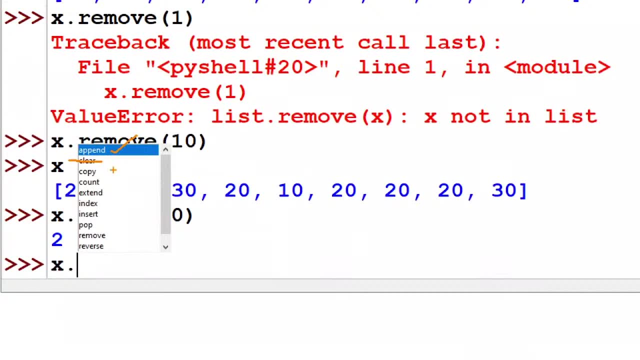 i can show you actually, guys. so there is an append method, is there actually? i discussed only clear copy. i said that i don't discuss it now. i'm not going to discuss it now. count, i have been got discussed. pop remove: i have been got discussed actually, guys, totally, there are 11 methods. are 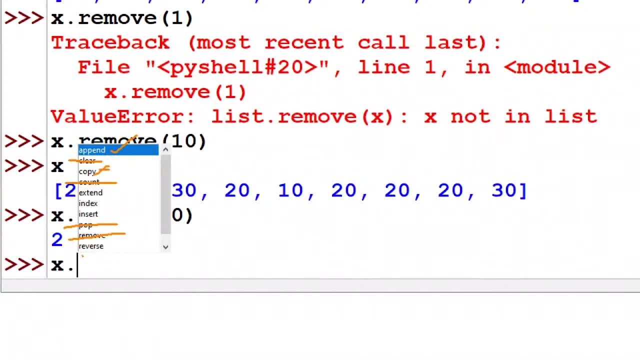 there. there is a one more. is there actually a sort? is there at the bottom? we have to scroll it down. we have to scroll it down. you can see a sort at the bottom. totally if you count it guys, 11 methods will be there. actually i don't discuss the copy because copy cannot understand now itself. so 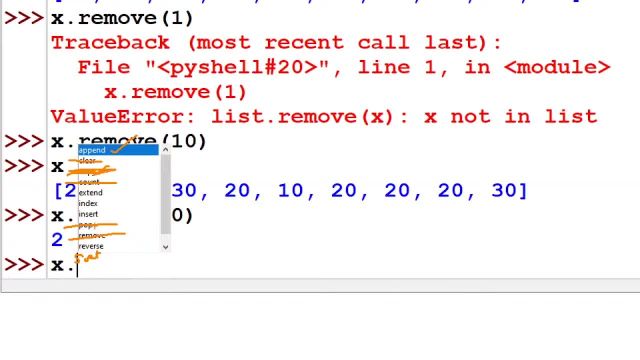 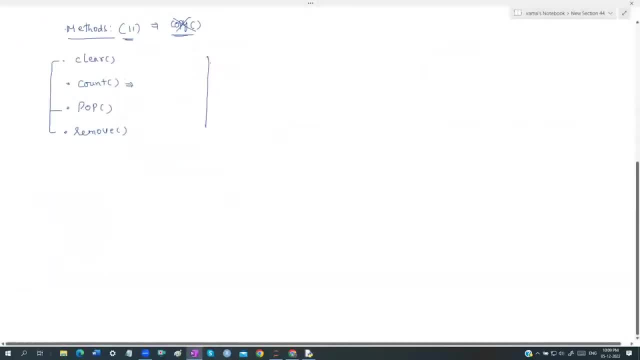 remaining. out. of that particular remaining 10, we already covered four. still we have a six methods are there? slowly, i'll discuss it, guys. now i'm going to discuss about another three more methods. actually, guys, one is going to be append. the other one is going to be a method called as an extend. 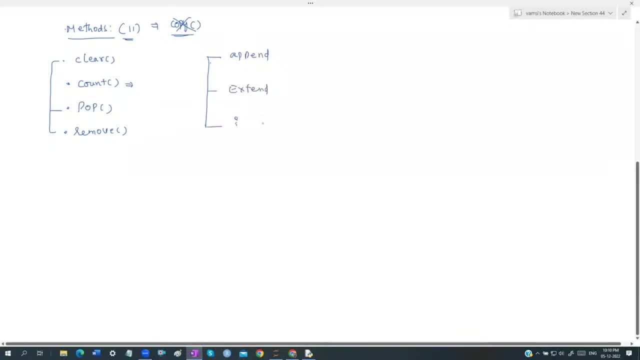 and one more is going to be what we call it as insert guys, totally, there are three methods. are there you? they are a little bit similar. that means they are not exactly the same guys, they are little bit same same cons. the same concept will be there. basically, these three methods are basically: 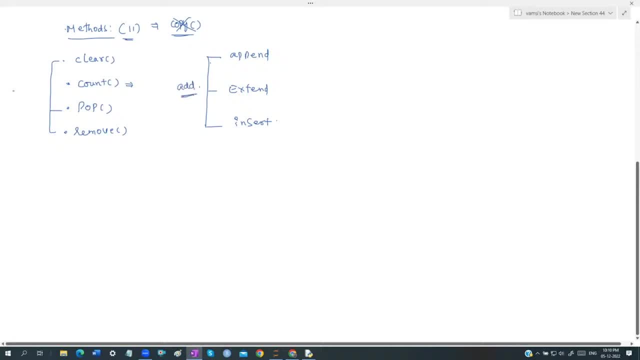 to add the elements actually, guys. clear, pop and remove. what they will do, guys: they will remove the elements. they are going to remove the elements actually, guys, whereas this append, extend and insert, basically they are used to remove the elements actually. yes, they are going to be basically. 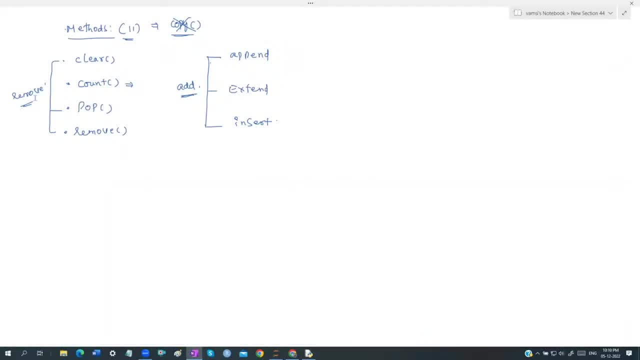 used to remove the sorry append, extend and insert. basically, they are used to add the elements actually. yes, they are basically used to add the elements. so all the three will do the same thing, but it's a slightly difference. it is going to do actually, yes. so, guys, who has been joined for the? 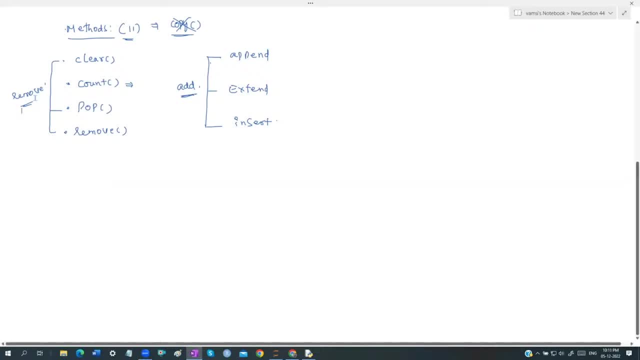 today's class. hope you can able to follow it. actually, even you have not joined from the beginning. they are very simple. i created a list. now what i did is i am just remove. i removed the element from the list. now i am going to be describing the elements and i am going to be 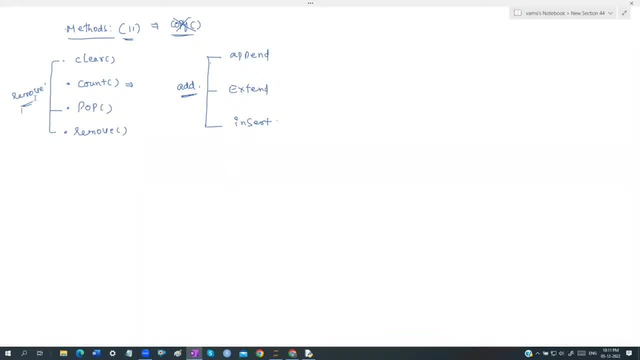 discussing about how to add the elements to the list. actually, guys, the names are very easy: append, extend, insert. almost all the three are telling the same thing: append, you can append the elements. extend, we are extending that. you can, you are extending the- uh, the list, actually, guys, by. 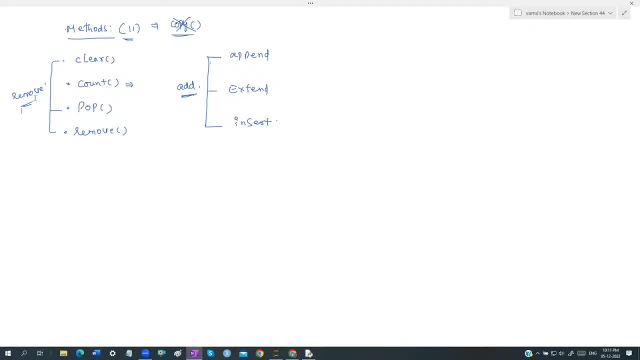 adding some elements actually and we are inserting the elements actually. and what is the difference between all these three actually, guys, let me explain you. append is going to be because we are. some of the points may not be gets connected to you. it will take some time, slowly, step by step. 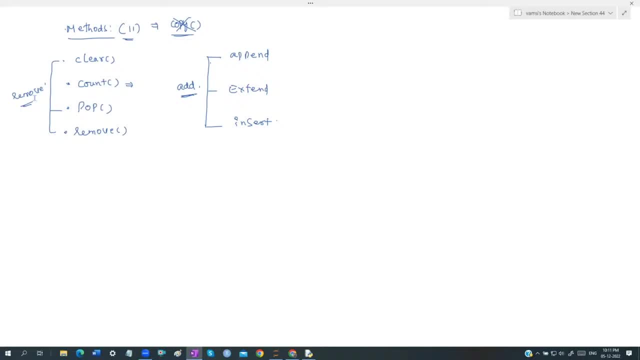 step by step. i'll explain it actually, guys, slowly, step by step. i'll explain it, not at the same time. we cannot understand it actually, guys. okay, simple to understand. append is going to be nothing. but easy to understand it actually, guys. append is going to be takes an input as an element. what? 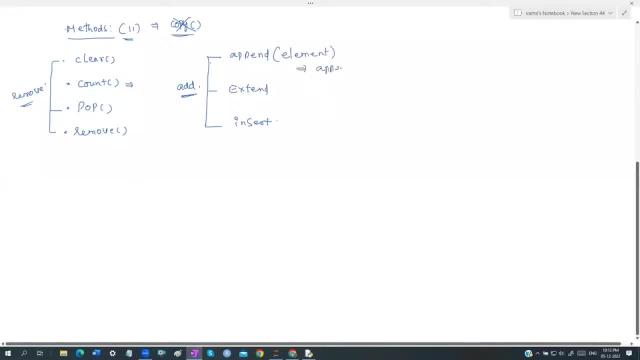 is that append will do, actually, guys. just it is going to append the element. it is going to append the element to the end of the list, actually, guys, to the end of the list. actually, it is going to be appends that particular element to the end of the list if list is already having five elements. 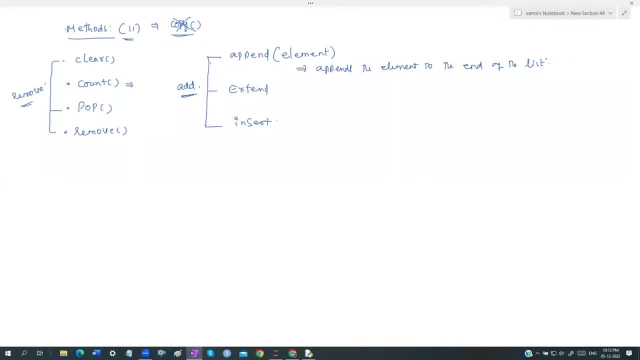 the new element will be appended only at the six. you know, already know what is appending append mode. actually, guys, you cannot add wherever you want to add it. we can not add wherever you want to add it actually. yes, it will be added only at the end of the existing. 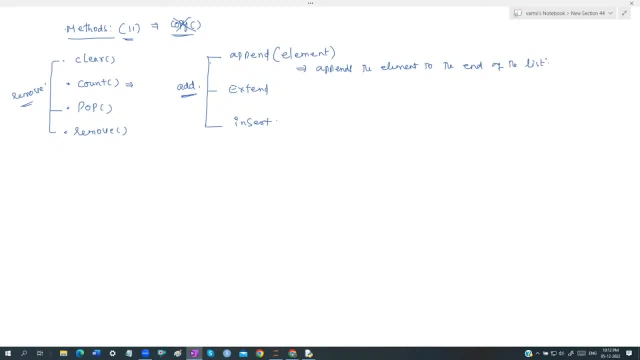 elements only it will be added. and one more important thing: i told you, guys, most of the methods won't return anything like, for example, talk about a clear method, guys. when you said clear, it won't return any output. whether it is cleared, whether it is not cleared, it won't return. 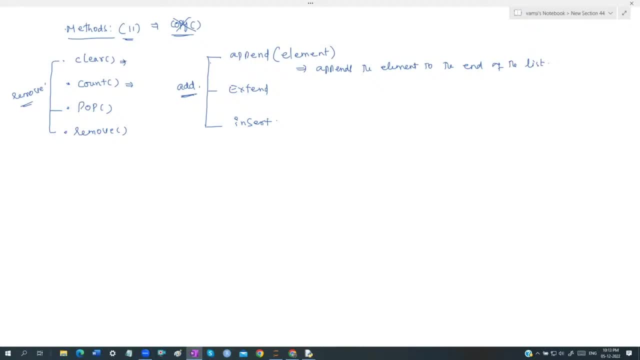 anything to you. if you want to verify whether it is cleared or not, we have to go to the list and we have to verify that. then only we'll come to know that, okay, these elements has been got cleared from the list. count is going to returns of element. actually, guys, count is going to returns an element. 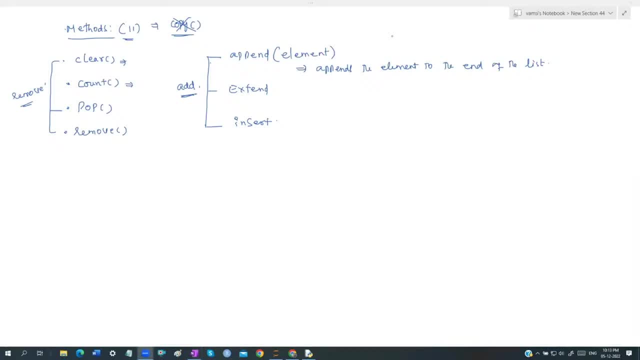 yeah, i'll explain it then. okay, fine, i'll explain it. so the pop and remove is going to be nothing, but if you don't mind, if you don't mind, uh, who is that participant name, right, murudula, right, just give me a second. yes, i think, murudula, right, yeah, murudula. do you have the idea about the basics of python? do you know? 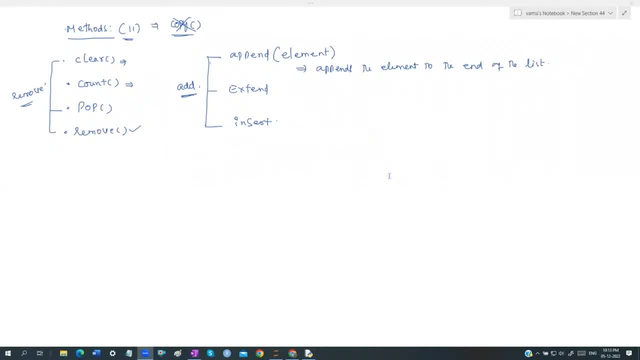 about the list. you have the list, okay. so, um like, do you know the indexes? so see simple example: it is 10, 20, 30, 40, 50, okay, so you know the indexes. no, this is 0, 1, 2, 3 and 4. is the indexes actually. 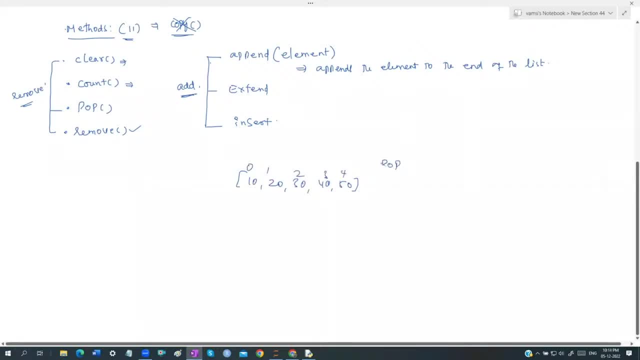 okay, pop is basically. pop is a method which is basically used to remove the element based on the index. so if i say pop 2, it will remove this 30 and it is going to return. so it will return 30 as an output to you. it's not giving the element, guys, it is removing and returning the values. 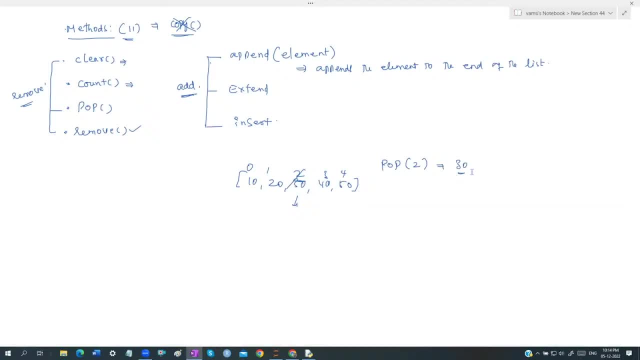 so 30 will be popped out, it will be sent out. so pop is basically used to remove based on the index. remove is nothing bad. i cannot say remove is completely based on the value. if i say remove 2, it won't remove. actually, guys, remove 40, then 40 is going to be removed from that particular list actually. 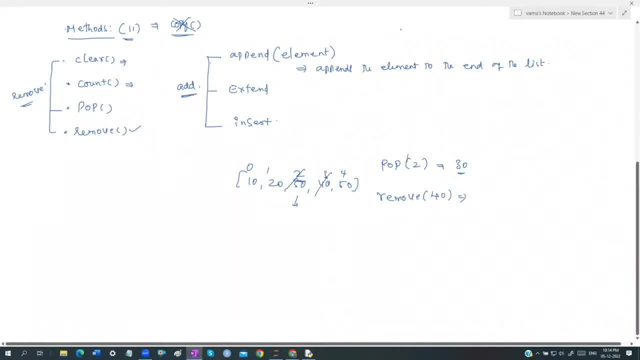 index it base and value based. yes, it's a base. remove is based on the value based. it's a value based. whatever the value we have been given, the value will be removed. so your question is like: if 40 is there for multiple times, then what? what will happen? actually, only the first occurrence of 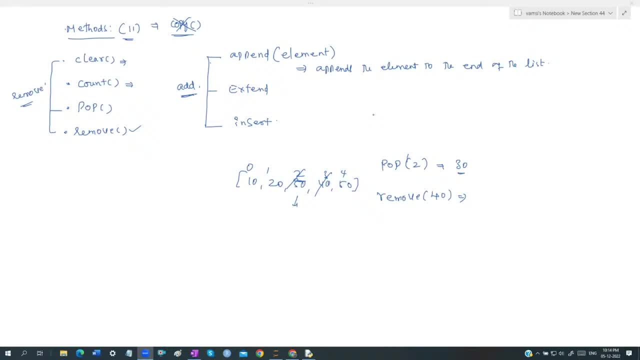 40 will be removed, but not all the forties. got it right. fine, okay, thank you, fine, thank you, guys. so that is about the pop and the remove method. okay, appends the element to the end of the list and, coming to the returning value, count will return. 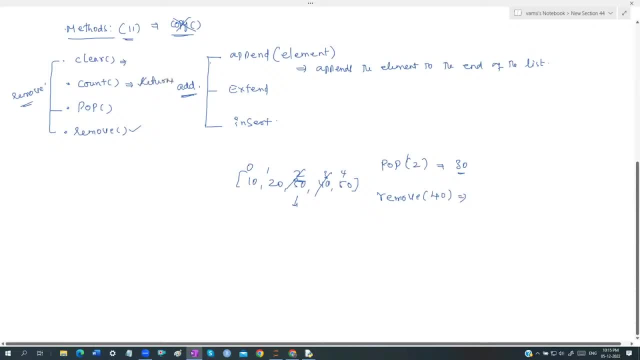 some value to you, guys. i'll conclude all the topics. guys, i'll conclude all the topics actually count will return. pop also returns, actually, guys. pop also will return you the value, which value it has been got removed. it will return it, actually, guys, but clear and remove won't return. 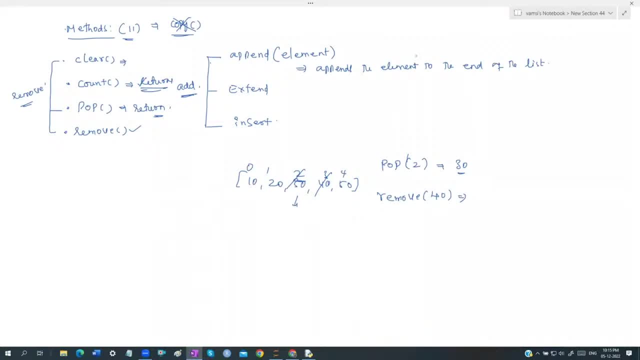 anything to you, not not only the clear and remove guys. even append also won't return anything as no return. extend won't return, insert won't return, sort won't return. none of the most of the methods. they don't return anything. yes, if you want to really know whether that action has been taken place. 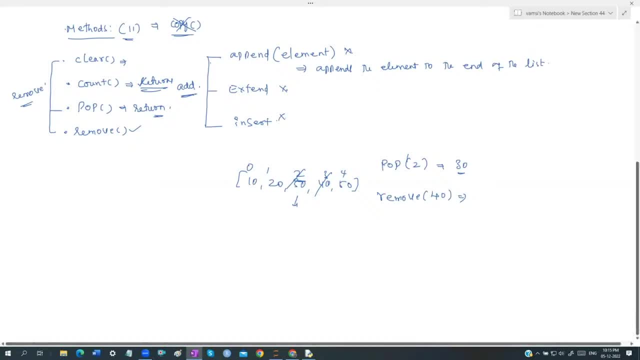 or not. you ask it for appending. you ask it to append some element, so element is appended, but it won't tell you any information. i sucks, i appended, i didn't depended. it's an error, nothing. it is going to tell you if there is any problem. it will tell you that there is a problem, is there? 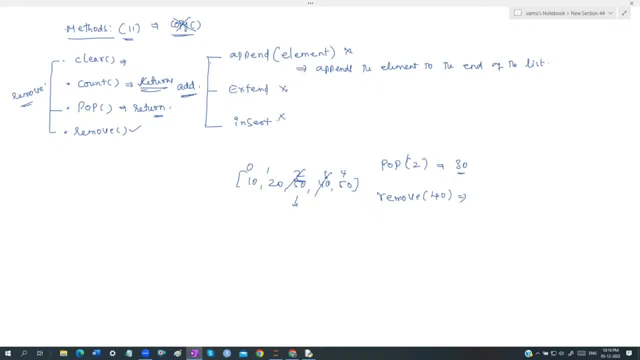 but in the case if there is no problem, it simply sits silently. guys, the method will sit silently. they don't intimate anything to you. so i have been done. i didn't done anything. it won't tell you anything. if you want to really check out whether that action was done or not, you have 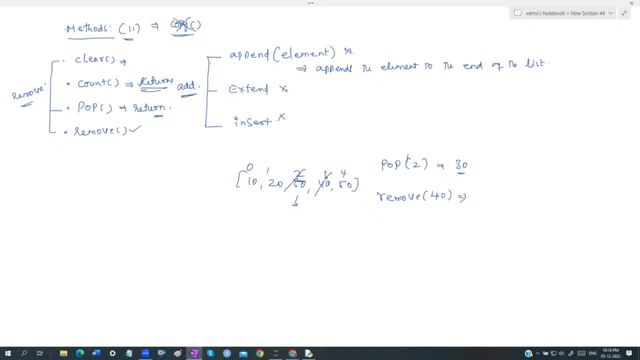 to go to the list and we have to verify it. actually, yes, this is appended, this is not appended, something like this actually, guys. so very simple technique, actually, guys. take some list, take some list, actually, guys. i said x is equivalent to nothing, but i said some elements. 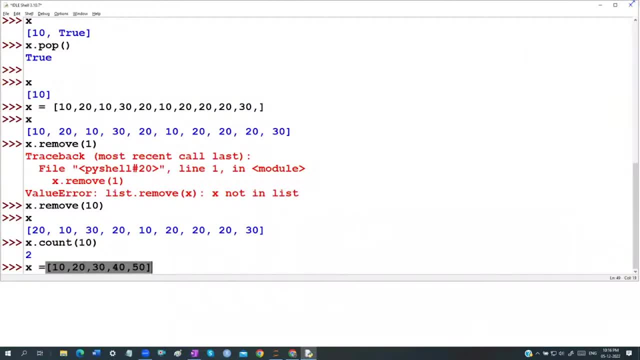 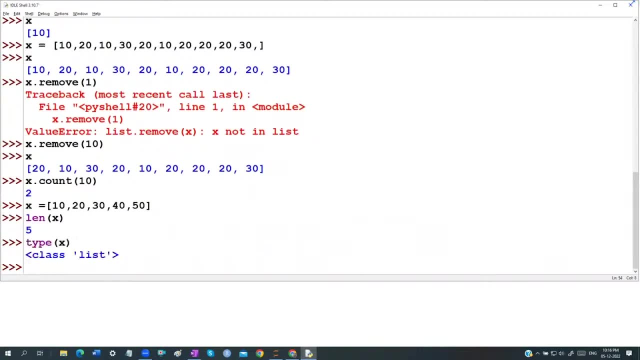 so easy to understand. i'm taking a sequence of elements, guys. apart from that, nothing is there. so what is the length of the x? what is the type of the x? then this phi and type is going to be x, which is going to be class list, which is going to be nothing, but it's a class list actually, guys. 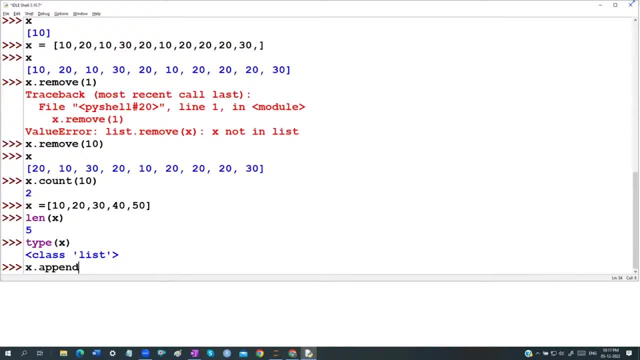 so now i'm appending: actually guys, x, dot, fn. everything is documented. actually, guys, everything is documented. so you guys, it is automatically showing you, like, which is going to be object. append the object to the end of the list. if i said 60, actually, guys, it is automatically. 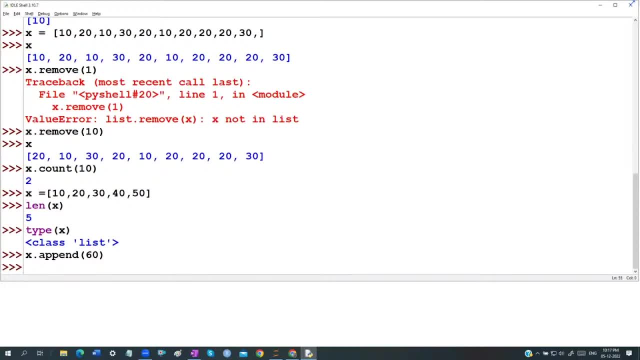 appended the 60. but see, don't expect that, sir, we'll get the string as the list, as an output, with that particular append at 60.. no, it won't give any output, guys. the output. you can see the result actually then. only you can see the result actually. yes, 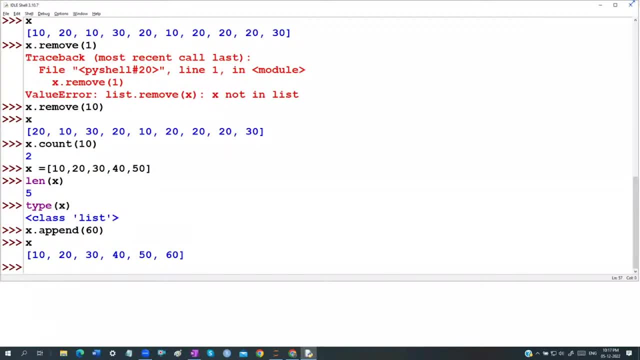 it won't return anything. whether i appended, i didn't appended nothing. it will tell you in some situations we don't know whether it is done or not done, so we have to verify it. really it has been got done or not. see the difference. but type won't change this actually, because type 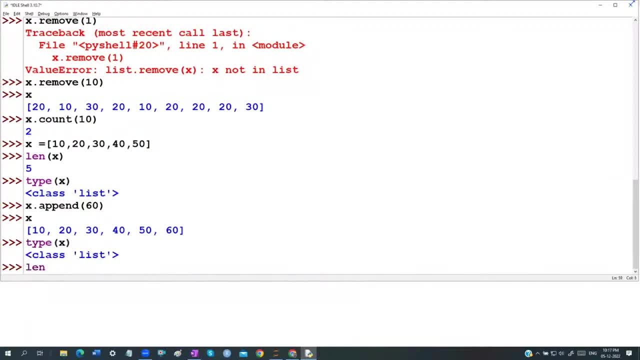 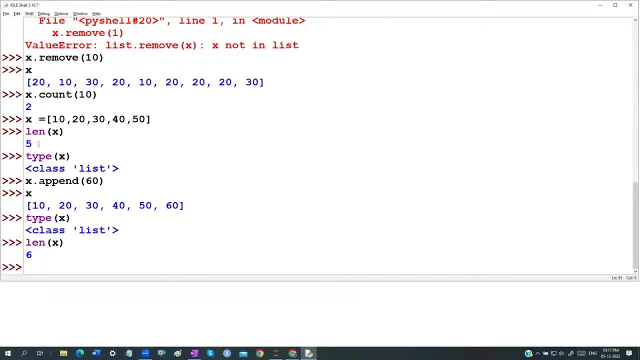 of the x is going to be still a list, only. what is the length also is going to be nothing, but it is going to be six very clear guys. earlier it was five and now it is going to be nothing, but it is going to be six actually guys. that is what we can see as of this particular difference we can 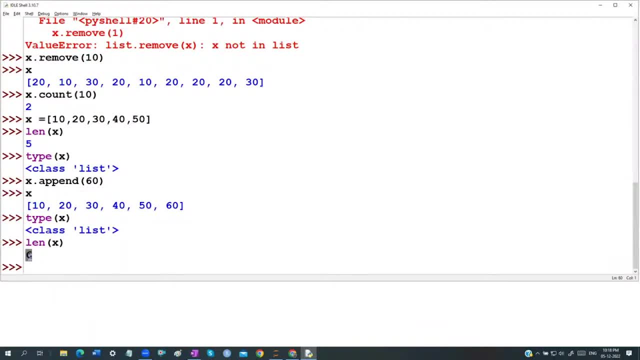 find it. what the point, guys? so it will always append only at the end of the list. you cannot append wherever you want to append it, actually, guys. so i want to append it to the first index, or if i want to append at the second index, that is not possible. that is not possible, actually, as 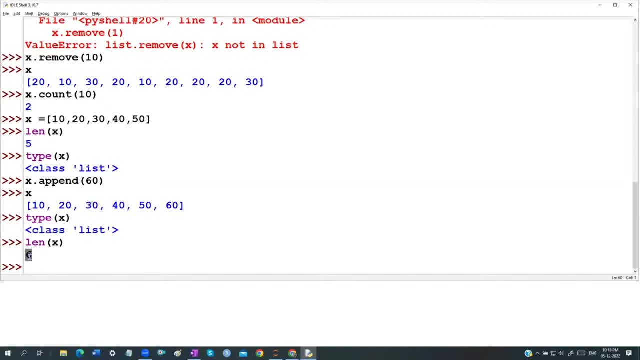 by using append method. if you want to do that, we have a other technique. is that again, i'm going to do the same thing? actually, guys, let us say which is going to be x dot append of. i said 70, actually, where it is appended. don't think that it will happen. always alphabetically, guys, no alphabetical order. it will. 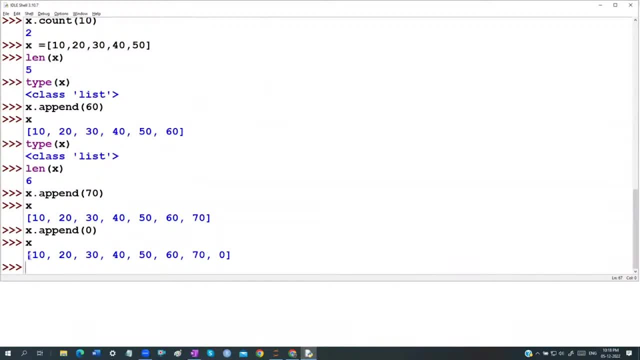 actually, or it is not only in ascending order only. so like, zero is going to be appended at the beginning, 80 is appended at the last. it won't do like this. actually, guys, whether the data is sequential or random does not matter. append is always going to append the element only at the end of the existing list, not at the beginning or not. 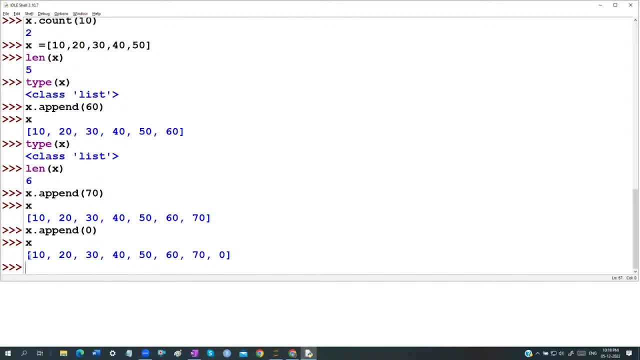 at the middle of the list. actually, guys, can you see zero has been appended at the last actual. the length has been increased. i think now it has been became eight. length of the x has been became eight, actually, guys, because we added two elements after the 70, so 70 is appended and then zero is. 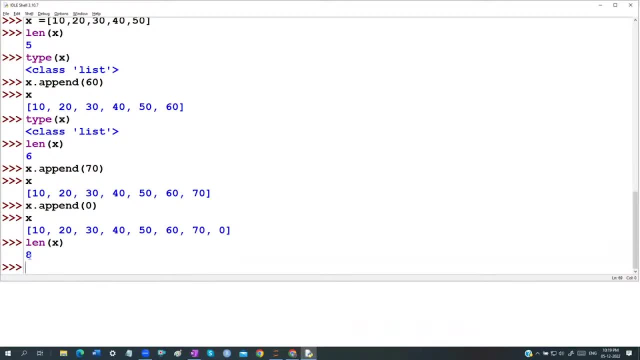 appended two elements we added now after 60, so it has been became eight elements total, it has been become eight elements. okay, if so, you can add up the elements, you can remove the elements, whatever you want. guys, you can do it actually. okay now. so next explain. next, let me explain about this. 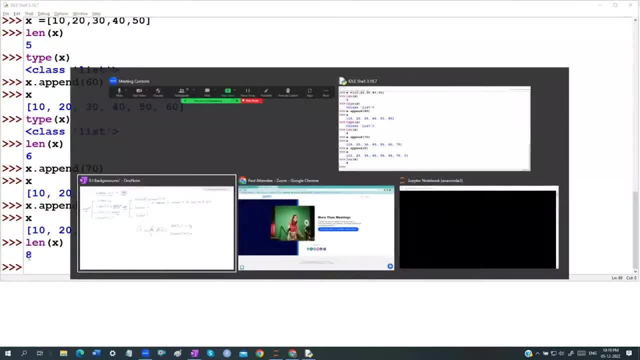 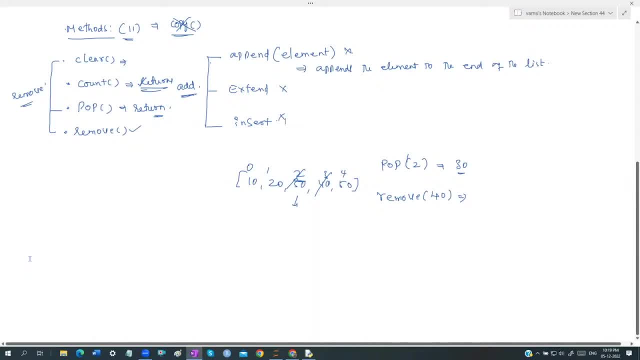 particular method called as an insert method. so maybe you understood the append method actually, guys, but some methods may be a little bit confusion for the guys who has been joined for the today's class, because you may not be having about any idea about indexes but nowadays, guys, everybody is learning python. everybody is learning python. everybody is learning python. 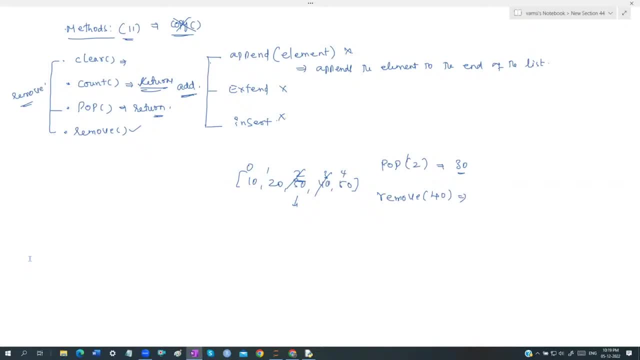 everyone is having a little bit core concepts of python, may not be having a complete knowledge about the python, but nowadays i can expect that whoever is learning- whether they're learning java, dotnet, etc- first of all they're learning python actually, guys. so i don't think so you guys may. 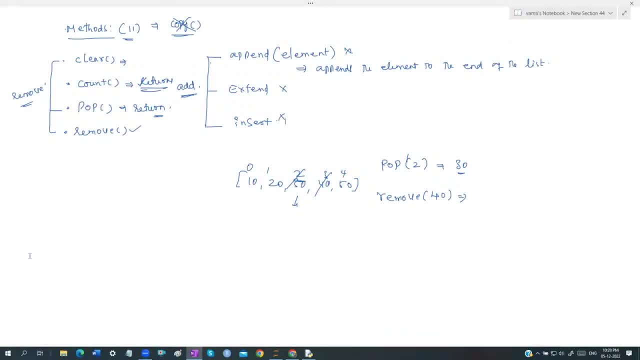 be having some difficulty in learning python actually, but you can. maybe some guys may not have the complete idea about that, but still they can understand this particular concepts actually. so now i have a method called as an insert method. is there actually, guys? i'm explaining insert method, not the extend method. 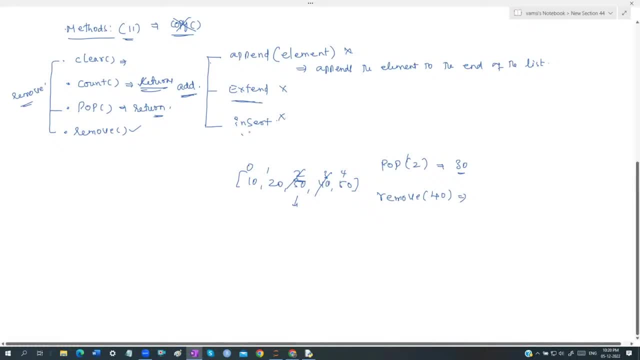 let me explain with the insert method. what is the insert method we'll do? actually, insert and append is the same same, same only. but only the thing is, insert is a method which allows you to add the element wherever you want. that means it will take two arguments, actually, guys. one is going to be the 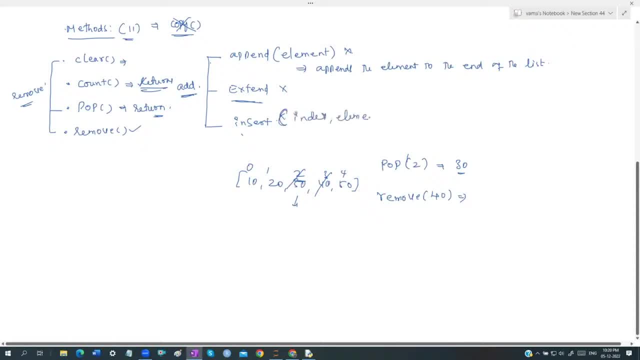 index it will take and it is going to be a insert and insert the element. now, this awesome method that allows us to think of our whole x cell size as an after saying the market at one point and earn at all of that point max on growth as an after we achieve good results and it will give us the star value. 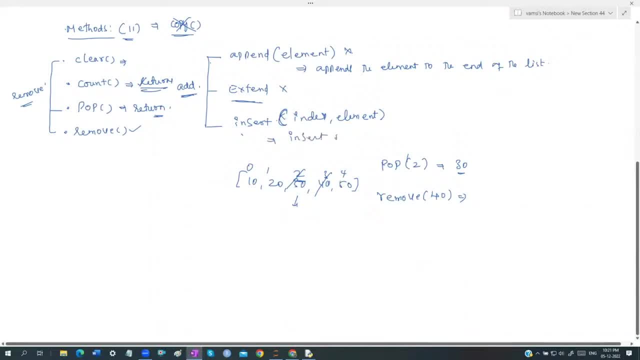 as thrust could always change. so it will give you some strength. so, yes, this is an example how it will give you some response time. to divide the X- T as auxiliary on uh, you want to add the index in the nature of the index, because the greater your index area, the higher. 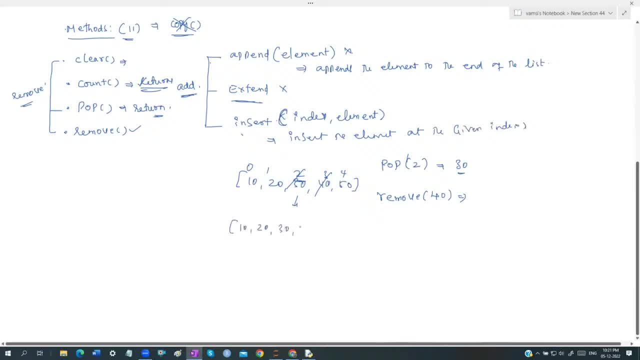 your use it over and other things that actually may be happening in this side and the way of addressing it is much simply hosted in western order. Umm Hi, good morning, uh, ok, 40, 50, for example. now i said let us say x equals to s. if i said x dot, i said insert, for example. 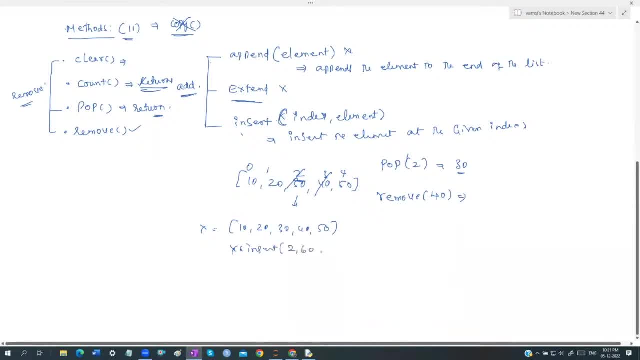 if i said 2 comma 60. actually, guys, one important thing: actually, guys, 2 comma 60 means it is 0, 1, 2, 3, 4. now don't think that that 20 will be replaced by 60. actually, guys, it's not replacing. 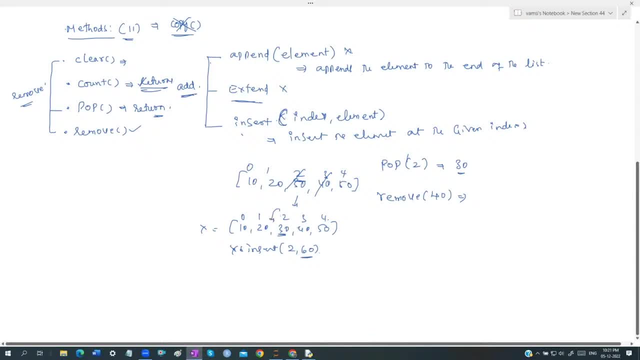 here, before this 2 index, that means, at the second index, it is going to be inserting 60. actually, guys, you are not replacing. then what happens? we know that, actually guys, if this becomes 2, this becomes 3, this becomes 4, this becomes 5, actually. so wherever you want to add, we can. 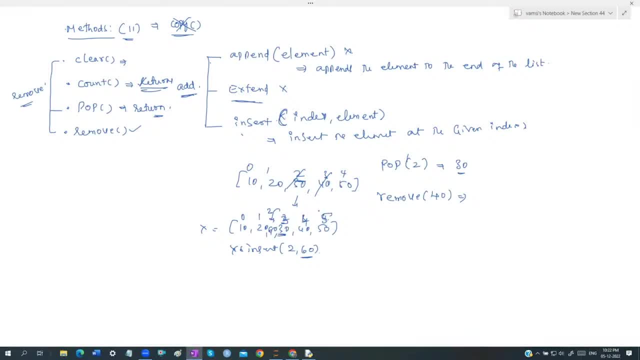 add it. actually, guys, we are not replacing, you are not replacing the second index with 40 x 60. actually, guys, before the second index, you are adding 60. that means the previous second index will become third index, before third index is going to become the fourth index and before the fourth index. whatever the 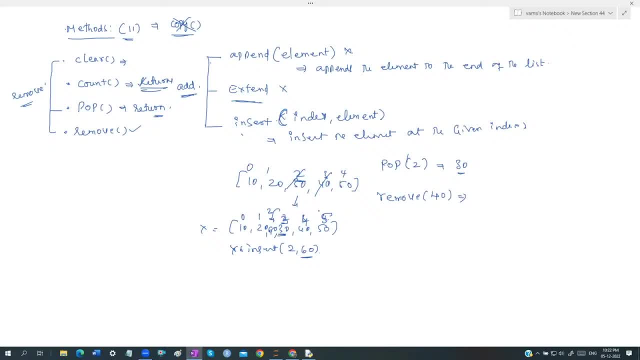 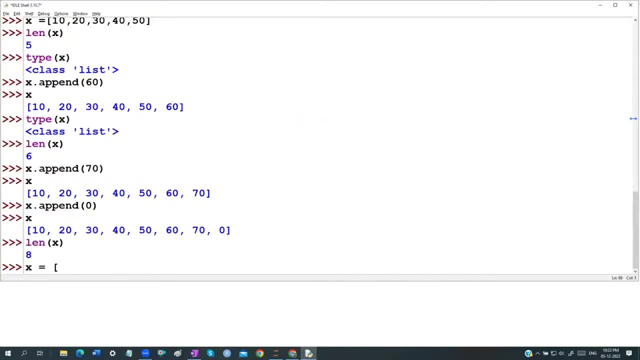 earlier fourth index is there. now it will become the fifth index. actually, guys, that is what we are going to call it, as this technique, what we are going to call it as in the insert method. actually, once again, 10, 20, 30, 40, 50, length of the x which we can see: 5, actually, guys, i said x dot, which is 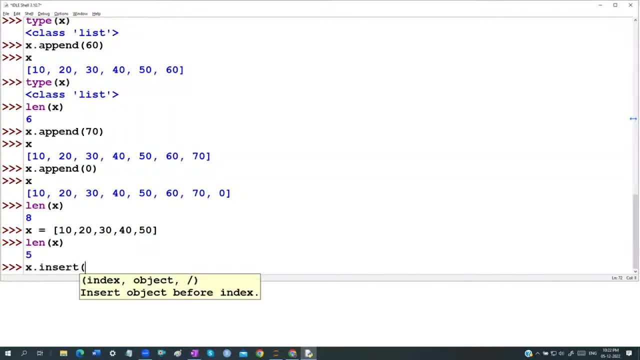 going to be insert of something like: can you see, guys, everything is going to be given the help. actually, guys insert the object before the index. if i sets 2 comma, which is going to be nothing, but it is 60, that means before the second index, it will insert the 60. actually, who is the second index? we know. 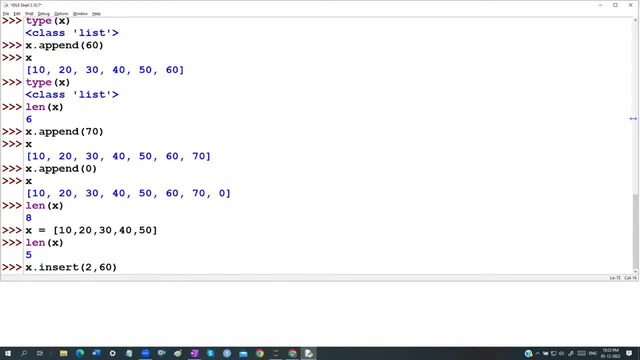 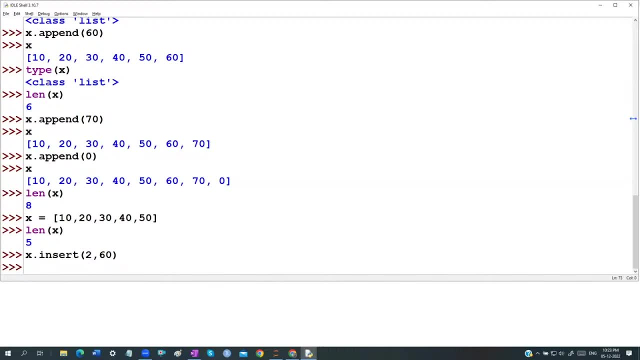 this: actually guys. 10, 20, 30, 30 is the second index, so before the 30, the 60 is going to be appended. actually guys. again, this is also nothing, but it's a lazy fellow. so it's a lazy fellow, actually guys. it won't tell you anything what has been happened. if you want to see, you, say x. 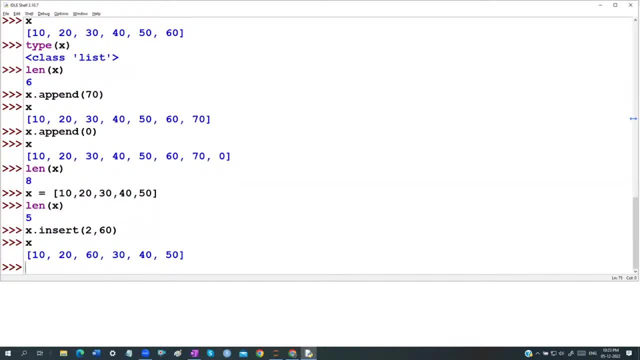 you can see the data like this: guys, 10, 20. it didn't replace the 30, actually. guys 30, 40, 50 is there, as usually. before the 30, it has been added the 60. if i say, what is the length of the x now? 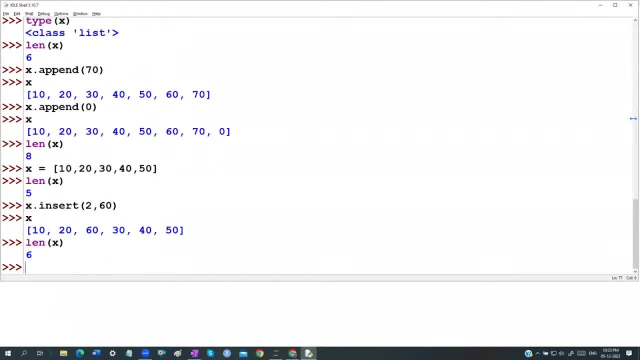 you can see that it has been became, which is going to be nothing but 6, actually, anywhere, guys, anywhere you can append actually guys, x dot, insert of which is going to be nothing but 0 comma, which is going to be 70 before the 0 index, it will be appended actually. 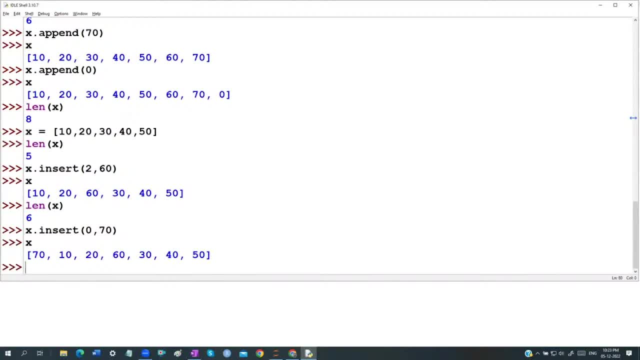 so insert will allows you to append the element wherever you want to append. x. the insert is sorry. the append is a method which allows you to append it even in at the end of the positions, end of the existing list. insert will allows you to append or insert the given element. 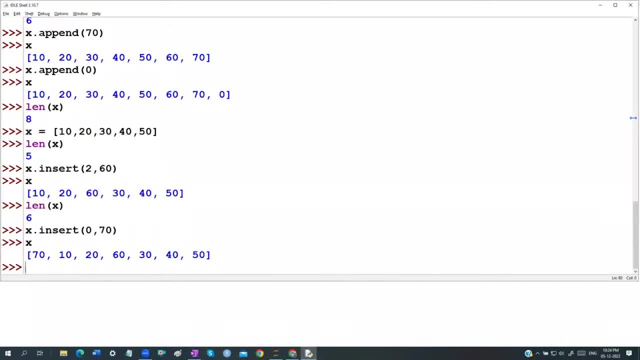 at the, whatever the index you require, it actually, guys. that is the difference between the insert and the extend method, what we have to understand it that's it actually, guys, slowly, guys, slowly. if you do the practice slowly, if you do the practice, guys, you can understand the techniques actually. 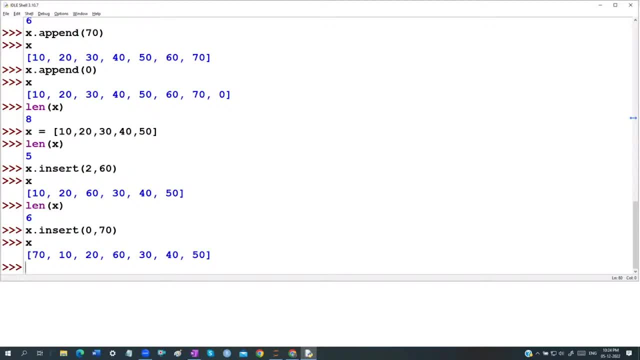 very simple concepts. python is not a complicated work to understand, it's a very simple actions, a simple concepts only, which we can work in a easiest way. we can understand it, actually very easiest way. we can understand it. actually, guys, really we don't require, really we don't require to work more about this particular concepts. actually, guys, 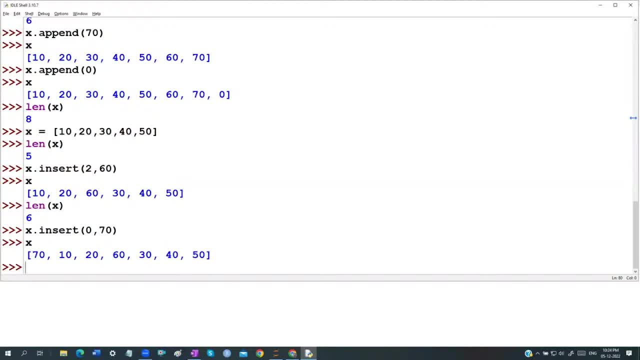 a very simple techniques which very slowly you have to understand it slowly if you start working with them. that's why in initial classes also, i don't take too much time actually, it's hardly 45 minutes, 50 minutes maximum. one hour will take the session actually, because all these are going to be. 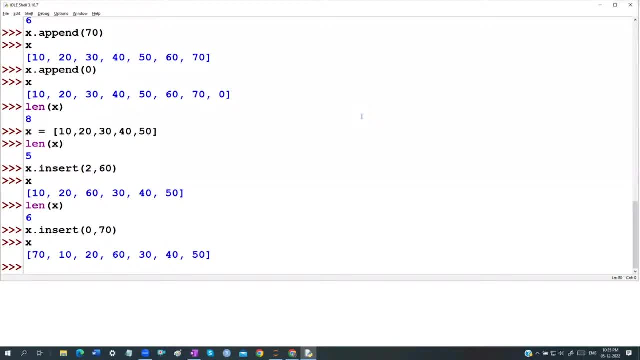 some kind of a beginning topics. actually, guys, they are going to be a kind of a beginning topics. actually. that is the reason why, generally, what we are going to do is- which is going to be a very simple applications only. we are going to be gets working with them, okay. so 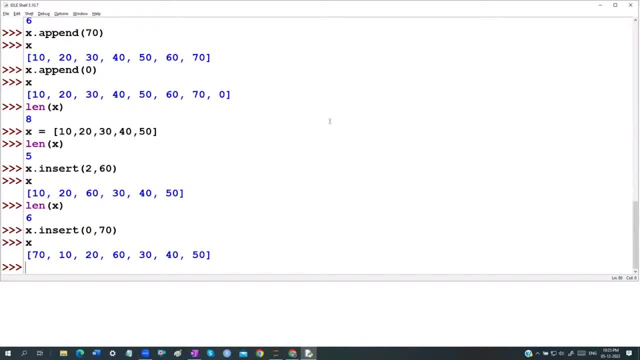 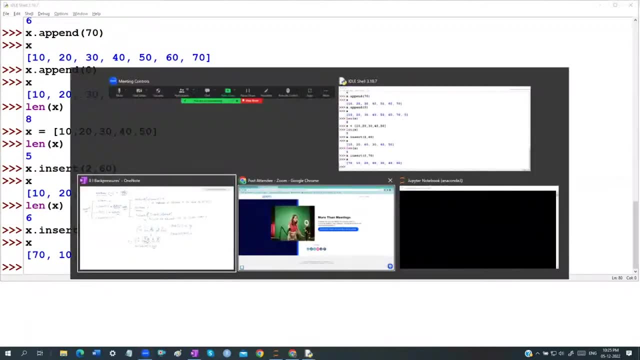 that is an ideas of how we are going to be gets working with the insight method. now there is a something called as an extent method. is there actually guys a little bit complicated to understand? little bit complicated means i can explain in a different way, but the concept 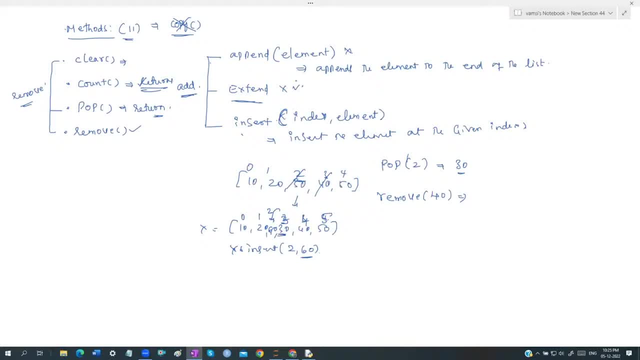 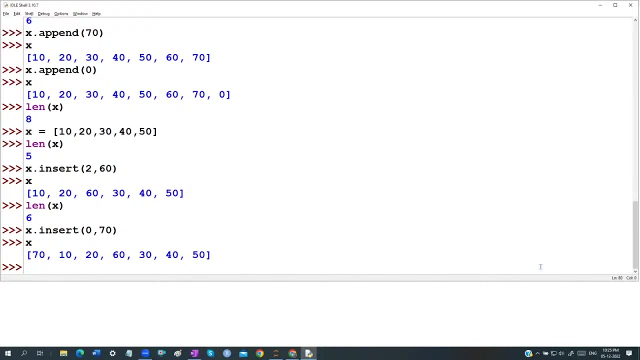 is slightly different. actually, guys, the concept is going to be slightly different actually, but try to understand in a easy way. later i'll connect the things actually. later i'll connect the things actually. yes, in a easy way to understand. actually, the concept is: learn. we are going to be explain very. you know, we are planing the practice, we are int donc. 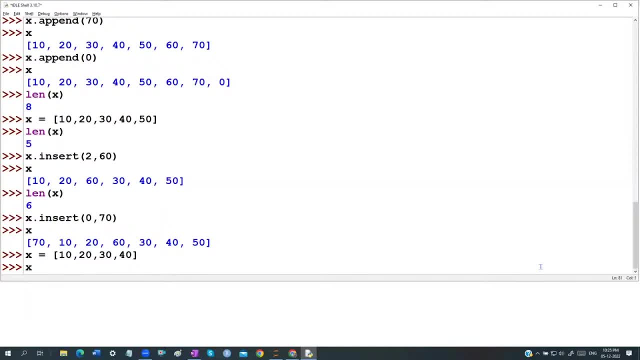 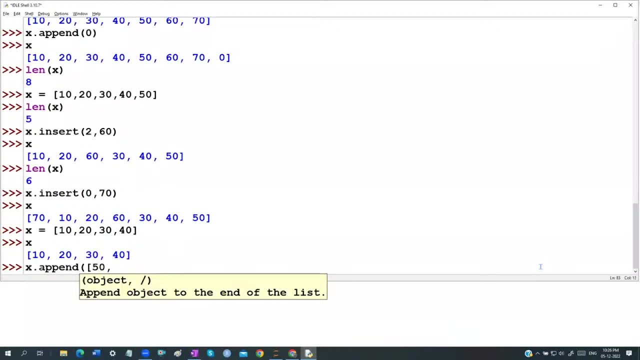 i'm going to use an example-like this and you learn this example. therefore, you could have this familiar idea. so that's component we learned in process, in the process, to understand, and i'm going to use contract whenever and yes, so that means you can see that i can apply. 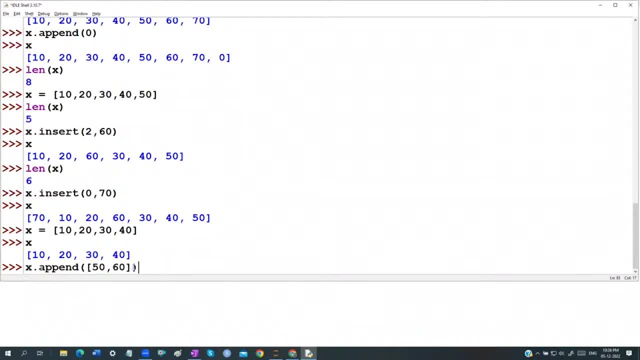 my old concept about contract, usually that i can, the concept same, with which i think about different versions. so that's why all of that get connected. yeah, that's the idea. you don't have to think about a certain elegant, then you start side by side using your concept. 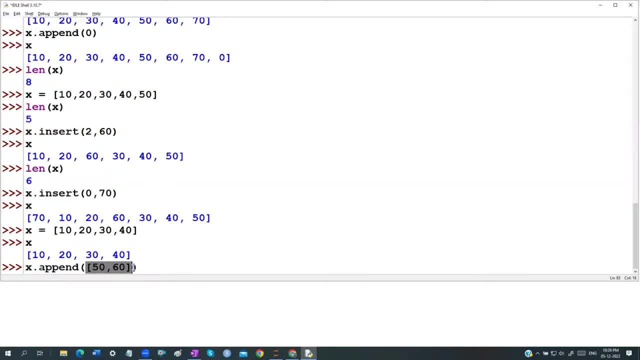 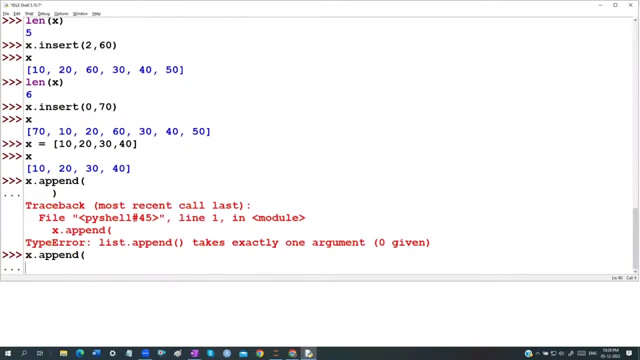 actually. so 50 is one element, 60 is one element. no, guys, 50 and 60, both of them has been appended as a one element only. it is going to be appended as a one element. actually, guys, sorry, sorry guys, it may be x dot append of. yeah, x dot append of. i said, which is 50 comma 60. actually, let me append. 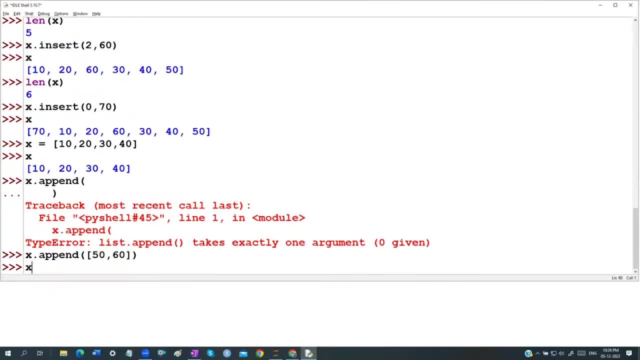 it actually, guys, once if you see the x. previously x is containing only four elements, guys. now i added two elements actually, but two elements has been not added individually, guys. 50, 60 is come and added as a one element only. so if you see what is the length of the x, it won't show you. 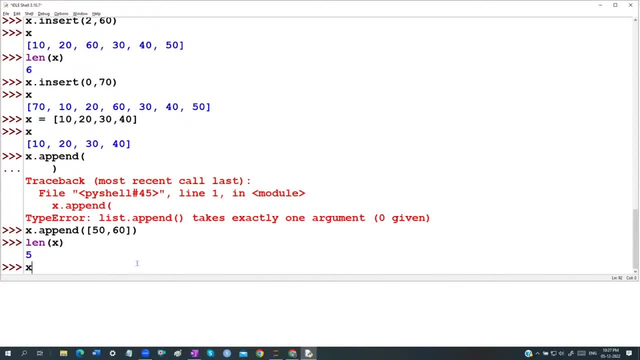 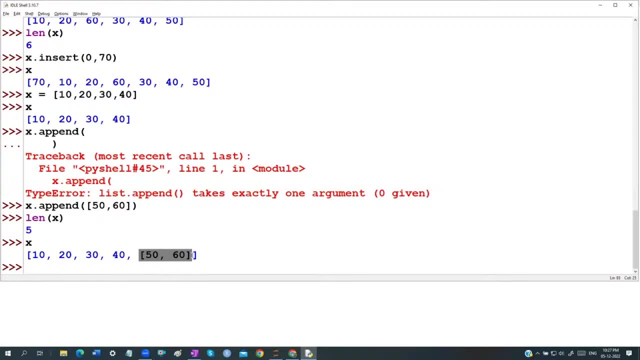 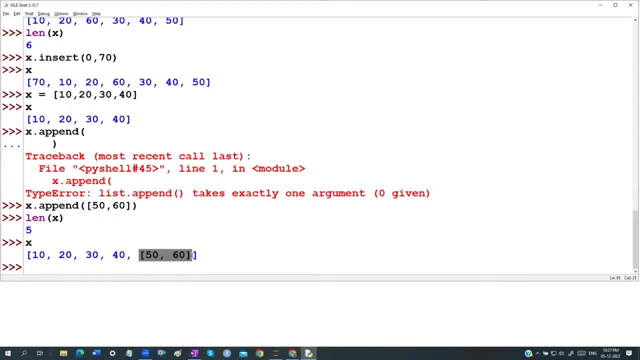 don't worry about that. don't worry about that, sir. you said that list is a collection of only values. no, list is not a only collection of values. i'll tell you guys: collection of objects, list is actually collection of objects, actually guys. so the guys who has been already joined. 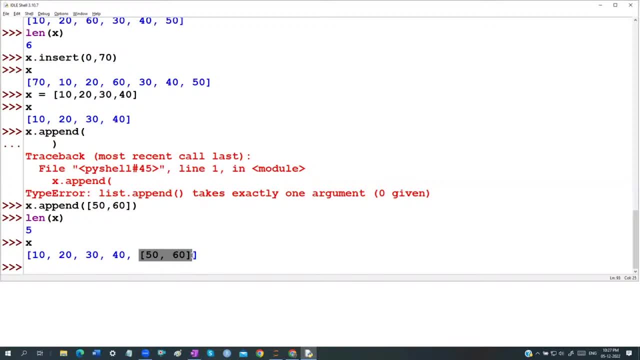 the joint earlier you got a little bit idea about object, but some guys who has been joined today they may not have the idea. you may not have the idea about objects, but don't worry, but keep in mind like whenever we are appending a list of values like that, they will not be added as individual values. guys, they will be added again. 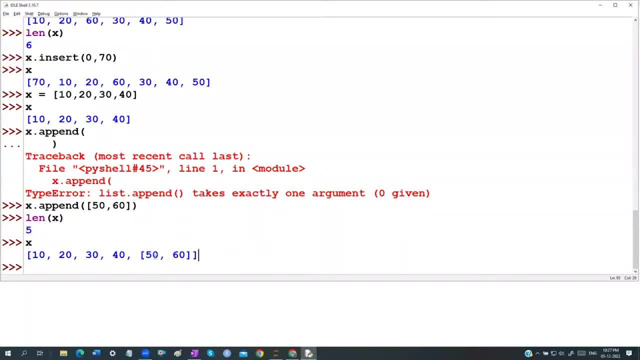 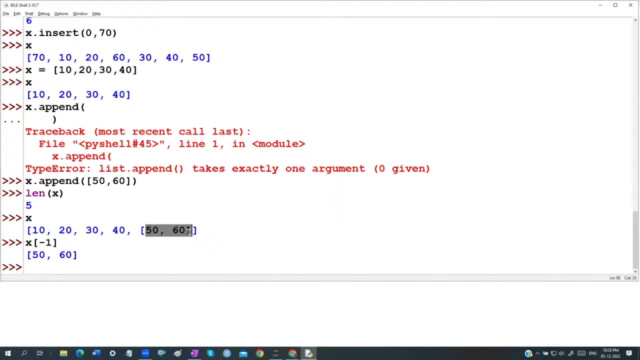 as a list. actually, this is nothing but a list of list, actually, guys. a list inside a list. this is list, actually, guys. if i, for example, if i said x of minus one, you are not going to get the last element actually as 60, we will get the result as 50 comma 60. actually, guys, that means you are. 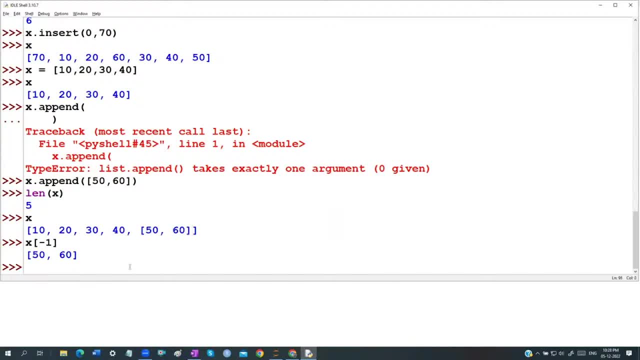 totally getting like a list. only we are going to be getting the output that is x of minus one. that is nothing but x of minus one. don't worry, guys, i'll share you those particular details and all these things. so once again i'm showing you guys x dot. if i said pop, the last element will. 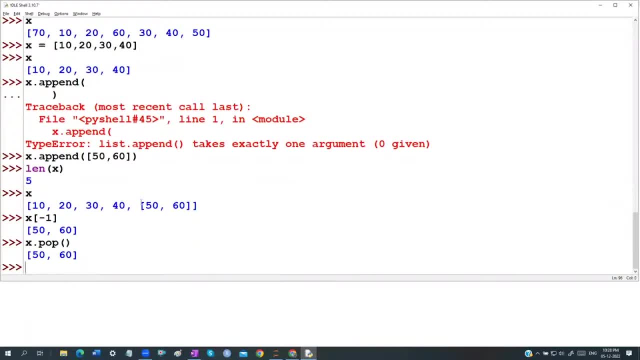 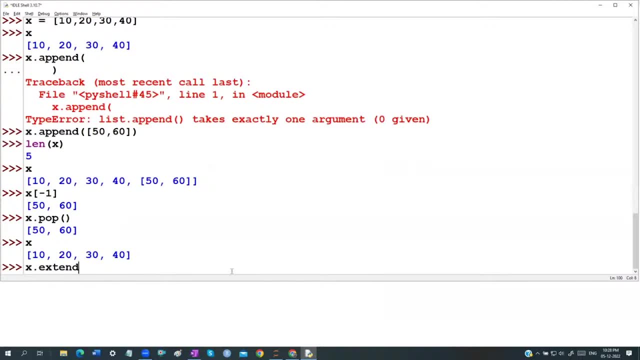 be removed. last element means not 60, guys. 50 comma, 60 is going to be one element actually. now see the difference, guys. when i said x, dot, extend, actually, guys why you don't understand this concept? because it is. it is. see the difference clearly, guys. when i said insert and append. 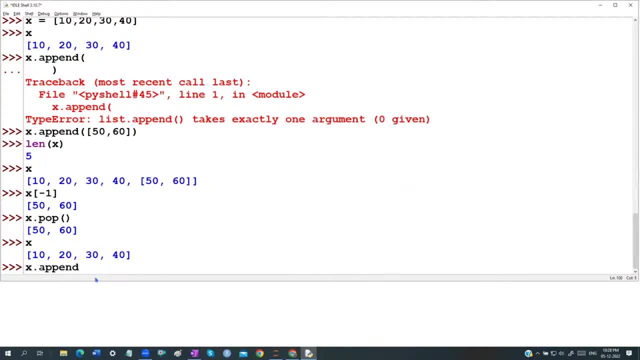 the input is an object. whenever i said x dot insert, that also is going to be nothing, but it is an object. but whenever i said it is an extent, it is going to be nothing but what we are going to call it as iterables, what is iterable for the timing leaving, guys, i'll. 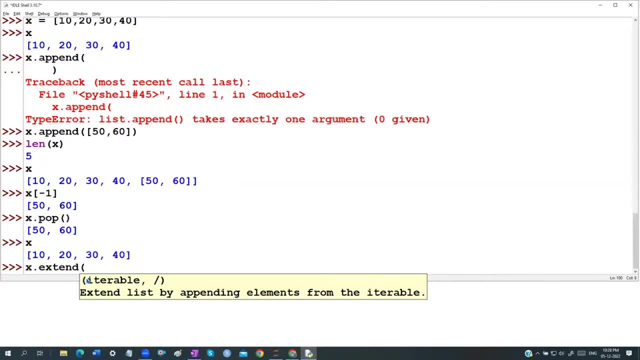 again come back and explain why. i told you know, i'll connect all the things. one after another will connect the things, because all it a time. you cannot understand it. actually, guys, that is going to be what i call it as an x extend. actually it is an x? dot extend. actually, guys, forget about the iterable. but one thing you: 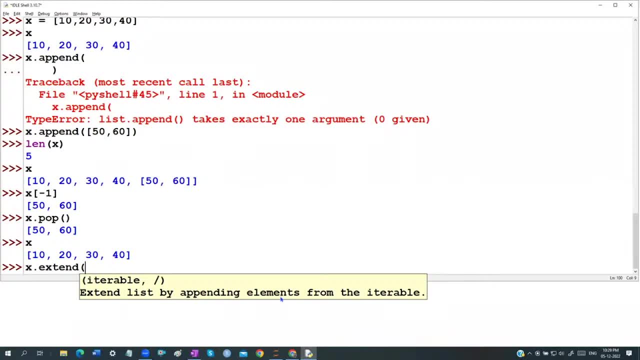 can find in this: extend the list by appending the element from the iterable. that means the difference between extend and an append method is: if you append a list like this, total list is appending to the x actually. but whenever i said extend, it is not going to be appended as n, it is. 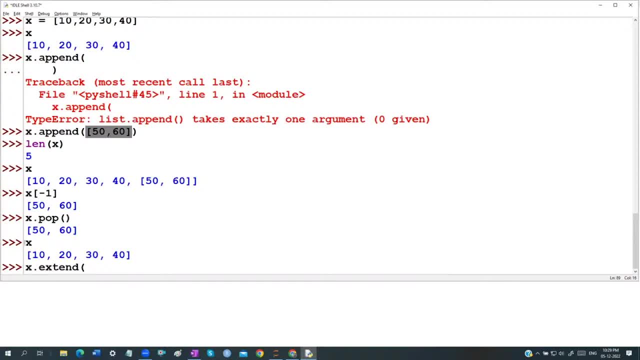 not going to be adding this as an object. what it will do is it will append the individual elements. actually, guys. that means 50 separate, 60 separate. actually same thing. i'll do it. actually, guys, 50 comma 60. i'm appending, actually guys, now, what you can find it of actually guys, it won't append. 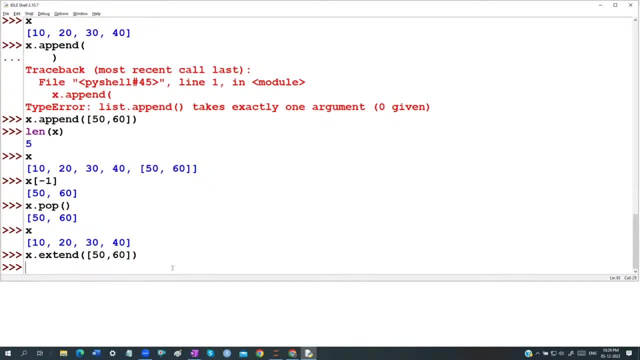 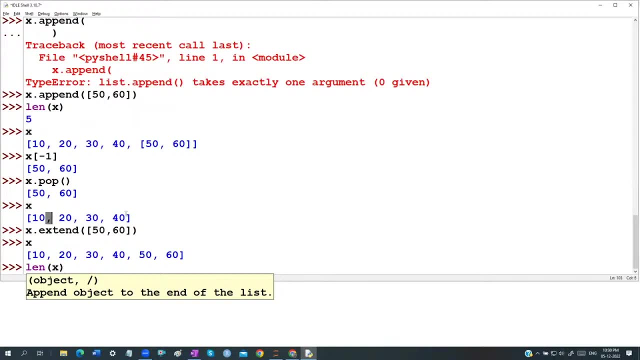 the 50 and 60 as a single element. like this: actually guys 50 separate and 60 separately, you can find what is the length of the x. previously the length of the x is four guys, but now the length of the x is not five. it is going to be nothing, but it is going. 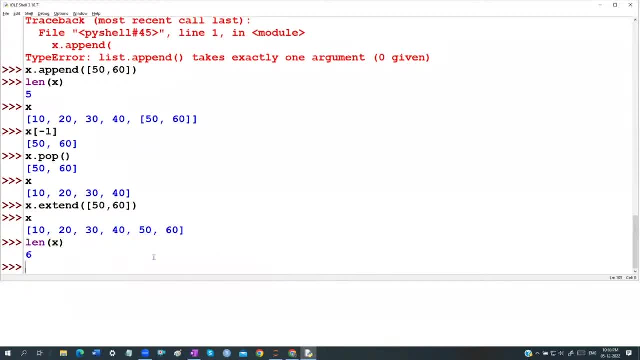 to become six is the result? what it is going to becomes actually, because it is not adding the total elements. actually, guys, not, it's not adding the total elements as a single object. each object has been appended individually, which is 50 comma 60 actually. so that is the difference. 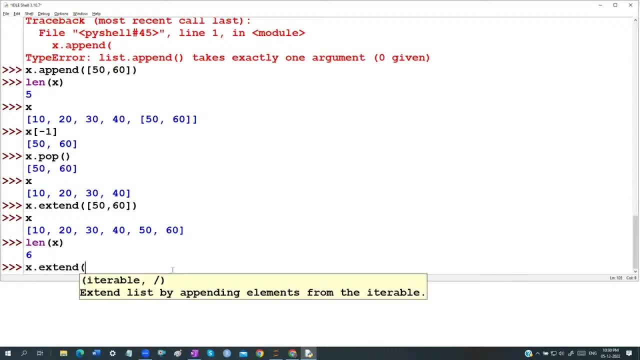 between the extent insert and append. actually, right now you don't know what is iterable, but in our coming classes i'll explain, like, what is meaning of an interval. then again i'll come back and i'll explain this particular concept, guys. so you can see it, guys, we are extending. 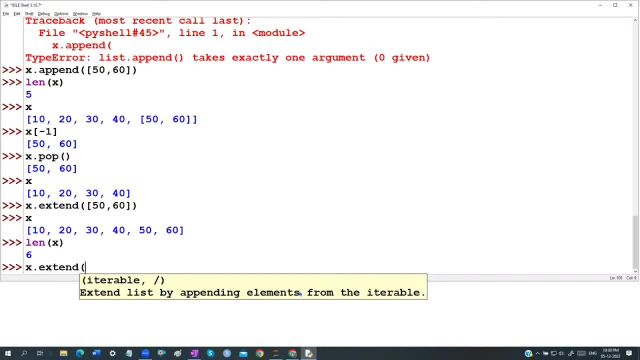 the list by appending not the elements to the list, it is element from the iterable to the list actually. so whenever we appended a list of elements, it is appending as a list only in insert method and in the append method, but in the extend method, even if i give a list of values also. 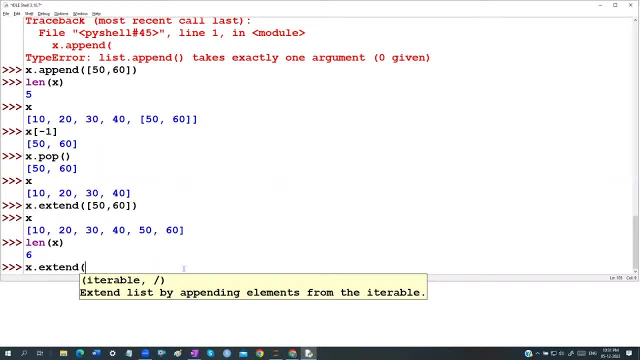 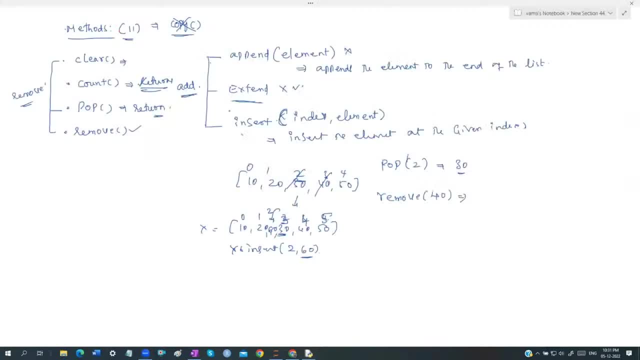 they are appending as an individual values rather than any single object. actually, yes, so totally we have been got discussed about, and another three more methods. so totally we covered about seven methods. actually, guess, apart from copy. apart from copy, it is going to be seven methods actually, that's right. clear, count, pop, remove. clear and 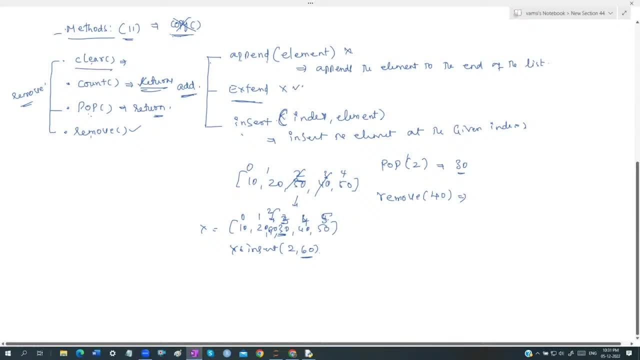 count, pop and remove are basically used for removing the elements. append, extend and insert are going to be used for appending the elements. count is only for counting the elements, actually, guys. so seven plus count is anyhow it is going to be eight. there are another three more methods, actually, guys, very simple methods. one is an index. 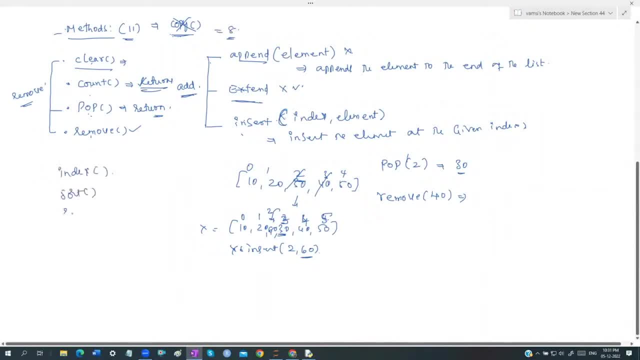 is there, the other one is going to be sort is there and there is going to be reverse, is there actually, guys? only three methods are there. so tomorrow we'll discuss about that and then i'll start with the next object called as an tuple. okay, tuple is very easy, guys, to understand the tuple and list. 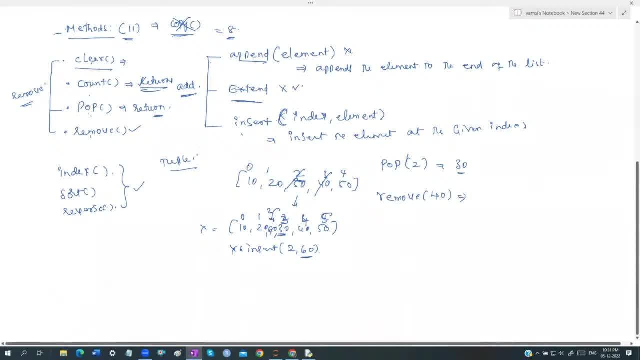 same like a list. only tuple will be existing. so after that i'll plan. actually, guys, don't worry, because some new batch new people has been joined and we don't know whether they really join the sessions or not. so i'll see for a couple of classes. 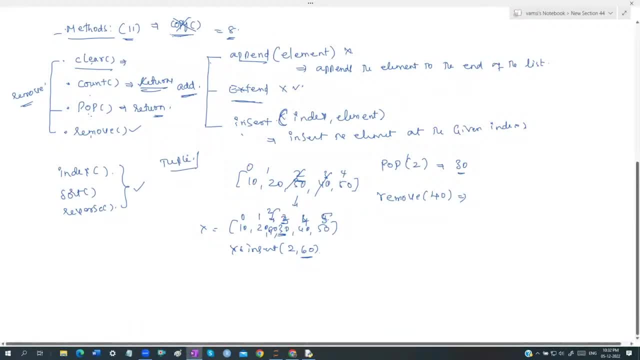 if more number of new people has been joined, i'll arrange a backup session, guys, okay? so depending on the number of participants, i'll decide it. i'll decide it in a couple of days. so, guys who has been joined for the today's class, don't worry about the backup classes. 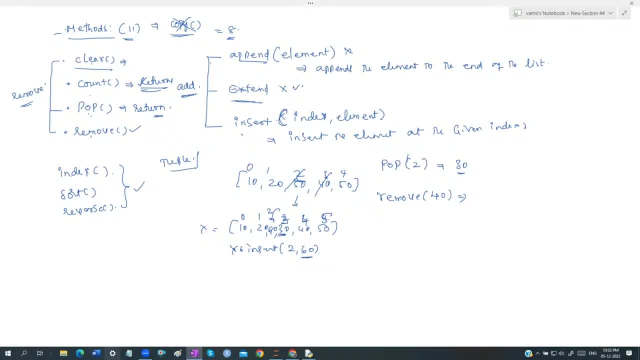 will give you the recordings or i'll take a backup session, if it is required, everything i will. i will put everybody on the same page and then we'll start with the regular classes. guys, okay, so that's it. uh, that's it for the today's class. guys, um, guys, anyhow, some people has been joined. 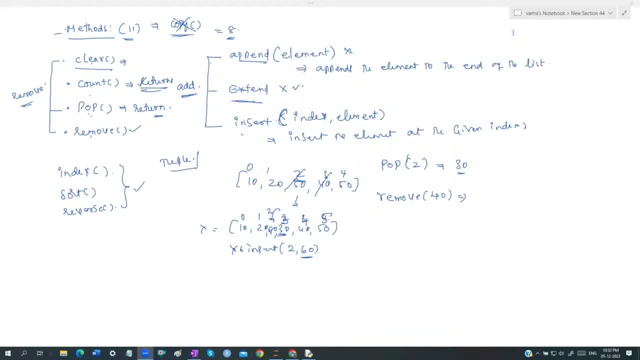 for the today's class. now, if you have any questions, uh, i can. i can spend the time, guys. 15, 20 minutes. i can spend it, no problem. if you have any questions, guys, either you can unmute yourself and you can speak or you can have a chat panel. you can see that you can type in the chat panel. yes, yes. 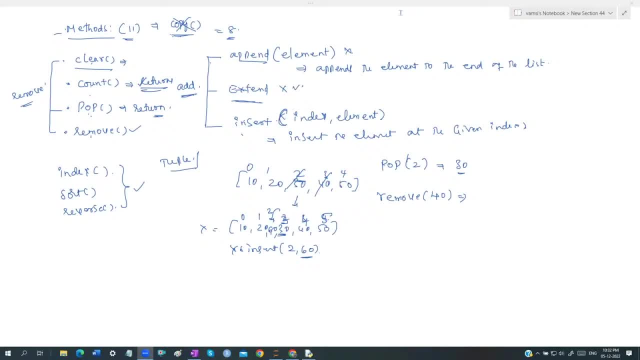 like it's not related to this. like, uh, we are working on a project, sir, okay, okay, okay, in which we are working on a different project. so we are working on a project, sir, okay, okay, okay, um, we had one client, uh, she had told me that, like, um, she had written a code for some, some aiml projects. 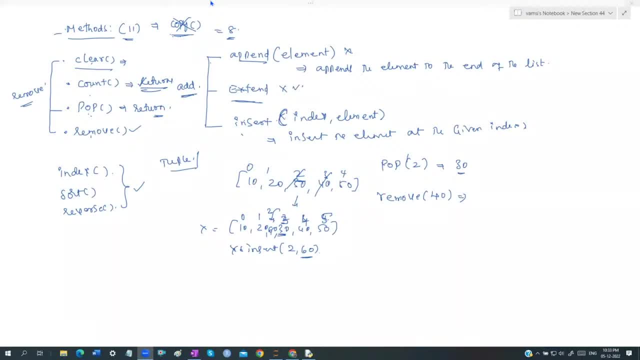 okay, okay, okay. what difficulty we are facing is we are unable to upload it into the client's system. so, like it is basically a us and uk based company, okay, okay. yeah, it's working perfectly in our systems, but we are unable to connect to the client. we even tried, like by using vpn, sir, okay. 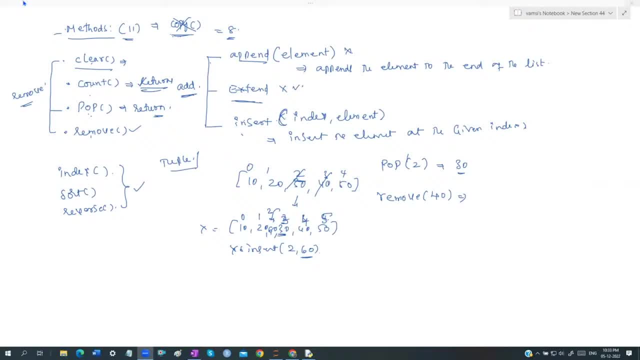 okay, we are unable like we are, might be the issue. i, unless and until i can't see the code and all these things, i can't say it. no, like what libraries you are using, what type of vpn connections you are using where you are trying to shift that particular data. so if you have any problem, you can just connect one to one. 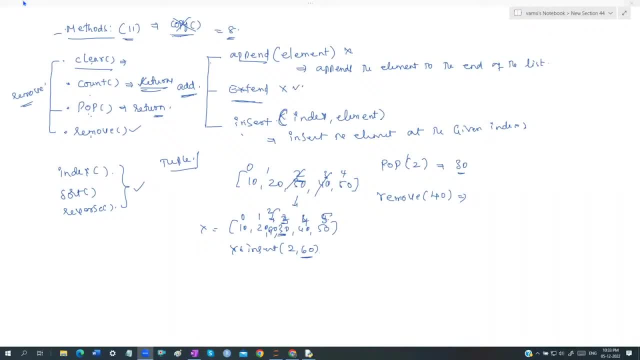 session one-on-one, we can connect it and then i can. if you can, if you have any option to show your code or you can explain that, then i can go, for then i can explain you like what could be the problem actually. sure, okay, so you have my number, right? no, sir, no, i'll ping you my number, just if. 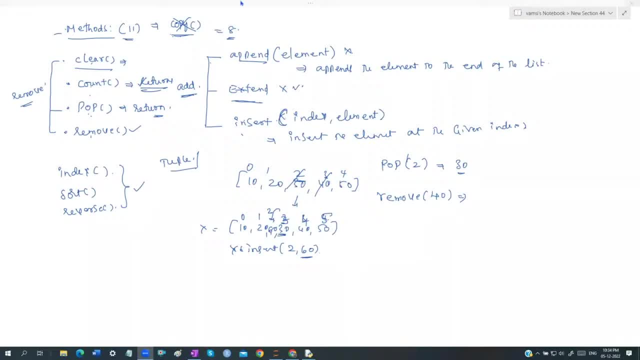 you have any questions personally, you can just ping it to my number. i'll ping you my number, sure, okay, yes, his name is uday. no, i think two days are there actually. uh, what is the name? right, okay, okay, i'll do it. yeah, right, guys, um, anyone guess? if you have any questions, 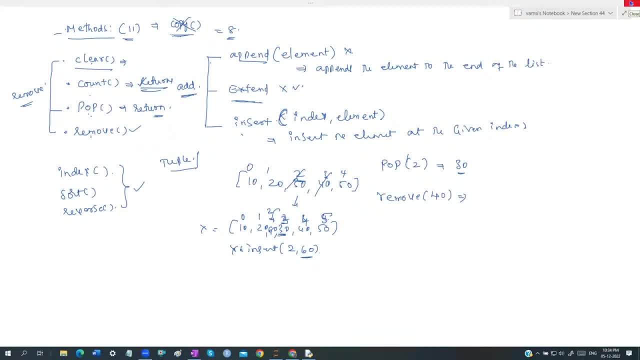 yep, yeah, i can. okay, i'm sharing with all of you guys. um, you can just take on my number. so this is my number, actually, guys. eight double zero, eight zero, double seven, double one seven. it's my number, yep, so if you have any questions, guys, you can just feel free to discuss with me now or you can call me. 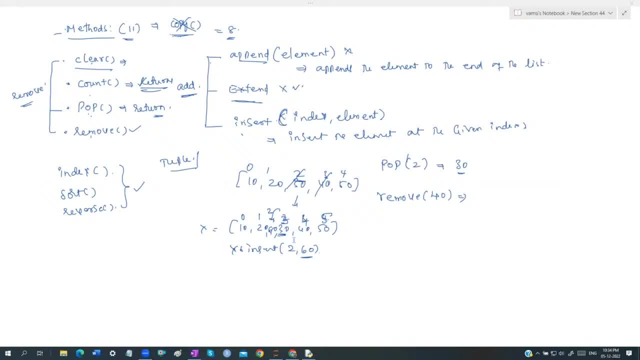 you can message me on the whatsapp or telegram- we have both telegrams and whatsapps are there- or you can call me and you can discuss with me. anyone guys, any questions? yeah, just couple of days, we'll create that. everything is ready. just only thing is we. 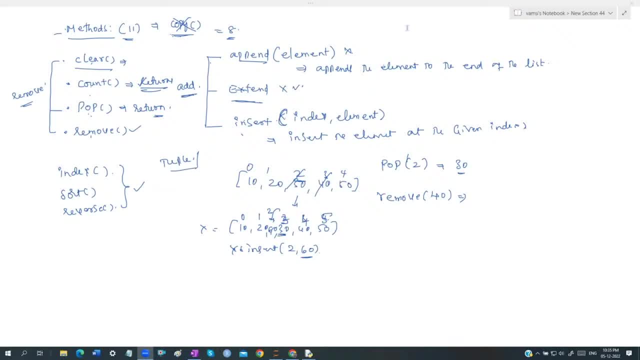 have to share because new guys has been joined for today. so we want to just um, just make it within one or two sessions. we'll just close up the sessions and then we'll start up sharing that particular all the, all the things. actually, okay, fine, yes, guys, anyone who has been joined for the today's class. if you have any questions, 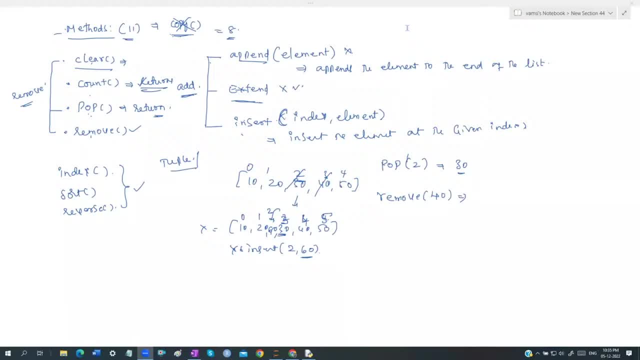 yeah, hi, i'm shi. this is manohar. yeah, i'm manohar, yeah, yeah, i have one question, like at the end, at the end of this, uh course, uh, like, uh, we're going to get any kind of, you know, uh, practical kind of. 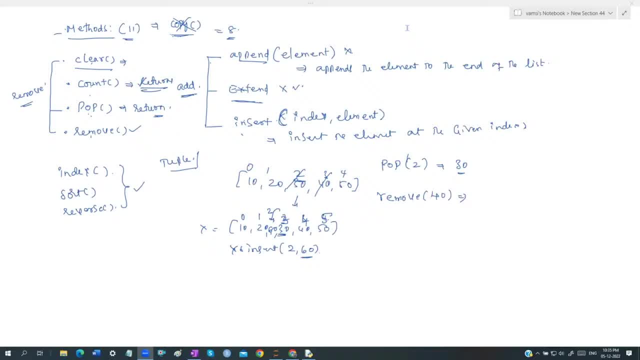 use cases. yes, yes, every see. it's not only at the end of the course. your data science itself is going to be like an uh, um, uh. it's a kind of an practical implementation, only it's not like a theoretical concepts. so every example will do with some kind of a real data sets only we are going to do with. 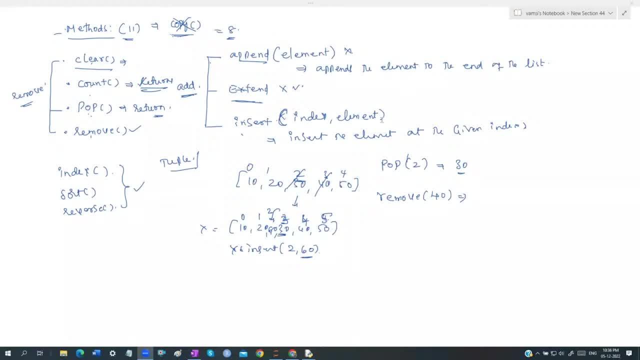 that. so every example, every algorithm is going to be a kind of a use case only, so it's not like we don't work with something like a small, small data sets. we don't work because all our data analytics and all the data science requires a real data sets we require- i can. 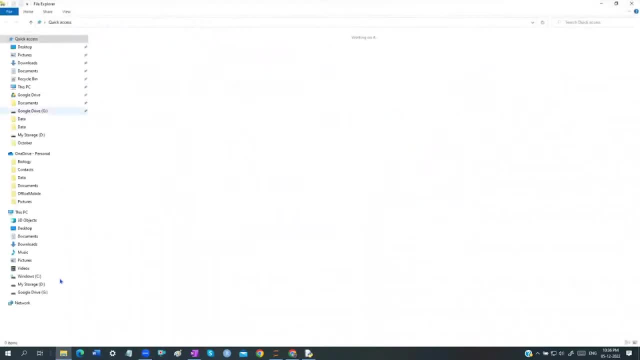 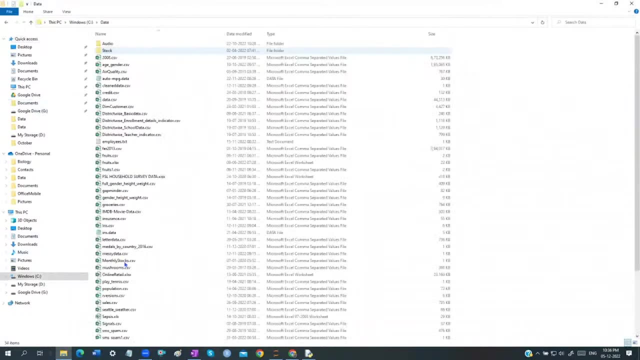 say that every example we'll see is going to be a news case. actually, like i can tell, just show you some data sets which we are going to work with them. see, all these are the data sets which we are going to work with them. it's not like a dummy data. that means we are not creating the. 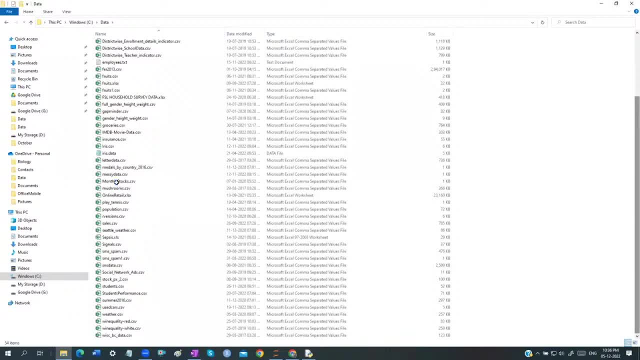 data. i am not creating this data manually. it's a real data sex, actually. so it's. this is not a real data set, maybe, but you can see some kind of a data that is going to be something, but you can see some kind of a real data sets. we can work with them. actually, these are all stock prices of the various 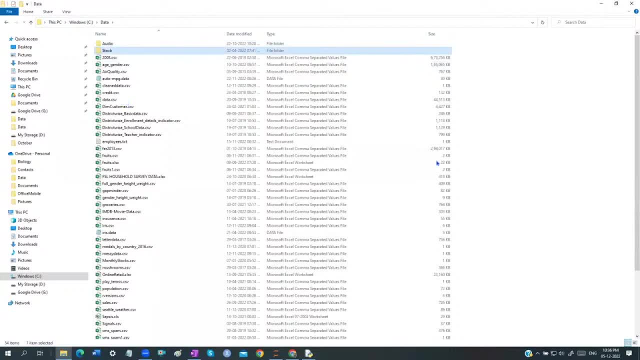 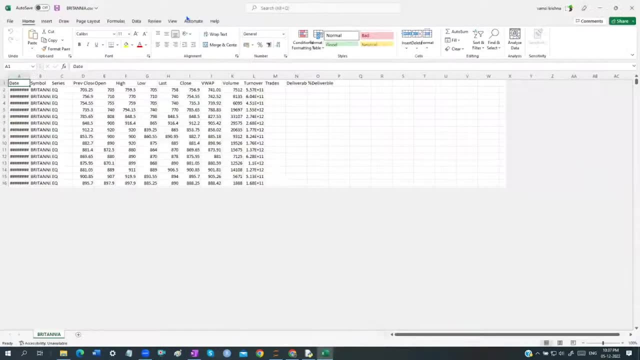 companies from different, different dates. you can see that particular data actually. so every example we'll see is going to be use case, it's. i think you are asking about something like a project. do you mean to say, do you mean to say, that at the end of the course, do you want to have a project? 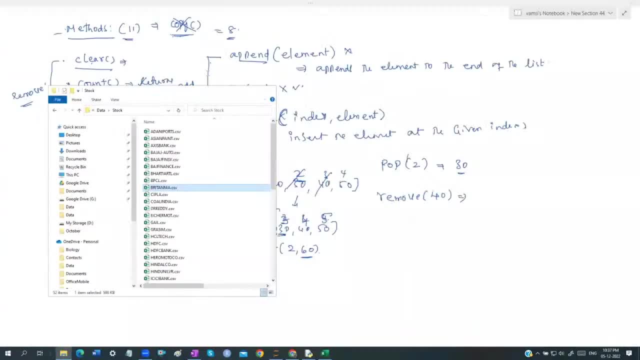 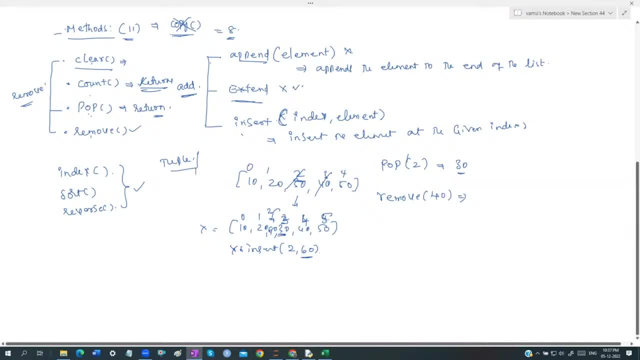 or are you talking about use cases? use cases, use cases. every example is a use case, every algorithm is a use case. only we do it actually. okay, okay, fine, right, yes, yes, um, okay, fine, right, yes, um, get a course completion certificate. uh, roy, uh, from durga soft, you will be getting a course. 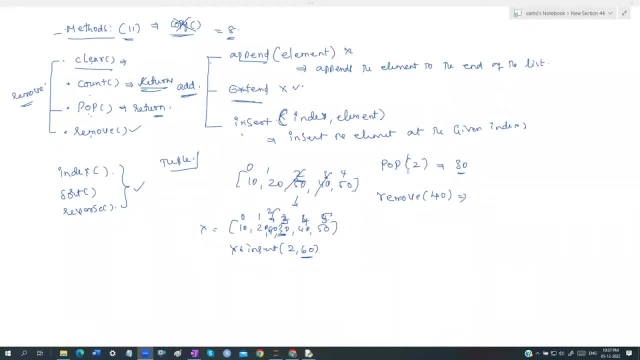 completion certificate. but, uh, one suggestion i can give you is: uh, i was only a consultant trainer. no, so just you get some confirmation from durga soft people also, but even so, earlier also so many people asking me the same question. uh, but as part of the basic information from the guys they will be giving, 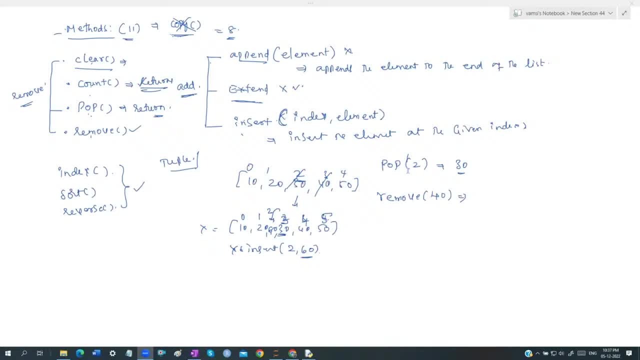 some kind of a course completion certificate, but please confirm it. one more side from my back-end team also. so okay, and if we go with this, you know the training or data science, uh, are we able to uh get through? you know the certification? absolutely, absolutely, absolutely, yes, absolutely absolutely. 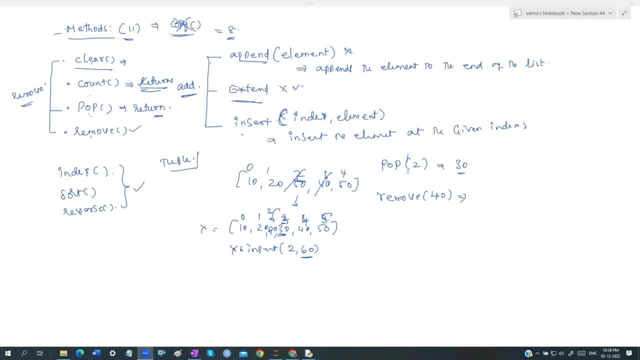 we can. we can do it actually because, see, whatever the course curriculum which i am going to follow is almost all um in parallel with the microsoft recommendation, or it's going to be some kind of an uh the certification oriented program only. and even my self, uh, i was certified from 888 hyderabad. so, like whatever the course curriculum they design, what? 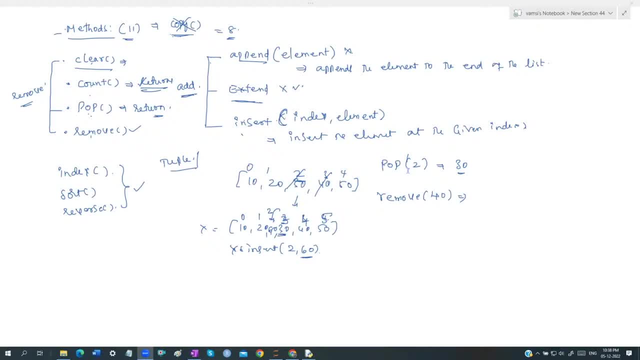 are the course curriculum with parallel to the microsoft or any um, like any other certification program, like aws or amazon. we have it actually as we have from different certifications, so in parallel with those um programs. only, uh, my course curriculum is also going to be gets designed. so 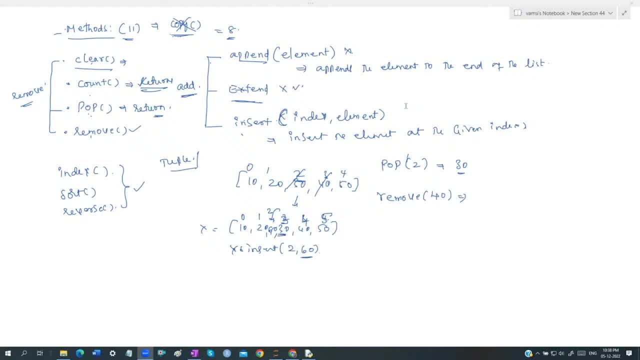 if you want the two things, either you can for an interview, uh, perspective, or a job oriented like a to, as well as even if you want to clear anything like n, which is going to be certification programs, you can also clear that particular certification programs. okay, okay, fine, right, guys, any more guys? 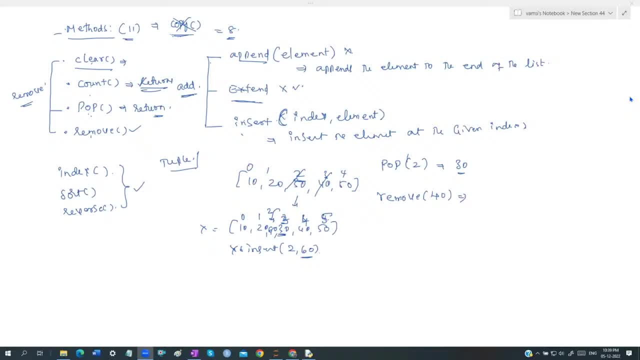 okay, so we'll do one thing, guys. uh, thanks for attending the session, but today it's a little bit late night class, so everybody is going to be uh, get tied, uh after your work and all these things. but uh, spare some time, guys, and spend some time, um, just not not only attending the 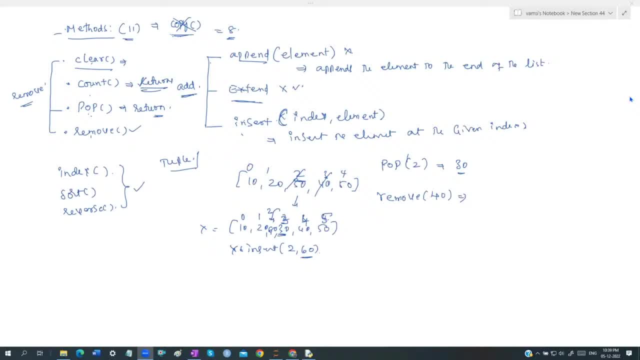 trainings. just, we have to go through all the practice and all these things. we have to do that. so, guys, um, i'll see you tomorrow, uh, same time, at 9: 30 pm. uh, please join by 9: 30. i'll start 9: 30, 9. 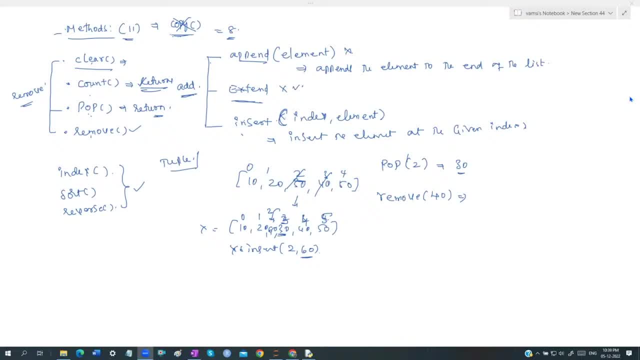 30 if i'll start the session. uh, i'll see you tomorrow. please attend three to four classes, actually, guys. then, um, i can take a backup session. if you feel that, if you really feel that there is a backup session is required, i'll guide you through that, actually, guys. okay. 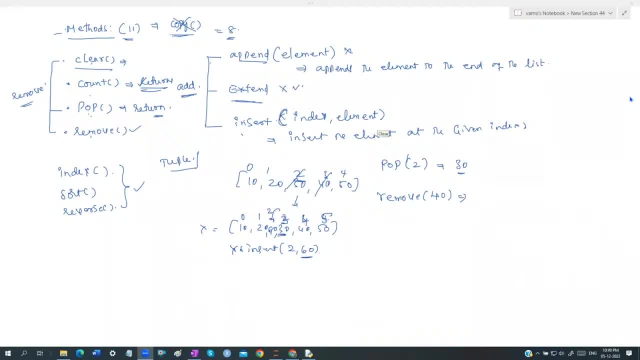 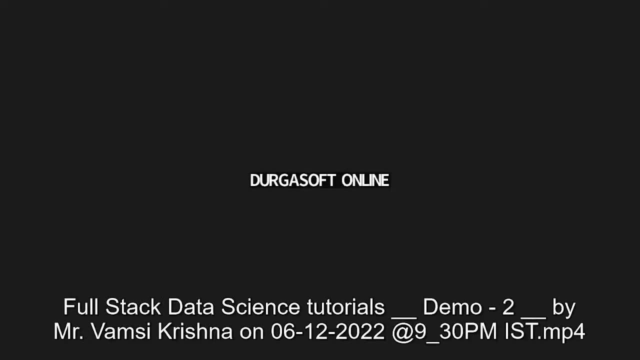 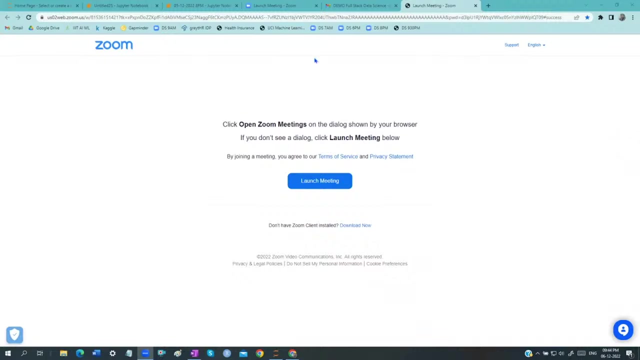 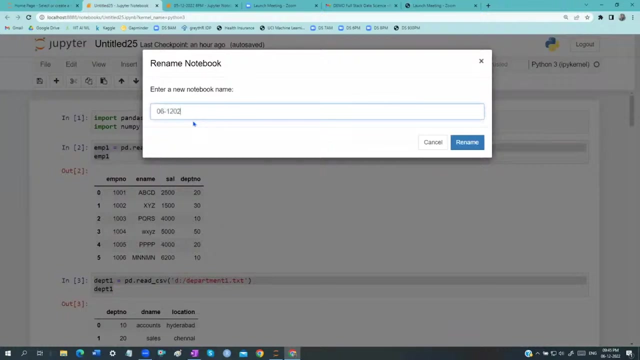 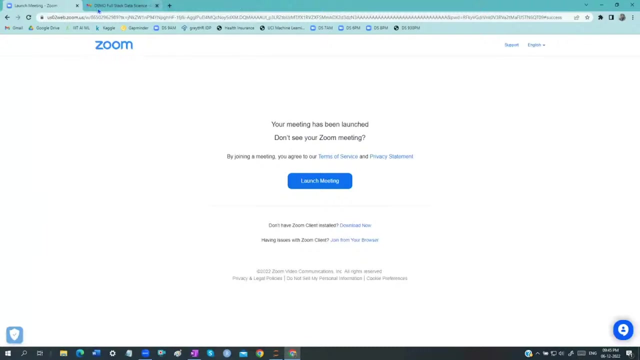 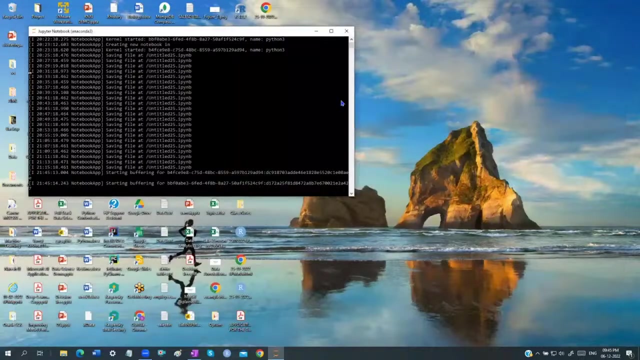 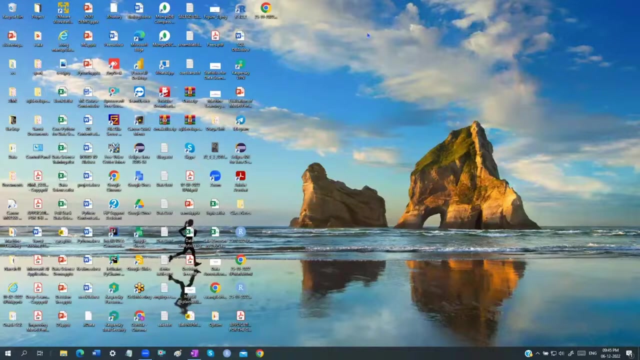 so, thanks for all of you guys and, uh, good night guys, all of you, thank you, thank you guys. you, yeah, hi, um, good evening all of you guys. uh, hope all of you can hear me. so, good evening, yeah, right guys. so, guys, um, let's continue from the the last session, guys. 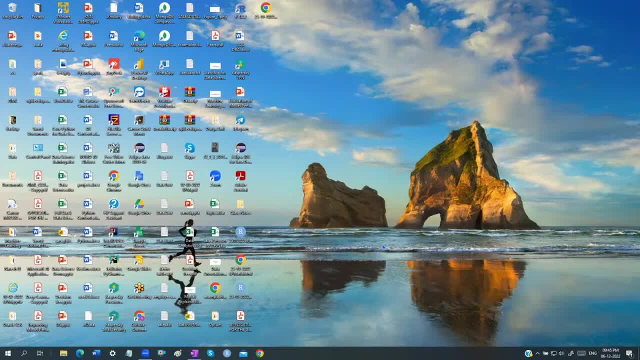 just give me a second. yeah, so, guys, um, in the last session- i was talking about the last session- we have been started with, uh, something about the, uh, the list, uh, what is actually a list. we have been got discussed. uh list is going to be nothing, but it's going to. 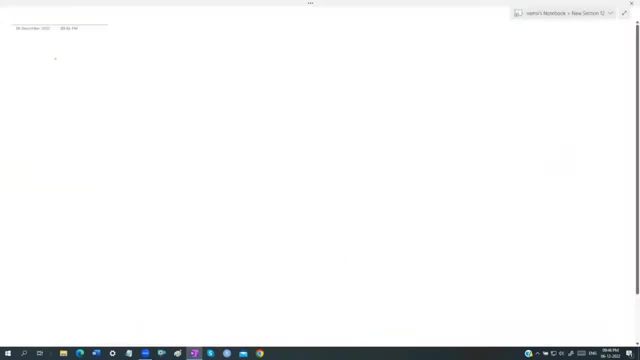 be what we are going to call it as an immutable object, what we are going to call it as actually, guys, okay, so list is going to be a kind of an mutable object. uh, just give me a second guys, just a minute once. uh, guys, uh, anyone has been joined for the today's class? uh, today is your. 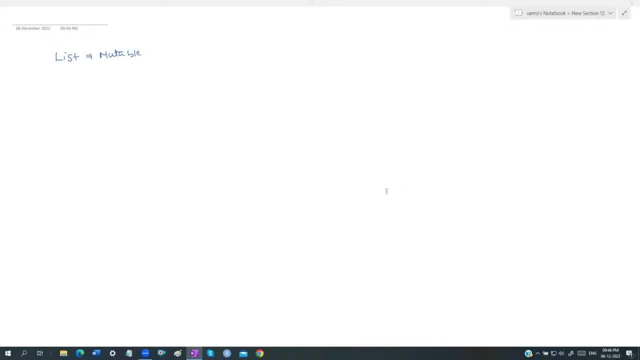 first class. is anyone? is there guys? i think i can see some names. yes, say it. i think today i will join the first class, right, yeah, yeah, okay, okay, uh, have you, um, have you attended any workshops of mine? uh, not yet, this is okay, okay, any others guys? shirak shah, i think i can see some name. venkat. 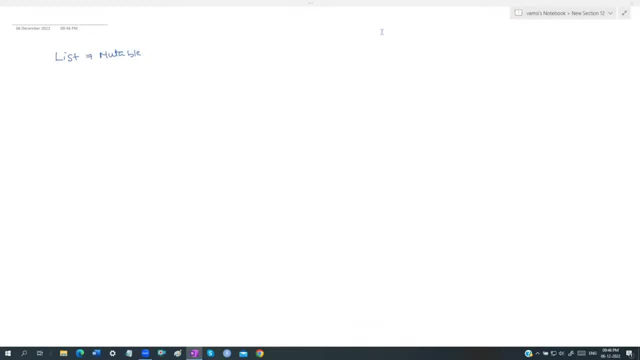 so that i can just tell you guys, like, what has been happened. i can just tell you about that. oh hi, yes, venkat, i have been attending your classes from the beginning, beginning, okay, okay, fine, okay. venkat means: uh, we have venka from, optimum venka from. oh, okay, okay, okay from us, okay. 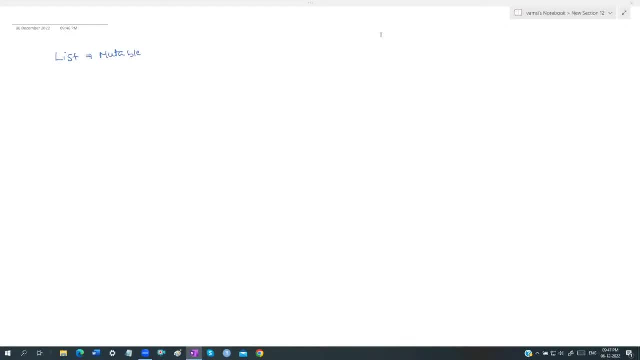 fine, guys, okay. so, guys, um, if anybody has been joined for the today's class, uh, just let me explain, guys. uh, we have just uh started um a couple of uh weeks before. uh, just a part of introduction. so, if anybody has been joining for this class, it's okay. if you guys want. 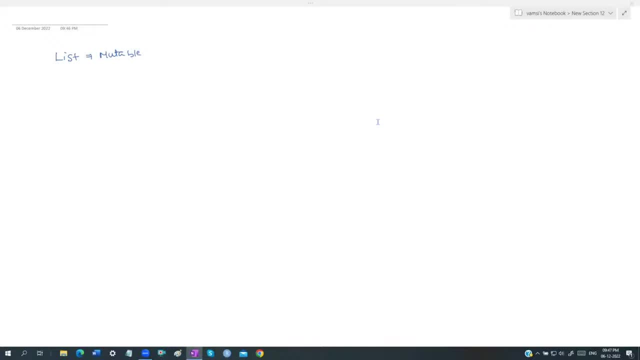 was happened and it's an only introduction part only, as i already told you that i'm going to take a backup session for the people who has been joined lately, because more number of people has been got joined lately, so i'll take a backup session and, apart from that, i started with the 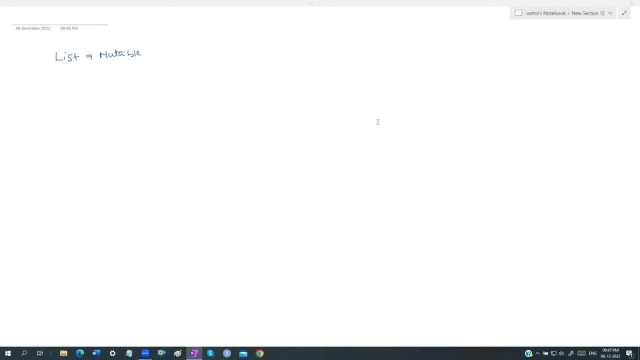 basics of python only, guys. so if you really already have an idea about python, you can understand it. but no worries, just we can understand the things, guys, because python is a very easy and simple language to learn. don't worry about the whatever the classes you have been caught missed so either. 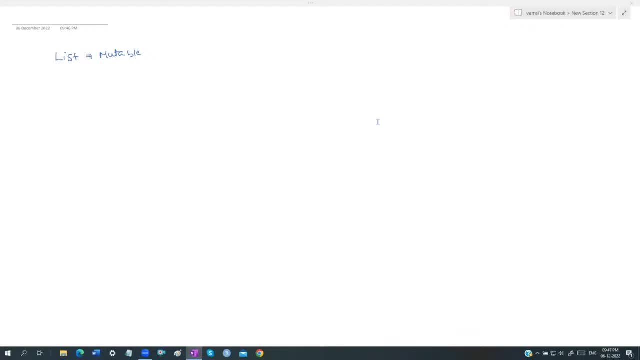 you will be getting a recorded videos or i'll take up a backup session, depending on your requirement, guys. okay, fine. so, guys, we have been started with something called as a list, which is going to be. what we discussed about is: list is nothing but a mutable object. actually, guys, what is this term? 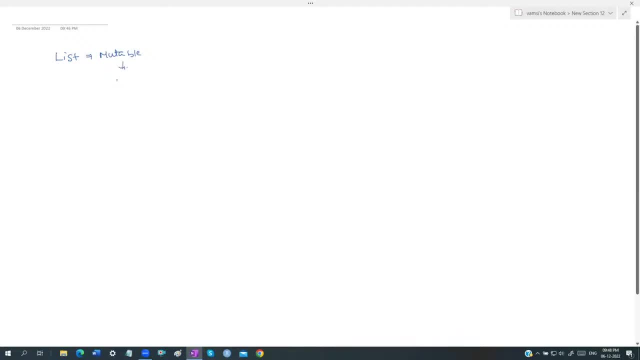 called as a mutable. mutable is nothing but what we are going to call it as: an which can be modified, which we can modify, actually, guys. so today we created a list, we can add up some elements. what is, first of all, list? actually, guys, a mutable object which is going to be gets contains a collection of some kind of 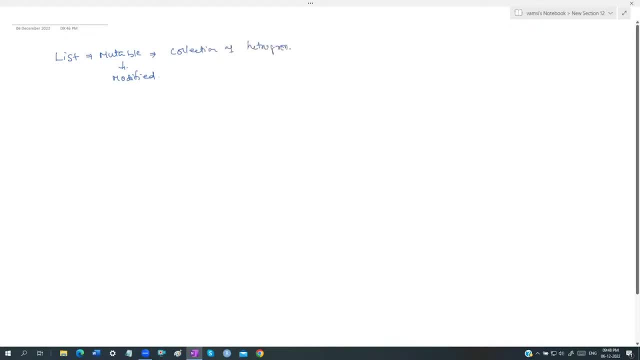 an. it is going to be some kind of an heterogeneous values. actually, guys, it is going to be heterogeneous data or heterogeneous elements. what we can say about that? so how to create a list? also, we have been got discussed so repeating almost all from three, four days. we are repeating all the basics. 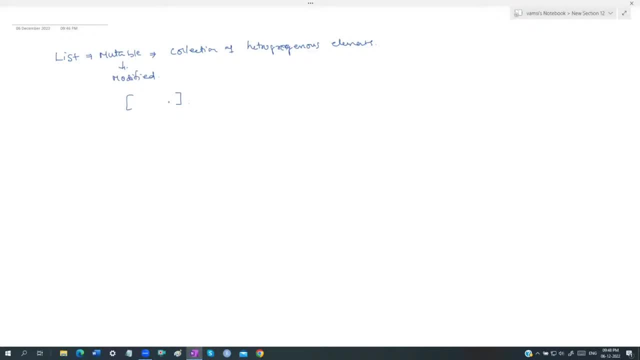 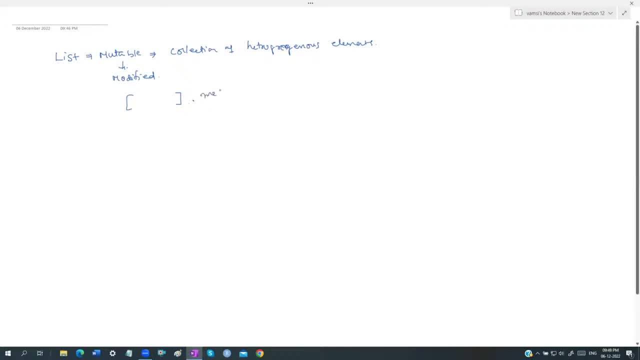 is. we have the relationship between this, how configurable the database is, is what would be associated with the list. actually, now, what pulled up was a held and, shall we say, the random detector, and this is eclipsedorus, but also this: already have a map of our wrote. 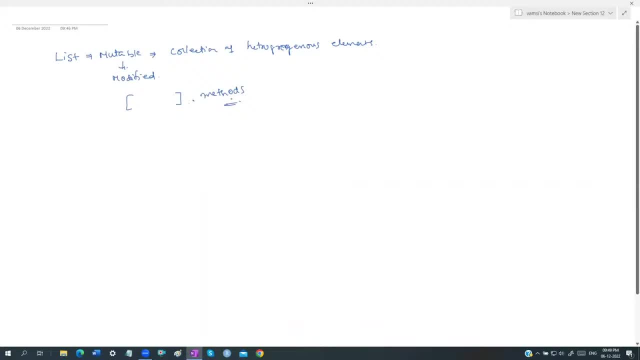 driving propia shown in the top left heading. so where there is only oneза, which is on the left windows, one addition to the other, and this is used to talk about some of the things that we need to take into consideration around, rather from any Tech rich addition, you know. 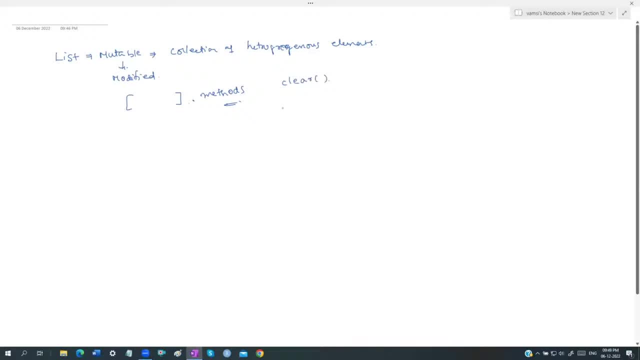 you'll umpire this into: uh, these modules, what others might, and I don't know, but somehow use it to remove the elements. actually, guys, once again, quickly, clear. yesterday we have already discussed about that remove and it is going to be pop. actually, guys, so clear, will remove all the. 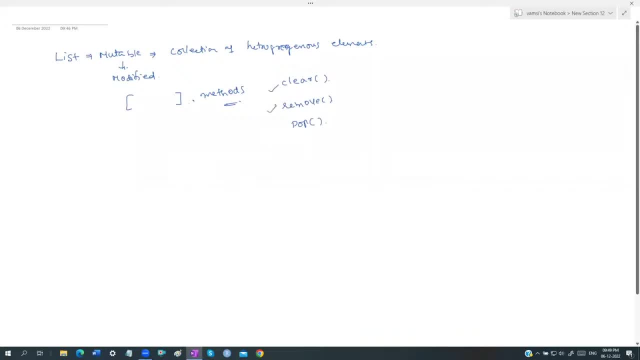 elements remove will remove only the required, required value and that too, only the first occurrence, only pop is basically based on the index, actually, if you want to add the elements. actually, guys, yesterday we discussed about three methods. we have been got discussed. one is going to be, we have been seen about about the append method and apart from that we have been seen about the. 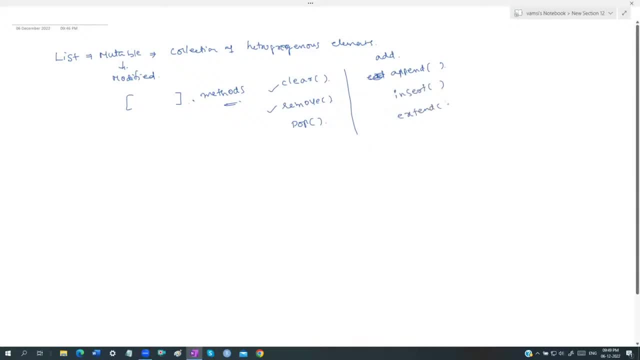 insert and we have been seen about an extend method. actually, yes, append and insert is almost all the similar with a slight difference. actually, guys, the difference is: append will add the elements only at the last. insert is going to be at the required index. before the index we can add. 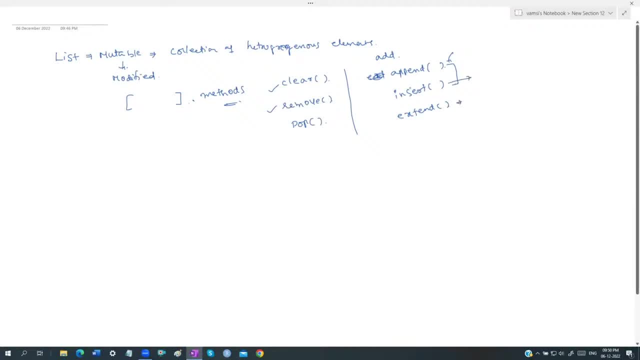 actually i told you the difference between extend and the append method slightly difference actually, guys. extend will is basically used to append individual elements, whereas the append is going to be appends, which is going to be all the elements at a time. actually, slowly, we will study. we already studied about. 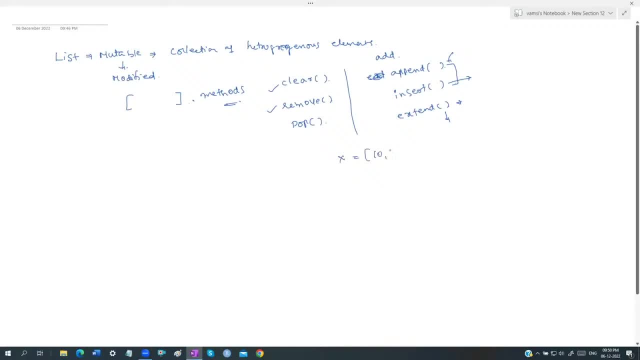 those particular applications. for example, if i say x is equals to 10, 20, 30, 40, for example. i told you the difference. actually, guys, when i said x, dot, append off, which is going to be. if i said 50, 60. we cannot append 50, 60 individually, guys. if i append the 50 comma, 60, then the result is going. 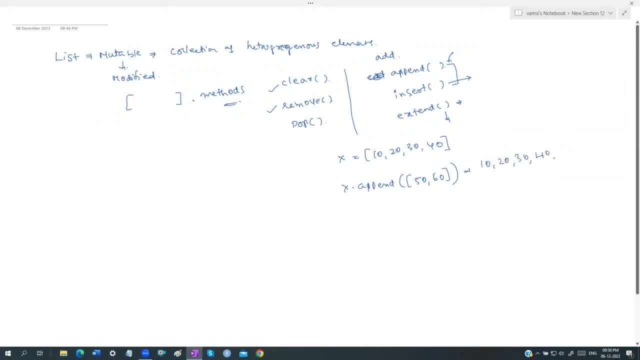 to be something like this: guys: 10, 20, 30, 40. it won't append 50 and 60 as an individual values. actually, this is how it is going to be: gets appended. actually, a list inside a list will be appended. same example if i said extend method. actually, guys, if a same example if i extend method. 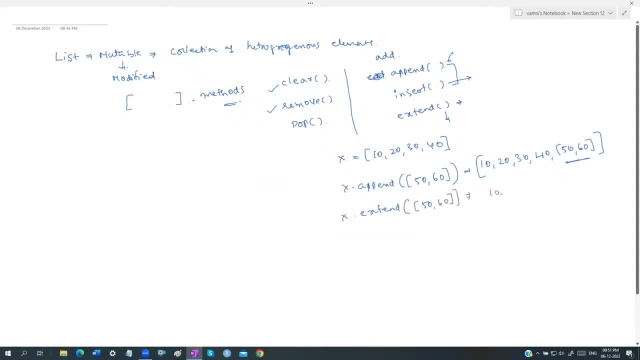 by using 50 comma 16, then there are going to be individually. they will be appended, actually, guys. individually means the result is going to be 10, 20, 30, which is 40, 50 and 60. actually, guys, because right now you don't know what is meaning of an iterable concept, actually, actually. 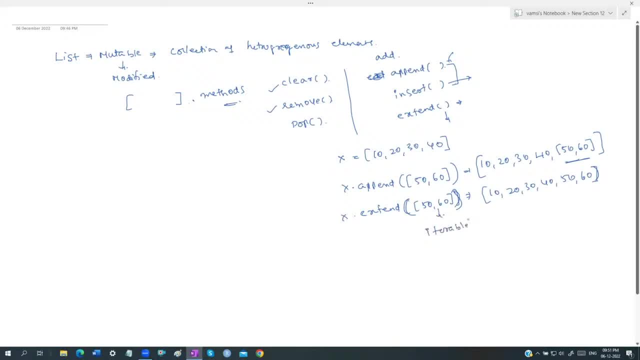 this extent is going to, takes an input as an an iterable object. right now we don't know what is an iterable object for the timing. skip some points actually slowly. we'll add up the things actually so clear: remove, pop is already discussed. append and extend, and x the append extend and which is: 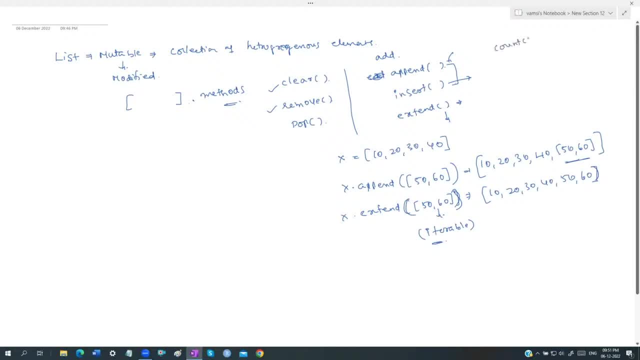 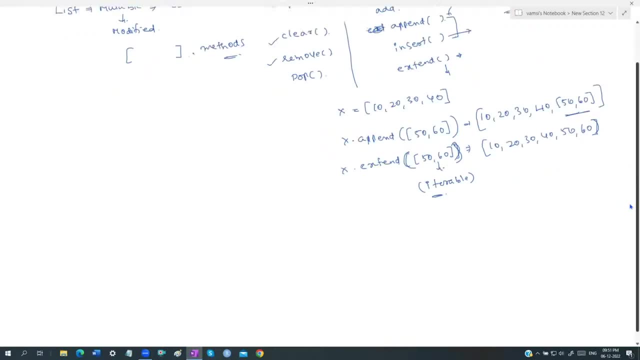 inside. we have been discussed, and already we discussed- about a method, what we are going to call it as an account method. count is basically used to count how many times a particular value appeared in the list, actually, so how many times a value is existing in a list if you want to count? 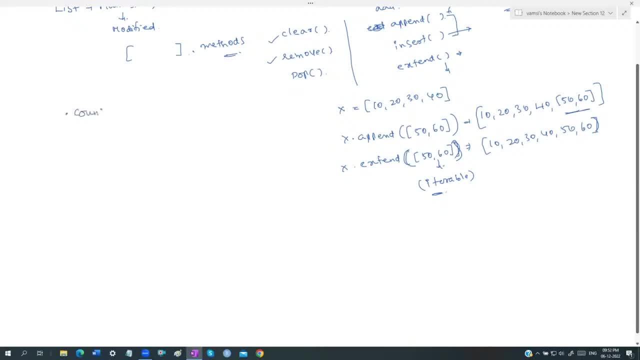 in simply the list dot, which is going to be a count, and give the value, whatever the value, you want to count how many times this value occurred in the list. it is going to tell you three times, four times, zero times. if it is not there, we are going to get a zero value, actually, guys. 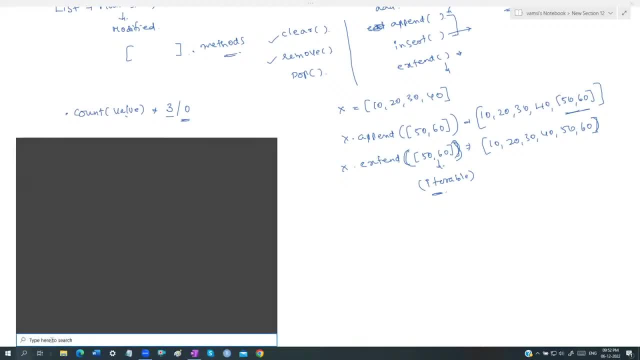 okay, so quickly, guys, just quickly, two minutes. i'll just complete of that. so this is going to be the ideal i'm opening here where the i'm going to write all the python script and the python code, what i'm going to be writing it actually, guys. 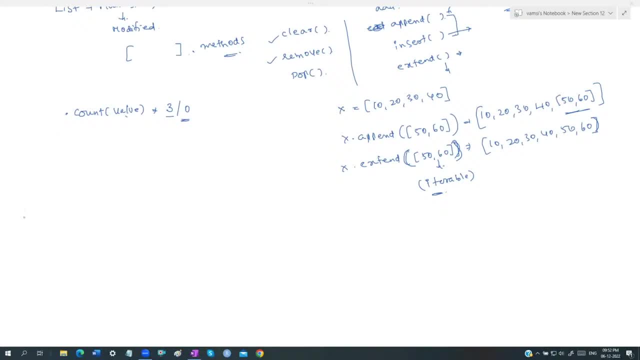 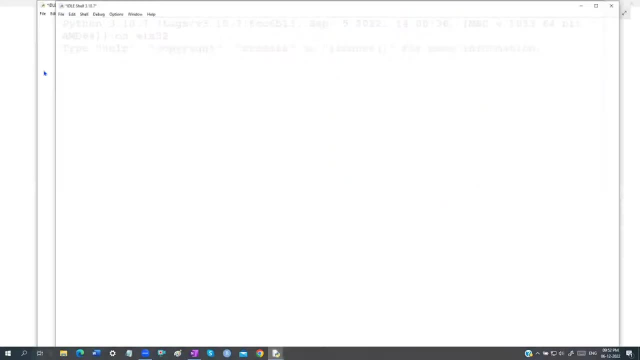 so who has been guys once again, who has been joined lately? so don't worry, um, i will take a backup session, uh, to cover all the previous topics, what we have been already. you have been lost. okay, have a look at this one technique, guys, otherwise we'll be sharing the backup session. 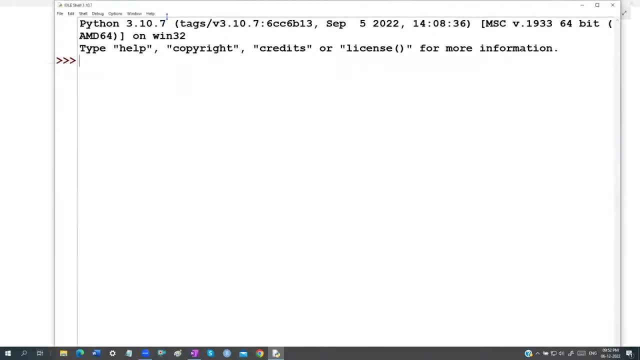 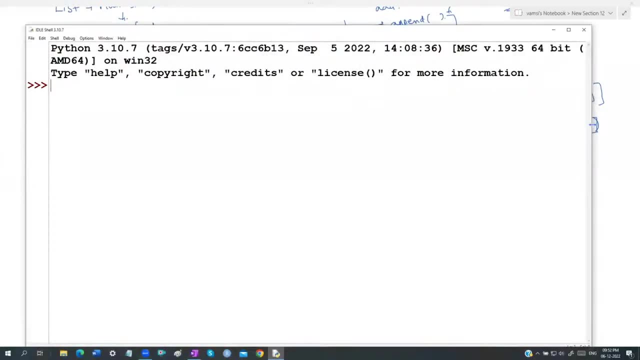 so the videos will be there. nowadays, everybody is doing the same thing, guys. they were sharing the video files, uh, the recording video, so that you can- uh, you can- just go through the videos and we can cover the previous topics. no worries, i'm going to take a backup session for that. 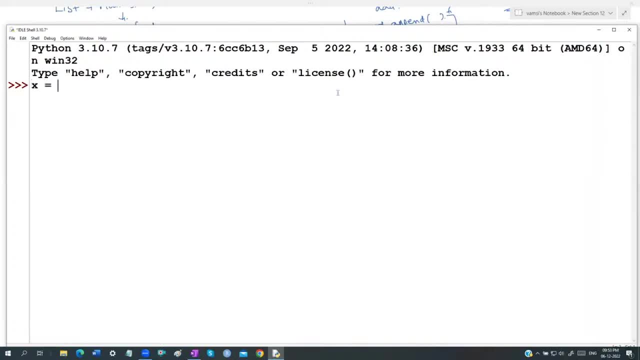 okay, have a look at this one, guys. x is equivalent to nothing, but it is going to be 10, 20, 30, 40. so it's going to be the elements, whatever what i have been added. actually, x dot. append off if i said 50. 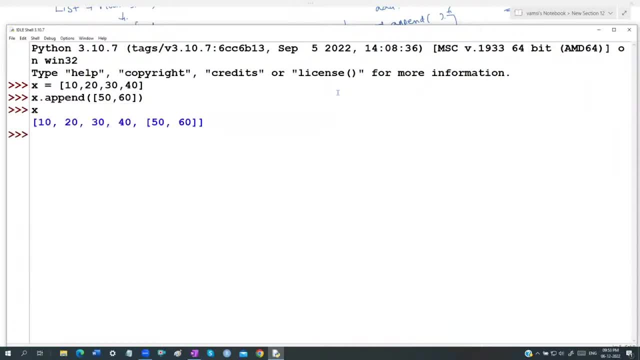 16. it is not going to be appending the 50 and 60 individually. actually, guys, you can see, 50 and 60 has been appended like this: actually, now i said x dot append off, which is going to sorry if i said extend off, if i said extend off, which is going to be the same technique, like 50 comma 16, they are. 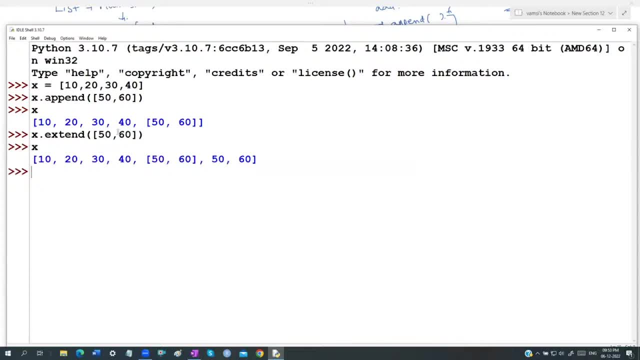 not appended as a single elements. actually, guys, they are not appended as a single element: 50, 60 separately. it has been appended. so if you append like that, it is going to be what we call it as an append. if you add, append like that, this is what we are going to call it as extent. what? 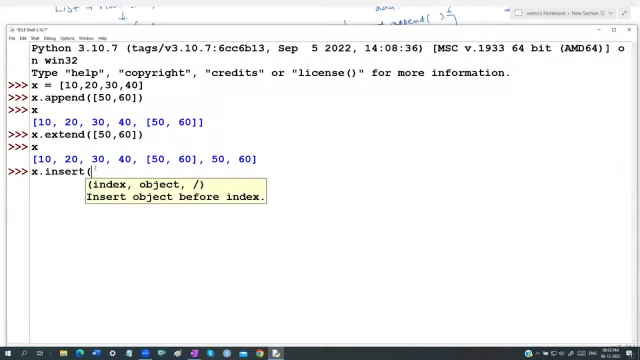 about the insert also. actually, yes, insert is also going to be appends at the given single element only. but we have to specify where you want to append it, actually, guys. for example, if i said 2 comma, it is going to be 50 comma, 60, then automatically 50- 60 will be appended as a. 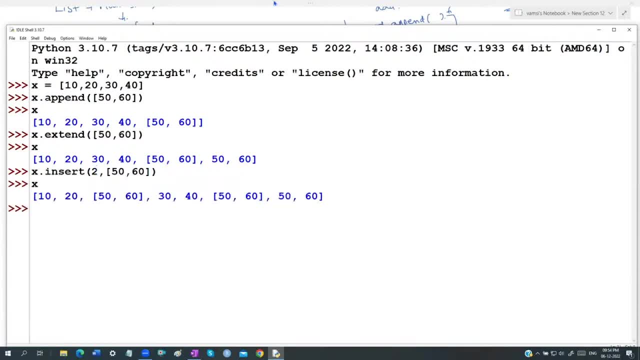 single element before the second index, it is going to be appended. actually, guys, that is what is going to be happening. yes, manohar, yes, go ahead. uh, yeah, in this extend method it should follow a particular format, like you know: 50 comma, 60, or it can be any like 50 plus 60 or something like how it is going to treat in that. 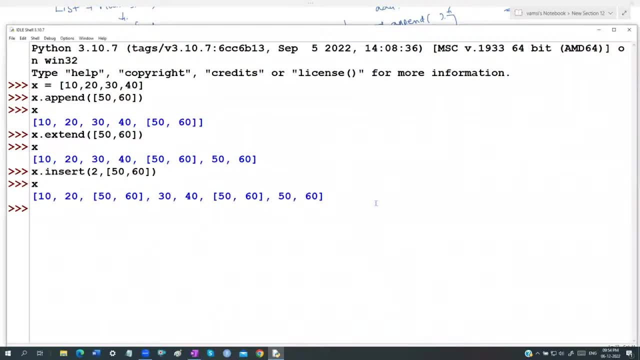 case, 50 plus 50 plus 60.. it's an addition. it will becomes an addition operation. no, no, it should be always separated with comma something. it's a separate with the commas only. okay, it is separated with the commas only. for example, if i said: this is the value. for example, if i said: 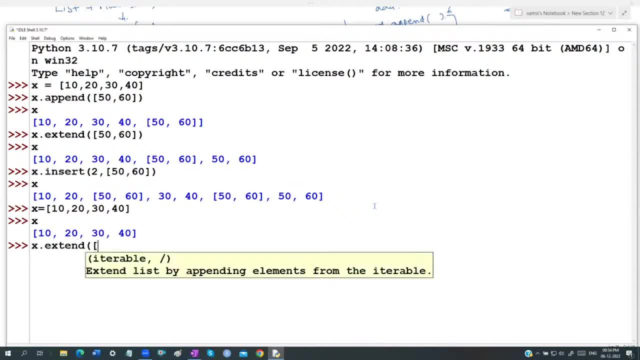 x, dot, extend off. for example, if i said, as you are saying, that it is going to be 50, um, okay, 50 space, space, no, no, it won't be, it won't be taken actually, because, uh, it's going to be something like an- okay, can you see, perhaps you forgot a comma. actually, because it won't accept. 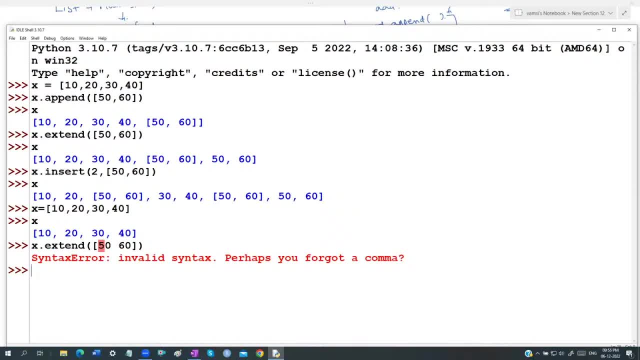 that actually okay. if i do 50 plus 60, it will. it will work actually, but it is going to be works as an addition operation operator. it is going to becomes actually it appended, but it appended. the result of 50 plus 60 as a 110 is the result it appended actually, right, okay, okay, fine, right, right, guys. 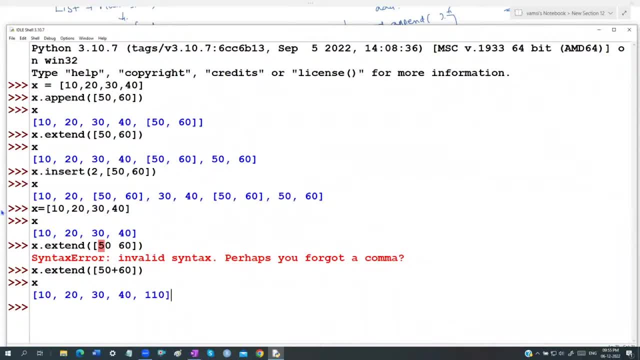 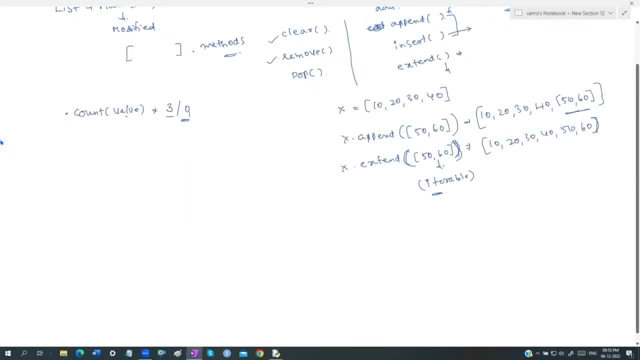 so this is going to be, uh, the one of the thing, what we can do. it actually, i guess now, up to now, whatever the methods we have been seen, guys like insert, append, extend, clear, remove, pop- all these are very, very simple methods actually. just anybody can just learn it actually. 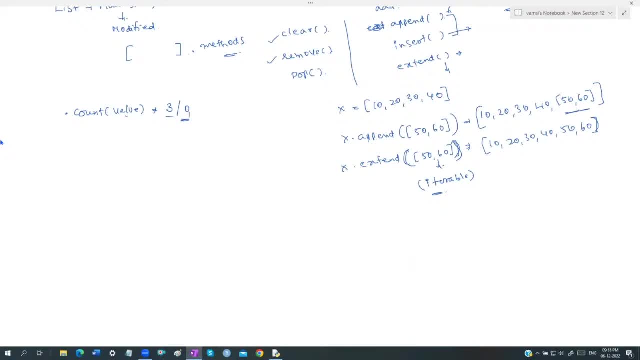 now it's not a complicated function, but compare with the previous function. the next function which i'm going to discuss is a little bit complicated work. actually it's a little bit complicated. that is going to be nothing, but let me do one thing. guys, i have some x is going to. 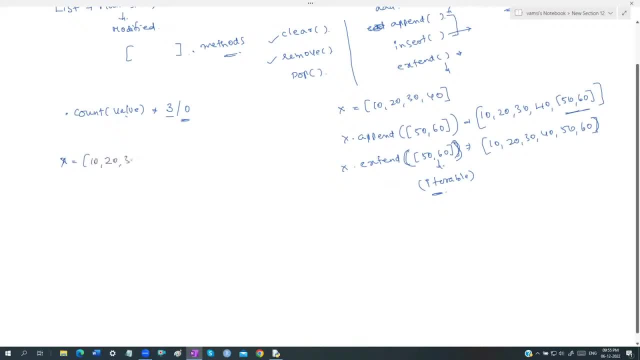 be there which is having some elements like 10, 20, 30, 40, just an example- 40, 50, 60, let us say 70, 80, 90. actually this 80, 90, 100, for example, total i take 100 elements. sorry, 10 elements. 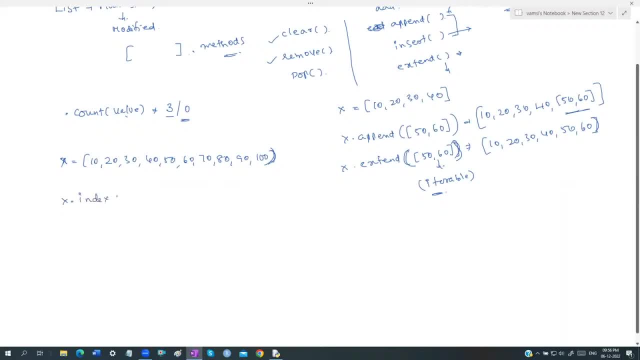 now what i said. actually, guys, x dot index. the method name is going to be guys. it is an index method. actually, guys, what is this index method will do? actually, guys index method is going to tells you the difference between count and indexes count will tell you how many times. 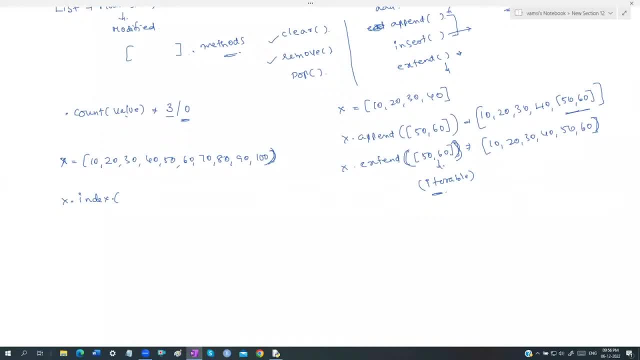 that particular value has been occurred, the number of times the value is occurred index is going to tell you where that particular value has been found, at which index i have been found. actually, for example, if i said which is going to be, i said, for example, guys 50. you know the index? no, guys 0. 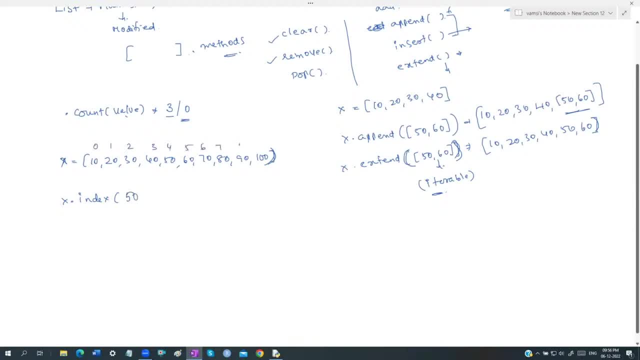 1, 2, 3, 4, 5, 6, 7, 8 and 9.. so obviously it is going to tell you. it is not telling you where is the fifth, how many times 50 is available. it is going to tells you, like it, which index i have find at. 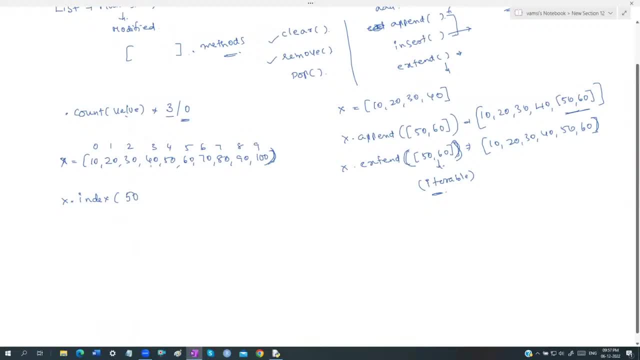 the 50. actually, obviously, we'll expect the answer as which is going to be nothing, but it's a 4.. but sorry, as you said that, um, sir, as you said that it is a little bit complicated, what is the complexity of this actually, guys? that is, you can sp, you can specify in between. 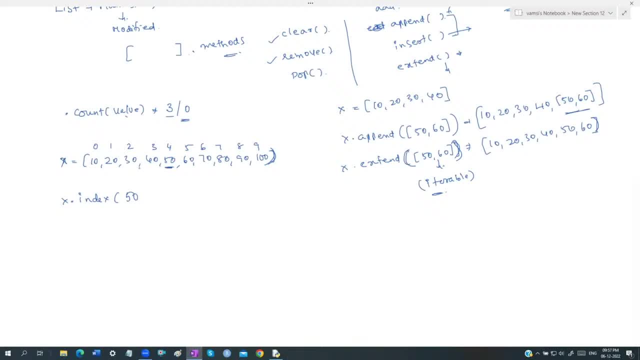 which two indexes i want to search. actually, yes, by default. if i don't specify, it will try to search directly, starting the searching from zero and goes up to the last. actually, one more thing is it will only tell you about the first occurrence. only even 50 is there. for one more time. 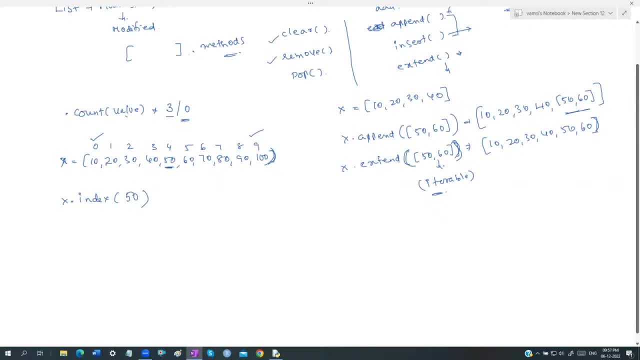 it does not gives you all the occurrences of 50.. only the index of the first occurrence of the given value. only it will find it off. but what is the extra thing we are having here is where to start your searching. also, we can specify guys. for example, if i said 0 comma 4, for example, 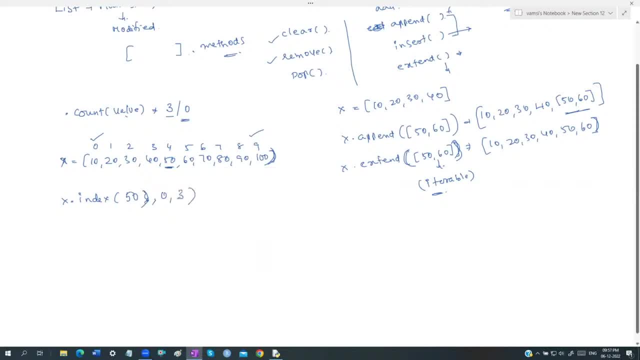 guys, or 0 comma 3, for example, then what it is going to do is: guys, you know what is 0 comma 3 guys? 0 means starting, 3 means which is going to be stopping, and throughout the python we discussed: actually, guys, this is going to be not included. this is excluded, guys. that means it is. 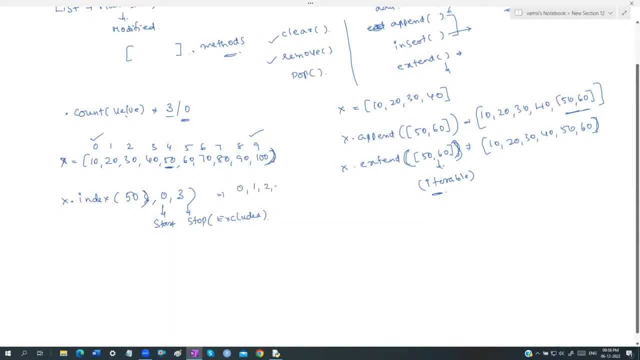 going to check only the indexes between 0- 1 and- sorry, 0, 1 and 2. only it will search. it won't search for the third index. actually, guys, that means in between these three indexes. only it will search out. where is the 50 is going to be there being the 50 was not there, it is going to throws. 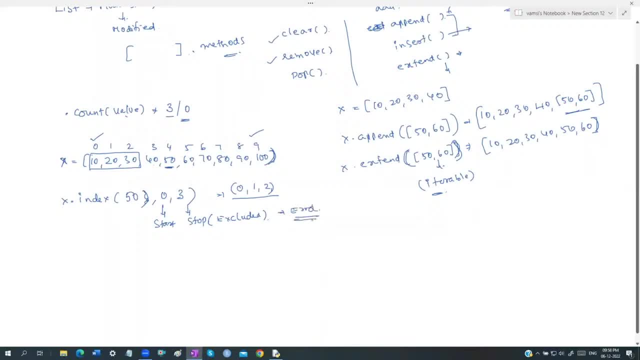 an error. actually, guys, if it is not there, it is going to throw the error actually. so by default, if i don't specify anything, it will start with the first index and goes up to the last index. wherever the given value is there, it will tell you the index. 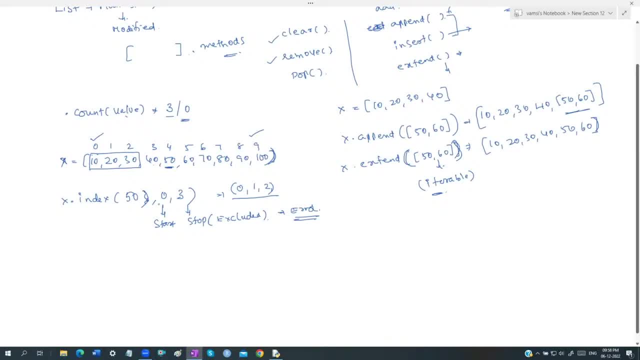 but there is an extra option: is there where to start your searching? for example, if i said, actually the 50 is there at the fourth index, actually, guys, for example, if i say i want to start searching from fifth index, actually, so it will start searching from the fifth index, it will. 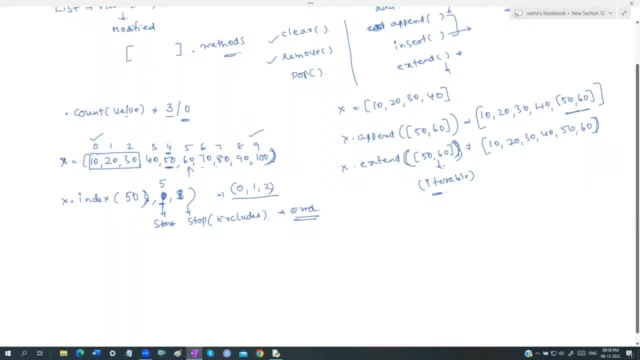 find out. do you find the 50 in the next elements? no, you will get an error. actually, if it is there, it is going to give you the value, actually, guys. okay, so it's a little bit a complicated way, because it is going to be taking totally three parameters. actually, guys, it's taking three. 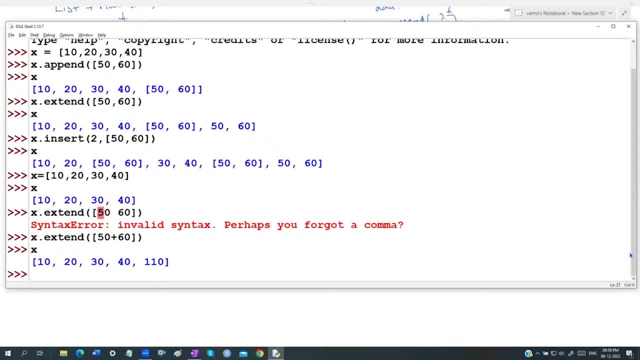 parameters. it is taking it actually, guys. up to now we have been seen clear: does not takes any parameters, guys, no arguments. it will take it. remove and pop is going to takes one argument actually, guys. remove will take one argument. pop also will take only one argument only. 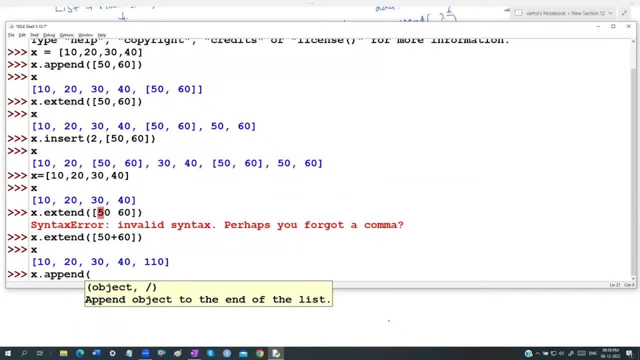 next one, append, is also going to take one argument only and insert is going to takes two arguments. actually, guys, index and the object and even the extend is also going to be- tells you takes only one argument only. it will take it, which is an iterable object. but whenever we talk about 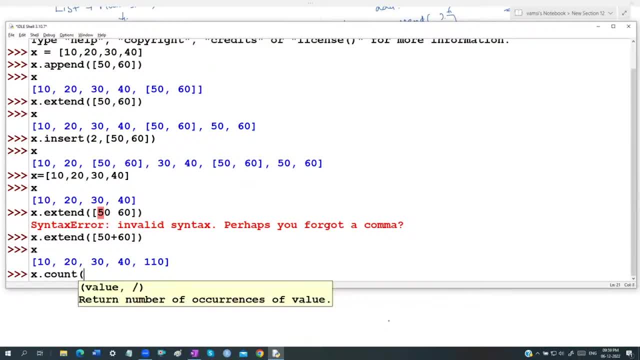 a count. count also returns takes only one, one input only, which is nothing but a value it is taking. but see the index. actually, guys, index will take three arguments. guys, value whatever the value you want to return what, whatever the value you want to search. return the first index of the given value. 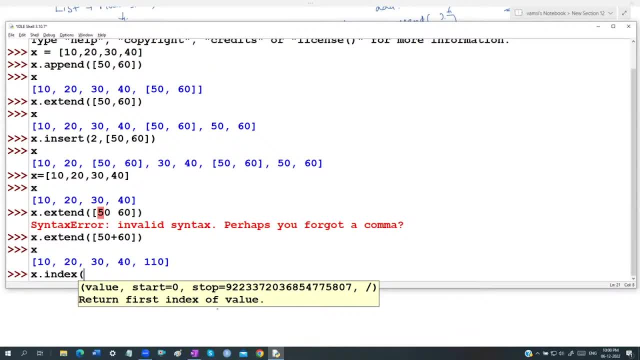 wherever it finds, the index it is going to tells you, actually, guys, starting is going to be zero, see the stopping. actually guys, a very, very, very, very large number. actually guys, a very large number. if i don't specify it will start with zero and goes up to the last element: almost all a very huge number. it is. 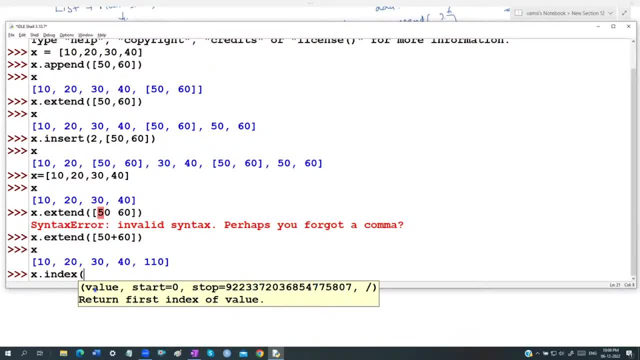 taking it actually. yes, now let us talk about x dot index of. i want to search for 40. actually, guys, where is the 40? is there in between zero to the last element? it will start with zero and goes up to the last element. index is going to be nothing but it. 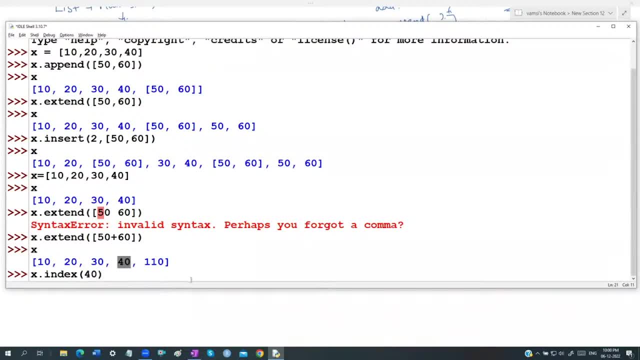 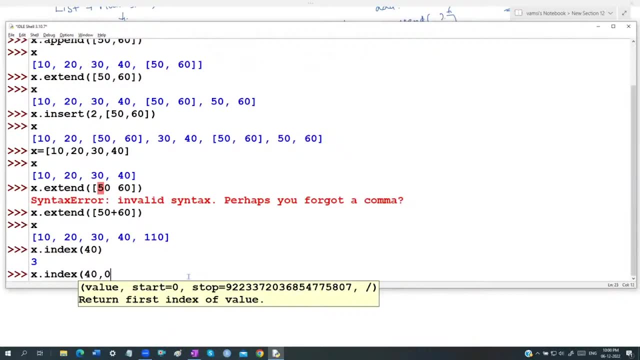 is a fourth element. we know that index is three. actually, guys, your index is going to be three actually, but if i said x naught index of 40, i said that i want to search only between zero. and let us say that only the third index, only third, is not included, actually, guys. 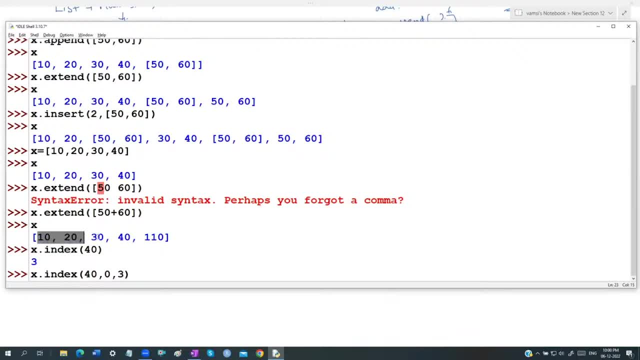 when i said 0 comma 3, it only searched for 0, 1 and 2. only in this particular three elements is the 40 is there we are asking. please find out the index of 40 in between 0 to 3. i didn't find any. 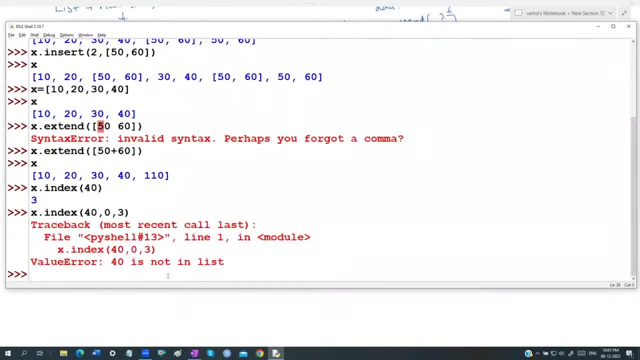 kind of a 40. there you are going to get an error. actually, 40 is there in the list. 40 is there in the list, but it is not existing in between the 0 to 3, 3 is not included. we know this actually, guys. 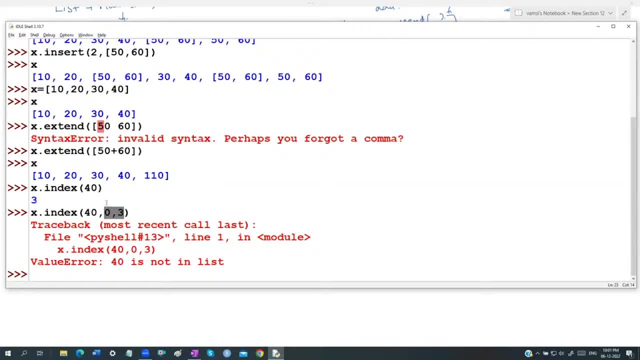 really, if 3 is included, we have to get the 3 as the result, because that is that sorry. 40 is there in the third index. actually, if you want, we can take a little bit more numbers. let us say this actually, guys. let us just an example: x is equivalent to nothing but 20, 34, 12, 45, 67. 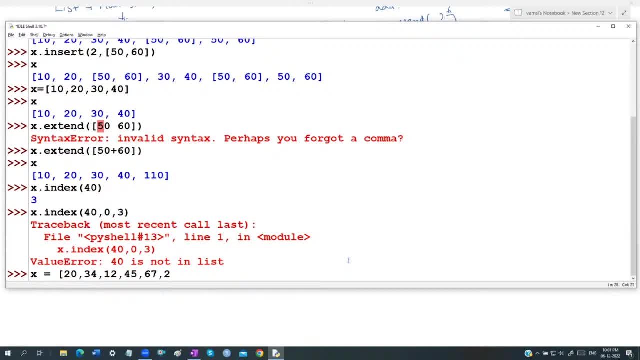 25 and it is a 10 and it is a 2 and it is a 3, let us say 40 and let us say 96 and let us say 72, some random numbers only. i'm going to be taking it. actually, guys, i'm taking some kind of a random. 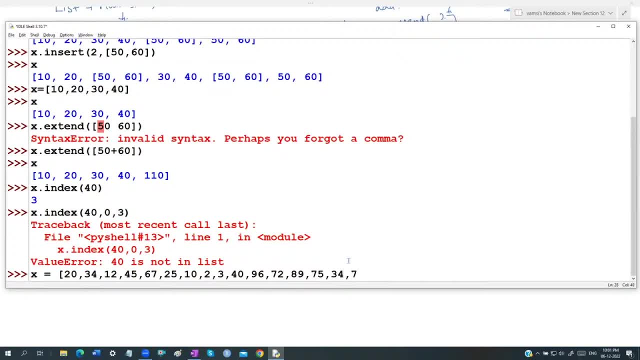 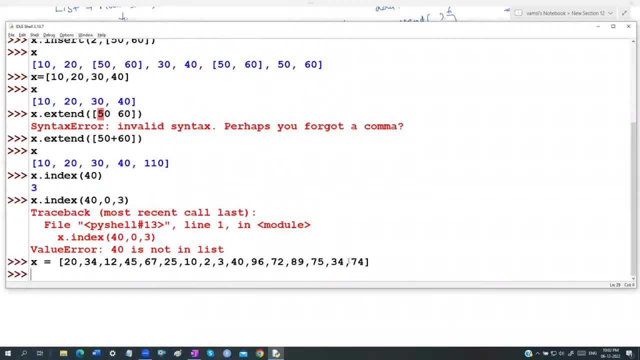 numbers. only i have been got taken. actually, let us say something like n, 78 or something like a 75 or 74, i have been got taken. just an example. i'm talking about that. i know that in that the least value is two guys, let us say that the least maximum value is two guys. let us say that the least 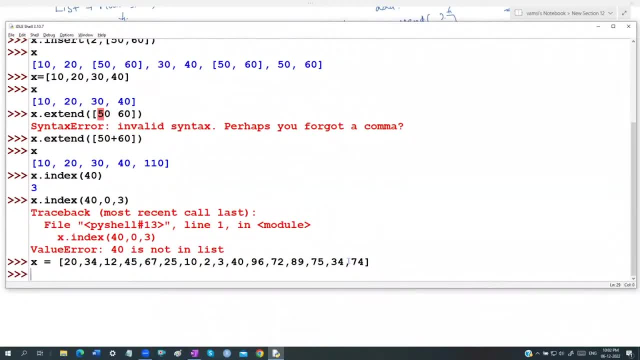 marks. let us say these are the marks of the students, guys. sorry, these are the marks of the students. now i know that least value is going to be 2 and the highest value is going to be 96. actually, highest value is 96, isn't it? now i want to know which index has got the least value 2. 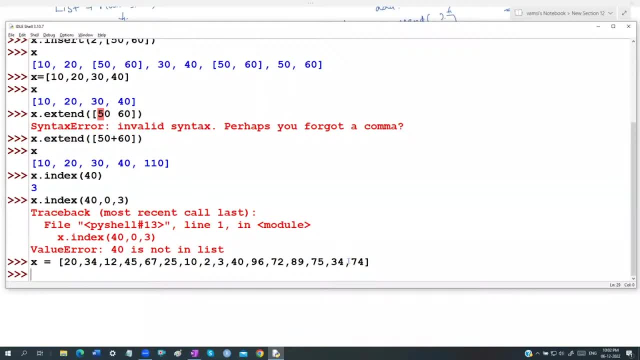 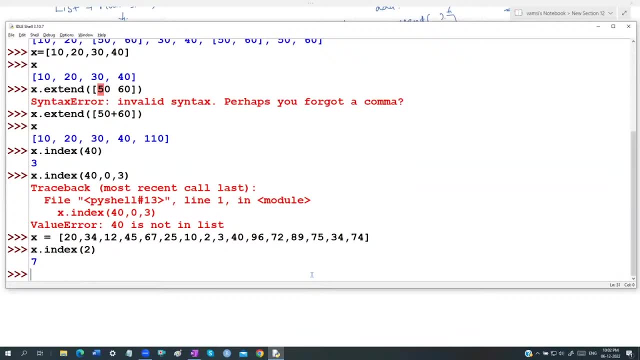 and which index has got the highest value, which is going to be 96. actually, guys, a simple process: x dot, which is going to be the index of 2, it is going to tells you so at which it is going to be there. seventh index means it is the eighth element. actually, guys, seventh index is: 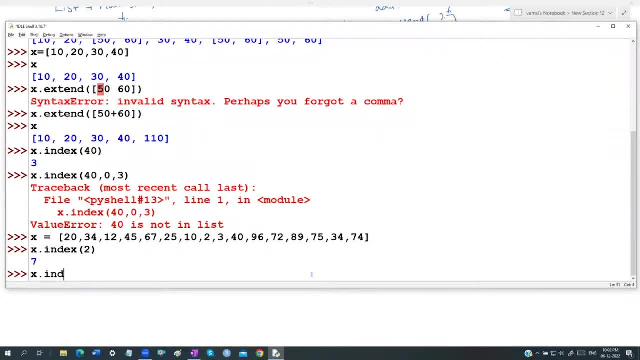 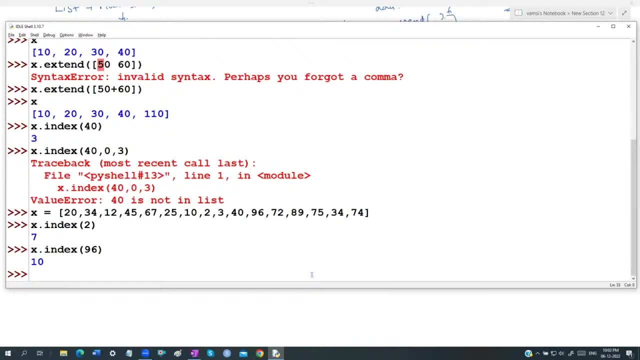 nothing, but it's an eighth element in the list, actually, and where is the highest value of which is going to be 96, actually, guys? so it is going to tell you that it is going to be at the 10th index. actually, it is going to be in the 10th index actually. for example, if i said x dot index of 2. 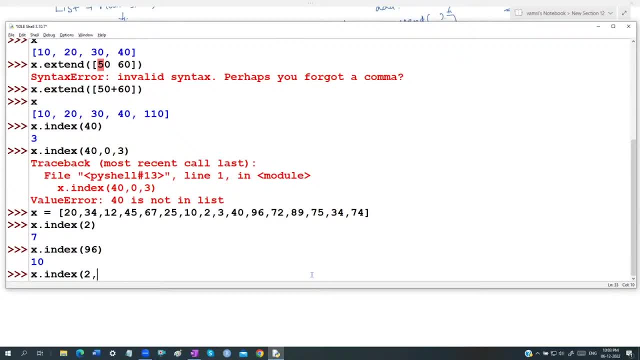 but i don't want to go for all the elements. i want to check for from the eighth element. do you have any two is there? i'm asking the starting index at eight. actually start from the eight, go up to the remaining elements and tell me do you find that particular two? no, i didn't find that particular two in the. 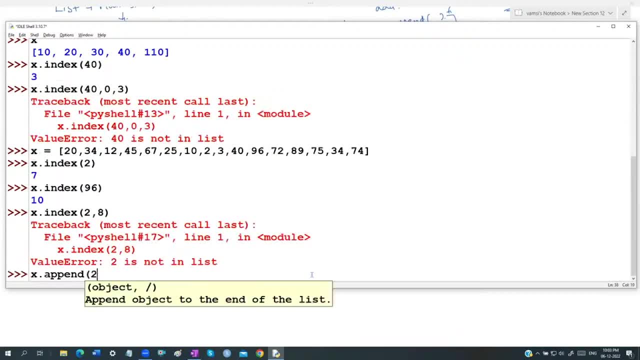 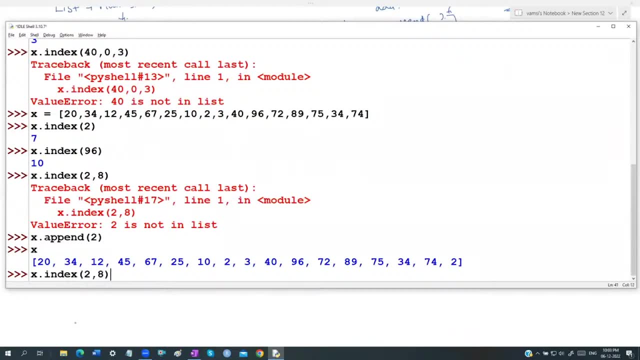 list. i said: x naught append of two. actually guys, you can append the elements: no, guys, now there is two. is there for second time? actually guys. now you ask: x naught index of eight, two comma eight. so this is zero, one, two, three, four, five, six, seven, eight guys. it will start from here. 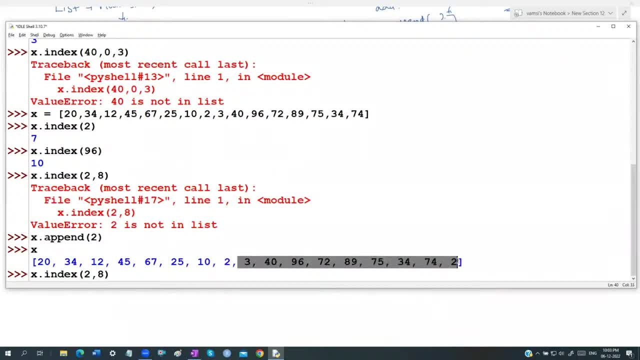 and it tries to find out where is the. who is there, as the case. so two was found in the last index actually, so i don't know how many elements are there, but if you count it, one, two, three, four, five, six, seven, eight, nine, ten, eleven, twelve, thirteen. 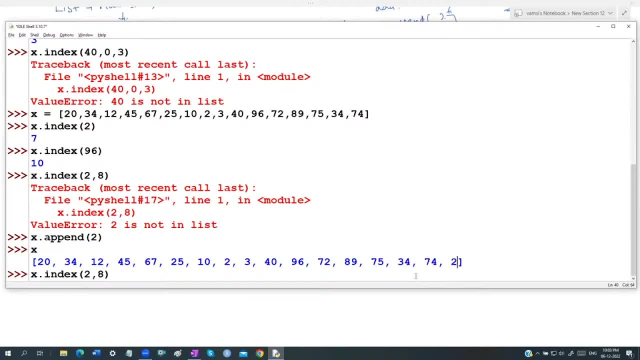 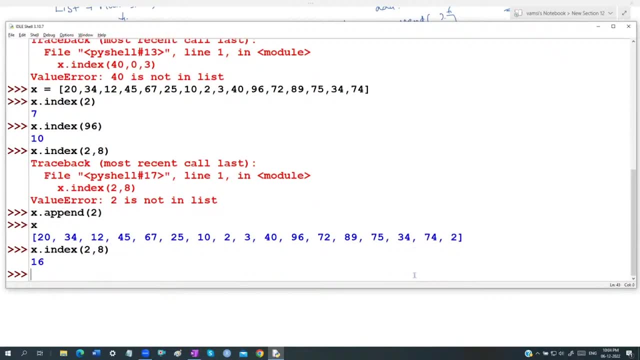 fourteen, fifteen, sixteen, seventeen guys. so it is going to be there. at the 17th element, which is going to be the index is going to be nothing but 16 is the index. actually index is going to be same as it is, guys, i'm not saying that. start from the eighth index, count it. 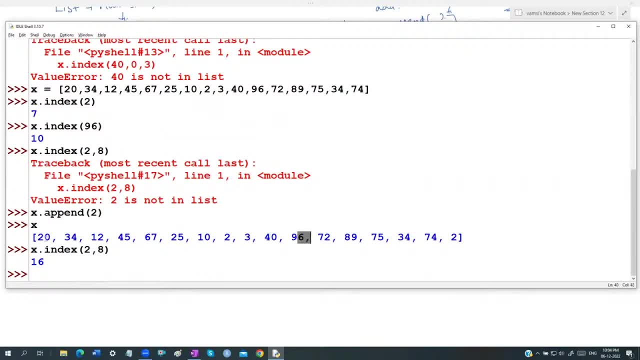 0, 1,, 2, 3.. I'm not counting it. actually, guys, Counting is from 0 only, but I'm starting searching from the 8th index. actually, Start from the 8th index. Do you find any occurrence of 2? Yes, 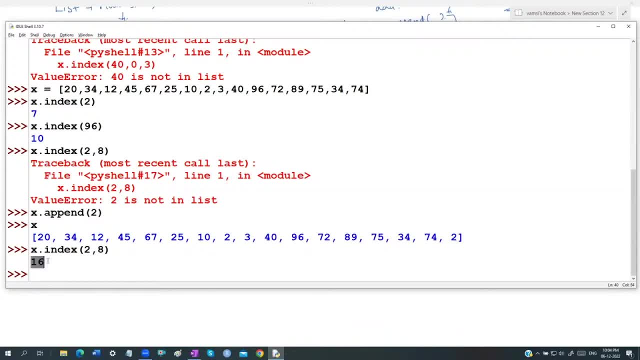 I find that the occurrence of 2 here, which is going to be nothing but the 16th index, actually guys. For example, if I do the same thing by writing x0 index of 2 comma, which is going to be, I said, 8 comma 15- actually guys, 8 comma 15 means we know that In between 8 and 15th index. 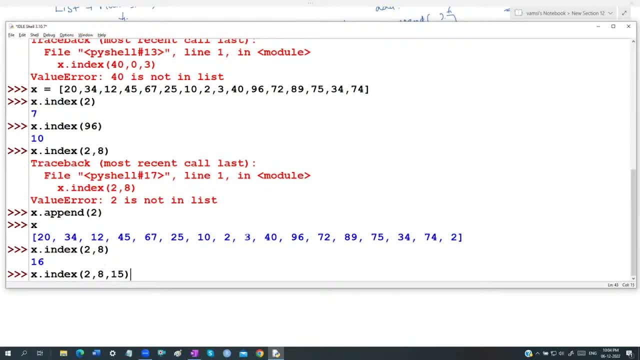 only it will find it of actually guys. I know that this is 8.. 15 means 15 is not included guys. 8, 9,, 10,, 11,, 12,, 13,, 14.. Only in these particular 6 or 7 elements only. it is going to check for the 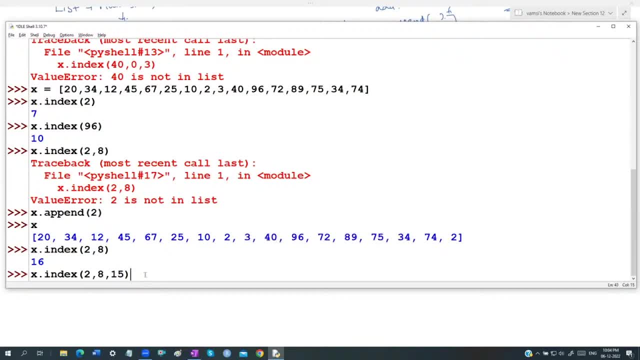 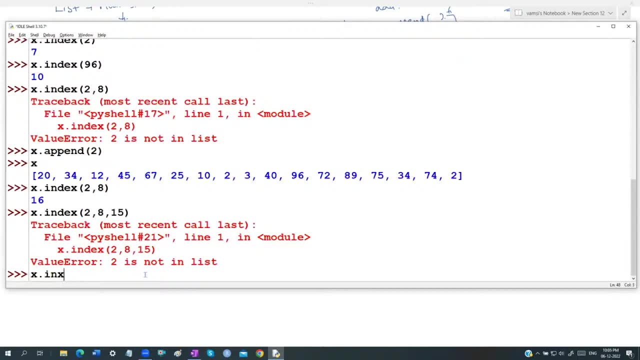 2 actually, but 2 was not there, Then obviously we are going to be getting an error, actually, guys. So x0 index will work with a single argument. It can work with a single argument, guys, as well as even it can work with two arguments, I think. 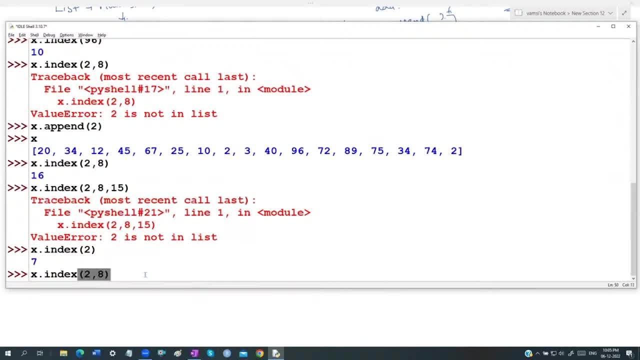 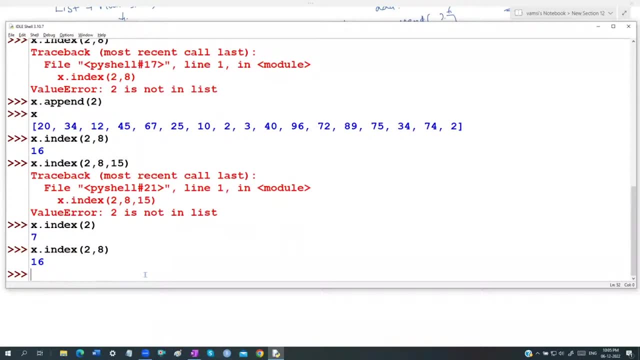 you may be having a little bit idea about this, guys. No worries, In Python we are having a discussion of functions concept. When I discuss about the functions concept, then I'm going to discuss completely about this arguments concept. once again, It works with two arguments as well. 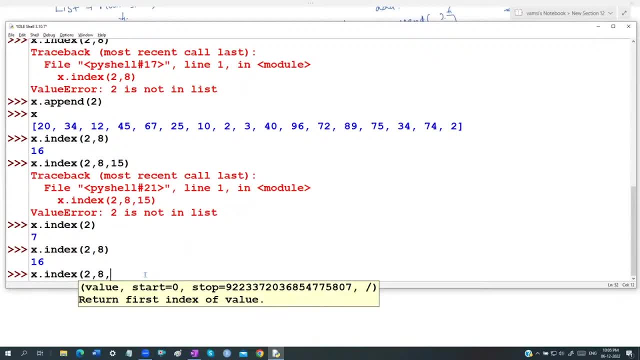 as it can even works with, which is going to be three arguments also, it is going to works. actually, guys, We can also write the third argument, like 5,, 6,, 7,, 8,, 9,, 10,, 11,, 12,, 13,, 14,, 15,, 16,, 17,, 18,, 19,, 20,, 21,, 22,, 23,, 24,, 25,, 26,, 27,, 28,, 29,, 30,, 31,. 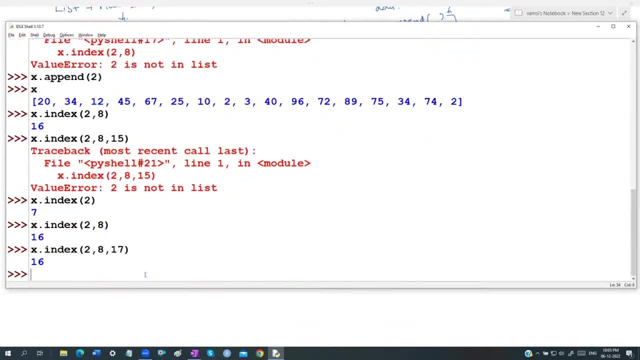 32,, 31,, 32,, 33,, 34,, 35,, 35,, 36,, 37,, 38,, 39,, 40.. So I will write it as a 17. actually, guys, Execute it is going to works, but beyond that, if you give, you will get an error, actually guys. 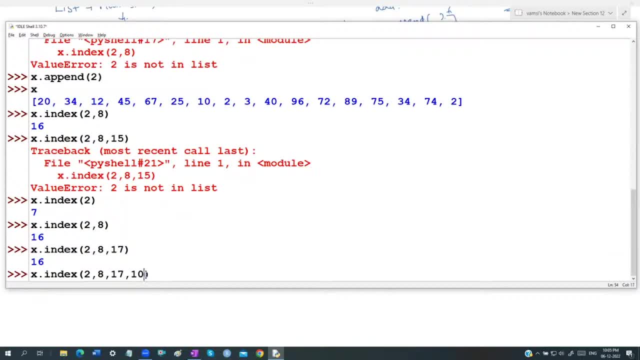 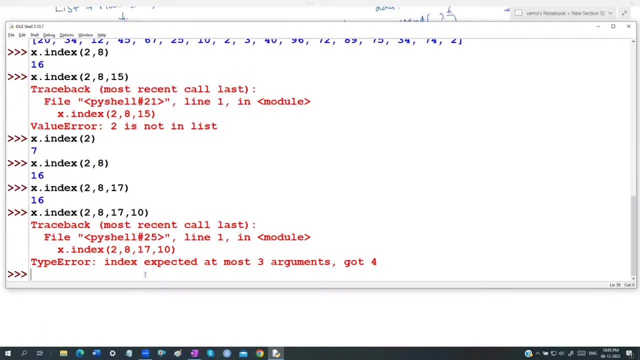 Hope all of you have an idea about that While you are calling the functions. while you are calling the functions, how many arguments we have been got defined. only that many arguments only. we have to use it Anyhow as part of our course curriculum. we are, as part of the Python discussions, we are already having a discussion about the functions. 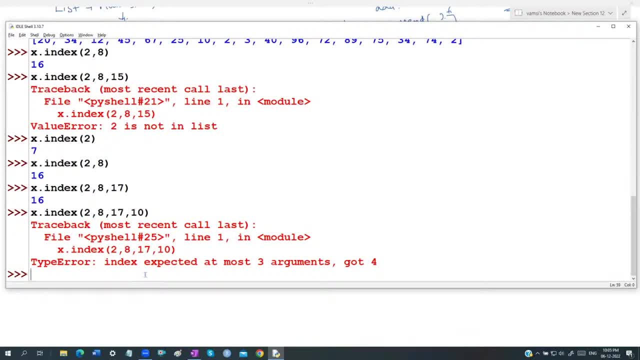 concept. guys. We look into the functions concept. We look into the functions concept. We look into concept more and more. we are going to look into them. first. we look into the more into the functions concept. okay, so we have a discussion. if i want to find the value before index 8, i should use: 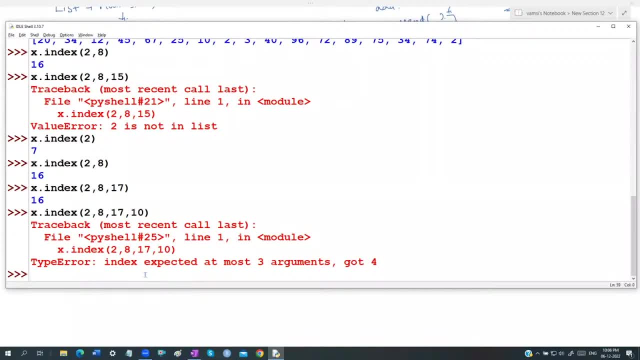 the negative indexing or is there any other way to mention it? you want to check, i want to find a value before index 8, for example, between 1 to 8, let's say okay, then you have to specify that actually. okay, there is a technique. is there x dot index? is there no? no, it's not negative index. 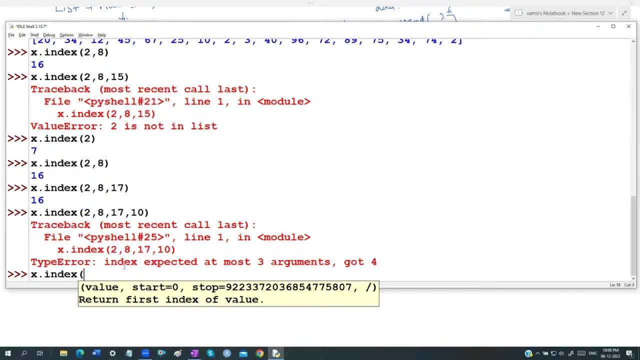 um, okay, okay, actually, um negative index means nothing, but it will start only from the right hand side index. only see, if i say negative index, for example, if i said negative index of, for example, x dot index of 2 comma minus 4, in that case what it will do is minus 4 means. 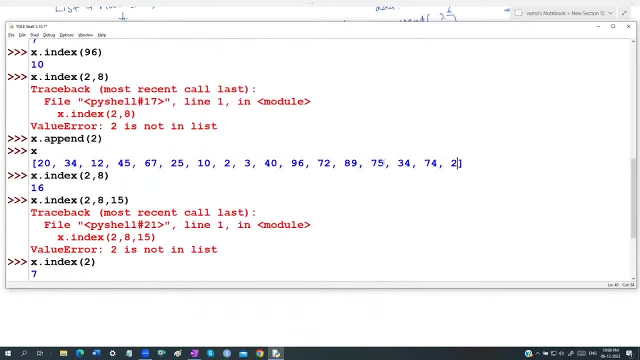 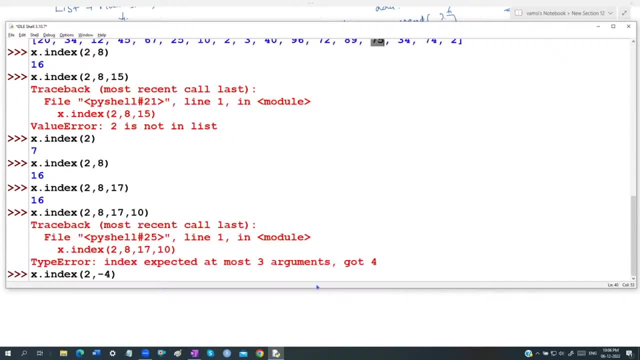 minus 1 minus 2, minus 3 minus 4. it will start checking from here only okay, okay. so then the result is going to be obviously: 2 is, at the last, only, which is going to be obviously. we'll get the 16 as a result, as usual. 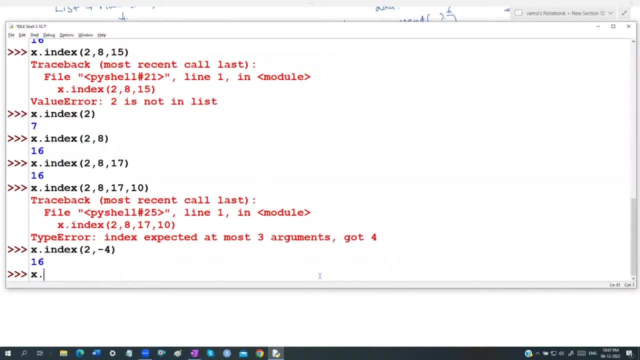 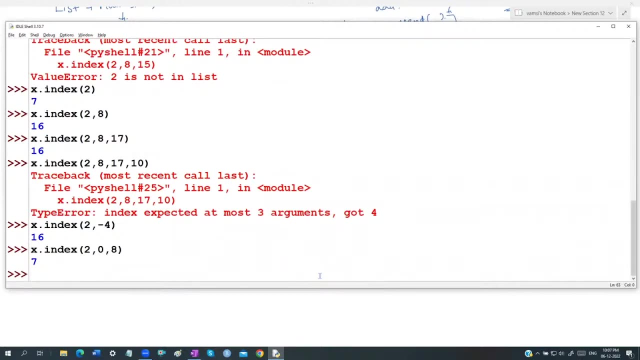 okay, okay, that does not matter about that, it is going to be. for example, if you want to search before the 8 means, then you say that it is 2 comma 0 comma, 8, so before the 8 only it is going to search for the index actually, okay, yeah, then you are going to be getting 7 because 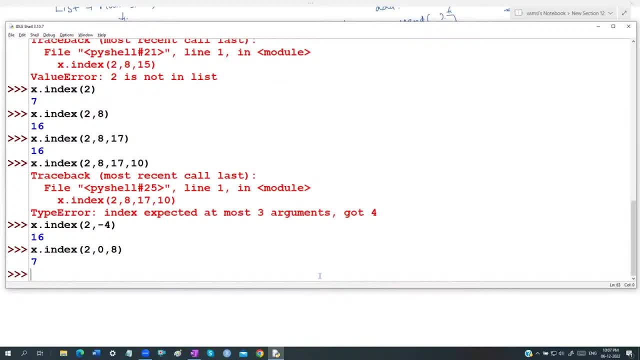 it is there at the 7th index before the 8. only want to check it out. actually, you are going to be getting 7 because you are going to be getting 7, because if you want to make it complex later, that means in the coming applications, we'll put it in a loops. 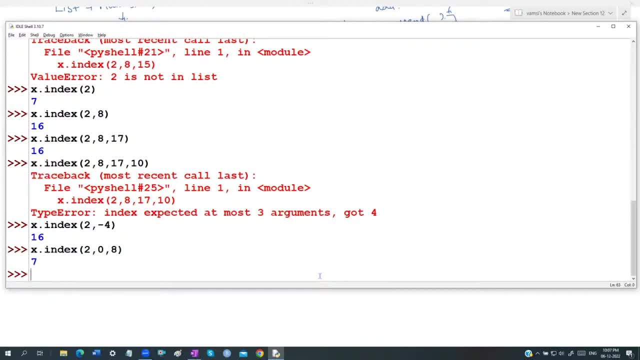 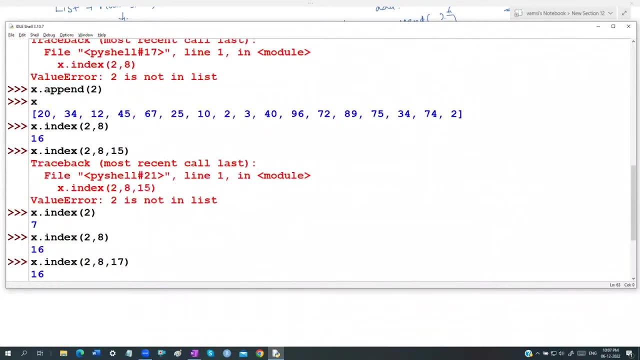 we'll write some if conditions and then you can write the applications. actually, in case, if we give a range between no zero to eight, no, no, it won't work like that. it's an. arguments are completely uh, these, these functions, these methods, scope is very uh, limited. only, whatever they define, they have to work like that only. okay, if you want to do that. 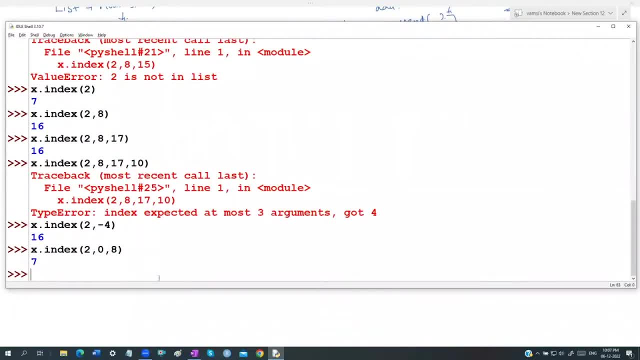 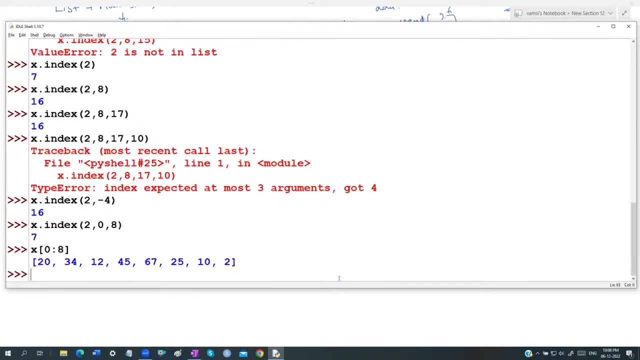 there is another, techniques are there that means see, uh, in that cases, what we are going to do is: first, we are going to do some kind of a slicing like this actually, okay, this is a concept of slicing concept. we are going to do that. this is actually a list only. 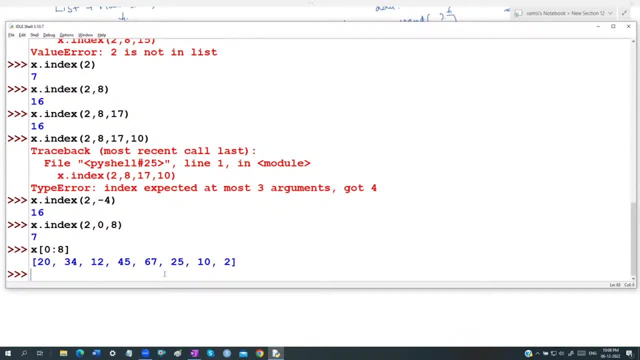 then you can find it off. for example, x of 0 is to 8. within this particular range, dot, i can say the index of 2. actually, now what is an output will come? actually, x of 0 is to 8 is going to be one list. so how many elements are there? one, two, three, four, five, six, seven, eight, we are going to be 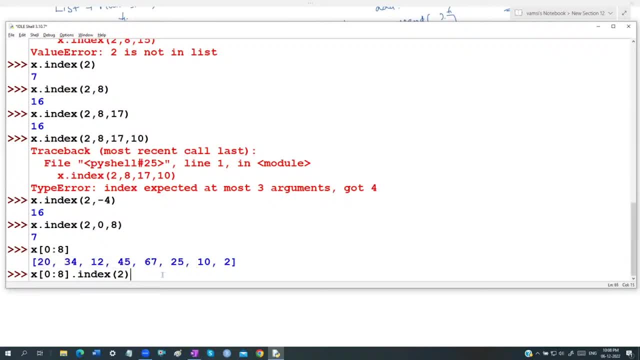 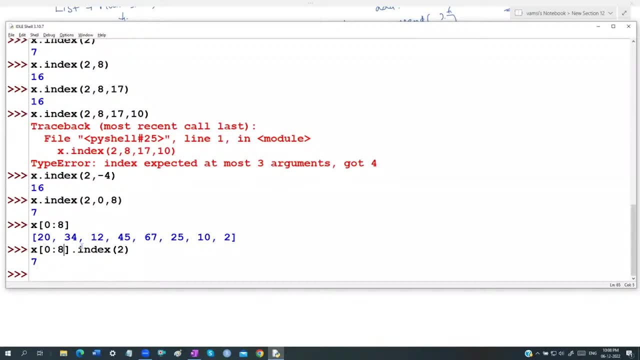 that is, um, we are getting eight elements, then obviously the index is going to be nothing, but seven will be the result. for example, if i said eight is two, uh, maybe, uh, if you have already attended slicing concept, so what is meaning of eight is two? actually, eight is two means: 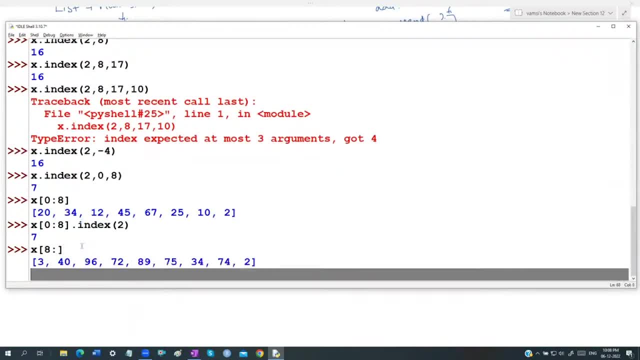 starting from the eighth element. remaining elements will come actually. so in this case, if i said which is going to be dot index of two, now it is going to be with respect to two, that means this index will be taken as zero. now zero one, two, three, four, five. 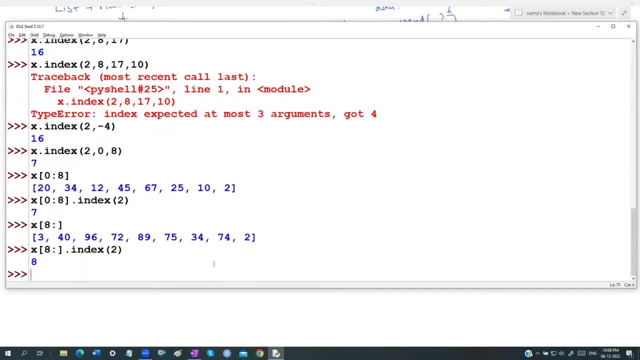 five, six, seven, it will become eighth index, it will become actually. so we have to use some combinations and we have to work with their applications. actually, yeah, i'm sure my question is, like you know, if you have a duplicate, you know number like two, right, if you have two occurrence. 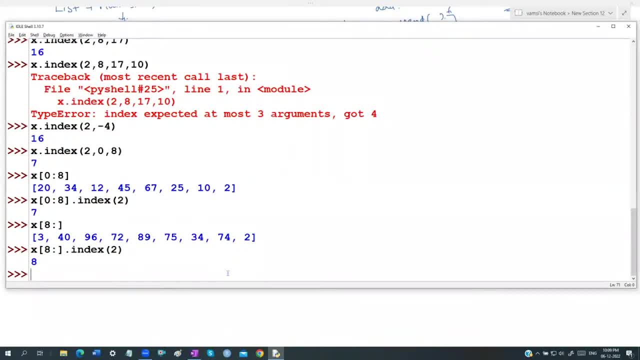 so i'm going to get two indexes at which place is actually no, no, first one index only will come, only first index, only first index only. that's why see you here also we have the second index. is that two is there for two times right? correct when i said x naught? 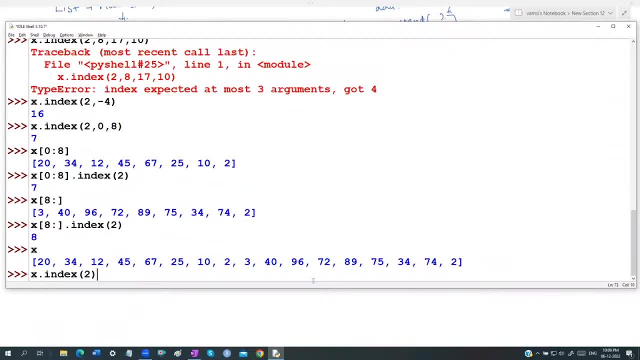 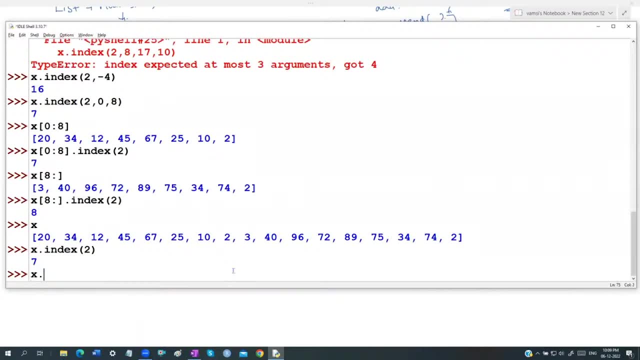 index of two- it always starts with the zero index- and find out. the first occurrence is going to be here, which is going to be at the seventh index. okay, yeah, okay now. the idea here is: now you want to find the second occurrence, then what you have to do. i know that the first occurrence of two is: 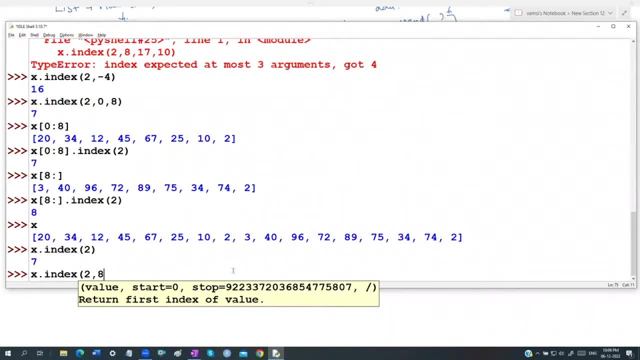 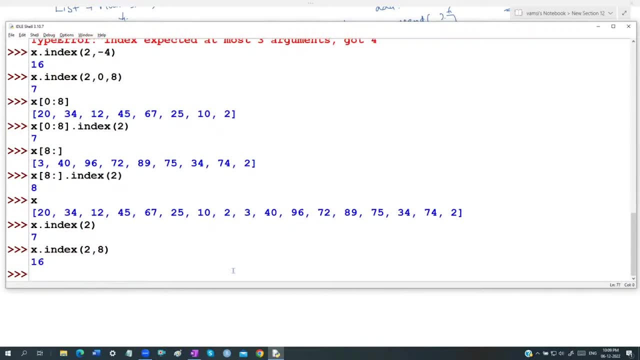 there at the seventh index actually, then i'll start from the eighth index. i'm going to start with that. then obviously i'll know, i'll come to know about the second occurrence of this particular values. okay, okay, okay, thank you, but these are all the basic things. so python provides you a lot of advantages. 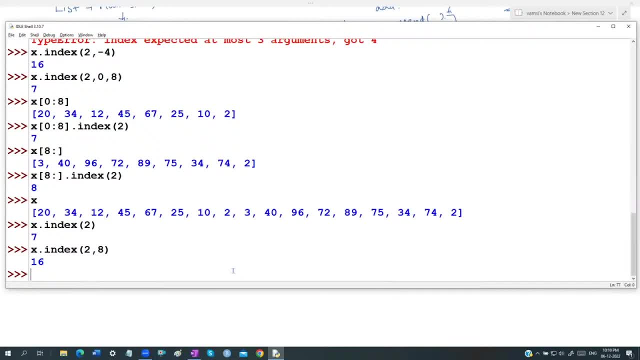 that means these concepts, we. if you really want to do that, you need not to do like this only in a complicated way. in coming applications, we have a lot of techniques and lot of implementations will come. you can use those particular things and we can do it actually. okay, fine, yes, right. 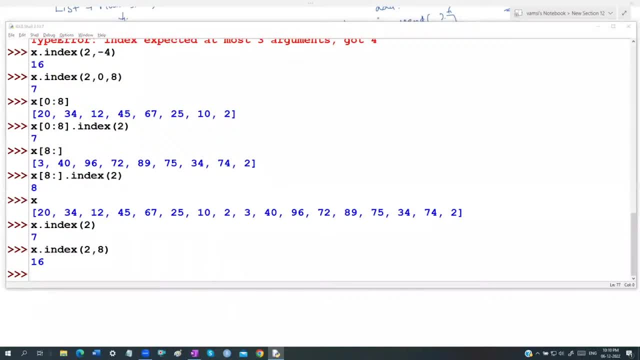 yeah, yeah, hello, uh, so, uh, is there any uh predefined function to get that maximum or minimum? yes, absolutely, we have it actually so directly we are having, see, we are directly having the kind of functions. actually, what is going to be the minimum of x, what we are? 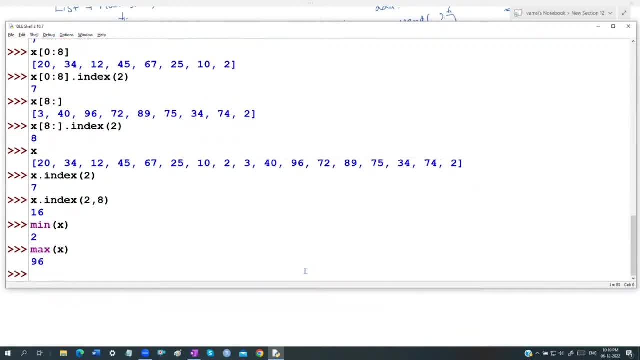 going to be getting. what is the maximum? of x is going to be there, so you really don't require this actually. but things, guys, one thing i want to explain here is this list, and all these things are the one of the basic structures of the python actually. so how to do the manipulations on this? 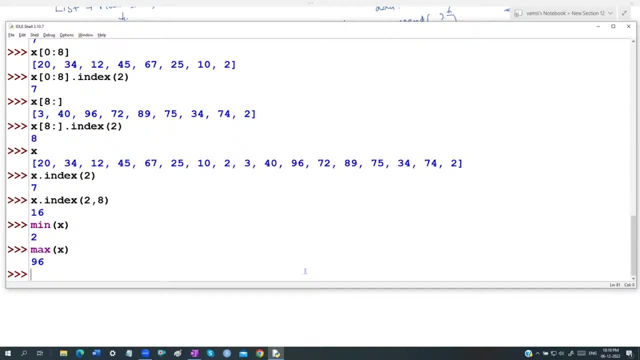 list. we don't recommend them actually, because it's not guaranteed that a list will always contain always a numbers only. sometimes it may contain some numbers, some strings, some bools and some floats. it may contain different, different values, so you can do that, but what i'm saying here 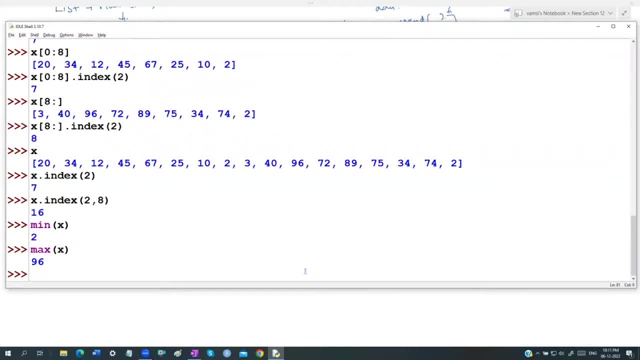 is, instead of using this min and max functions here in python we are having a very, very advanced levels applications are there. advanced level mathematical applications are there. whenever we go there, we can do that kind of an applications further timing. what is a list? how to handle the list by using that? 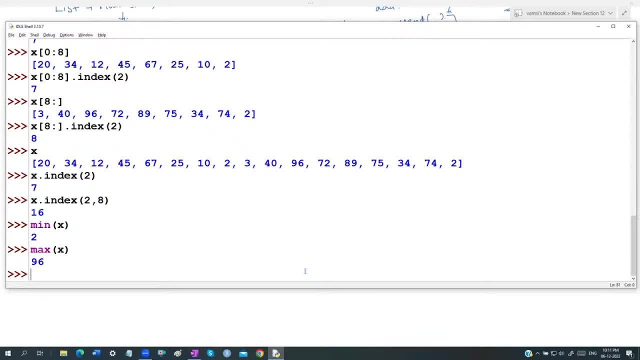 particular methods, that's. that's it actually, guys. don't try to do any manipulations with the list, like: what is clear, what is remove, what is a pop, how to append the elements, uh, how to go for this particular extent. all these are ideas only to make you understand how to use the methods. actually, guys. 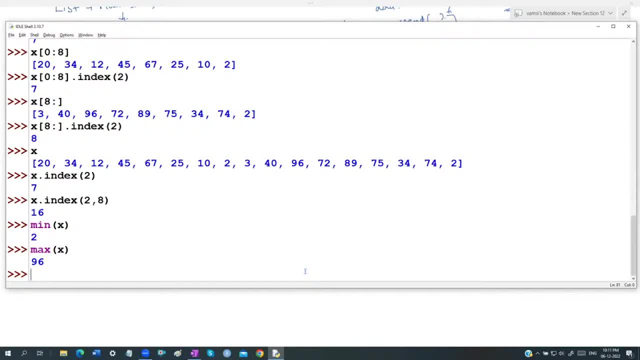 actually we are using some. i'm explaining some methods, actually guys. out of that i may use only three methods only i'm going to use maximum guys. i'll use append method or extend method. only these two i'm going to use mostly remaining i don't use at all. but why we are discussing here is this is: 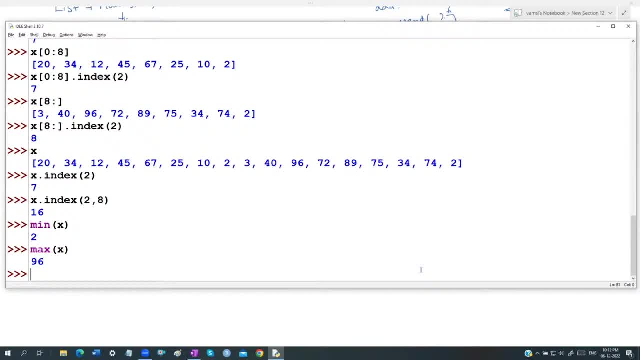 my first object i'm explaining, so i have to explain each and every method that is associated with that, whether there are used or not used that we discuss it later about that being. it's my first example of a of an whatever the object in python remaining objects. they don't have it actually, guys. 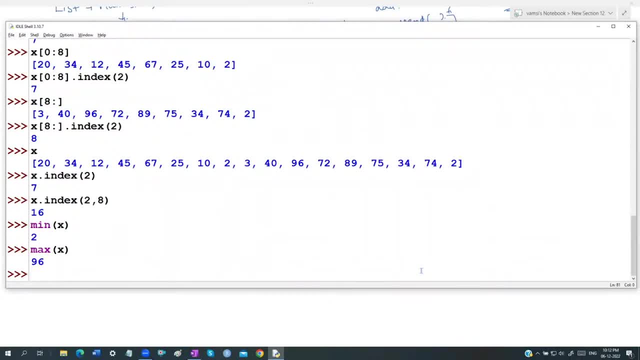 is the first object. i'm discussing about that. that is the reason why i'm explaining all that kind of methods actually. but you will understand why we are learning. we'll get some clarity about that. we'll understand the concept behind that, so in coming classes it will become very easy for us. 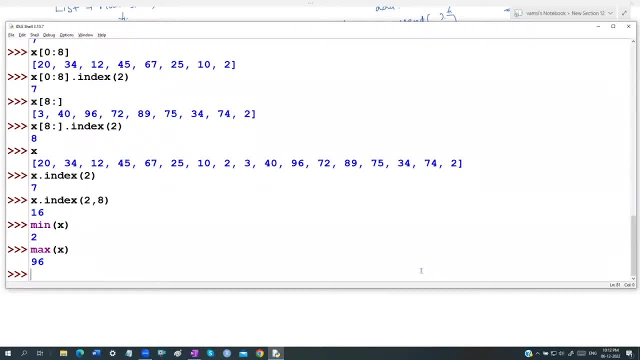 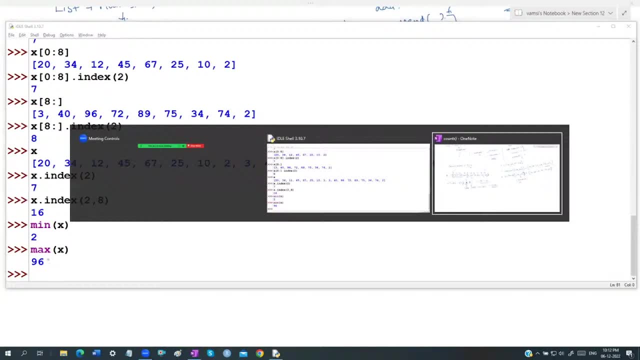 if i discuss only one or two methods and leave it, you don't get a practice on that. actually, that is the reason why i'm explaining this. okay, fine guys. so once again, guys, what is going to be? this index method is going to be do? it is going to be nothing but dot index of. 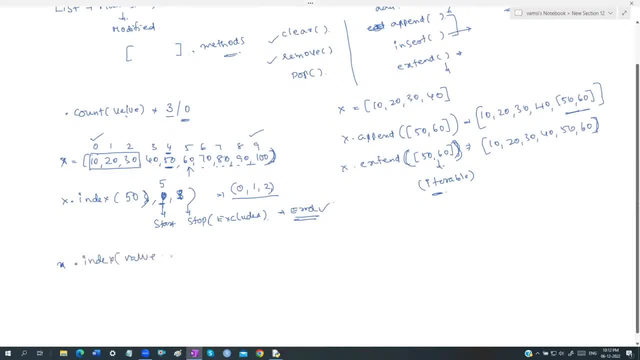 which is going to be nothing, but whatever the value, and what is going to be the starting and what is going to be the stopping value, actually, guys, so it is returning a value observed carefully, guys, i'm specifically pointing out, i'm specifically pointing out, actually, guess which methods are. 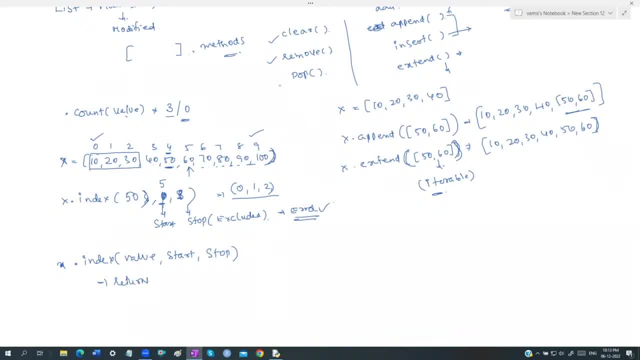 returning which methods are not returning? pop method will return a value back to you guys. when you run a pop method, some output will come, but when you use the remove method, no output will come. when you execute a clear method, no output will come. even append, insert, extend also, they don't give any outputs. count will give you. 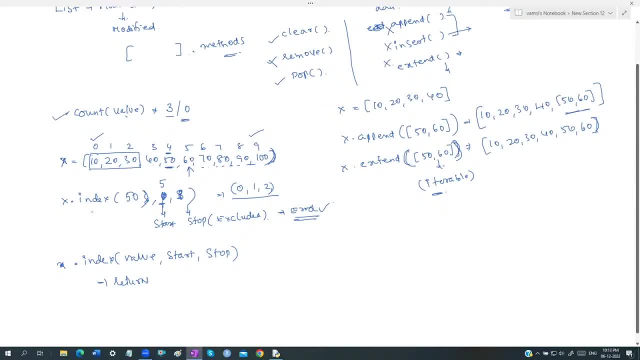 a output. actually, guys, count is giving an output, index is also going to be giving an output. so, out of the seven or eight methods, or nine methods, I discussed only two methods. three methods are returning guys. one is a pop is returning. I'll conclude: guys, totally, pop is returning count. 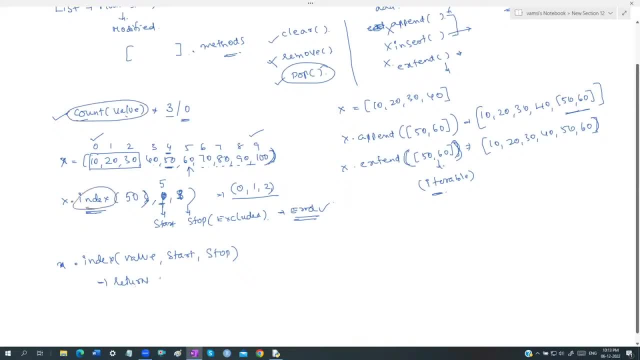 is returning and index is returning, actually guys. so what it is going to returns returns the, which is going to be the index of the index of the value. it is going to be the index of the value between, which is going to be the starting and the stopping, actually guys. so I need not to explain every time. 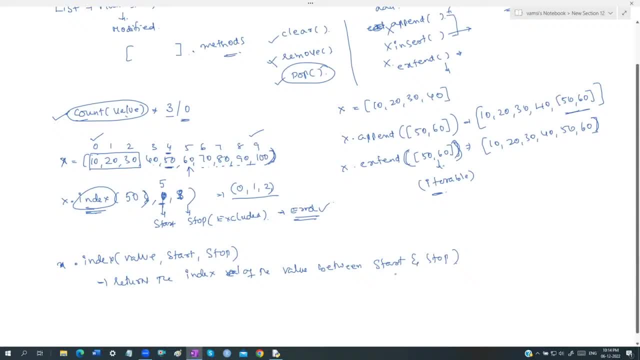 throughout the python. remember one thing, guys: wherever I am using start and stop, start is always, it is included, it is inclusive, and whereas the stop is going to be always, it is an exclusive. so whenever I said which is going to be 2 comma 8.. 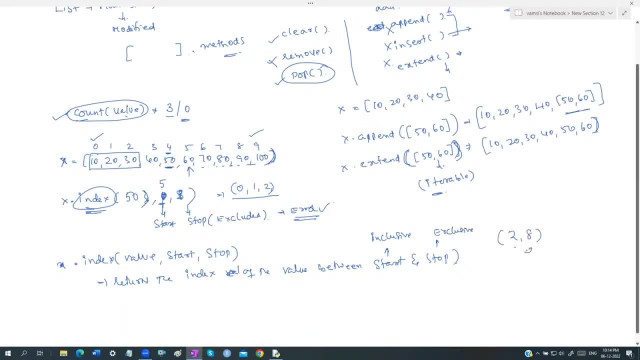 that is, start from 2 and stop before the 8. throughout the python. the concept is the same. it does not change us from one application to another application. throughout the python. it is going to remain the same, only guys. so given value: whatever the given value index is there. 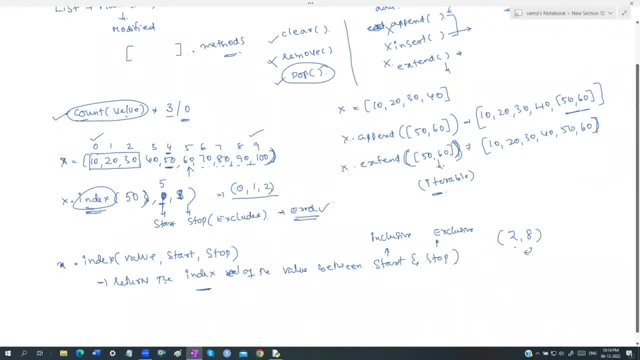 it will try to find out, but that to the first occurrence only guys. for example, same value is available for multiple times. it won't return the indexes of all the values. count is not like that. for example, count is there if the given value was not formed. it is going to return zero if the given 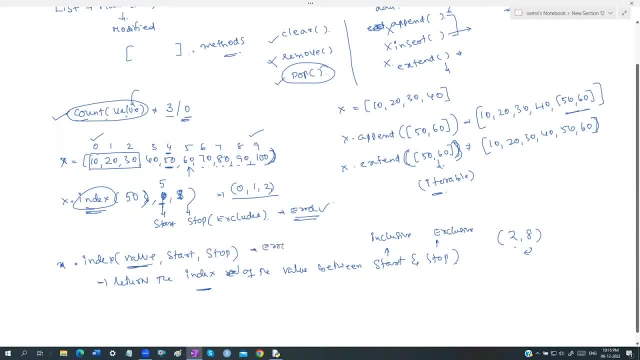 value was not found, it throws an error. actually, it throws an error, actually, guys. the value was not formed. i am going to raise us an error, actually, guys. okay, so this is going to be the next method. what i can talk about a little bit, a little bit complicated compared with the other. 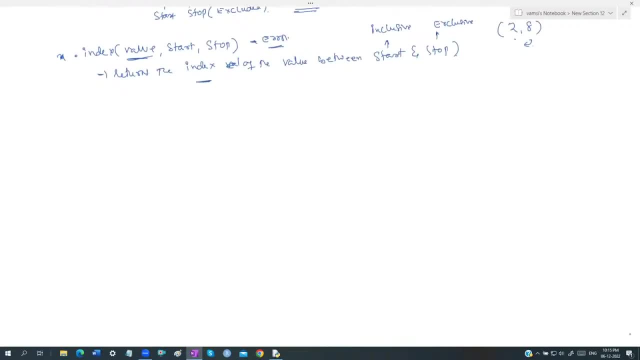 methods. actually, guys, now there are two methods are there which are going to be a very, very verse. simple methods actually. yes, one is going to be nothing but a method, what we are going to call it as an reverse. it's a very simple method, actually. guess, the name itself is saying that what is reverse will do all the elements in the inside. 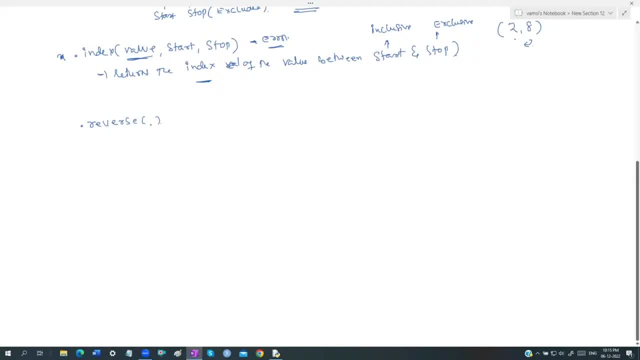 the list will be just simply reversed. actually, guess it will be very simply reversed. no, it's not sorting order. actually, guys, it's not any sorting order. left it ascending to descending or descending order, ascending order? it won't do it actually. yes, for example, i have a list, is there? 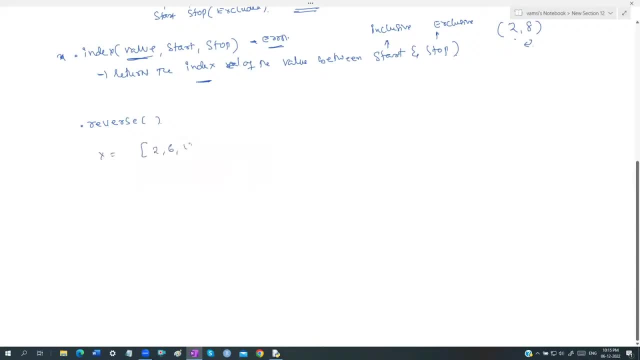 some x is having a list like something like 2, 6, 18, 24, for example, 12, okay, something like 6 and something like a 4. we have the elements, guys. now if i said what is going to be x dot reverse, simply if i said x dot reverse, you know, what it is going to do is actually guess. 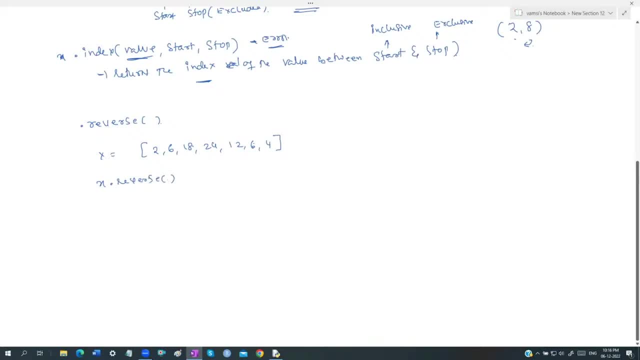 internally. it won't take any arguments, guys. no inputs, it will take it internally. all the data is going to be reversed. actually guess 4, 6, 12, 24, 18 and 6 and 2? actually, yes, you. but reverse also does not returns anything, guys. internally the elements will be sorted, so not. 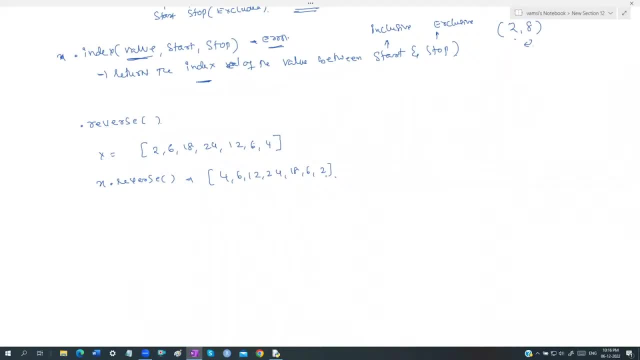 sorted, it will be reversed. but the outcome? if you want to see whether the elements are reversed or not, we have to print that particular value of x. reverse does not returns anything internally. it happens like this actually, guys, but if you want to see whether it is reversed or not, you have to. 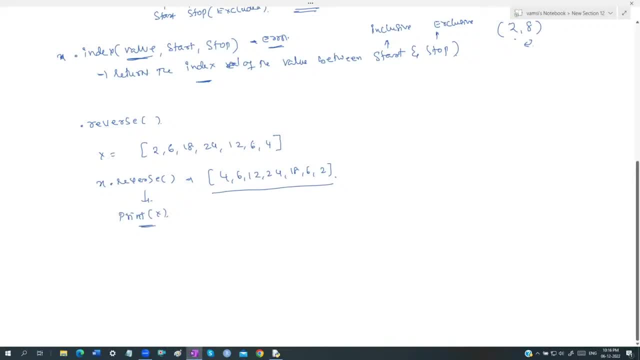 print the value of x. actually guess it's a little bit confusion to most of you guys. i'm saying that they don't return, they will return because they don't return, because they don't return, because they don't even have to do that, it is internally getting affected. actually, guys, it's internally. 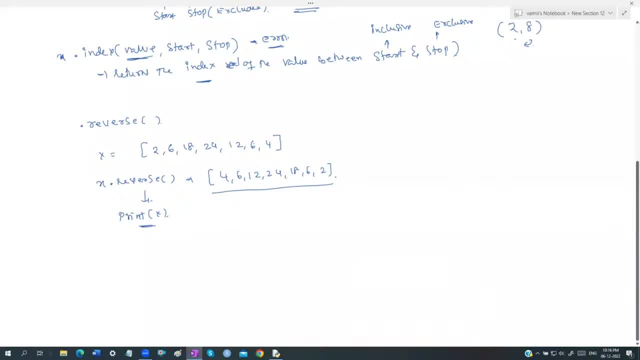 getting affected output. we don't see anything. that means when i write the x dot reverse, don't expect that directly. we'll get the output like this: guys, internally this happens. nothing output will come, whether it is really reversed or didn't reverse. nobody knows about that. if you want to see whether the reverse was done or not done, then we have to print the. 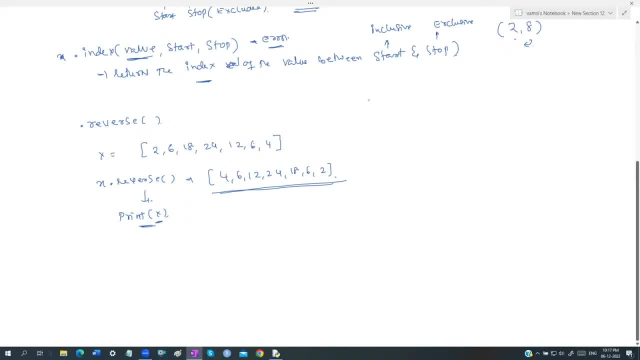 value of x. actually, guys, anyhow, the guys who has been already attended the previous classes. we already see about the slicing concept. actually, guys, sir, if i want to reverse these elements, i can do something like x of e to e to minus one. actually, guys, don't worry, guys who has been 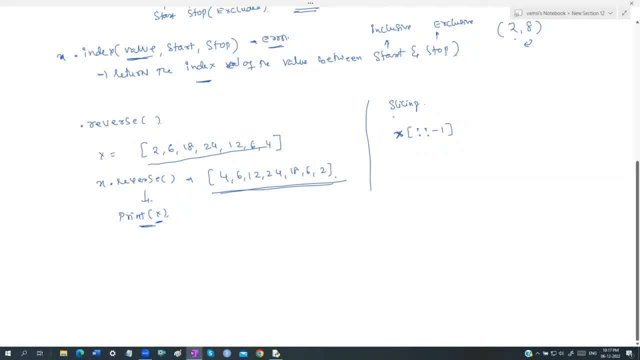 joined recently, so previous classes, we know that. so who has been joined earlier? you know what is the meaning of x of e to e to minus one. actually, guys, what is meaning of x of e to e to minus one? the elements it is going to read from the reverse order, by taking a step of: 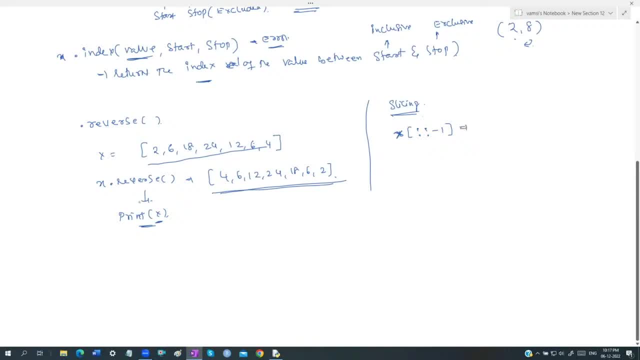 minus one. what is the difference between this one and this one is, guys, whenever i said x of e to e to minus one, the elements are going to be read in the reverse order and the output is going to be displayed on the screen. your output is going to be displayed on the screen, actually, guys. 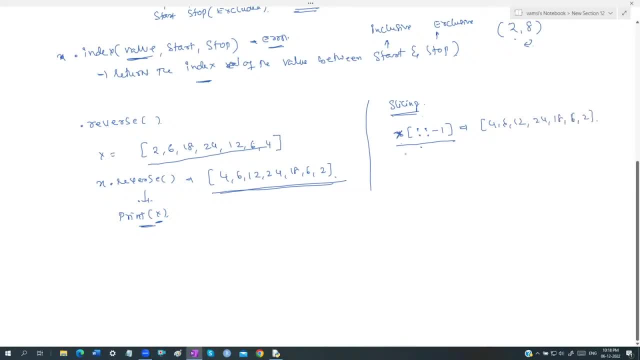 but your actual x is not getting affected. if i print the x value, it is, as usually: print this value, only guys, but not this value actually. so this is only. we are just reading the data in reverse order order, but your actual x is not getting affected. but x dot reverse is what it is doing, it is not. 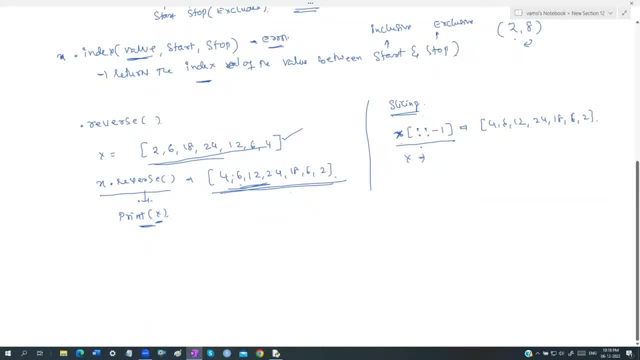 just only returning the output. it's not just only reversing the elements, guys. whatever the order, whatever the element that has been reversed, that will be again assigned back to the x. that means the effect is on the x variable, guys, but not just like a slicing concept. actually, slicing means 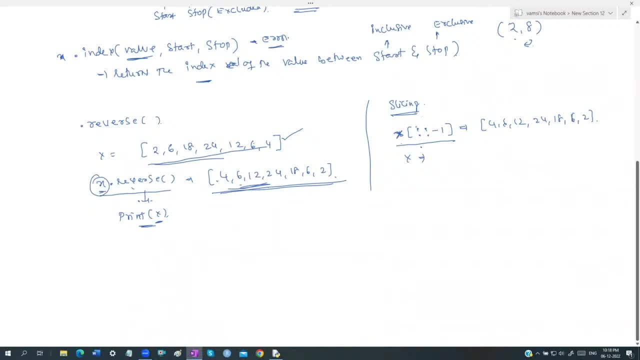 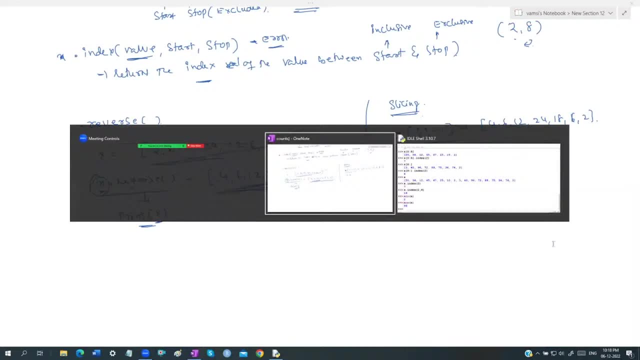 nothing, but it only just displays the output on the screen, but your actual array or the actual list is not going to be gets affected, actually, guys. okay, so just if you want to see the elements, i can just show you guys: x is equivalent to nothing but 4, 10, let us say 12, 8, for example. 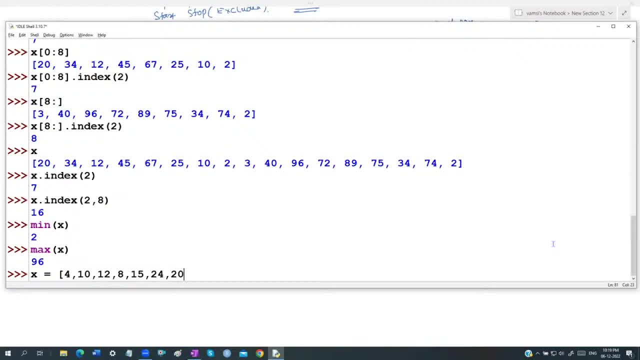 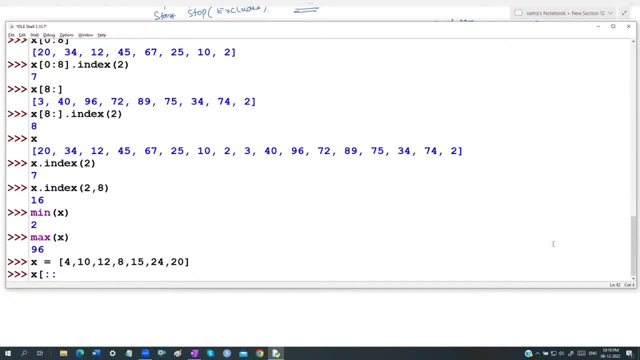 15 and some 24 and something like n 20. yes, just an example. not too many elements, guys. i can slice it like this: actually, guys, hope you remember this. what do you mean to say? x of is to is to minus 1 means just, it is going to read the elements in the reverse order. actually, guys, you can see. 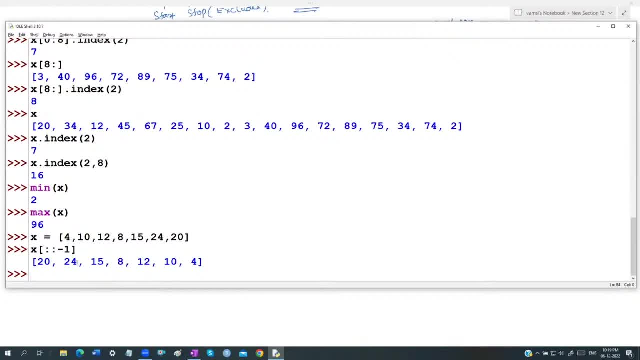 20, 24, 15, 8, 12, 4, 10 and it is going to be 4.. but what is this doing actually, guys? it is only reading the elements in the reverse order and it is displaying on the screen, but your actual x is not affected. your actual x will be as usually. 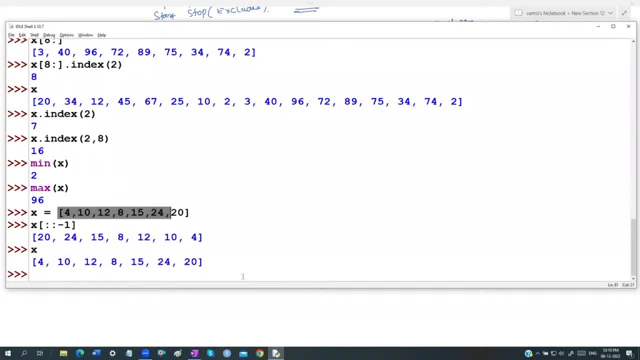 the same old elements, only guys. whatever i have given it has just reading the data in the reverse order, but your actual x is not getting affected. x will be remaining as same data, only guys. hope you understood the trick, actually, guys. okay, or in another way, if you want to explain this, i: 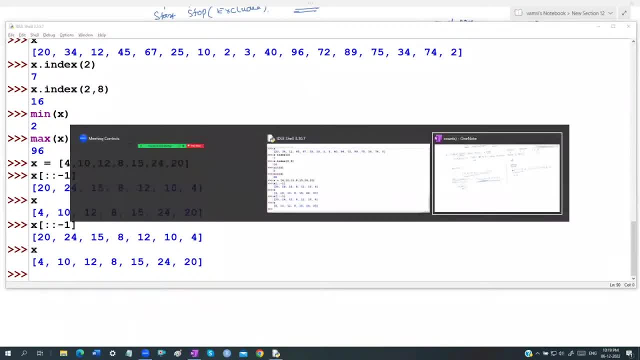 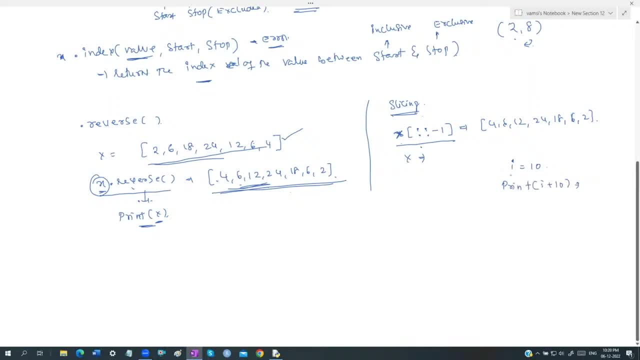 can explain in another way. actually, guys, in a programming language we have: i equals to 10.. when i said, print the value of i plus 10, you know what will be the result. actually, i guess i is 10, 10 plus 10 is going to be 20 only, but your actual i is not affected. guys, again, if you say print the 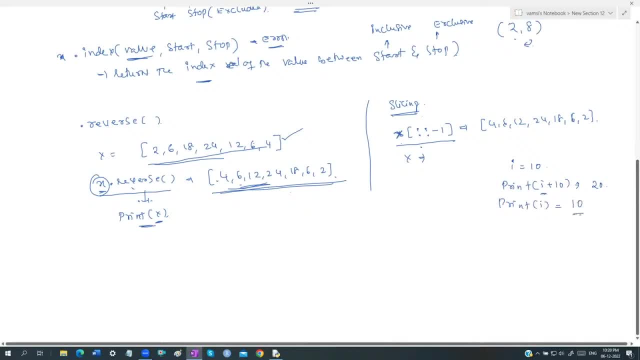 value of i. you know that it will be printing the result as 10 only, so this addition of 10 was done only for printing purpose. but your actual i was not affected actually. so i want to affect that particular i. i want to preserve that addition. then you know what you have to do, it actually. 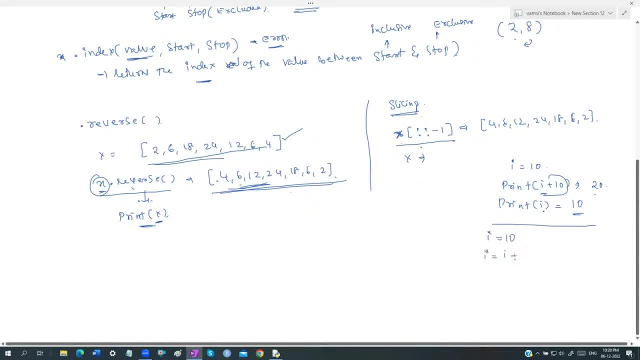 guys, i is equivalent to 10, you say i equals to i plus 10 and then print the value of i, then we know that the 20 will be printed actually. so the addition we are preserving back to the i actually guys. so this is nothing but just like. 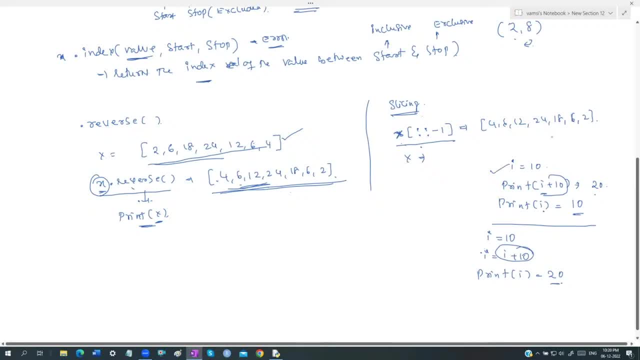 this concept only, guys, because we are just reading the elements in the reverse order and just displaying on the screen your actual x will not be affected. x, dot. reverse is nothing but what you are trying to do, guys. whatever the result we have got, you are again assigning this result back to. 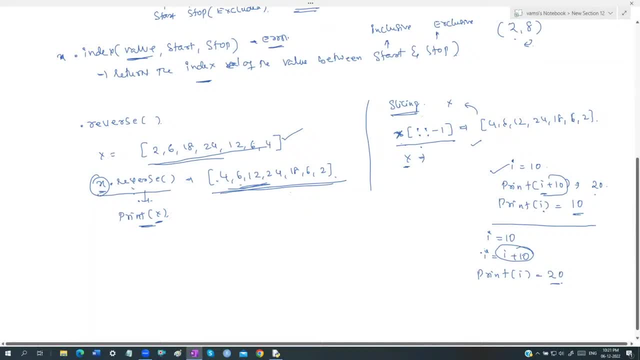 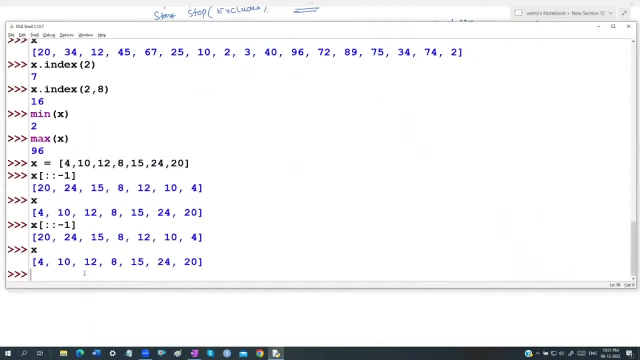 the x itself actually guys. so that is the meaning of this particular method called as the reverse. so once if you do the reverse, actually guys, it will be directly affected on the list. actually x dot, reverse. see the difference: actually guys x dot which is going to be reversed. it won't take any arguments. 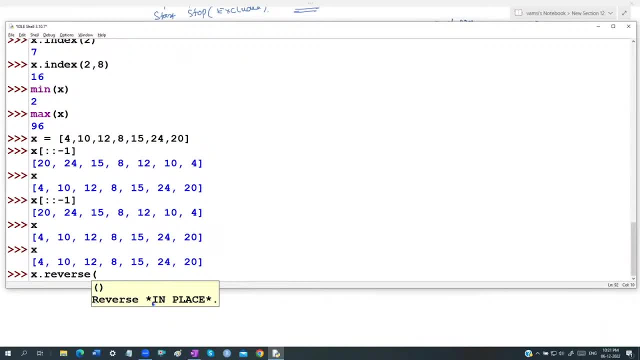 guys, and you can see very clearly: reverse in place what is meaning of. in place means in the place of the previous value of x. the new value will come. actually, guys, it will reverse the elements and that value will be replaced as the the previous value of the x in the place of the particular x. 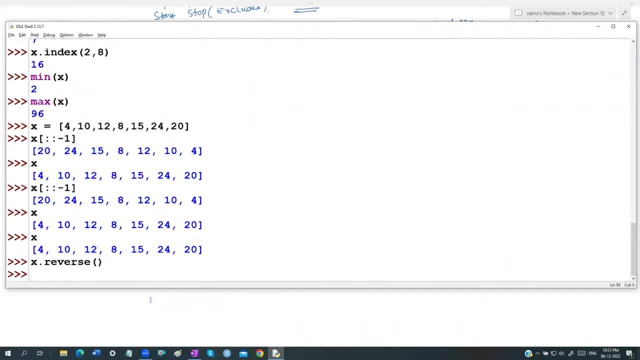 but outcome: we don't get it. any output, actually, guys. we don't get any output at all. no output will come, guys. clearly we can see there is nothing. output is coming, actually, guys. now, if you want to see whether really x is reversed or not, you can just write which is: 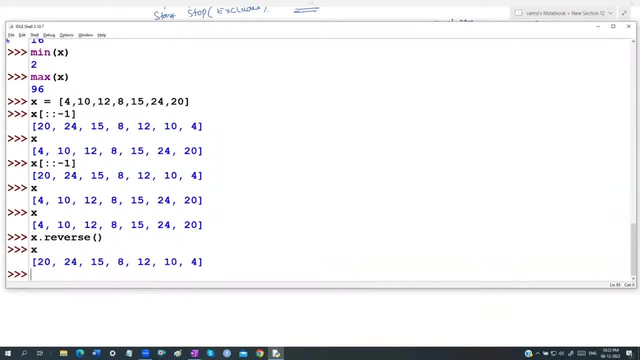 going to be x. actually, guys, can you see this? x has been completely modified, just the elements has been reversed. so slot of difference is there between x of is to is to minus one. it is going to be just reversing the elements and displaying on the screen, but your actual, the actual x is not. 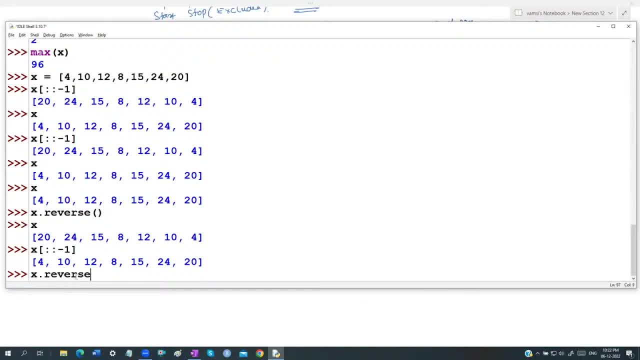 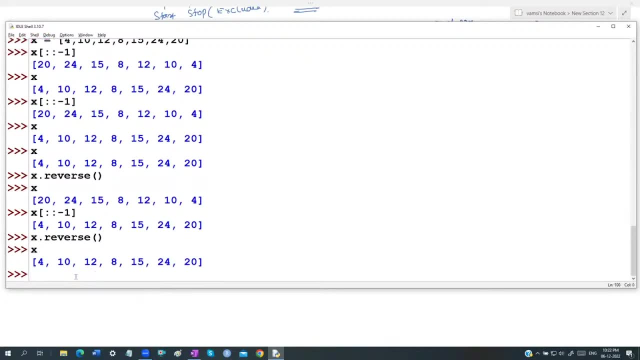 getting affected. but if i said something called as an x dot reverse, now you can see that the complete elements has been got reversed, actually, guys. so that is the difference between. slightly confusions will be there, guys. in the beginning there is a little bit confusion, but over the time period, 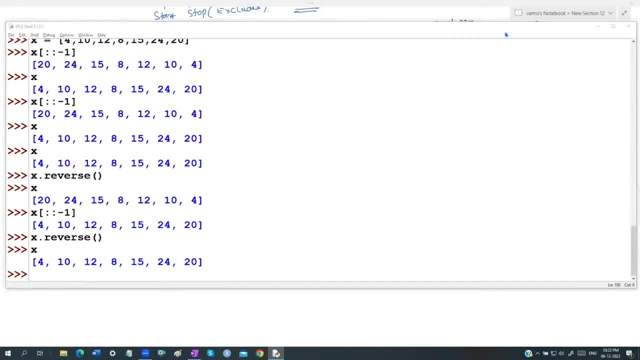 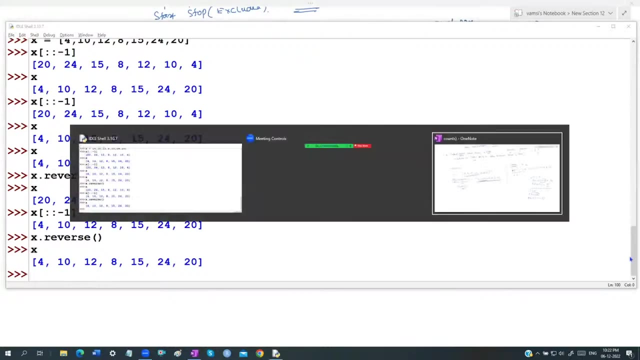 everything will be gets rectified. actually, guys, this is what we are going to call it as, yes, we can write it, but in python there is a small um, a small issue. is there actually? yes, um, it's a small issue actually, um, i think, roy, uh, hope you already discussed about that, like i think i, i remember. 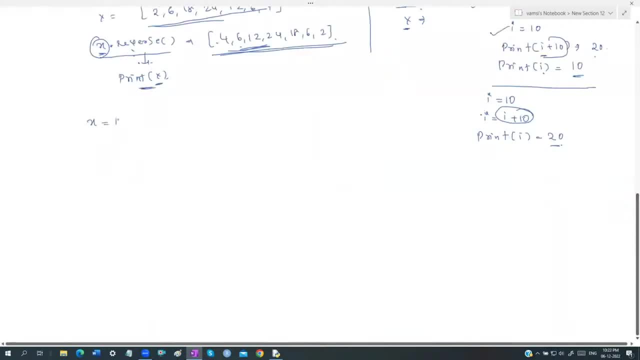 that you are joining from the uh beginning. you already joined in the earlier classes also. so x is equal n to 10.. so here you know that this x is called as an variable or an object. what do you call this x actually? will you call it as an object, or will you call it as an? 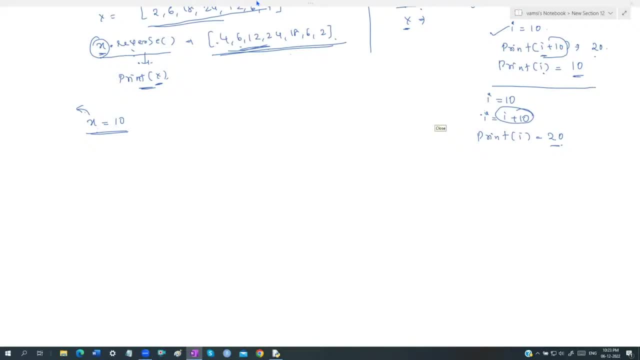 variable or an object? what do you call it as variable? no, in python, everything is going to be treated as an object only. okay, so what will happen here is: that is actually. i'm going a little bit out of the box, don't worry, because even if you don't, guys don't understand it also no worries. so, guys, what will happen here is in: 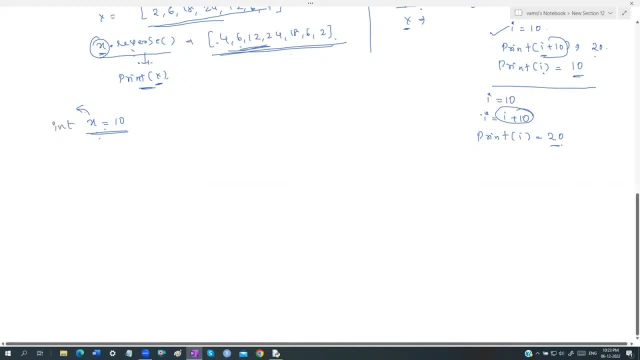 a normal programming language. when i said, like this, integer x equals to 10, you know what will happen. actually, guys, some memory will be allocated. the name of the variable is going to be x, the memory is going to be referenced by x, value will be 10.. tell me, guys, when you say x equals to 10, 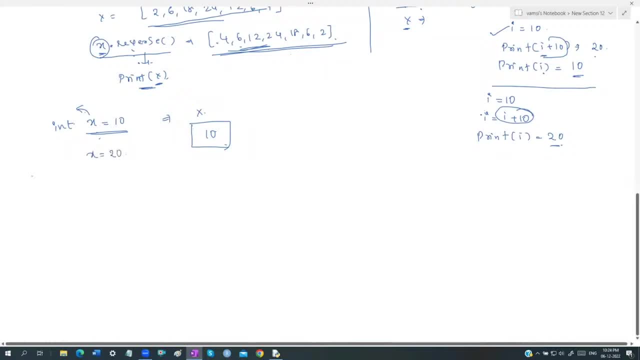 what will happen? can you tell me, guys? will it remove the existing x and creates a new x, or only the value will be changes generally in a normal programming language, as a normal programming language, anyone, guys? if i said x equals to 20, what is going to happen now? 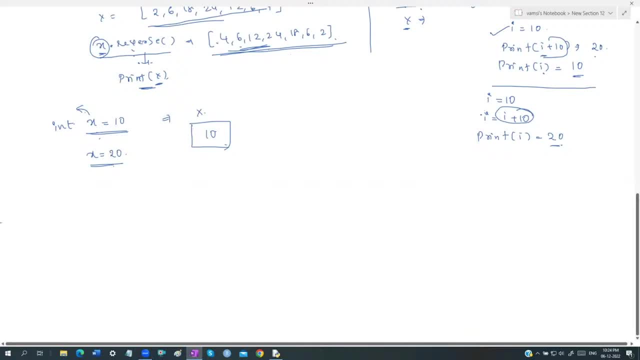 will it create a new variable or only the value will be changes, only the value will be changing. only value will be the old object it's. it will be there. only that means we know that the declaration is done only for one time, so memory allocation is done only. 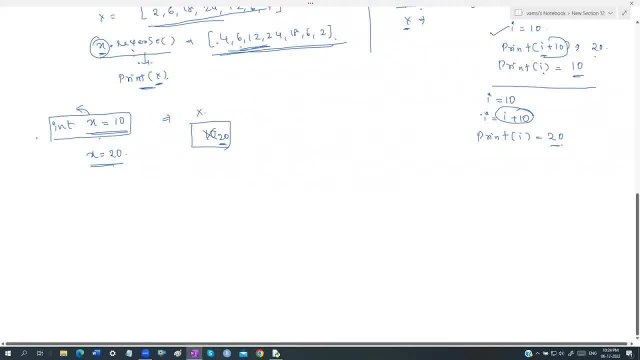 for one time only. your existing x will not be removed. your existing x will be there as it is. only the value will be changes to 20.. but coming to the python, x is equivalent to 10. here x is an object, actually guys. x is an object, actually guys. so it is going to be referencing to some memory which 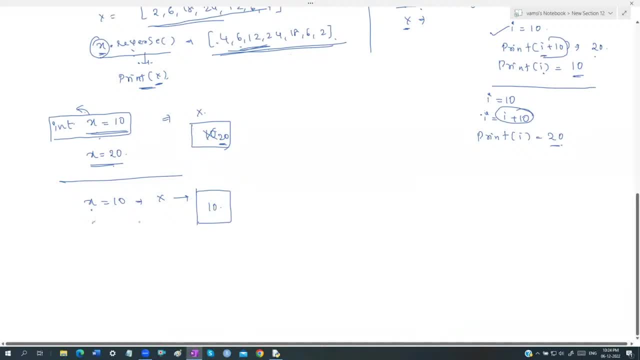 is containing 10.. when i said, x is equivalent to 20 in an object oriented programming. what it will do, guys? it will destroy this one and again creates a new one. actually, what the point, guys? just i'm telling about an idea, just for an idea purpose. i'm telling about that so, as you are asking that, 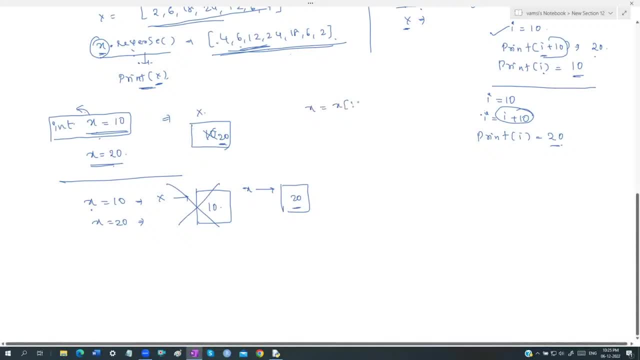 when i said x is equivalent to. why don't you write like this: actually x is x is 2 is 2 minus 1.. absolutely, we can write it, actually, guys, but what is happening here is it is going to create, a new object is getting created, so python is having one, one of the main issue, actually. if 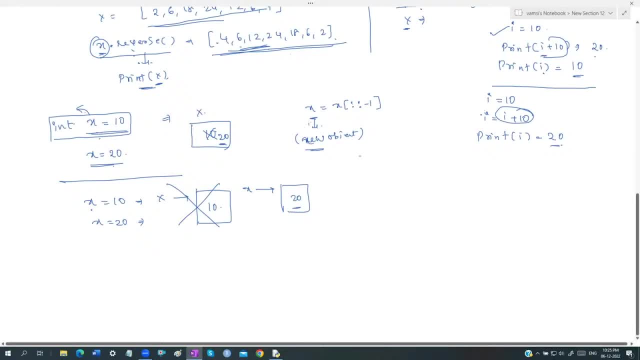 you try to assign like that, it is going to create a new object, even in python. actually, guys, if i said x equals to 10, x equals to 20, both are two different objects- actually this will be destroyed and new object will come. actually you may get a dot. so how can it? how can you say that actually? 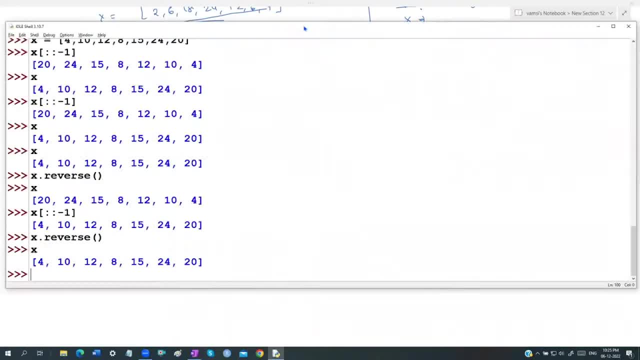 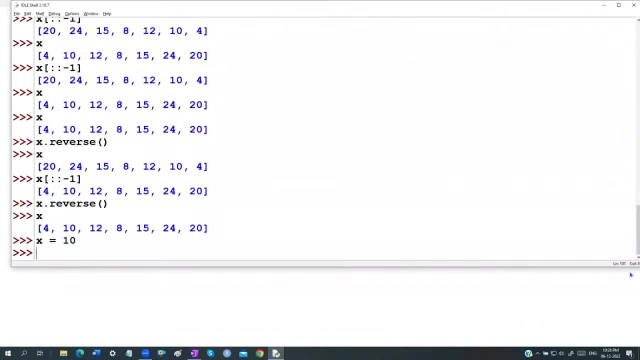 how can you say that? don't worry, i'll actually. i'll discuss this. actually, we have this discussion in our class. for the timing, i'm just telling you guys, x equals to 10.. every object will have an id. guess, every object will be having one id when every object you create in 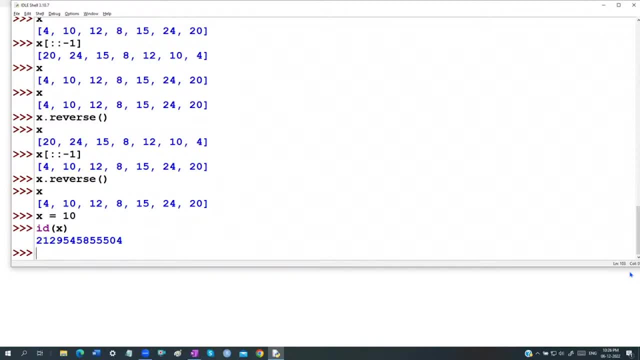 python, one id will be given. actually, guys, can you see? this id of x is going to be ending with double five, zero four. now i said x is equivalent to 20. guys now see what is going to happen. is actually id of x is going to be. this is going to be the id actually. so what has been happened, guys? 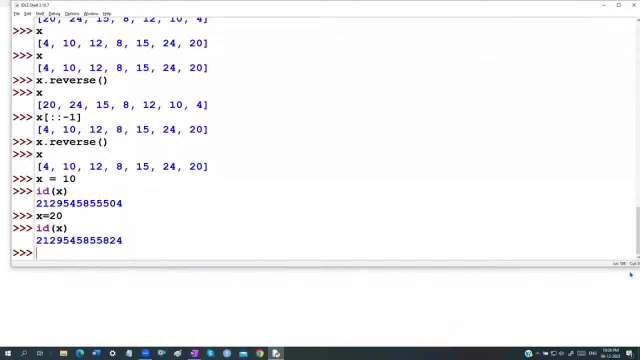 it is completely. the object was destroyed and new object has been got created. guys, you can delete the object. guys, i can delete the object. there is an option to delete an object. actually, guys, same technique. i'll show you guys. x is equivalent to, i said 10, 20, 30, 40, for example. 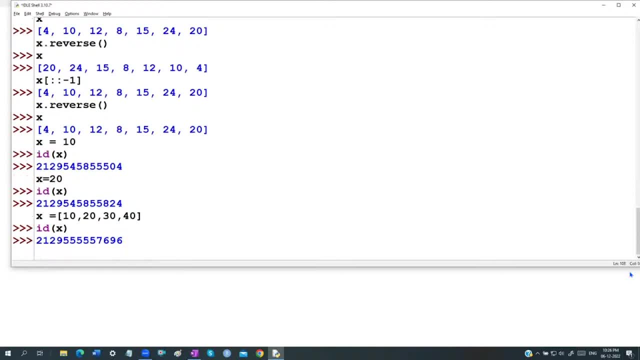 now, as you are saying that, okay, i'll say id of x. now i said x is equivalent to x of e is 2 is 2 minus 1.. no doubt elements are reversed, but the main problem here is internally. your object is changed internally. your complete object was changed, actually, guys, earlier. the object is ending with 7. 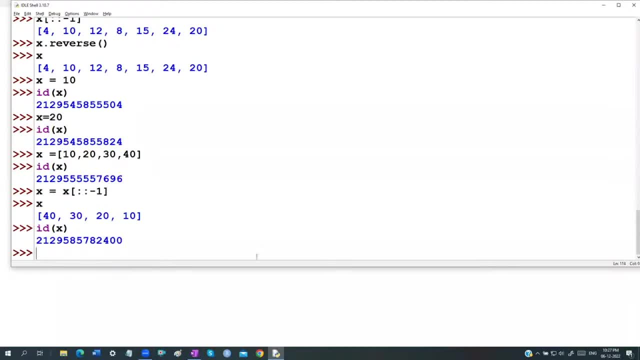 now the object is going to be ending with 2, 4, double zero. but if i said x, dot reverse, actually guys, what will happen internally here is object won't change us guys, the internally the elements will change essentially. now see, the x elements are reversed. id of x is going to be, remains the 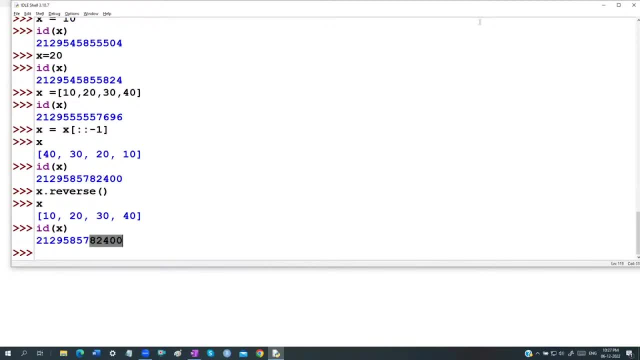 same object as it is. it is going to be reference, don't worry, guys, hope you. you got an idea about that, like why i am not assigning to a particular variable. got it right. so why i'm not assigning the object like this? because internally the python is having some 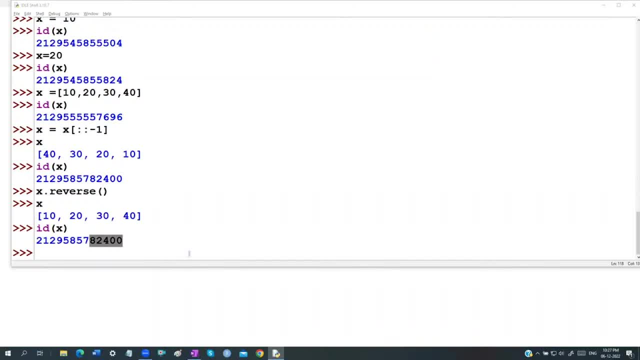 memory problem actually. so it will create that object, destroy some object and again creating a new object. it will take more load. why should i take that load actually? that's why we better to use the reverse method throughout the python. that the same technique. i'll use it actually. yes. 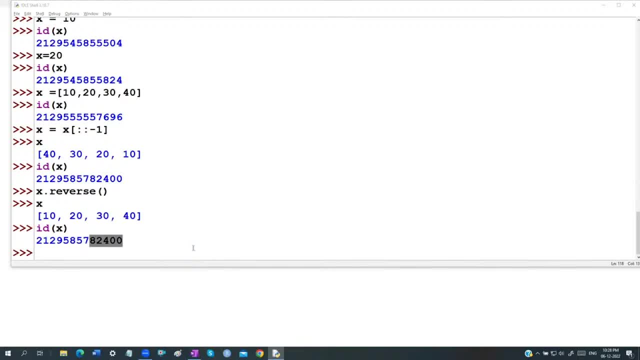 same techniques i'll use if you ask a, any man. if you ask for any changes, i'll make the changes, but i don't preserve by assigning back to the variable. we'll be having some technique. i use it, a word, no guess in place. this word will be very. 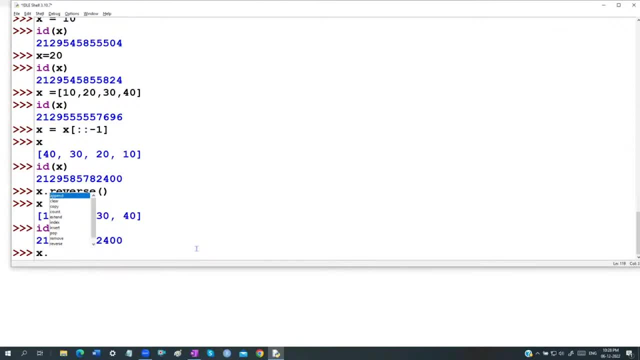 very frequently used in python. actually, guys, sorry x dot. when i'm using reverse, you can see one term called as an in place. is there this in place technique we are going to use very, very frequently in the python? actually, what is this option of in place will do? is actually guys, whatever the 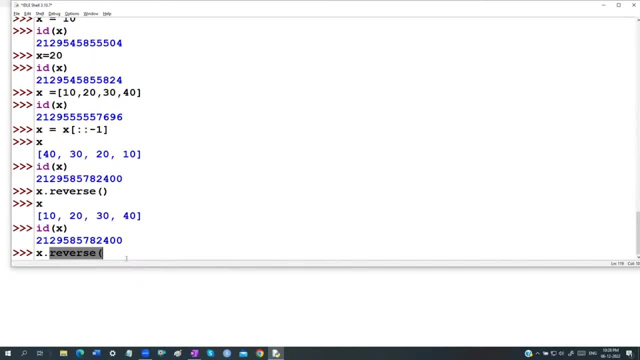 option you have been asked for, or whatever the manipulation we have been asked for, that will be reflected and that will be affected on your actual object. it won't create any new object. the internally the elements are going to be gets reversed. actually, guys, that is what the reverse will do. actually, guys, it's not any sorted order actually. 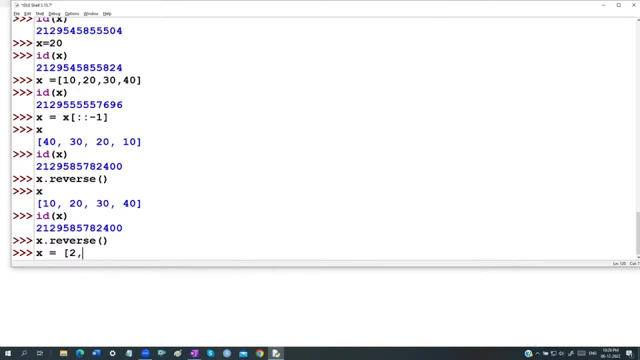 because the data was already in ascending order. so what we can find here is it is going to be something like: it looks like ascending and descending order. it is going to be looks like: actually yes, but whenever the data is in a random order, you can see that it is going to be just a reverse. actually yes, internally. the elements are sorry internally. 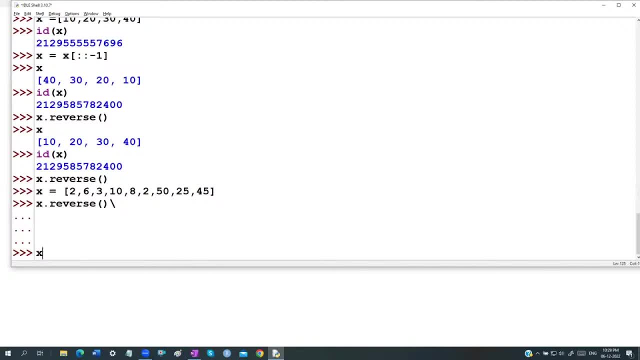 the elements are going to be gets reversed actually. yes, internally the elements are going to be gets reverse. you can see 45, 25, 50, 20, 8, 10, 3, 6, 2, but i want to put it in a sorting order actually. 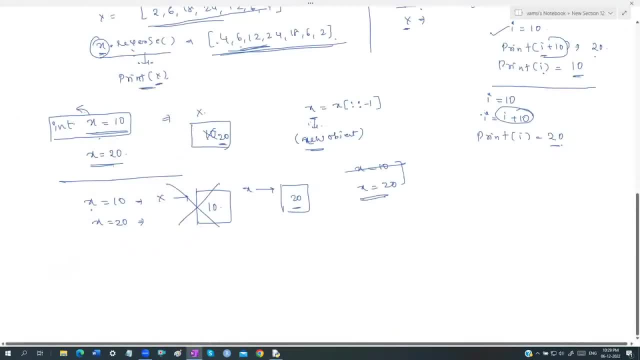 so what we have to do so reverse is only just reversing the elements. it is not returning any output, guys. it won't return any output back to you same as it is. we are having a method called ascent shot method. is there actually, guys, i covered all the methods. actually, guys, all the. 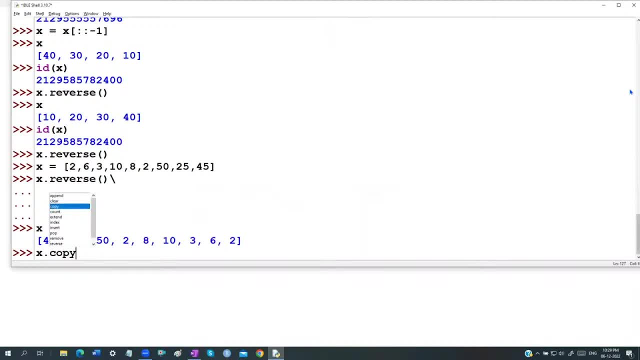 methods have been covered, except copy. you can see it actually as copy also. i can explain you, but you can't understand now itself: append, clear, count, extend, index, insert, pop, remove, reverse. and the last one is going to be sort. actually guys, sort is going to take one simple option, actually guys. 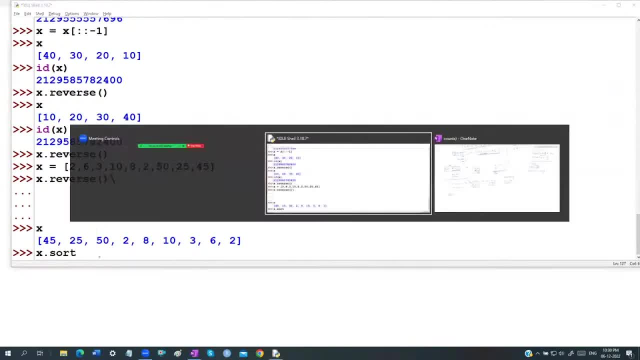 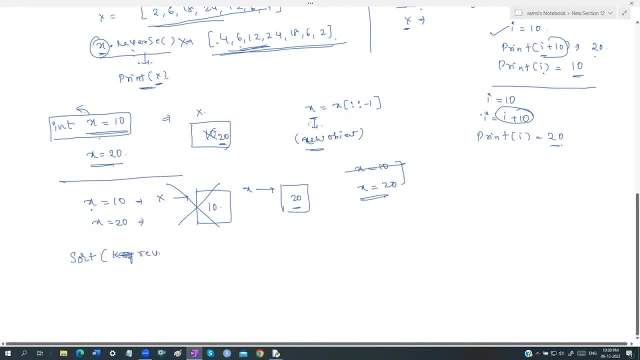 sorting. you know this, actually sorting also is going to be in place, only, just, it is going to take some order. actually, guys, which is going to be nothing, but simply i'm using a parameter called as reverse is equal to which is going to be true or a false. you know what is meaning of true and 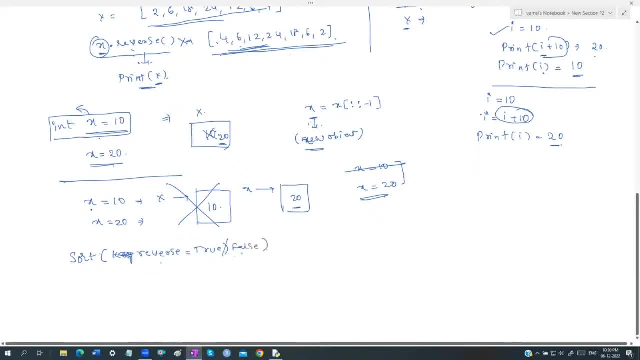 what is meaning of false? actually, guys, reverse is false, means it is in descending order. reverse is equal to true, means it is an ascending order. actually, guys, sorry, sorry, reverse is equals to true. sorry, guys, reverse is equal to true, meaning that it is a descending order. reverse is equivalent. 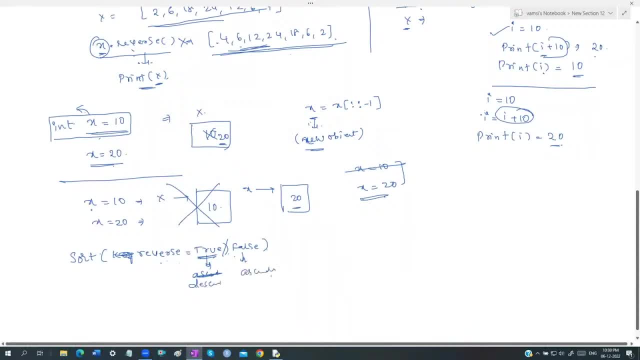 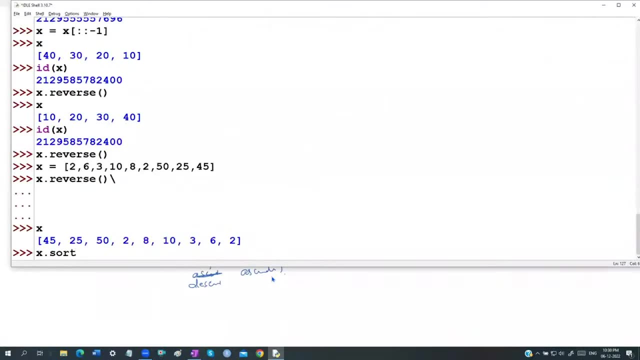 to false, meaning that it is an ascending order. actually, guys, just one parameter. it will take it reverse equals to true, reverse equals to false. so we have a parameter. actually, guys, i can say reverse equals to. i said false. actually, guys, very clearly sort the list in ascending order. 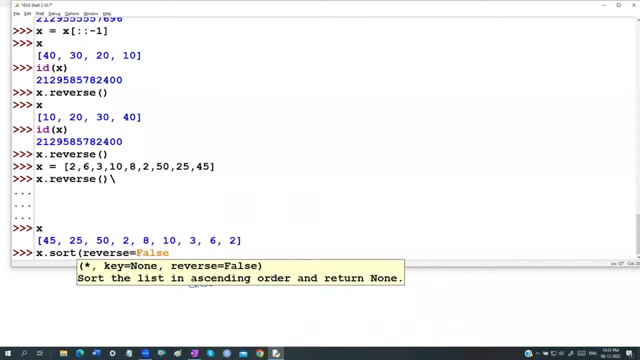 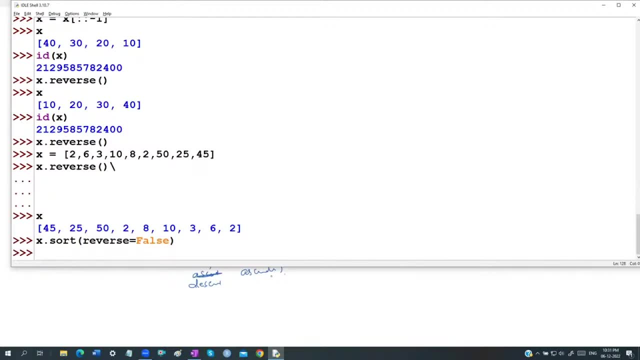 and again return. so i said: reverse equals to false. actually, guys, same procedure. it won't return anything, guys. it won't return anything output. don't think that, sir, i didn't get any output in the sorted order. sir, i didn't get an output. you don't get an output, guys, but your internal elements. 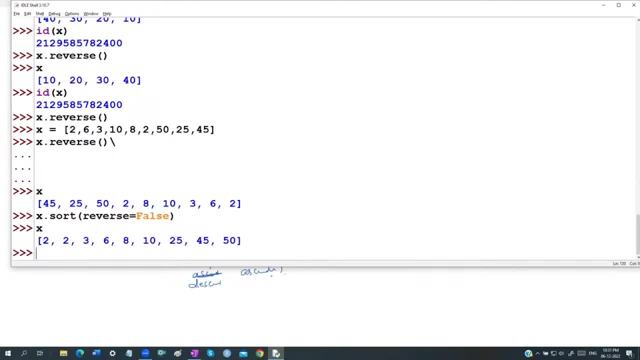 are going to be sorted order. you can see the difference: 2, 2, 3, 6, 8, 10, 25, 45, 50. so that is an ideas about this particular sorting order. actually, guys. so once again i'm doing this is going to be sorted order. so i say x, dot, sort, i want to do it in. i want to sort them in the descending. 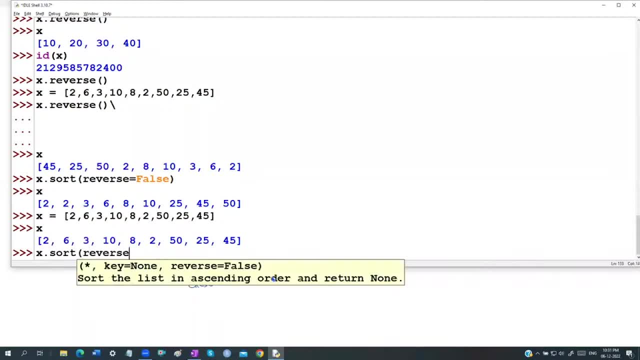 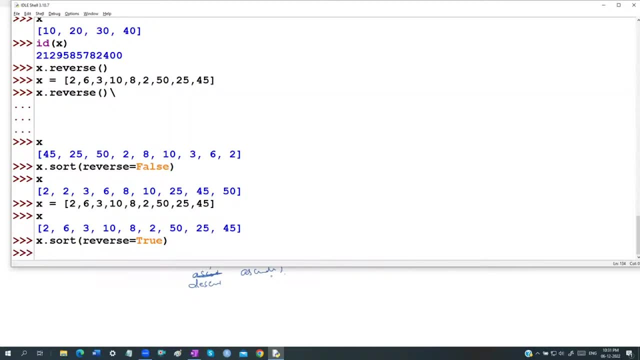 order. so i say x, dot, sort. simply, you say reverse is equivalent to nothing. but you say: which is going to be true? actually, guys, what is meaning of reverse equals to true, the, internally, the elements are going to be sorted in the reverse order. but, sir, i didn't get any output. you don't get any output. 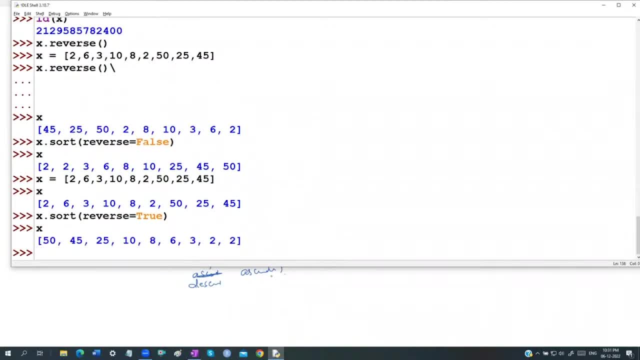 guys, internally, the elements are going to be sorted in the ascending order- sorry, descending order- and they will be again assigned back to the that particular object itself, actually. so these are going to be the techniques. what we are going to be gets calling it as guys, so reverse. 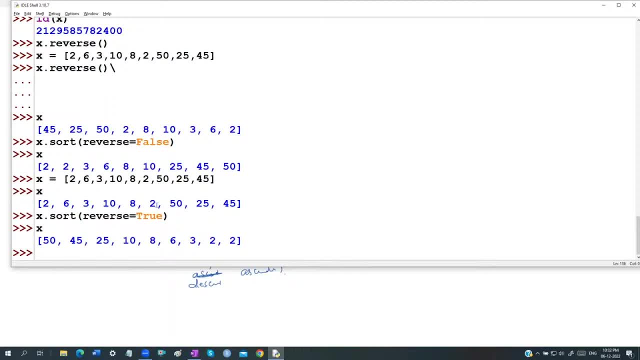 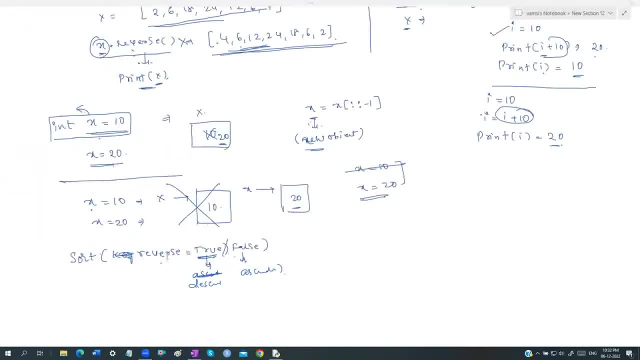 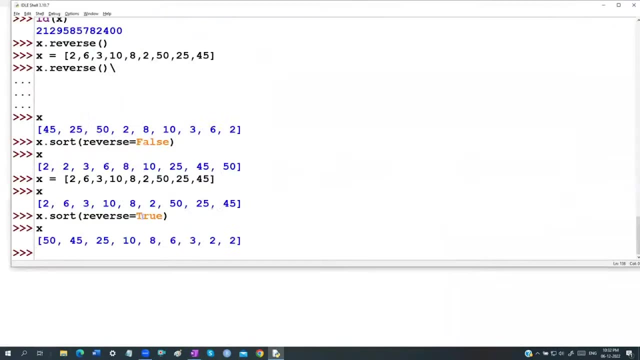 and sort. both won't return any output internally. the reversing will be done internally, the sorting will be done actually, guys. so let me conclude the concepts totally. guys, why we are using the reverse word within that parenthesis? it's an argument. it's an argument actually, actually. can we just use like true or false? you can use it, but as of now, the c is basically what. 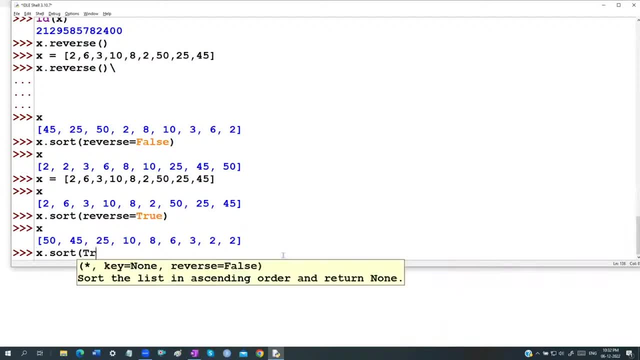 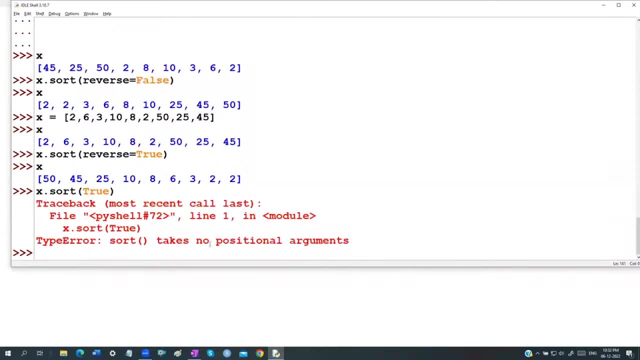 we will do here is: even i can use that. that is not. that is not going to be a problem actually, but what is going to be happening here is: can you see one? some kind of an error is coming actually takes no positional arguments. that means, as i told, you know, so we have a functions. 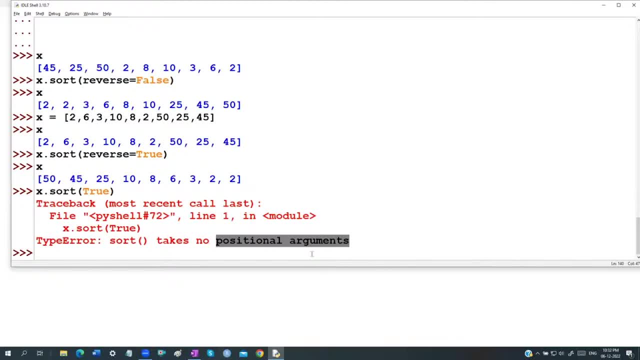 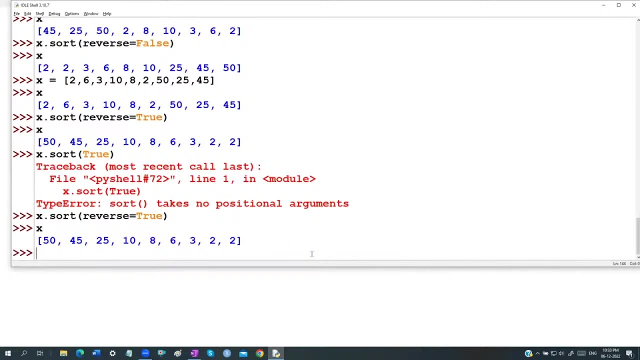 concept. is there actually? so position arguments and keyword arguments, okay, okay. for example, see, when i said x naught sort of, i said something called as an reverse is equivalent to true. it has been got worked successfully without having any problem. let us do the same thing. x dot count of. can you see a parameter called as value? is there? can you see the value parameter? 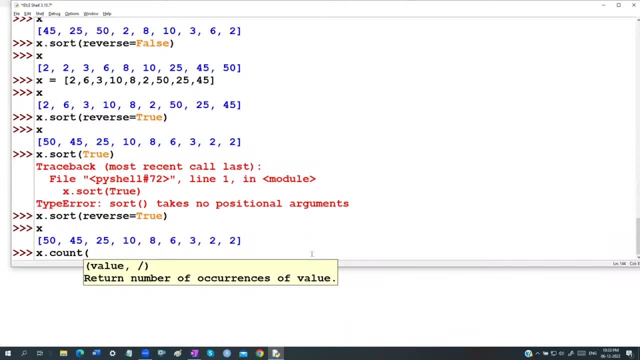 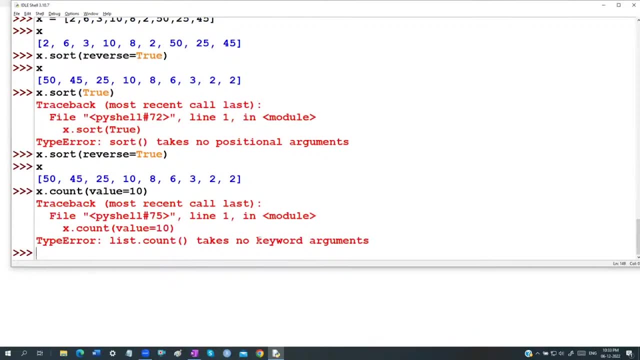 is there? no, there is an argument called as a value, right? yes, isn't it? if i write value is equivalent to, for example, 10, i'll get an error actually. so it is going to be a positional arguments and a keyword arguments concept is there in python. 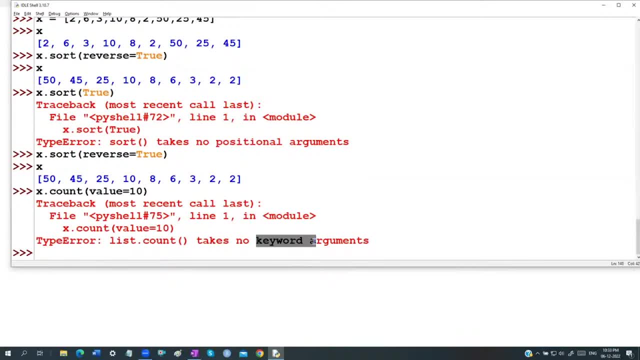 that is going to be, that. the whatever they defined is going to be like that. you have to define that. that's a syntax. that is a syntax, what we have to do. but anyhow, keyword argument, position arguments: we'll discuss it. actually, as i told you know, we have a complete discussion. 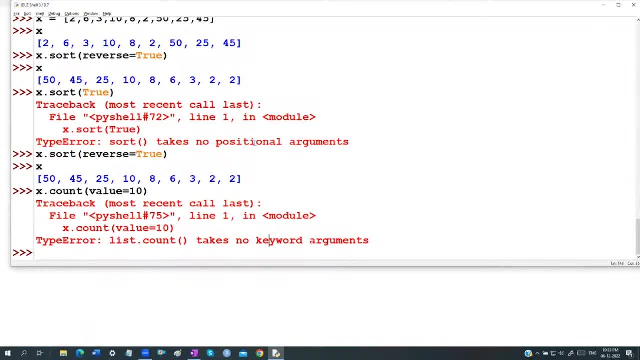 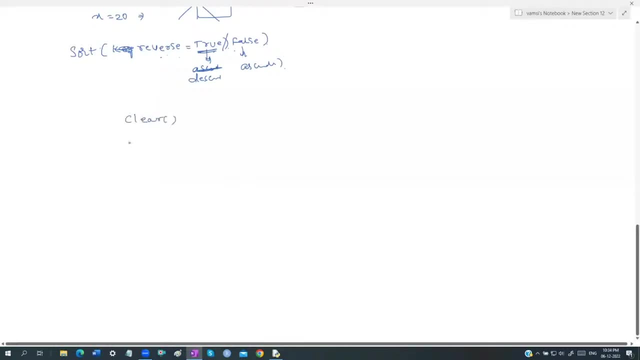 of functions concept. on that day we'll discuss about all these things actually, right, fine, okay, coming to the discussion, guys. finally, let us conclude the concept, guys, like the functions or the methods, what we have been got discussed, so all the methods. once again, i'll just rewrite it on clear which is going to be pop and which is going to be remove. 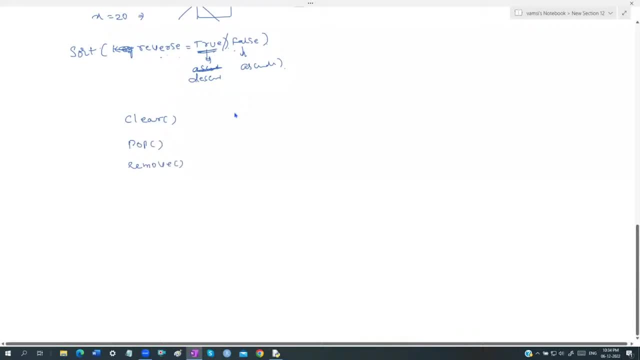 this, basically three, belongs to one category, like which is going to be a pen and which is going to be something like an extend and which is going to be insert. extend and which is going to be insert is going to be basically used for one type of category: uh, count and 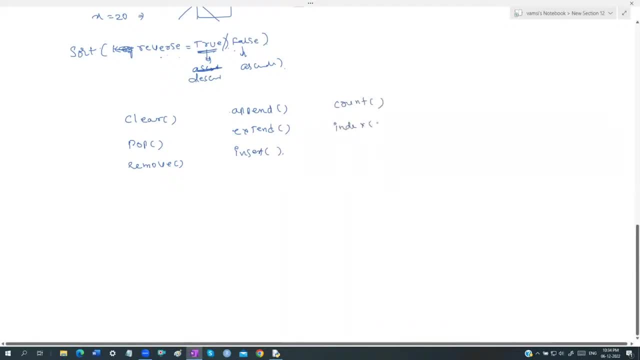 index is going to be one kind of a category actually, guys, because both are not the same, but counting is going to be counting number of times deducted. index is going to tell you about where is the given value is there, and sort and reverse is going to be one method actually. yes, both, almost all same. 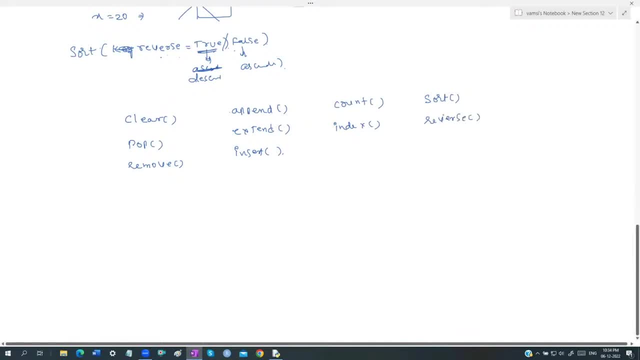 only. but sorting is ascending, descending order, reverse is only just reverse, the elements only, independent of ascending descending order. i didn't discuss about a copy method. actually, guys leave this copy method. so finally, if i conclude the concept: guys, which methods returns, which method does not returns? pop is going to return the value guys count is. 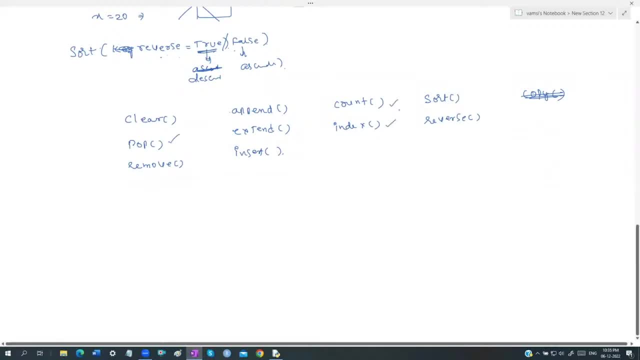 going to return. extend will returns remaining no elements, no methods will return any output. guys, clear won't return anything and remove won't return anything. append, extend, insert, obviously even sort and reverse. also, we have been seen nothing is going to be retained. but if you want to see whether there are cleared or not, whether they are appended or not, whether 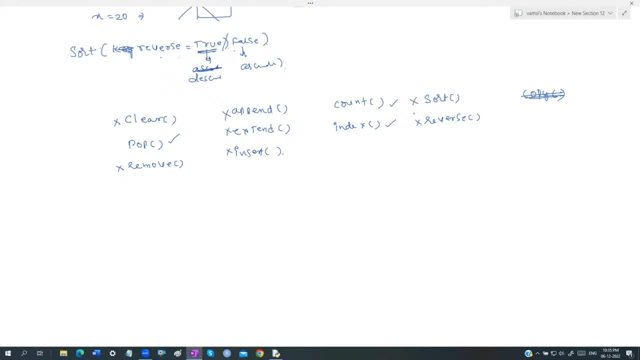 they have been reversed or not. we have to see the object and we have to conclude that, yes, it is reversed, it is sorted, it is appended, it is extended. it is extended, it is now controlled, it is fixed, as we have done. so it is going to be a part of the concept, which is why i 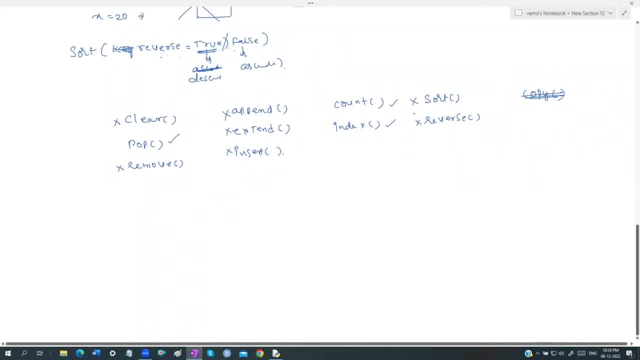 is inserted, it is cleared and it is going to be removed. but pop is going to tell you what value i have been removed. count is going to tell you what is account. index is going to tell you the index action: yes, okay, so that is going to be the one, what we can observe carefully, guys. so this is. 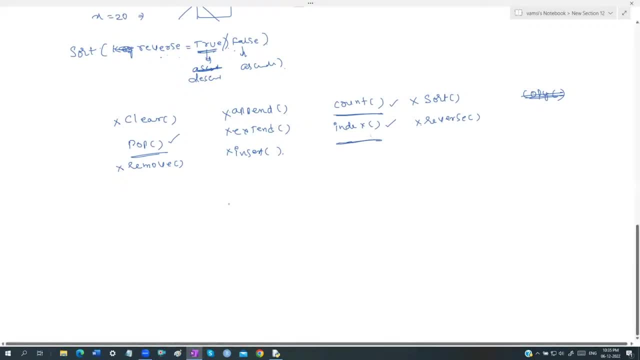 going to be about the list methods, guys. two minutes, guys. i'll just finish off it. the next object which we are going to discuss is an another object called as an tuple x tuple list, and tuple tuple is going to be a very, quite similar to which is going to be least guess, very 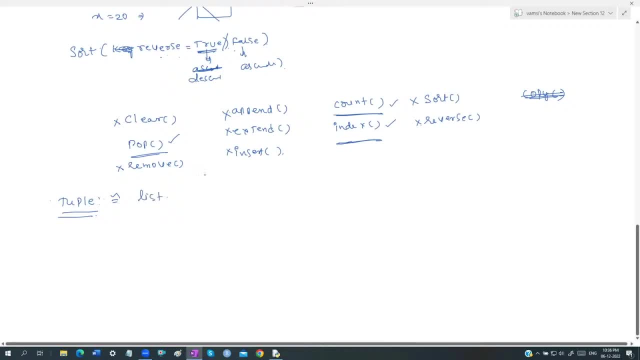 quite similar to list. then what is the difference? actually, guys? i told you the definition of a list. what is the definition of a list? i told you guys, first, initially, it's a mutable which we can modify. what is tuple actually, guys? tuple is going to be similar to the list. 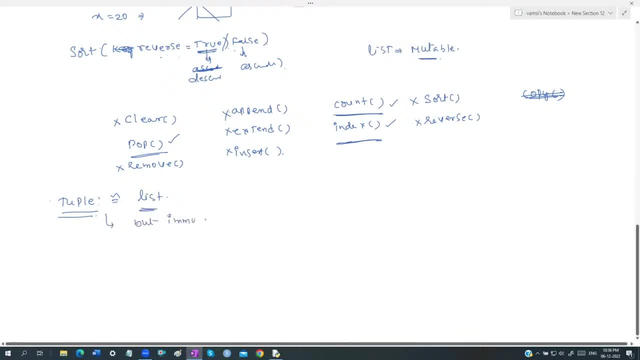 but but which is going to be what we are going to call it as an immutable object, guys. what do you mean to say immutable guys? immutable means which we cannot modify, which we cannot modify guys. that means once, if you create a list, we cannot modify further. it's like a constant value, guys. 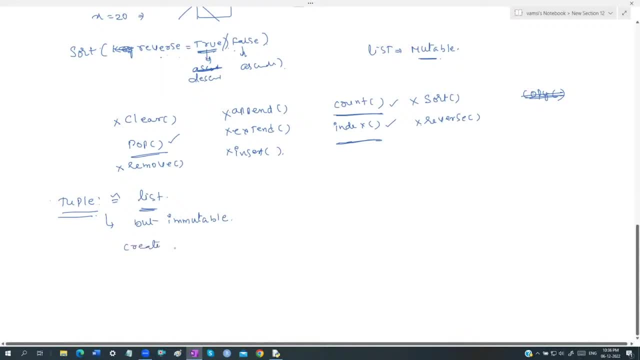 how do you create a list which is going to be? create a list, sorry, create a tuple. how do you create a list enclosing in square brackets? guys, how do you create a tuple? create a tuple by enclosing in- no need to use any keyword like tuple or etc. guys, by enclosing in which is going to be. 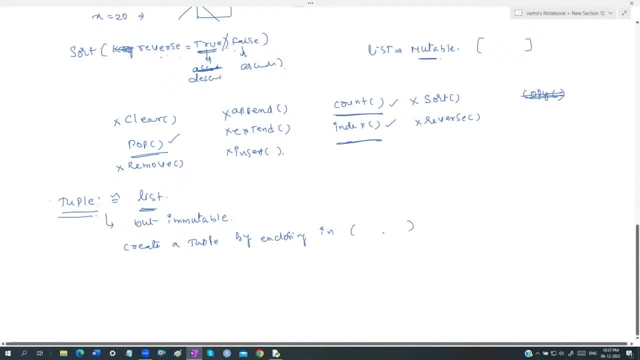 parenthesis, guys. simple guys. if i put the values in a square brackets, it becomes a list. if i put the elements within a parenthesis, it is going to nothing, but it becomes a tuple. actually, guys, now i can just conclude the concept. guys like what methods we can use, what? 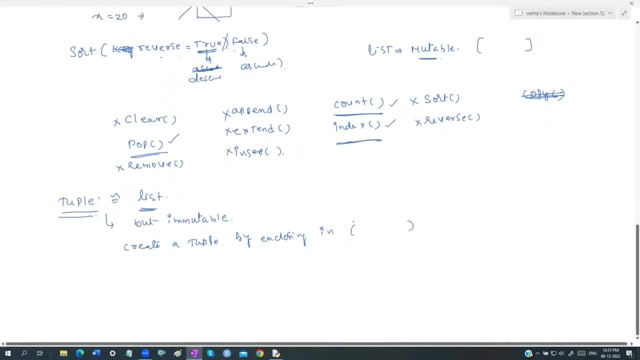 methods. we cannot use it. actually, guys. just let me conclude the concept. guys, same methods, no difference in the methods. actually, guys. but which methods will work on the tuples? which method does not works on the tuples? remember only one simple point, guys: tuple is not going to be gets editable. 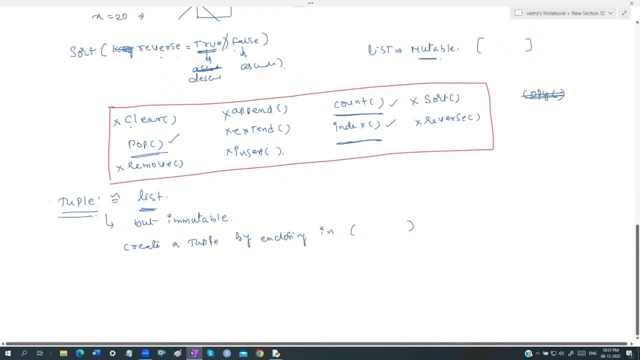 you can't edit it. so first of all clear. come to the clear. actually, guys, can anyone guess? can you tell me, will the clear will work on the tuple guys? no, no, why? because clear will try to remove the element from the tuple, which is not possible. next, what about pop? 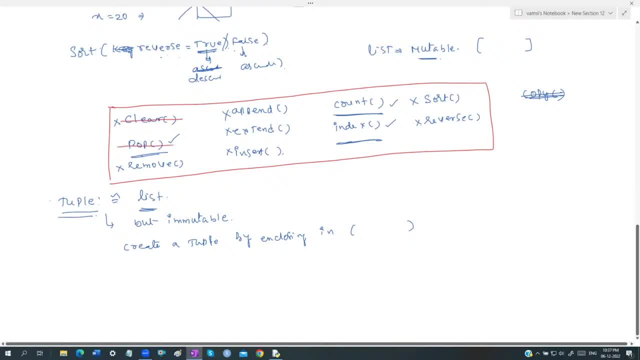 yeah, no, because pop is trying to remove the element. no, okay, so clear: won't work, pop won't work. remove those networks. what about extend, append and insert? no, no, because we are trying to add some elements, guys. what about sort and reverse? can it be done? cannot be done. 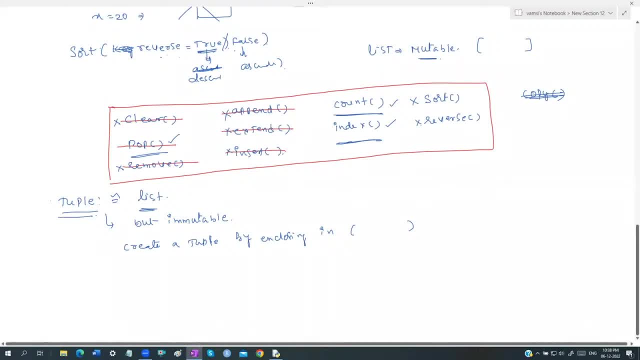 no, i think no, no, no, because that's actually one of the steps to be taken, guys. so sort is not only just sorting the data and giving you guys, internally, the elements are getting modified. actually, so sort one works and reverse won't work, guys. then only two methods will work, guys. what other two methods will work is? 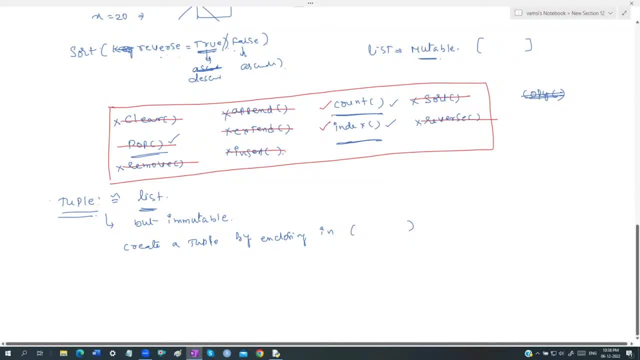 count and the index. only those are the two methods. it will work. that's it, guys. only minutes, only reading, only reading, just counting how many elements are there and to find out that particular index is there. so just two minutes, guys. i'll just finish off it so you can say which is going to be. 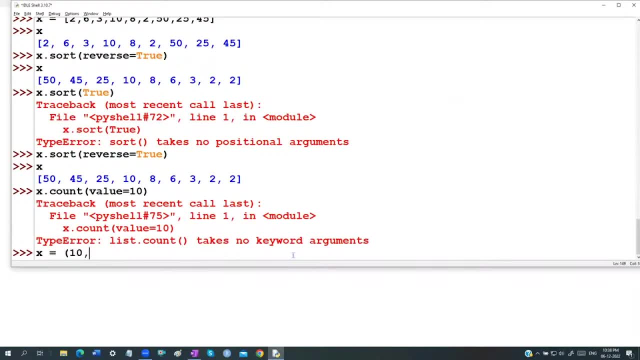 into just some elements: same element, similarly different. whatever you want, we can. what. whatever you want, you can give it. i told you know, guys, it can be heterogeneous or homogeneous, does not matter. very simple, guys. i enclose it within parentheses. guys, print the value of x very. 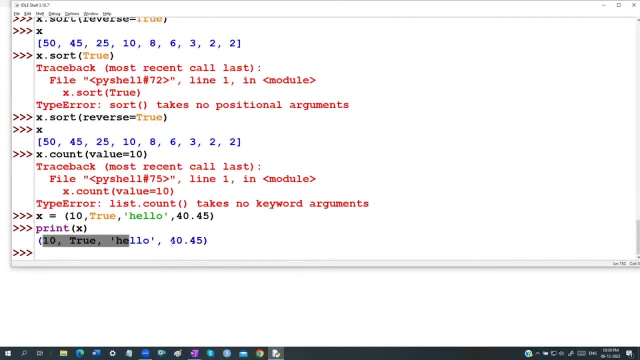 clearly we can see the elements has been got enclosed within parentheses. if you want to find out, you can just find the type of the x. previously when i said type the x, it has been given that it is going to be a list, but now we are going to be getting like a triple. actually. guys now say x dot. 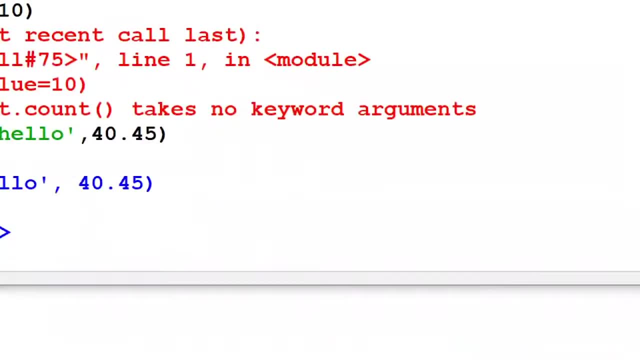 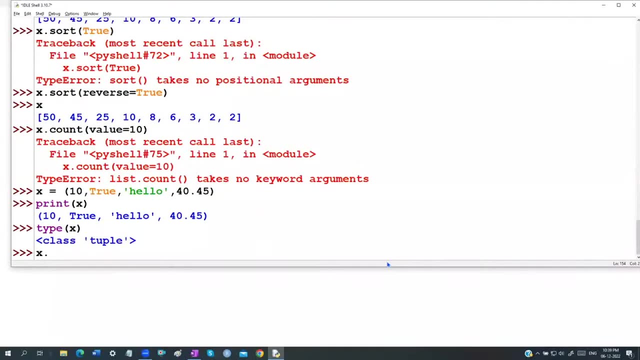 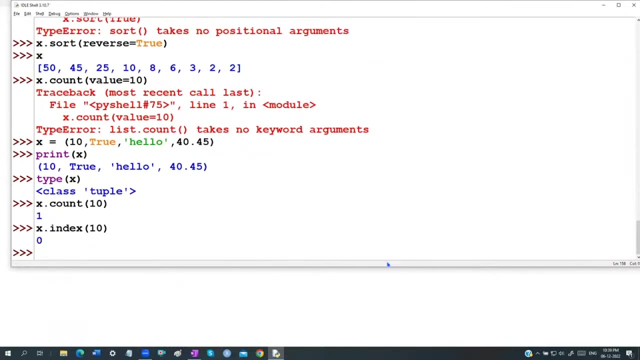 you see x dot, actually guys, once if you said x dot, we have got only and only two methods, actually, guys. i think i need not to show you, but i can just show you the value, actually guys. x dot, count of 10, x dot. if i said index of 10, 10 is there at the 0 index actually. but if i cannot say x dot, append. 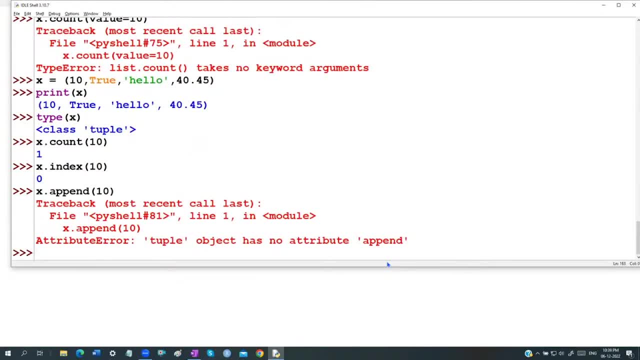 of 10, we'll get an error. tuple does not have a such kind of an attribute called as an append x dot. clear x dot which is going to be sort, or x dot which is going to be append, sorry x dot which is going to be something like a reverse. 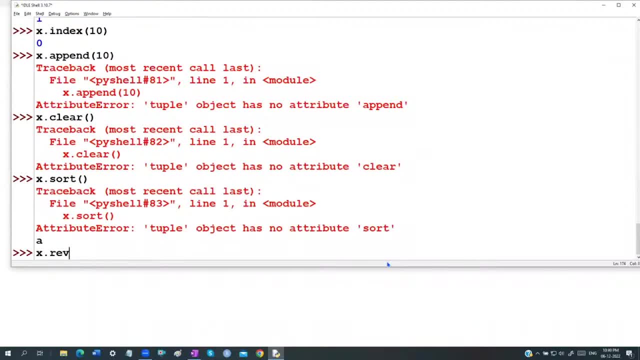 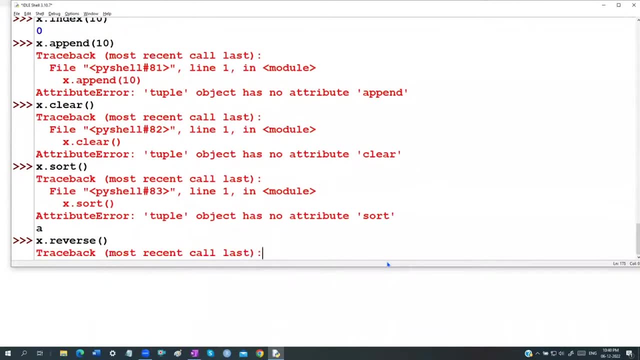 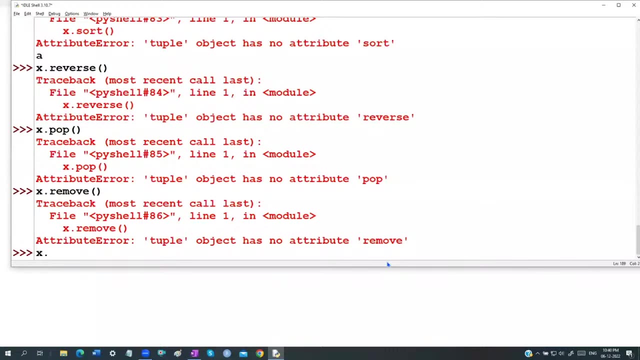 all this method does not works. actually guys, they don't work at all. x dot pop won't work, x dot reverse- sorry. x dot remove won't work. so they are not going to work, actually guys. why? because it's very simple. actually guys, it is an immutable object. but slicing, indexing, everything we can do. 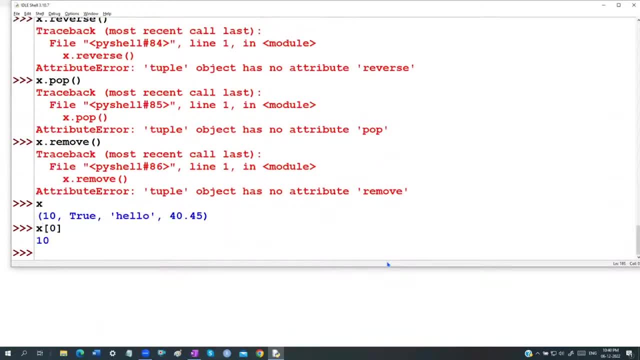 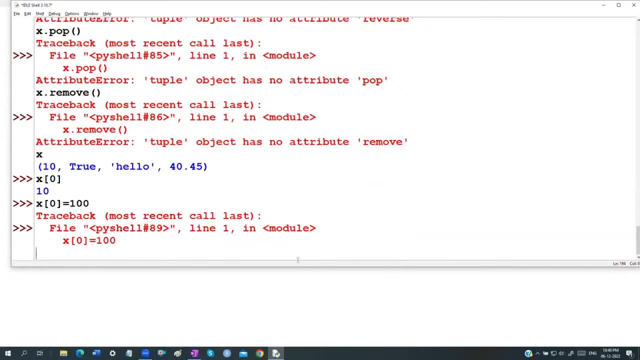 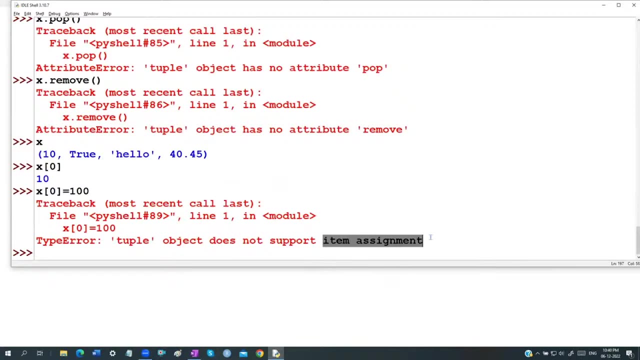 it actually, guys, x of 0. but if i said x of 0 is equals to 100, you are trying to modify the value of 10 to 100, actually, guys. so tuple object does not support item assignment. you cannot assign the value to that particular tuples. so tuples and list are very, very similar objects, guys. the only difference is: 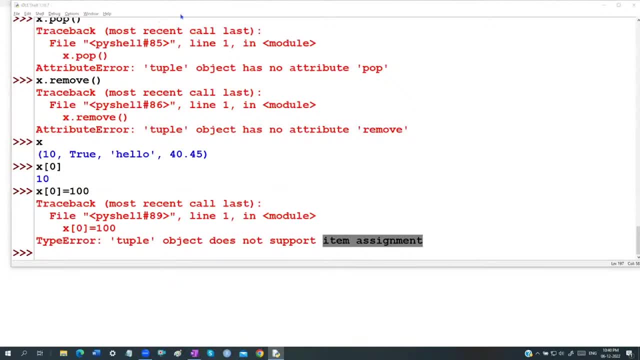 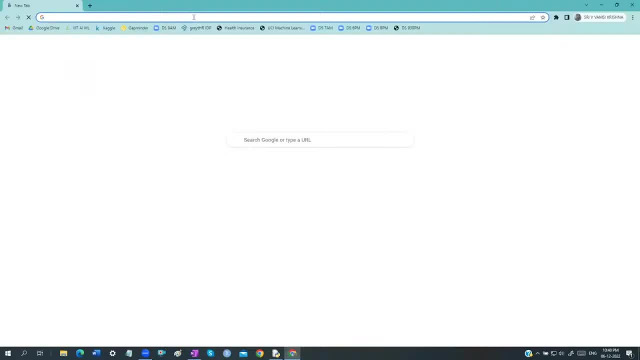 going to be nothing, but the list are going to be immutable, whereas sorry, lists are going to be immutable and tuples are going to be nothing, but there are immutable guys. so tuple was saying: which is going to be list in python, just, you can go through any document. that means as of now i'm 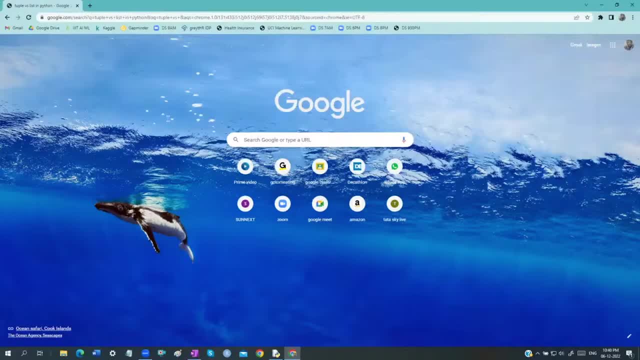 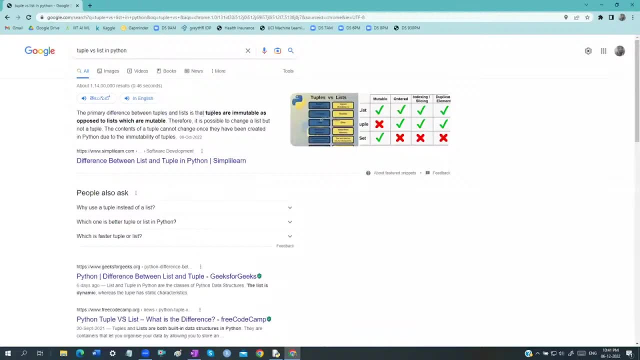 talking about them. guys, if you want to learn, you can just learn the things, actually guys, simple technique, simple application, what we can do. so primary difference between tuples and list is the tuples are immutable, as opposed to list, which are going to be mutable, actually guys. therefore, it is possible to change the list, but not a tuple. 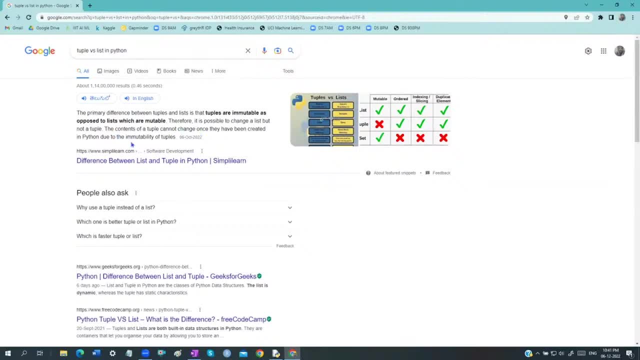 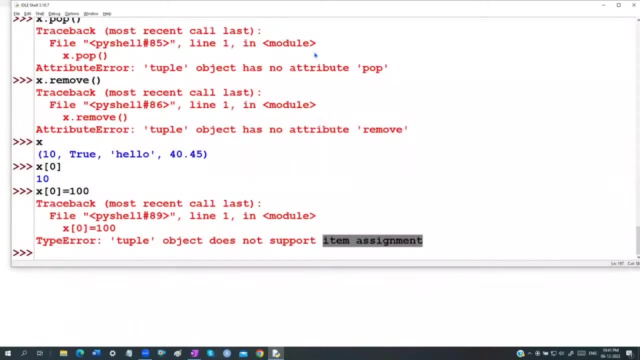 the content of the tuple cannot be changed once they have been got created in python due to the activity of the tuples. actually, simple, okay, so that is going to be about this particular object. yes, yeah, yes, yes, anyone anyone having a question? uh, won't she like what are like some? 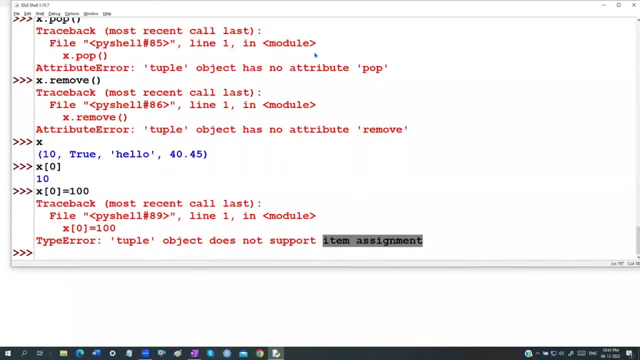 real-time examples where we use list versus couples, we'll use. we'll use it. we'll use it. see, that's why i'm saying that today. see, today we are learning the concept. like, what concepts are there? but in the, in the, in the actual applications, we'll see that. but remember one thing: we never use this tuple. that means we never will. 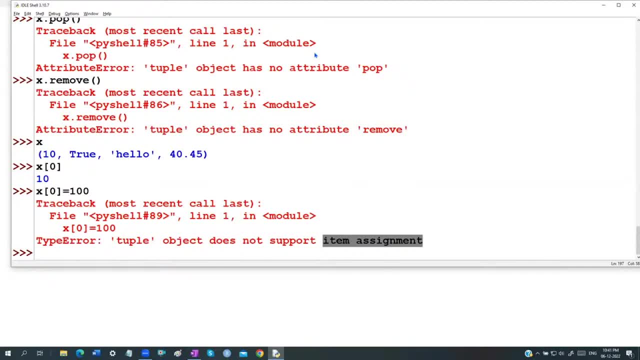 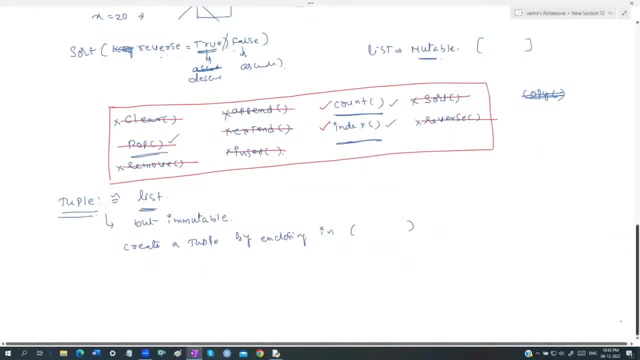 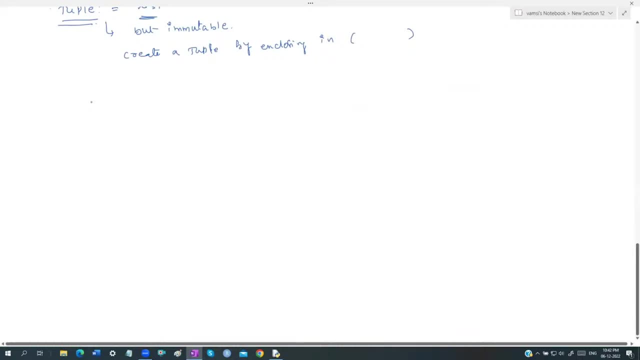 use them. it's very rare cases. we'll use it actually, yes, so i'll tell you like where do you use these tuples? and list is later whenever we are going to be working. so same like how we are using. see how we are using the methods and all these things we are using. in our coming classes we are going to 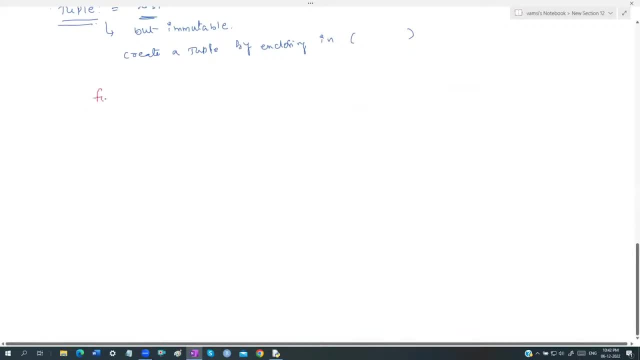 be using a different, different functions. we'll use this function. i'm going to be using a function. this function is going to take an argument as a list. what my point- one of the argument of the function is a list- or one of the argument of a function is: 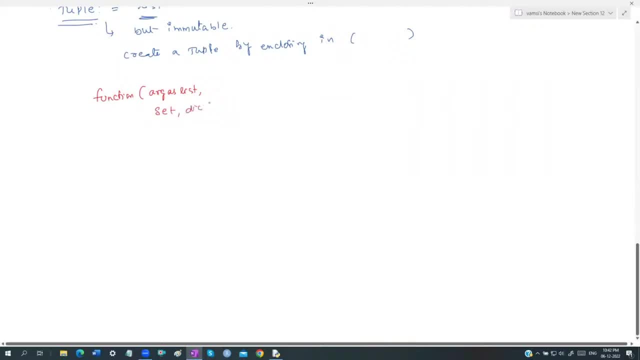 going to be a set or one of the function argument is going to be dictionary. i'm not saying that we don't use it, but the scope is very limited. usage only because in our data science we never want to write any logic. but i'll show you them, like: where do you use it and why do you use it? but most 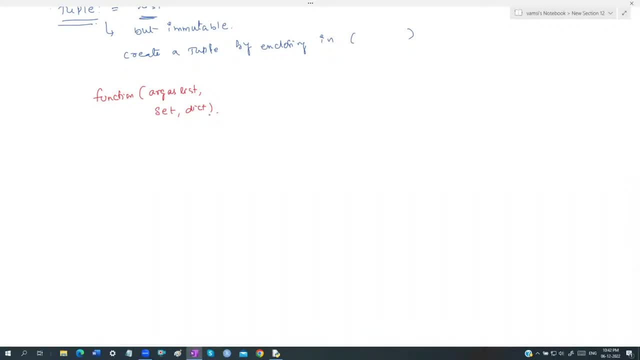 of the cases, these, whatever i am using- list tuples, etc. we are going to be using them as an arguments of other functions. we'll use it to understand that today we are discussing about that. okay, thank you. okay, but we'll discuss. we'll discuss some practical examples of that. 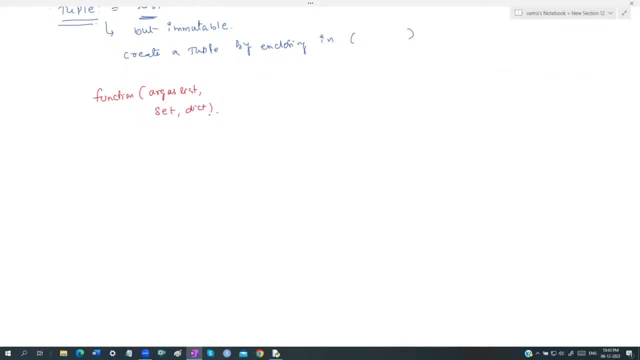 right, guys, okay, guys, um, okay. so just for today, we'll stop it here, guys. um, tomorrow, uh, we are going to start with an another new object called as and set action. tomorrow, completely, we'll work with a set object. only set means something comes to your mind, guys. 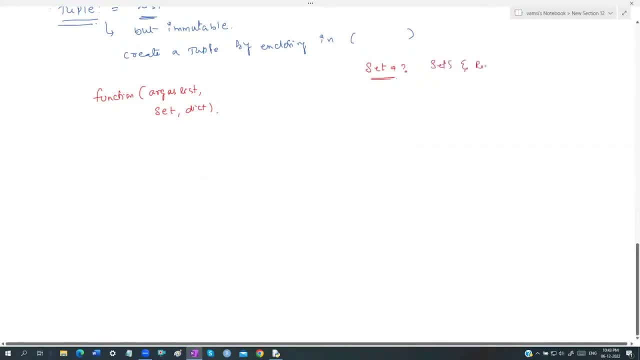 in mathematics we have a concept called as sets and relations topic. is there now, guys? so the same topic we are going to be working in the tomorrow's class with the help of a set object. we'll discuss it actually, guys. sets and dictionaries- two objects are there. let me complete those two objects, guys. 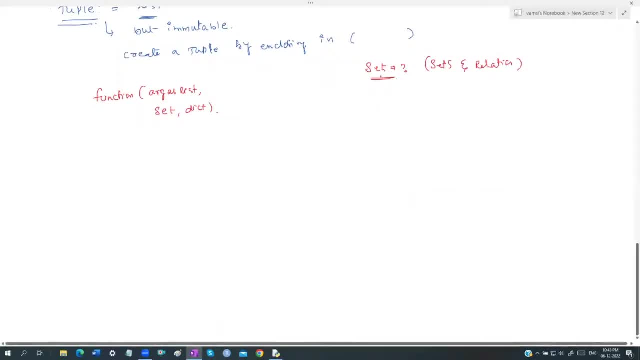 and then, as i told you know, so some people has been joined lately. i'll take a backup session. i'll plan for the backup session for those particular guys, guys, okay, so, yep, it's easily understand. everything is going to be easily. we can understand it. python, guys. python is not a. 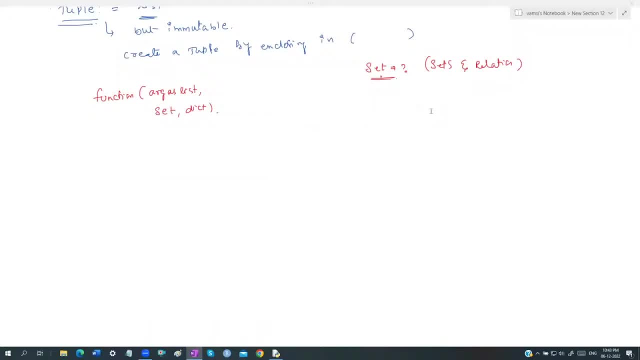 programming language at all. it's just an ideas in coming classes. we never think about python at all. everything is just a function. okay, oh right, guys, okay, so fine guys. um, that's it for the today's class. guys, uh, anyone? guys, any questions? if you have, i can just spend some time and then you can go. 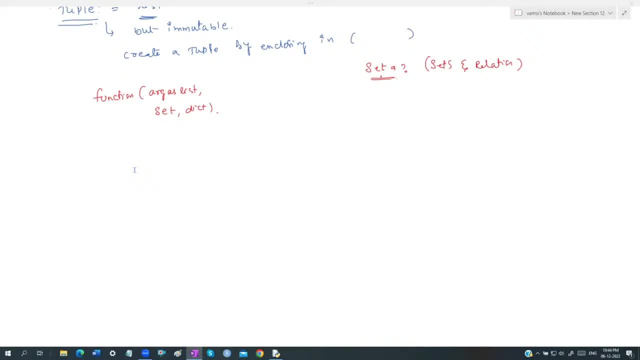 okay, guys, just for today, stop it. yeah, yeah, like we're going to get any uh, you know, uh materials to study. like, yes, yes, you will be getting, you will be getting uh, because, uh, this batch was a little bit delayed actually, uh, it is due to some. 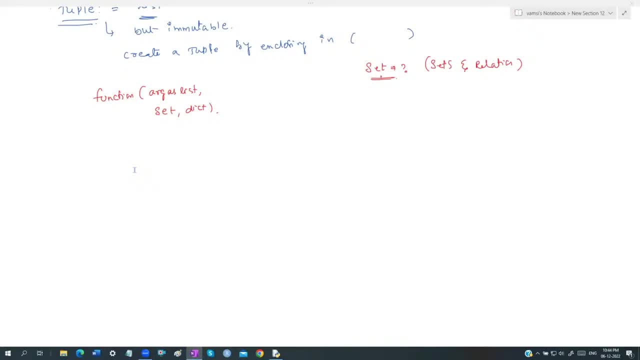 um, very few guys has been joined initially, and then, um some more people has been got joined. so just give me a one or two days of time, um once, uh, other guys also, if they have been, uh, if they confirm that they are continuing the classes, then i'll start sharing the particular materials. but 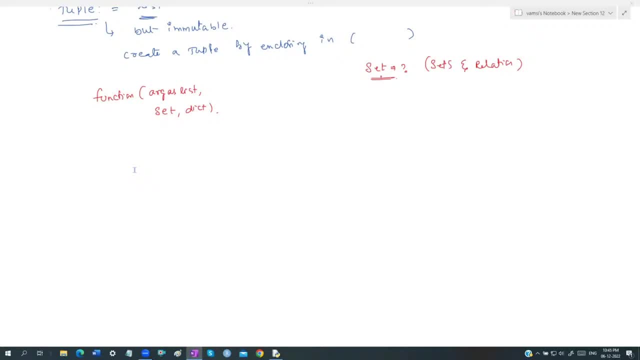 don't worry, because we are still in the beginnings. only, you know, we don't require that much practice. but you can install the python and just you can start with the basics, like basic practical applications. we can try it as often. okay, okay, fine, okay, guys. uh, thanks for today, guys, and we'll meet up in the tomorrow's class, guys. 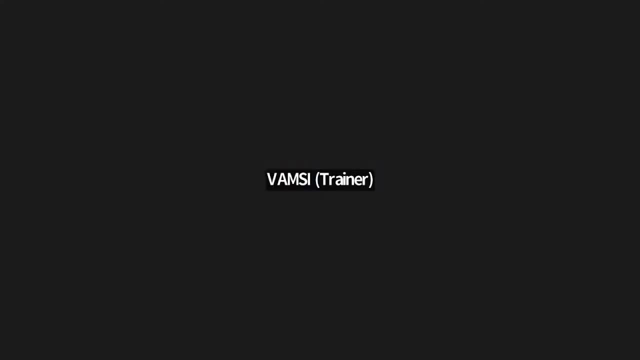 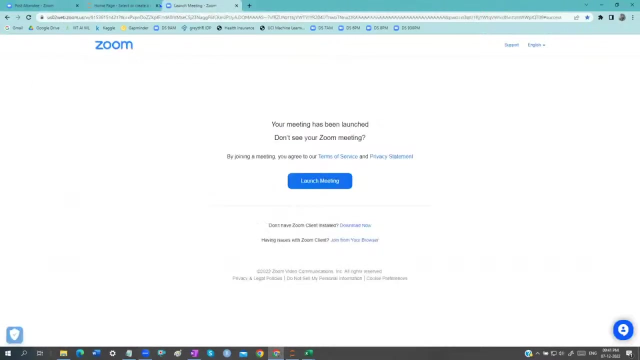 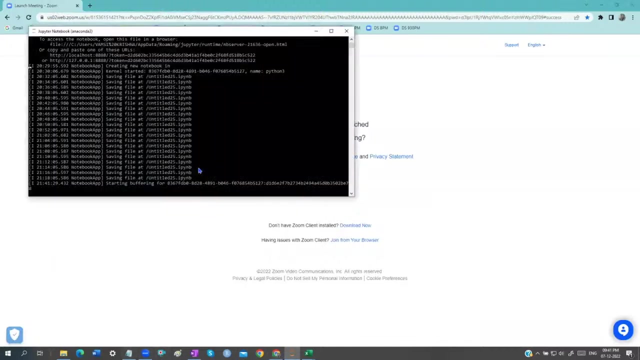 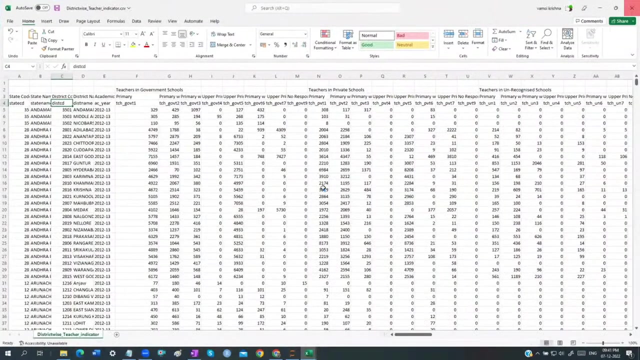 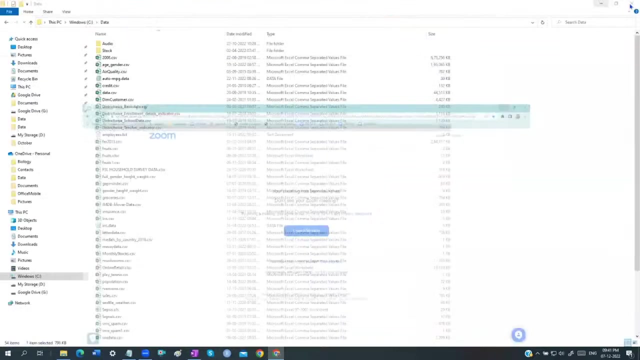 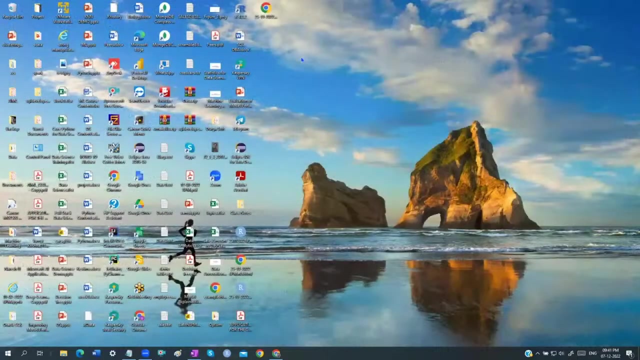 good night all of you guys. you uh hi uh. good morning all of you guys. uh, hope all of you can hear me. anyone guys, uh, can you please confirm? is a multiple guys? yes, sir, right guys. so, guys, um, let's continue with the the last session. guys, let's continue with the last session. 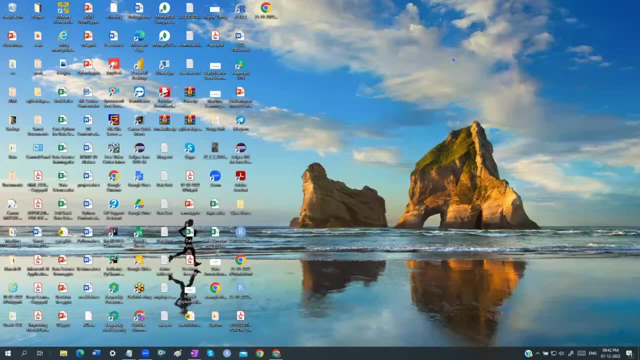 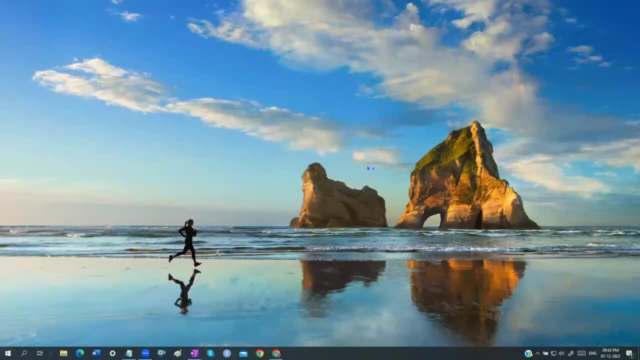 so, um, i'll take up. uh, as i told you know, guys, i will take up the backup sessions for the people who has been joined lately and i will discuss regarding that. i will confirm that related to that. just give me a second right, right, guys? so, uh, let us continue. 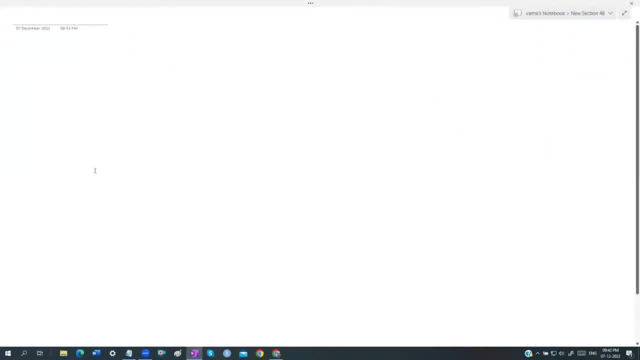 the session, guys. uh, from the last discussion, what we have been gotten, so mainly, guys, we have been studied about mainly two different objects we have been got discussed about that one is going to be the list and the other one is going to be nothing, but it's a triple actually, guys. 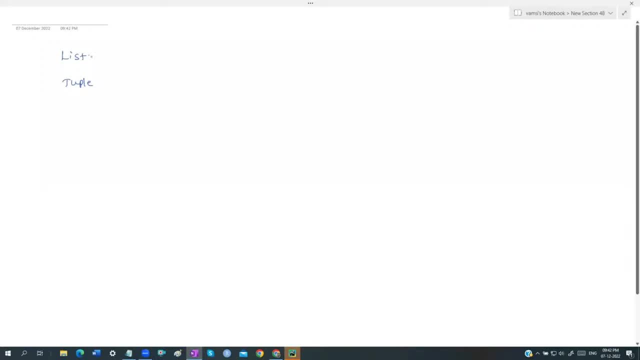 we have spent a little bit time on the list concept guys, because because that is the first object we have been got created, so, uh, we have to understand all the methods. it has been taken some time actually, so mainly we have been seen how to create a list and, apart from that, how to index and 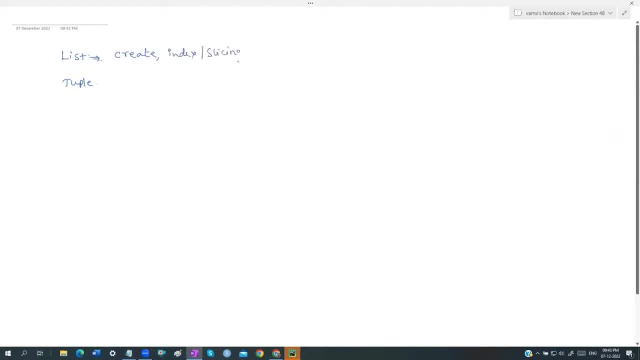 how to slice them. actually, guys, we know what is indexing and slicing. maybe some guys who has been joined lately, uh, maybe they don't have the idea about what is indexing and slicing. but does not matter, actually, guys. apart from that, we have been discussed about the different methods, actually, so at least we have. 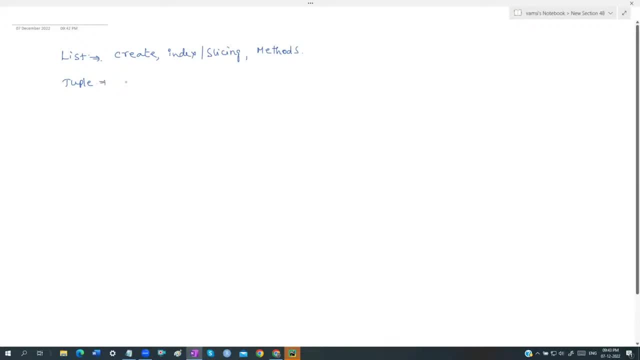 discussed about the different, different methods. same tuple also, guys. uh, creating is the same. only difference is: put them in the square brackets is a list. put them in the parentheses is a tuple, actually, guys. same concept. indexing and slicing is going to be same technique, actually, guys, there. 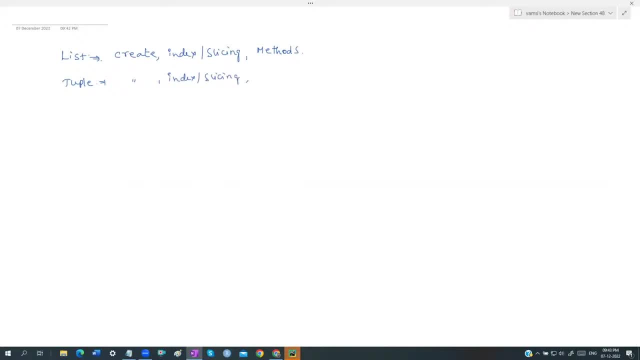 is nothing difference will be there and, apart from that, coming to the methods. just a minute, guys. right, coming to the methods. we have been seen some kind of a methods, but all the methods, whatever that appeared. yeah, so all the methods that appeared in the list may not appear in the tuple, actually, guys, because 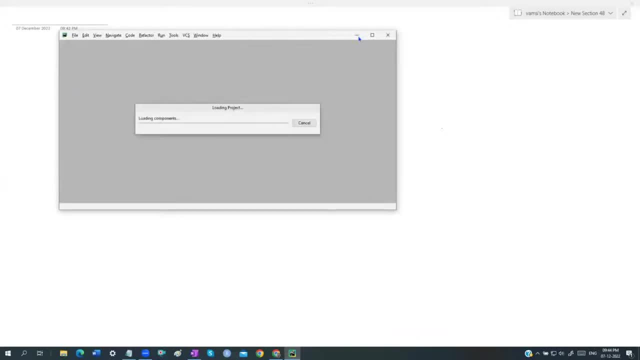 list is a different object, whereas the tuple is a different kind of object. but similarities are there, but only. the difference here is triple is going to be a mutable object, guys, whereas a sorry triple is going to be an immutable object, whereas the list is going to be nothing but what we. 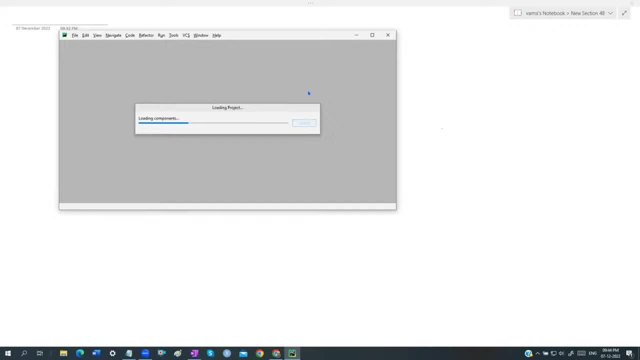 are going to call it as an immutable object actually. so what is our definition of? uh, what is the meaning of mutable and immutable? actually, guys, it can be modified. guys, it can be modified. once it has been got created, it can be modified, whereas tuple is going to be what we call it as an. 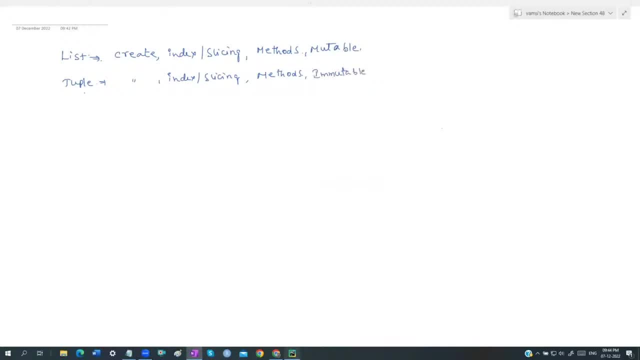 an immutable object what we can say it actually gets. so that is the difference between what we have been got discussed about a listbonsonesse division, one triple, but slicing indexing is the same actually, guys, methods- only two methods are there in the triple guys. what are the two methods we discussed, guys? one is a count and one is an index- only two. 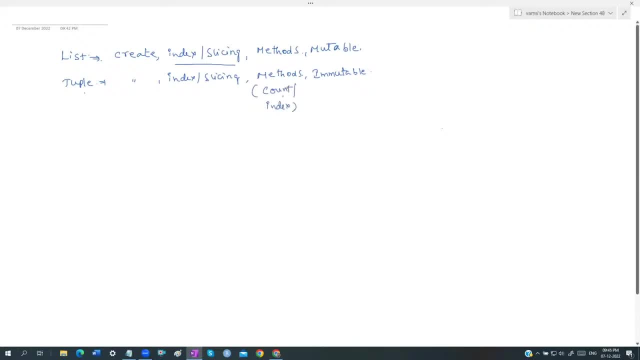 methods are there actually, guys? remaining methods won't work. why? because is we know that clear will try to remove the element from the list. we can't add the elements, we can't remove the elements, we can't modify the elements. but indexing slicing is the same technique, actually, guys. how to index and 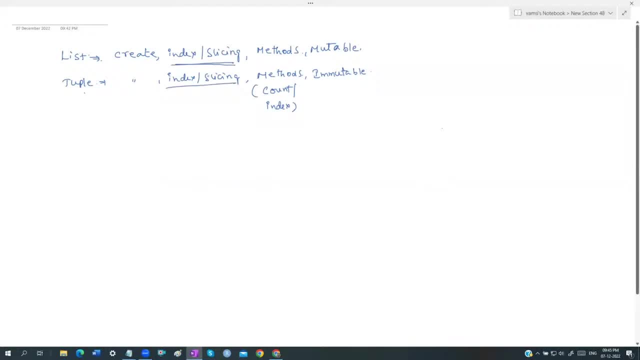 how to slice them. we know that both of them are going to be a collection of heterogeneous values only, but not homogeneous values. okay, uh, it need not to be homogeneous, but how to create a list and how to create a triple. we have been got discussed about that, guys. okay, and just before 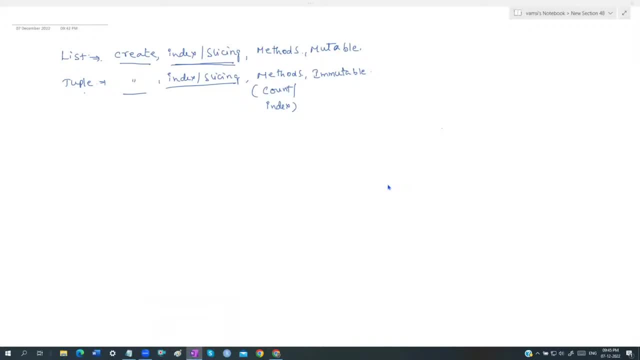 starting the session. guys, i hope all of you have been. anybody guess who has been joined for the today's class? i think i can't see anybody who has been joined for the today's session. um, saeed, i think. uh, is your first session, saeed hussein? no, no, i actually have joined yesterday. 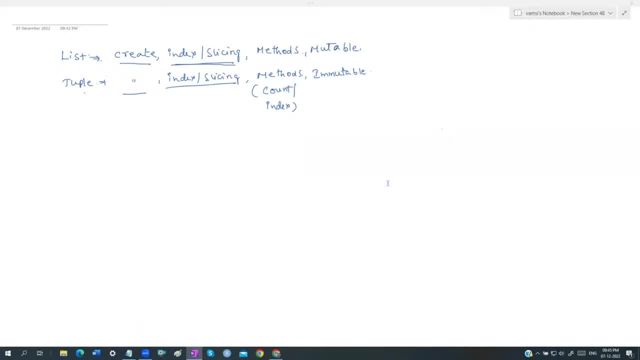 okay, okay, you joined us today. okay, keshav, manohar, yeah, i think all the guys has been um. you have been joined yesterday, so maybe join us today before yesterday, so i think. so, guys, i nobody is there who has been joined for the today's class. if anybody is there, please let me know. 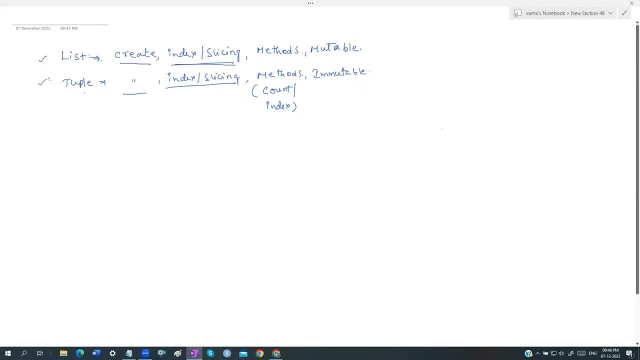 guys, just i'll tell you what has been happened actually and how to cover the previous sessions. okay, so once again, guys, there is a list and a tuple concept is going to be there, guys. so, uh, how to create a list and how to create a tuple, just once again, quickly, two, three minutes. 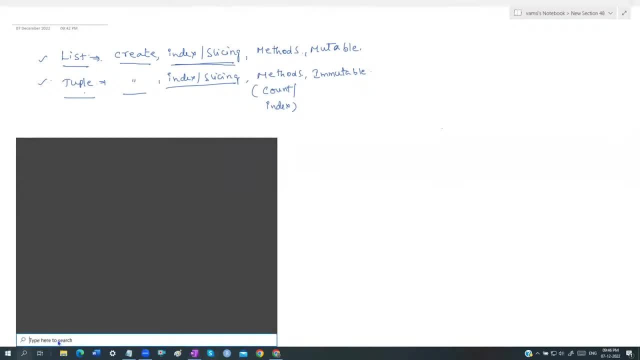 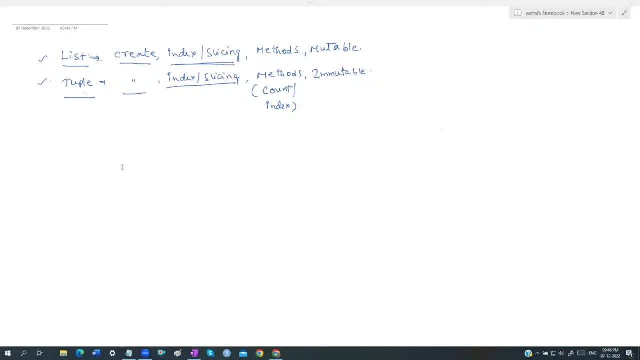 i'll just finish off it, guys, so that we can get some again, some kind of a conclusions. what i can do is, guys, so let me open the ideal guys, let me open the ideal. let me open the ideal guys, but as i told you know, guys, we don't work with the. 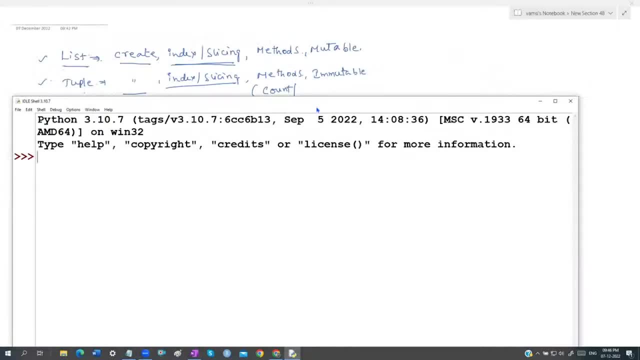 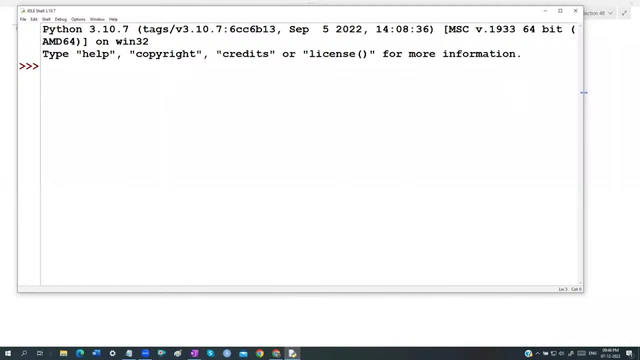 ideal for completely. that means complete course. we cannot run it on the ideal actually. yes, only as a beginners, only we can study them, but after that we are going to use an a better ids. we are going to be using them actually. better ids will use it actually. once again, guys, a quick. 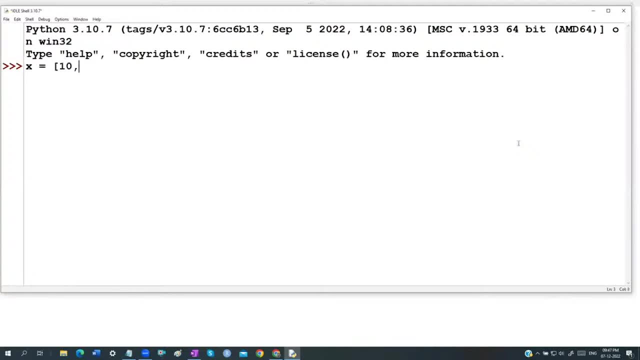 understandings, guys. let us say x is equivalent to nothing. but either i told you we can give a sequence of numbers or don't give it easy to understand. i'll take it actually, guys, type of the x very clearly we can see. x is a list. you can also. 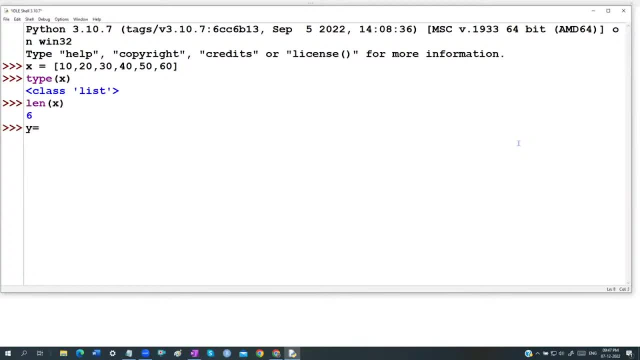 ask: what is the length of the x? same example, guys. i said y equals 2, which is going to be same numbers, same numbers. i'm giving it actually, guys, but it is going to be a triple. actually, guys. what is the type of the x? type is a function which will let you know about what kind of an object it is going. 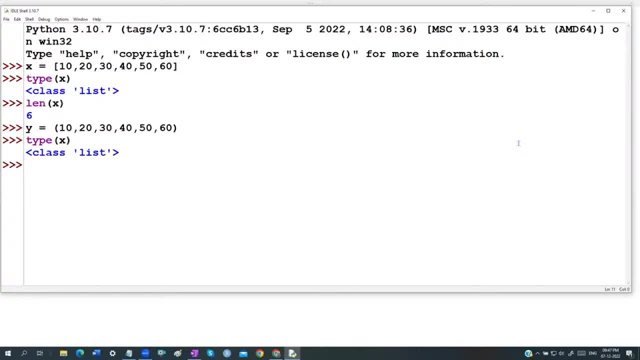 to be there. so class x, which is nothing but it's a class list. and what is the length of the y? you can see that it is going to be nothing, but the six is the result: same length, same data. next, print the value of x, x. print the value of y, both you can find it in a same values, but both of them are going. 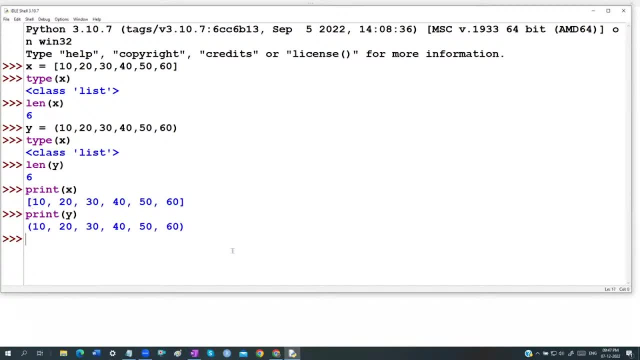 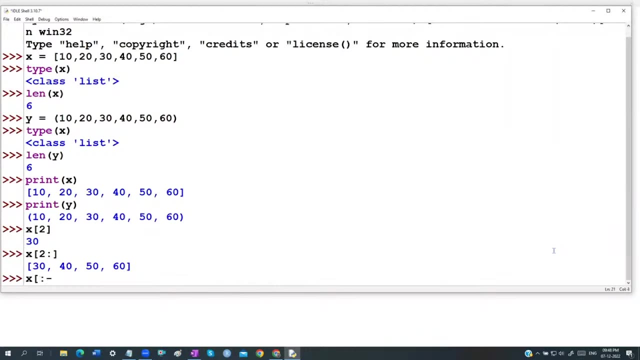 to be represented in a different way actually. so how to slice and how to index? actually the same technique as x of 2. we know that we are going to get a third element. x of 2 is 2. starting from the third element, we'll get the remaining elements. if i said, x of which is going to be minus 3. 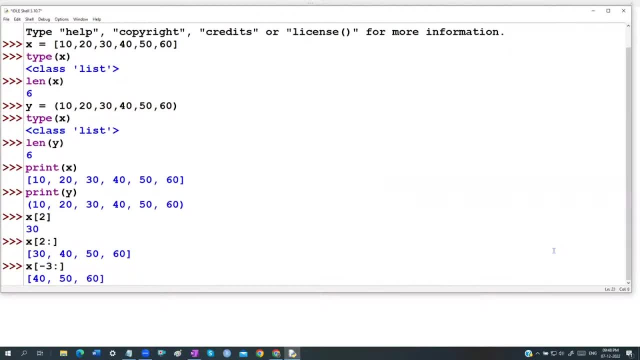 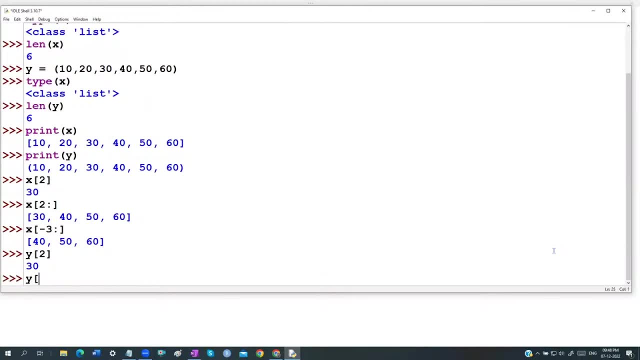 minus 3 is 2. actually, guys, it is going to be nothing. but the last three elements will come actually, even if i said y of 2. also, the same result will come even if i said y of 2 is 2 actually. yes, but one slight difference. you have to find it off. you know what is meaning of a slice. 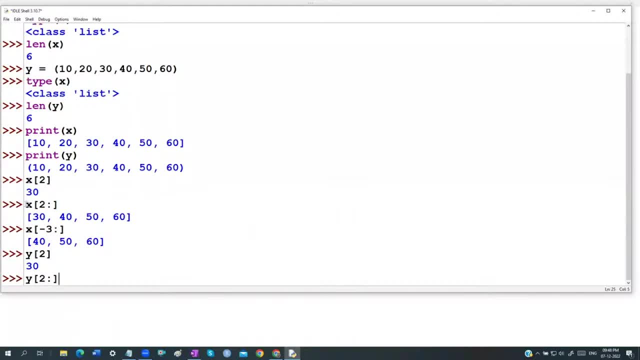 slice is nothing but a piece. so if i take a slice from the x, result is again a list. only guys. you have taken a slice from a list. the result is again a list. you are taking the slice from a triple, so result is going to be again a triple guys. result is the same, but here. 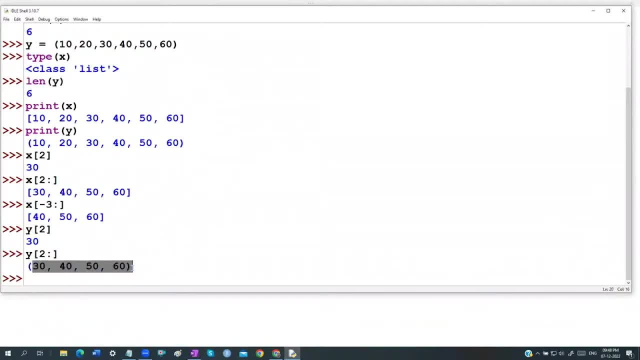 we are getting a list. and here we are getting a triple. actually, guys. same technique. whenever i said y of minus 3 is 2, result is the same. what is minus 3 is 2? actually, guys, it is going to be nothing but last three elements. we have to get it actually. so whenever i slice a list, we got a list. 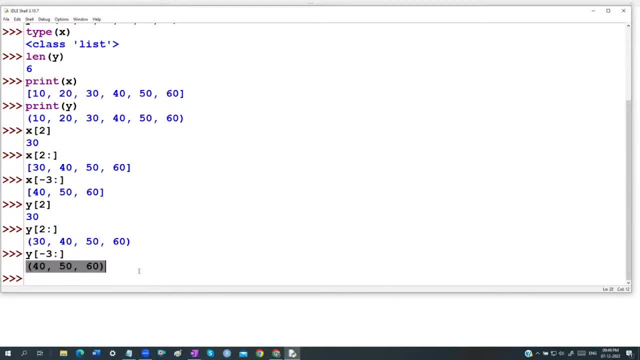 when i slice it triple, we got a triple. actually, same technique, same application. if i say x of minus 1, it is a indexing. actually, guys, it is y of minus 1. actually, the result is the same result. both of them are giving you only as an, an integer value. we are 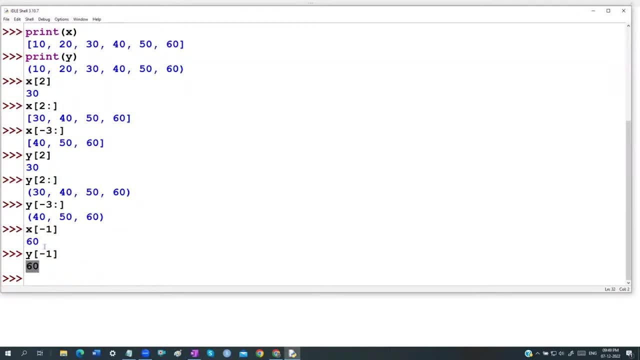 getting it actually, because indexing can give you any value, but slicing will always give you at least. slicing will give a list, a triple, slicing will again give a triple only. but what are the methods associated with? actually, guys, when i said x dot, i told you know there are totally 11 methods. 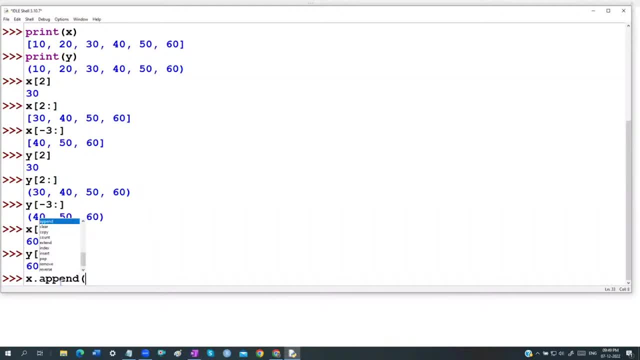 will come. i can append the data. actually, guys, i can append the data to the x, actually 70, i can append it. but same example: if i said y dot append of 17, you will get an error. actually why? because append is a method which is associated only with a list class but not with a tuple class, and tuple is an immutable object. 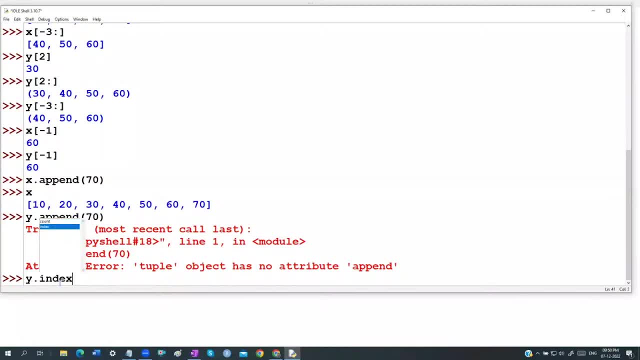 when i said y dot, only two methods will come. actually, guys, what are the two methods we can see? only count and index. only two methods actually count: will count how many times the given value is there. index is going to tell you where is that particular value is going to be there actually. 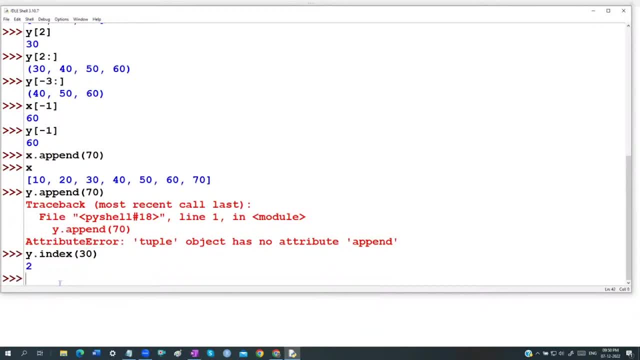 was there. it was there in the second index. what we can say? so concept is very straightforward, guys. there is nothing complications, nothing logical part will not be there. everything is just we have to know how to use it, actually, guys. okay, so there are two more objects, are there, guys? let me complete. 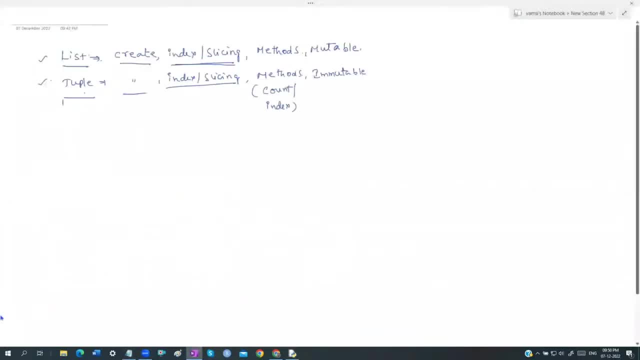 the two more objects and then i'll take up the. i'll go back to the backup sessions guys. i'll talk to the guys and then i'll decide it really. do you require a backup session or do you can manage? according to that, i will take a backup session. let me complete. maybe today, tomorrow i'll complete. 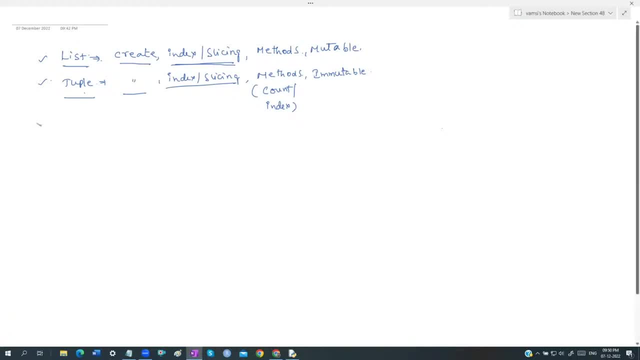 of it, actually, guys. so today we are going to be discussing about a new object called as, which is going to be nothing but a set object completely. the today's session will be on the set object, actually, guys. concept is simple, but only the thing is: more and more functionalities are there. 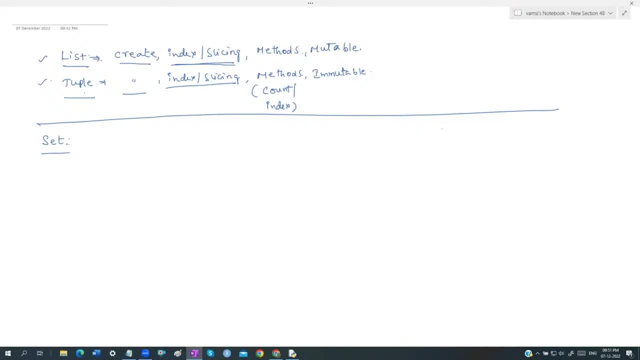 so i have to explain those particular topics, actually, guys. so once again- which is going to be nothing but the same concept- what we are going to do is we are going to take a backup session another way, because, basically, we are not setting it up to on, we are going to take a backup session. 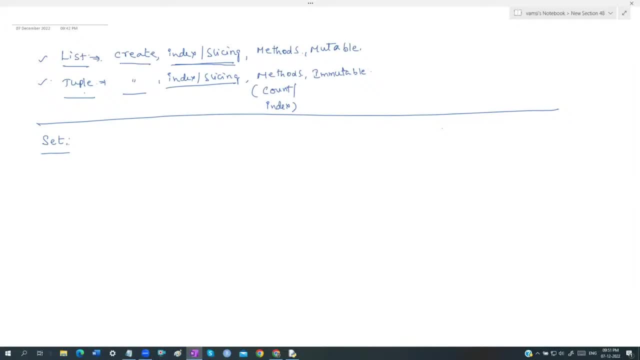 but this concept is not going to be a set object because actually, when you check on n, you will see the below right. it has something like a set object. get all these things and we are going to be doing so. in this case, we are having a set object. ok, it is going to be a set object what we are going to be. 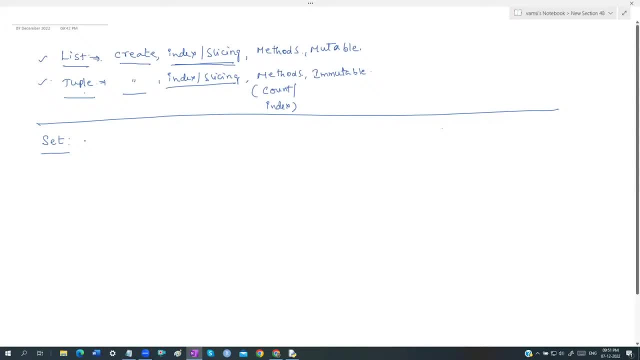 gets doing is going to be nothing but what we can say that it is going to be set object. actually, remember, no guys, that is going to be nothing but sets and relations, set operations, okay, which is going to be something like an intersect. we have union, we have something, part as a minus, i hope. 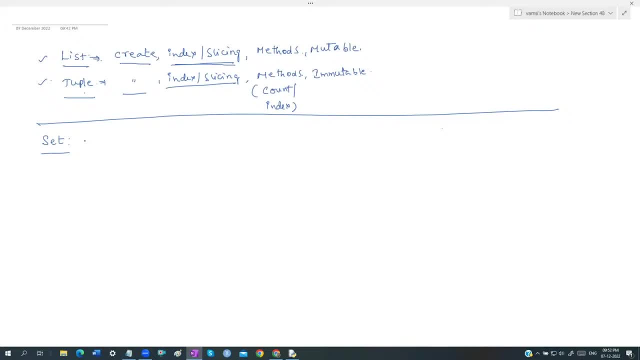 you remembered, guys, we are working with something like an set, operator, subset. it is going to be super set we are having. so same topic is going to be set concept, actually, guys. so in mathematics also, you remembered, guys, how do you represent a set? a, it is going to be like this: we are going 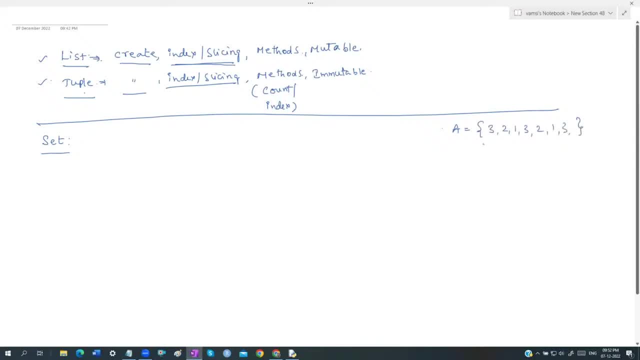 to be representing, actually, guys, it is enclosed within curly brackets, actually like this, or a curly braces or a curly brackets. what is a set actually, guys? set is also: what is the difference between list and tuple? both of them are going to be same. and one more thing is going to be nothing. 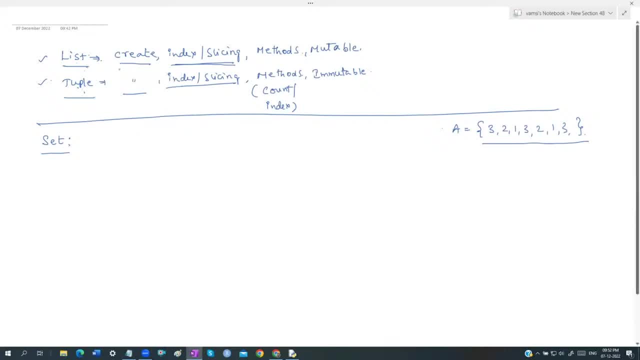 but one more thing is going to be nothing, but both of them are same. and one more thing is going to be nothing, but only just is: both of them are homogeneous or heterogeneous. one is a mutable, one is an immutable. what is a set object? actually, guys, set object is going to be nothing but what we are going to call it as, and, guys, it is nothing. 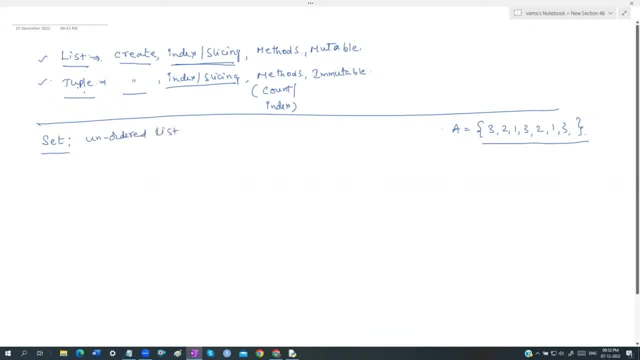 but an unordered list. what is meaning of unordered list? actually, guys, unordered list. i'll tell you, i didn't complete it. actually, what is meaning of an unordered list means, for example, in a list, when you are creating a list, if i give the values like 10, sorry, 20, 10, 30, 40, if i give the values like this: 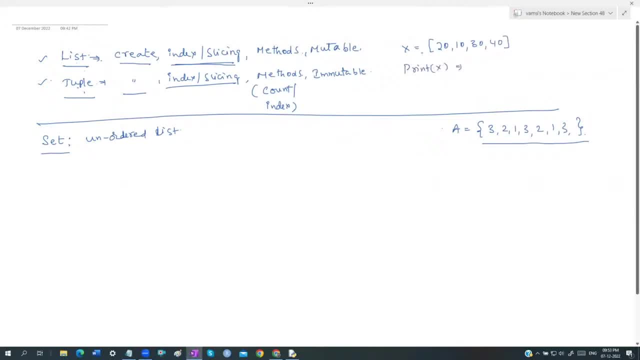 in the value of x. it will maintain the same order actually. so it is going to be: preserves the order actually. we'll say that it will preserve the order actually. yes, it will preserve the order. even whenever i work with the tuple also, the same order is maintained, which order you give. 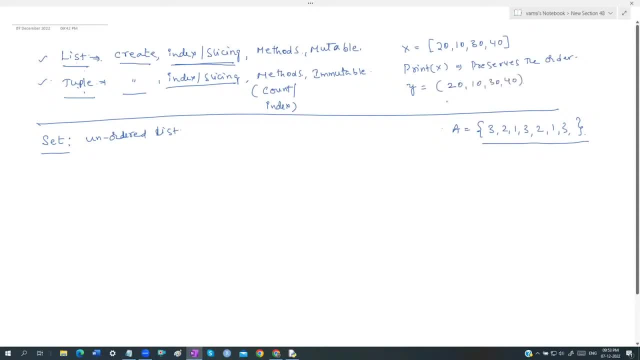 same order it will maintain. it does not change the order. actually, yes, but what is meaning of a set is unordered list. actually, what is meaning of an unordered list means you give one value, you give some order, you give some value, you give some value, you give some order, you give some order. 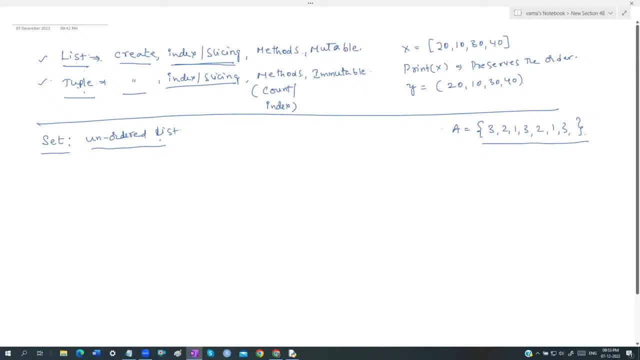 we'll get a different order. guys, you give some order, we'll get a different order. if i give this order, there is no guarantee that it will get the same order. only, it does not preserve the order. actually, it does not preserve the order. it is an unordered list of one more thing. actually, guys. 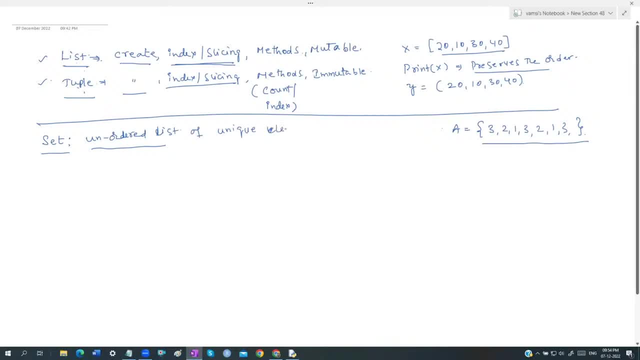 it is an unordered list of unique elements. you know what is meaning of unique elements. actually the values or the elements which cannot be repeated. but in list, we know this. actually, guys, we can have multiple times. i can have the same number as many times you can have it even in the tuple. also, you can have the same element repeated number. 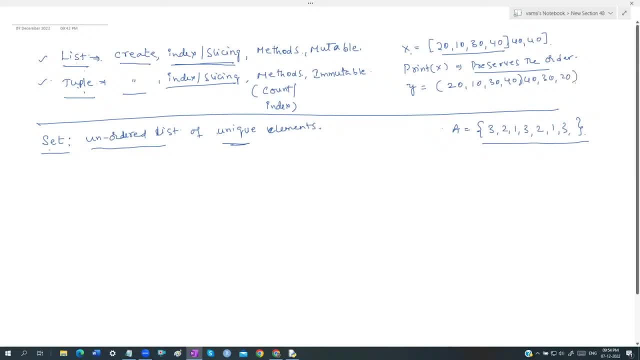 of times, but when it comes to the list, only two features are there, guys. one is unique elements. that means the value should be. the element should be there only for one time. the element should be there only for one time only. it is going to be what we are going to be gets doing this actually. 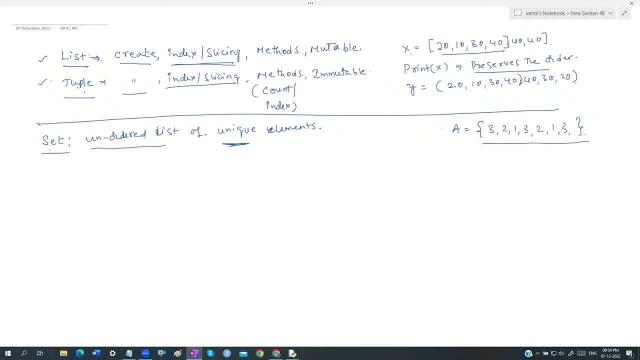 so this is going to be the one what we can say. that and one more thing is going to be nothing, but you can see that, which is going to be what we can see, is it is going to be something like an unordered list of values. actually, guys, what we mean is an unordered list of values, means. 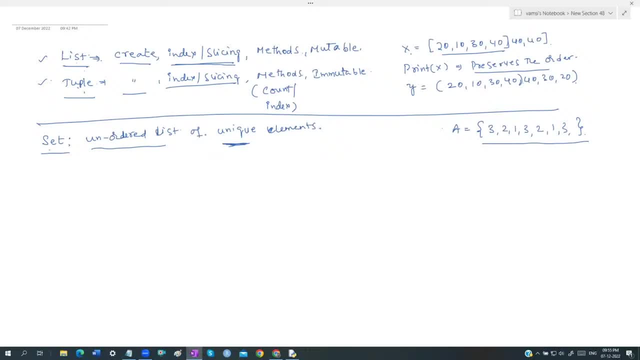 whatever the order we give, it does not use the same order as it is. it gives something a different order. we are going to get it. actually, yes, we will get a different order. your input is one order, but your output is another order. so, due to it, does not maintain that order. indexing and slicing is not allowed on the set object, guys. 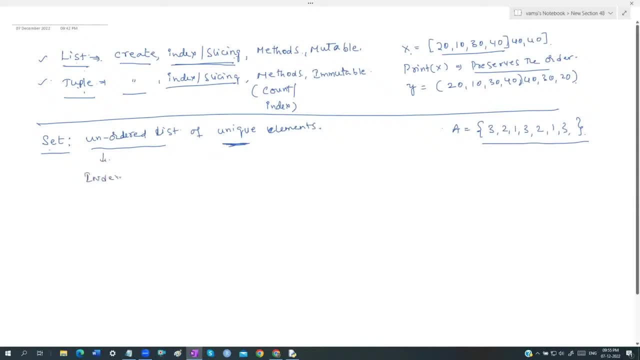 it is going to be. indexing and slicing is not allowed, so we cannot get from a set. if we want to get third element means we can't get it. actually, guys, indexing and slicing is are not allowed. actually they are not allowed. on the, indexing and slicing are going to be not allowed. 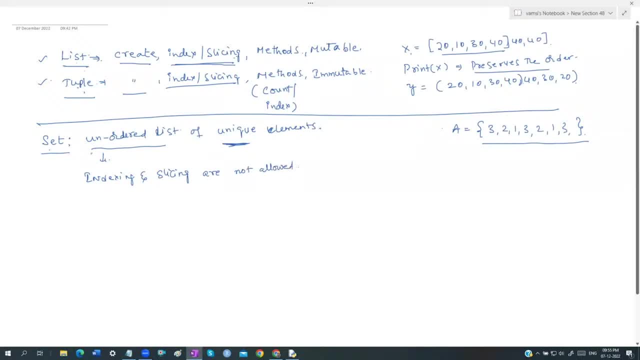 why it is not allowed. actually, guys, because whatever the order we give is different, whatever the order that comes is going to be different. actually, and that too, if i give the values, even if i give the values, like this, guys, you give the values, repeated values, you give it, it does not throws any error, but it takes only unique values only will be. 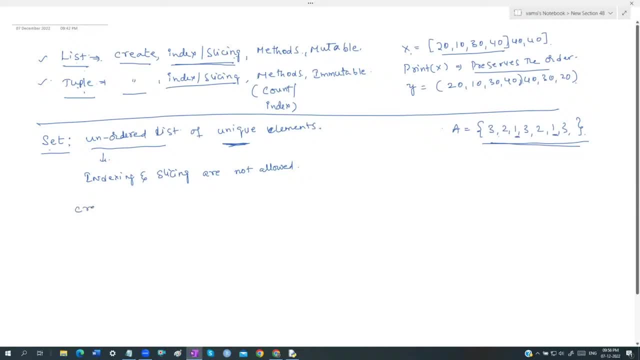 selected, actually guys. but how do you create a list, sorry? how do you create a set? create a set by enclosing in parentheses, sorry, enclosing in the curly brackets, actually guys, the curly braces or the curly brackets. very simple, guys. so square brackets. if we enclose, it will becomes a list. and if i use a parenthesis, and we are going- 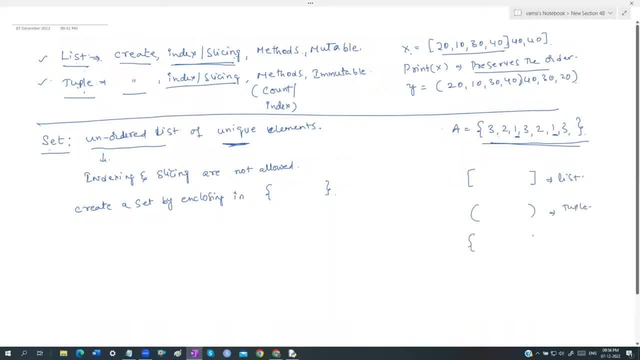 to call it as an h-tuple, and whenever i use a curly brackets, we are going to be getting which is going to be something, what we are going to call it as an, a set object, what we can call it as. so for a normal, if i show the same example to a c programmer, tell me if i said, x equals to this. 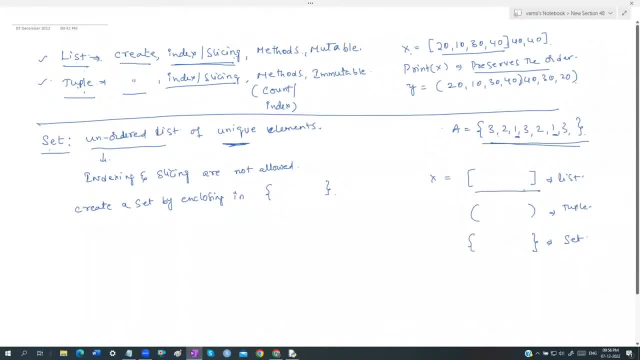 much. what is the type of the object it is? he cannot say about that in c language because c programming, java programing, we are having an habit of writing list, tuple set something. we have to use the keywords actually, but in python you don't use any keywords. actually, x equals to square brackets, y is equals to some. 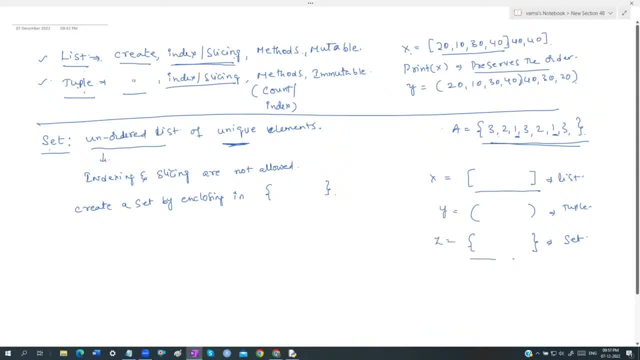 parentheses. z is equals to calibrances, it will automatically becomes a set, but it does not preserve the order, actually guess- and it is going to accept only unique values, only being. the order is not preserved, so indexing and slicing is going to be not allowed on this particular. 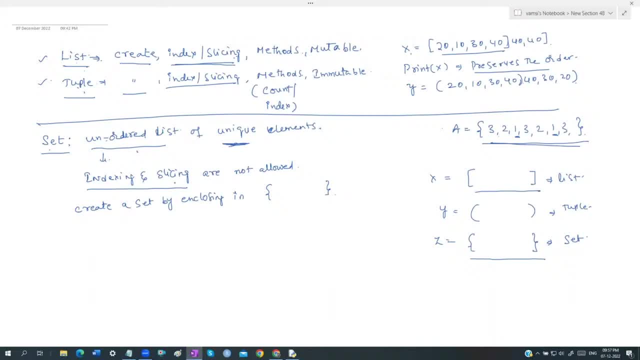 set objects, actually guys. indexing and slicing is going to be not allowed on the this particular object. what we are going to be gets doing this actually guys. okay, so that is going to be the concept of how we are going to be gets working with the set object, but we have a number of 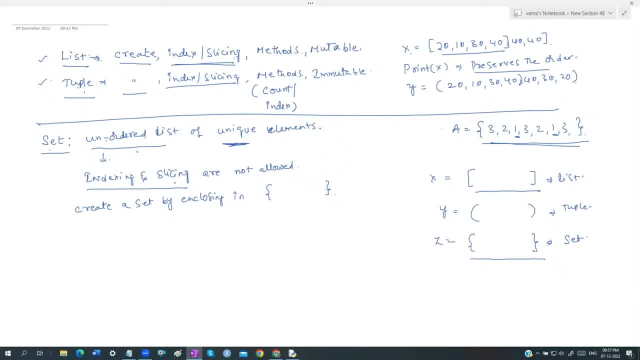 methods are there, guys, but nothing is there. only thing is, i have to just do some practice on that. it will take some time, but otherwise it is going to be a very simple. techniques only, guys. let me create the set objects. how do you create the set objects? so let me show you how to create the set. 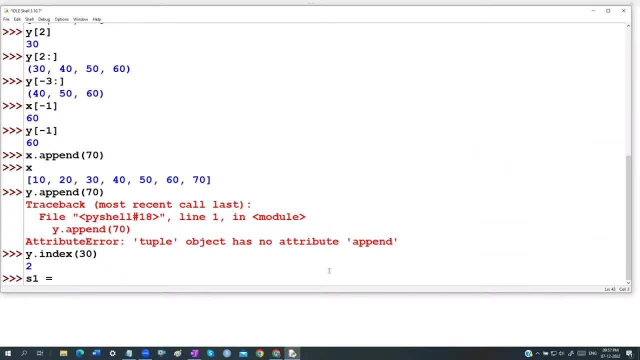 objects. actually, guys, let us say s1 equals to, for example, guys, just, we have to use the curly brackets, just use the curly brackets. actually, guys, 20, 10 again at 20, 30, 10, let us say 30 again, 20, 40, whatever the data you give, you can give it. actually, yes, just i'm giving some few values. actually, guys, 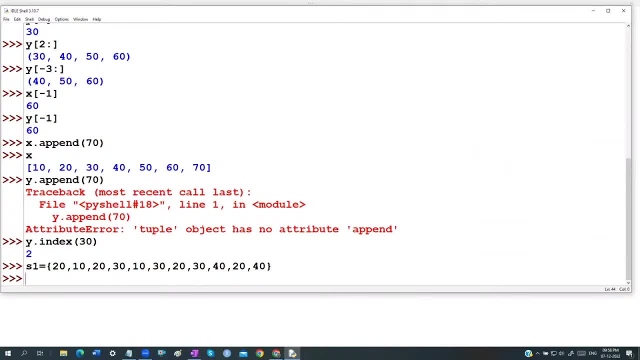 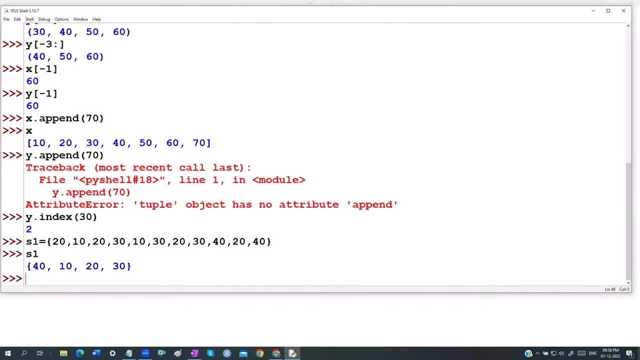 so don't think that i have given some 1, 2, 3, 4, 5, 6, 7, 8, 9, 10, 11 values. if i print the value of s1, see, whatever the output, we are going to get it actually yes, see the s1. actually yes, 40, 10, 20 and. 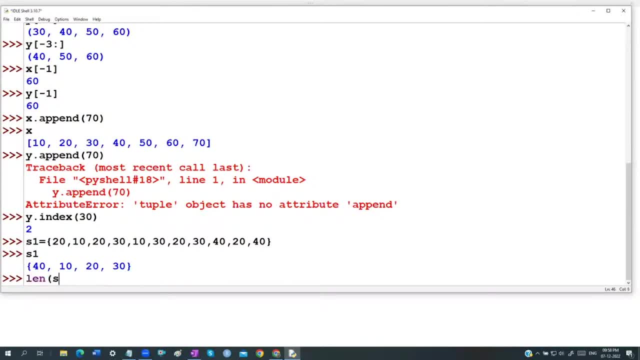 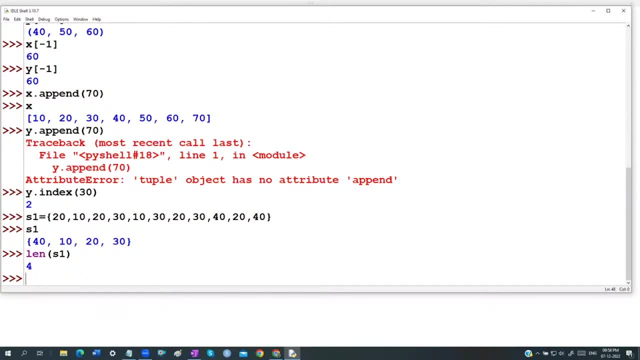 30, even if i said length of s1. actually, yes, length of s1 is not going to be 11. i given 11 elements, but when i said length of s1, you can see that there are going to be only four elements. are there because it will take only the unique values. only we can take it. if you have any doubt, i told you. 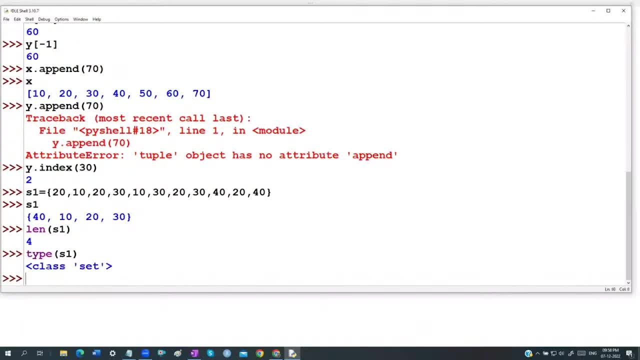 use the function, call as and type function. what is the type of the s1? it is clearly saying that it is a set object. that's it guys, just very simple. it is s1. what is going to be the s1 here? now? it is a list object. so what is? 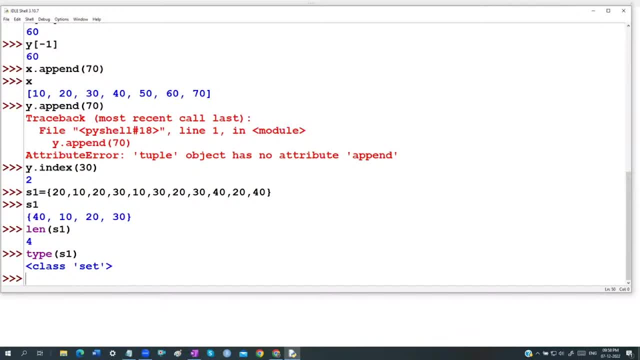 the length of the s1. instead of giving 11, we are getting only four. only why it is only four? why? because this we know that it is going to be a collection of only unique elements, only what we can see. and what is the first point i told you guys: indexing and slicing is not allowed, so s of 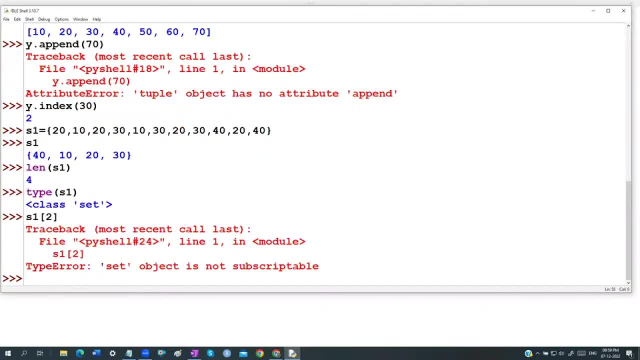 sorry sص, of which is going to be two. this is not allowed. actually, guys. set object is not subscriptable. we cannot subscript it, actually, guys, we cannot. subscripting is also nothing, but you are getting. you know what is meaning of subscripting, actually, guys. so getting some part of them which is not 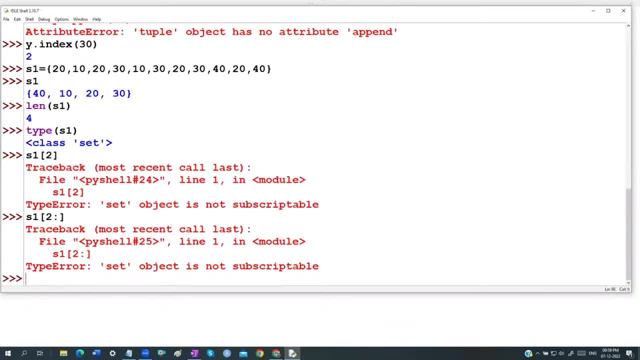 possible. even slicing is also not allowed. actually, guys, slicing, indexing is not allowed as of the set object because the main reason is they are not following any particular order in a list. if i give some values, i know that i have given 10 at second index. if you ask second index starting from second, 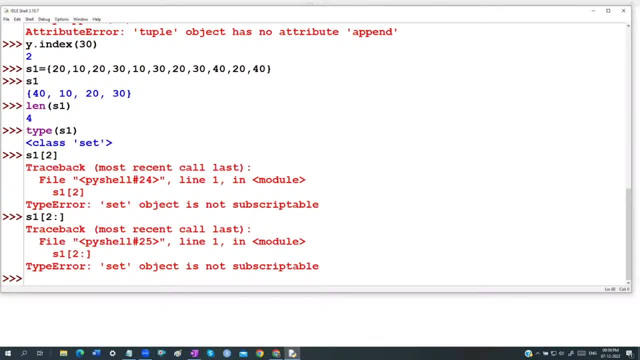 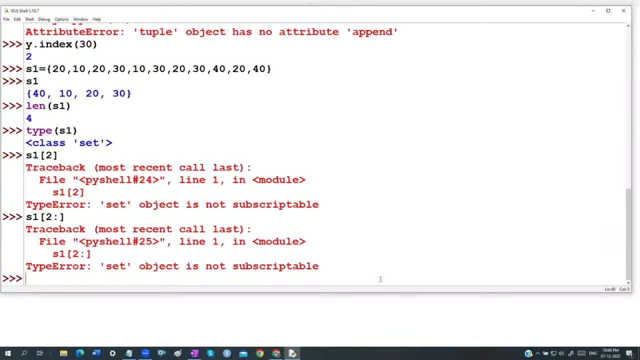 it's not like that actually. why do you require a set object, is i told you. i said also. i told you one point. these are going to be some of the. what we can say is: these are the basic things which we have to learn as part of the list. i'm not saying that they are not used. i'll tell you like why. 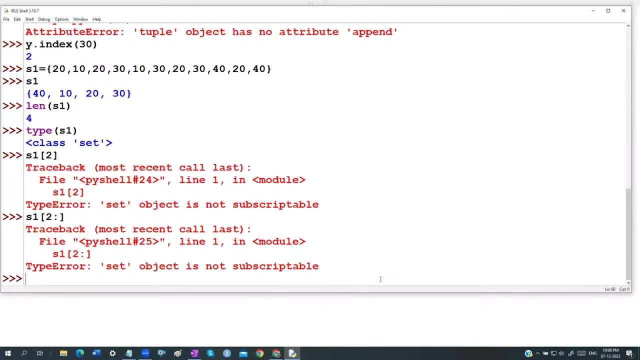 why we are not going to use this and etc. why do you use it? but just for a timing. let me explain that. so, as i told you that in python the list tuple sets dictionaries, these are the basic data structures. so that's the basic thing that we have to learn as part of the list. i'm not saying that. 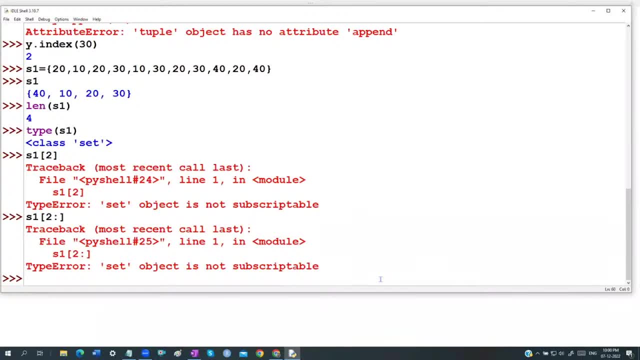 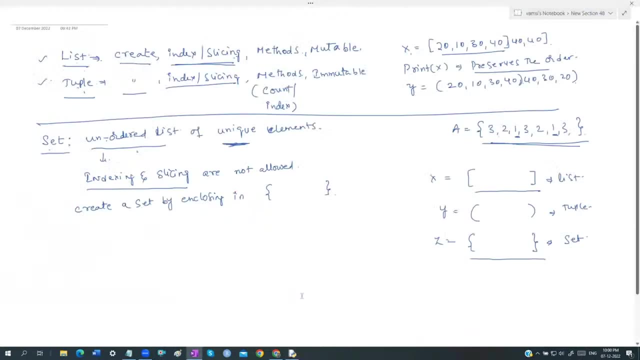 is the reason why you have to. if you are learning python means at least some basics. we have to learn it actually. why do you use it? actually, why do you use it? means i can explain that like i can explain it, but the things are like you may not understand the things actually. just let me. 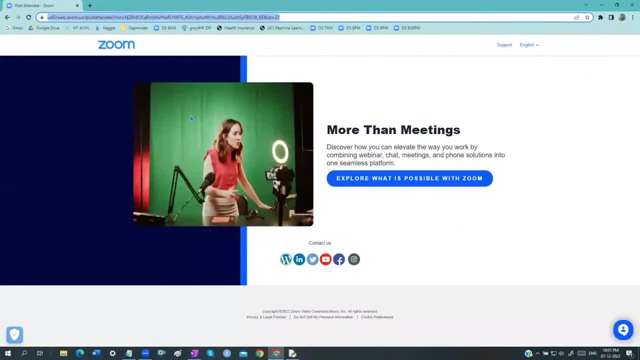 show you that application. actually, don't worry because being you have been asked for, like why we are going to be using that, i'll show you some practical application for that. i cannot explain the concept because you really don't know what is. um, i really don't know what i am. 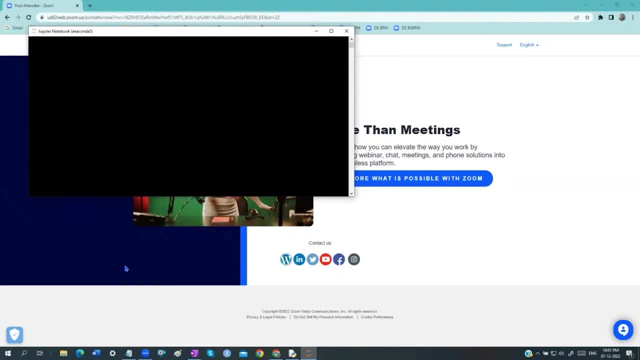 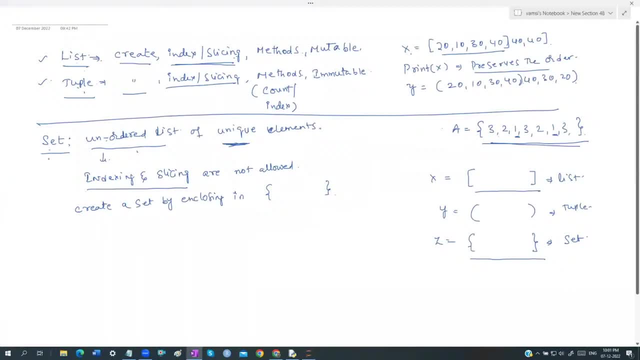 explaining that, but i can just explain the things like, try to understand it a little bit carefully. so let us say that, basically, why do you require here? is you know the set operations? no, like we have the concept of intersection concept. we know that actually. so intersection can be applied only. 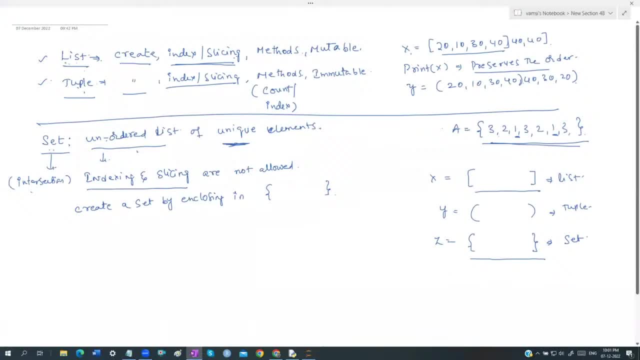 whenever it is a set object on list. we cannot say: i cannot find, uh, intersection between two list. we cannot find the intersection between two tuples actually. now just an example. i have some kind of an, i have some set, some values. are there guys, some random numbers, are there actually? just 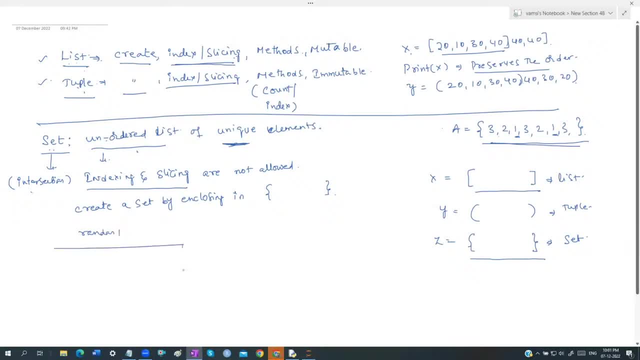 an example: some i'll take some random numbers, one actually, guys, some it is having some values like like some 20, let us say we have a 15. we have in 25. we have 11, 16, 18, 17, 43, some you may have also. 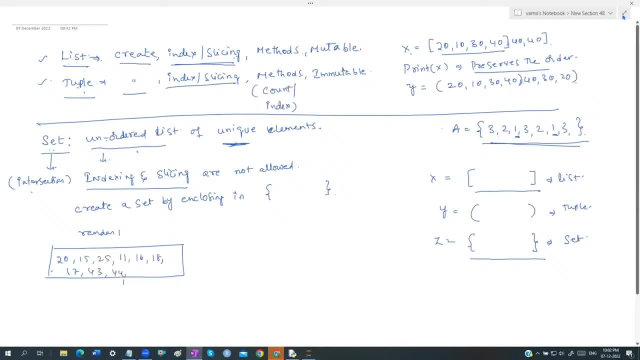 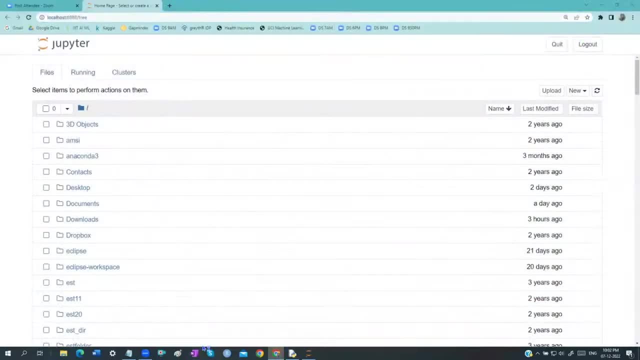 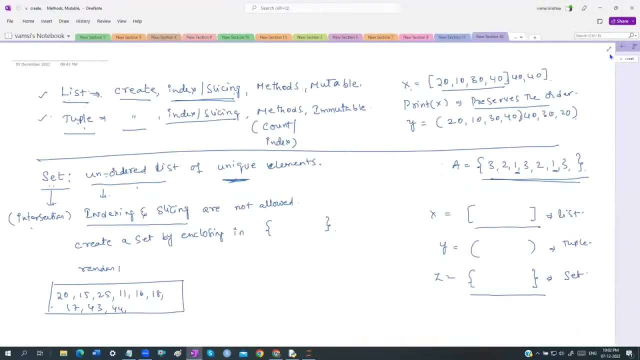 repeated numbers also does not matter. let us say 44. just a second: guys, actually white is blinking. let me just give a second. see, whenever the values are very small in numbers, we can easily identify that. we can easily identify that. but whenever the numbers are very large in numbers, we cannot do it. actually, guys like 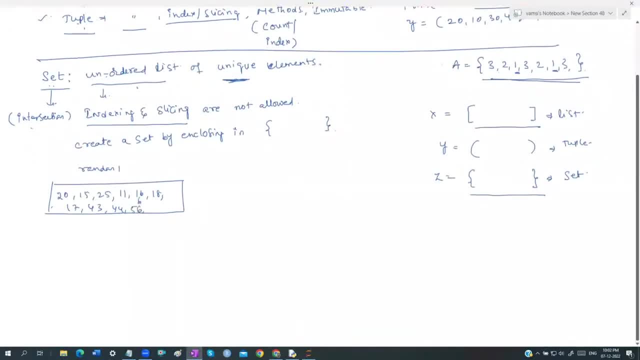 something like 44 and some 56 and something like. we have some 34, 32, something is the data. i have an another set of random numbers are there? i have an another set of random numbers are there, like, for example, 17, something like it. uh, something like 20, let us say 44, let us say 57 and 35. we have a 34 and we have 23. we have a 25. 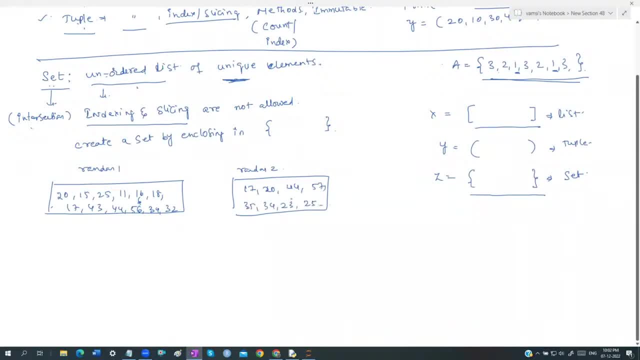 some numbers are there actually now. sometimes it may be required. that means, why do you use it means? later i'll tell you we don't have that many simple values actually. yes, but i want to. i want to find out how many common values are there between these two random numbers actually. 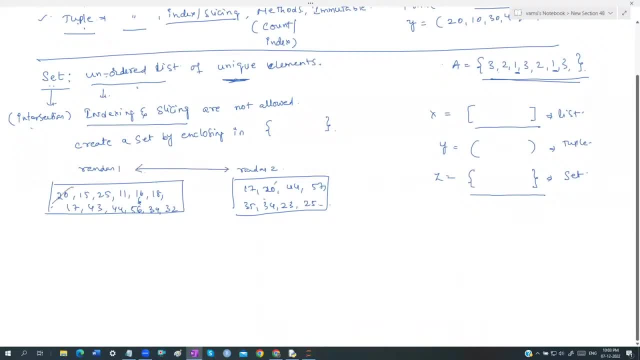 manually. it's a little bit confusion. actually it's a time taking process. 20 is there and maybe something like 10, 34. i think i have written 34. 34 is going to be there and even there may be 44 also. it is going to be there, something like that. i want to find out some. 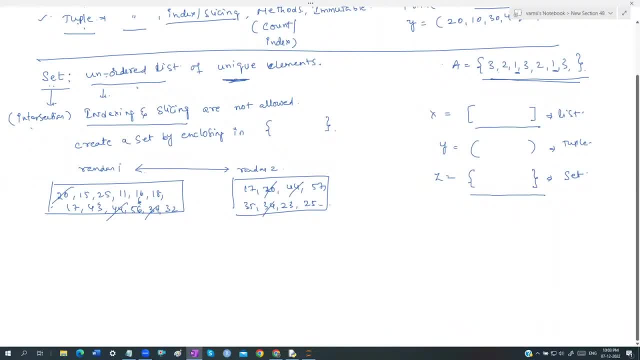 common values between them. so in that cases we are going to convert this random numbers to one set object and i'll convert this random two to the another set object and then i'll find out the intersection between them. but why do you use it means i'll go for? when you go for machine learning applications, i'll tell you. 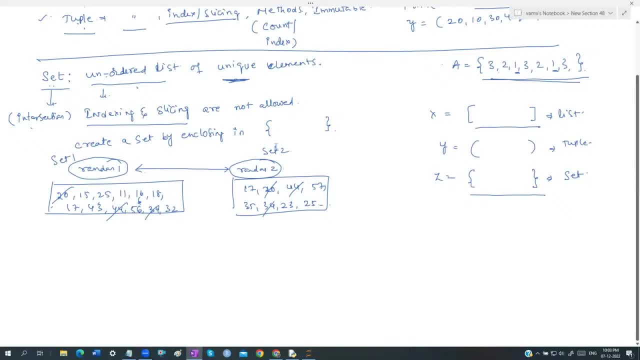 that actually in machine learning concepts, we'll discuss it actually, because in machine learning, what we will do is we are going to do some kind of an testing, we are going to do it actually. so this is going to be my test sample one and this is going to be my test sample two. 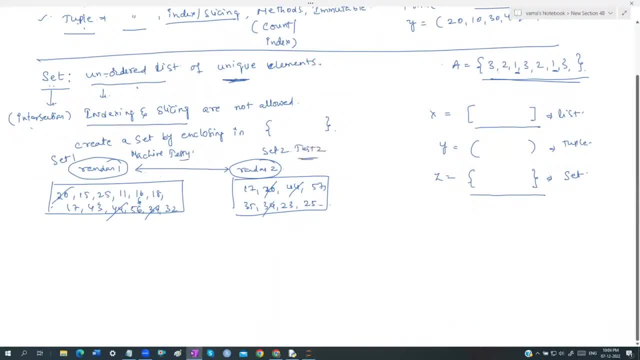 so in test sample one, set test sample two, at least how many samples are getting repeated? three samples are getting repeated actually. maybe out of 10 samples, three samples are getting repeated. that means 30 samples. 30 percent of the samples are getting repeated actually. so to make you understand that i'll use this set objects, we are going to use it but one or two times. 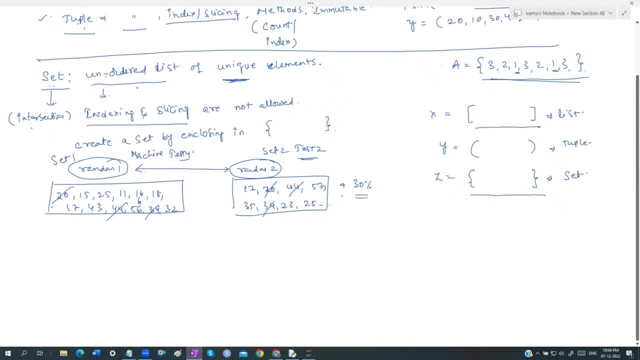 only throughout your machine learning, one or two times only. we have to use it. but if you want to using for one time also, we have to know the concept. so that is the reason why we are discussing about right okay, right guys, okay. so later we'll see them one or two times. we are going to use them. i'll. 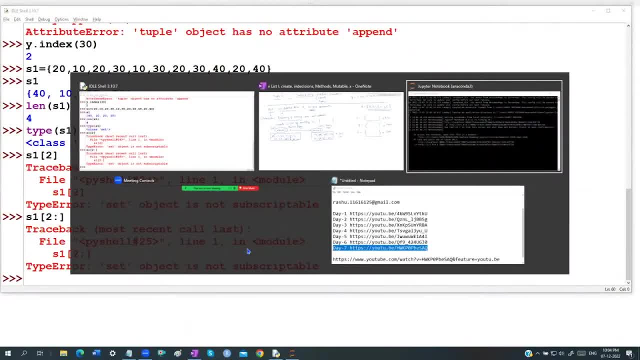 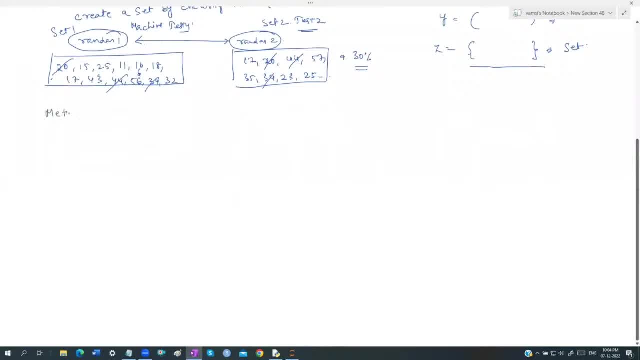 explain that, like, where do you use a set object actually? okay, now let us come to the methods. actually, guys, let us come to the methods. first, i'll tell you some methods which you can understand it easily. after that, i'll tell you some other methods which are different from the list, and 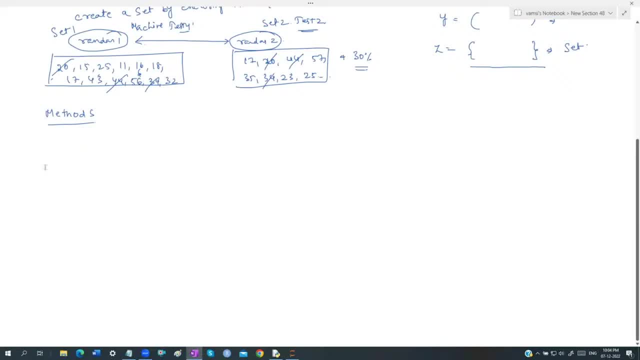 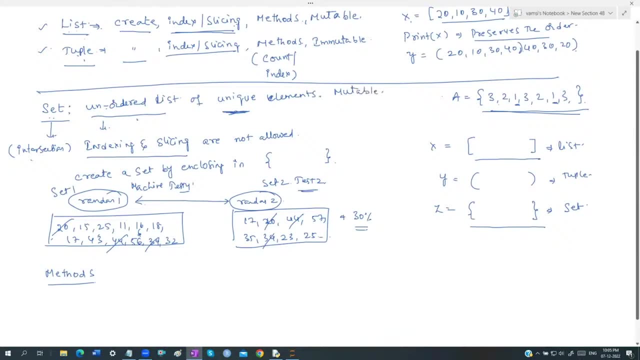 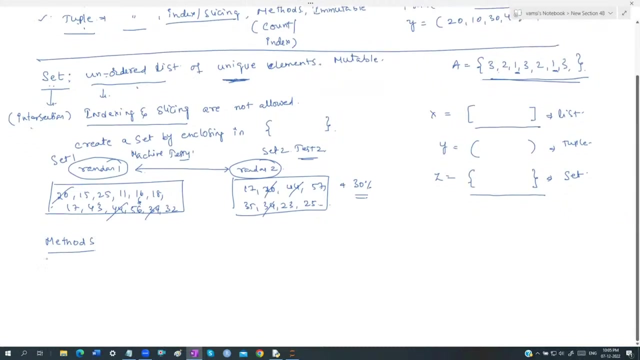 the tuples, actually, guys. so one more thing: actually, guys, it's a mutable object. only set is a mutable object, guys, means you can modify them. modify them means you can add some elements, you can remove the elements, whatever you want, we can do it. actually. yes, first one which is going to be nothing but, um, the method is going to be: how do you add the? 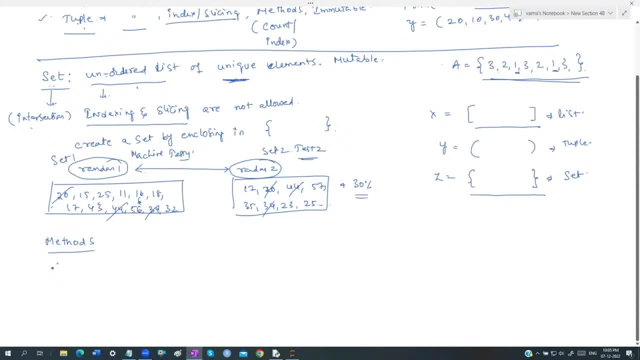 elements. actually, guys, normally in list we have append, we have an in. uh, we have an append, we have an extent and we have something called as an insert. but in the list- we are sorry, in the sets, we are having a method called as an add object actually, because add is a method and just give. 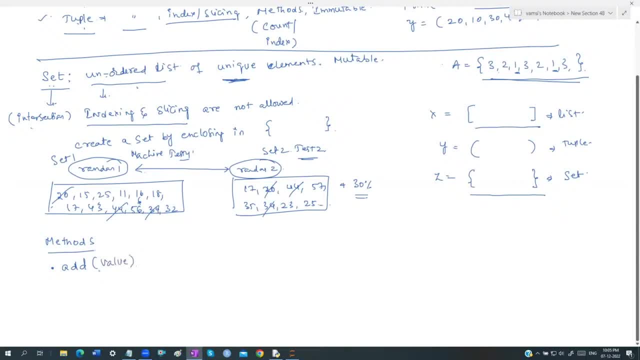 the value, actually, guys, but where it will be generally. why it is not append? you may get a doubt, sir, why it is not append. then, why it is not append mean generally appending means it is at the end, but here in set object we can't say that it will be appended at the end. actually, guys. 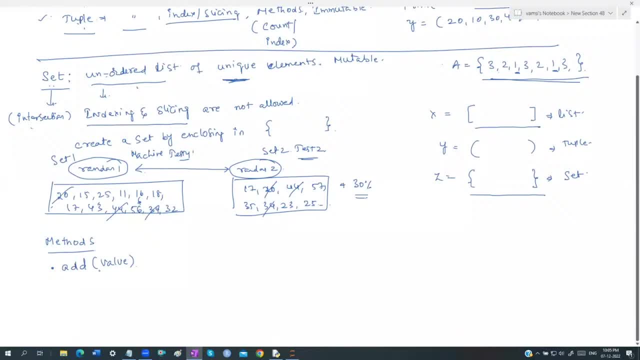 we can't say that it will be appended at the end. actually, that's the reason we don't say that append and extend, even in insert. also, insert is based on the index concept. i want to insert before the second index, i want to insert before the sixth index, but here indexing does not works actually. 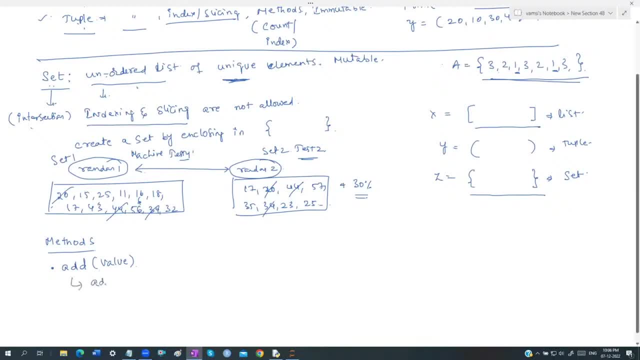 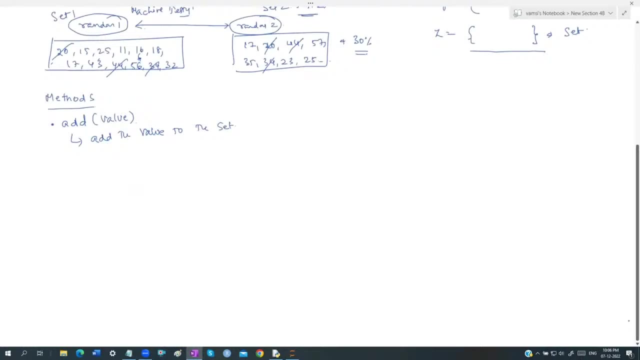 so it is going to be add. so what is add is going to do, actually, guys, it is going to add the value to the set, actually. but one small problem, actually, guys: if the value is already existing, simply it does not lose anything, it does not raises any error. also, actually, guys, because we know that, 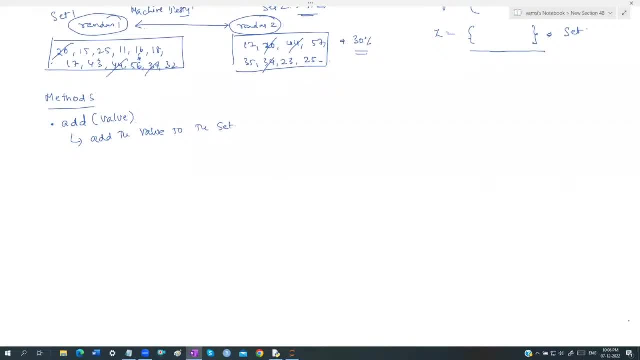 the elements must be unique. if already 10 was there. if we try to add a one more time- 10- it does not throws any error saying that 10 was already there. 10 was already not there. it does error actually. yes, sets are mutable. yes, absolutely, sets are mutable. just now i told you the point. 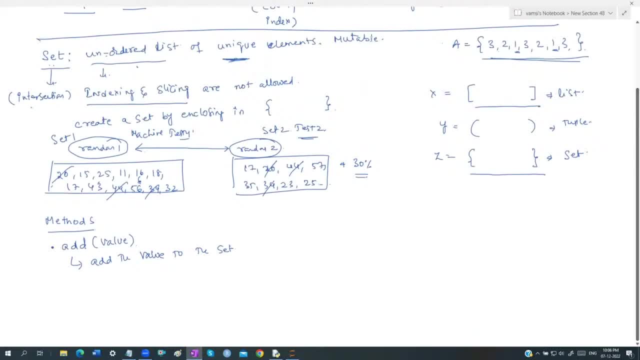 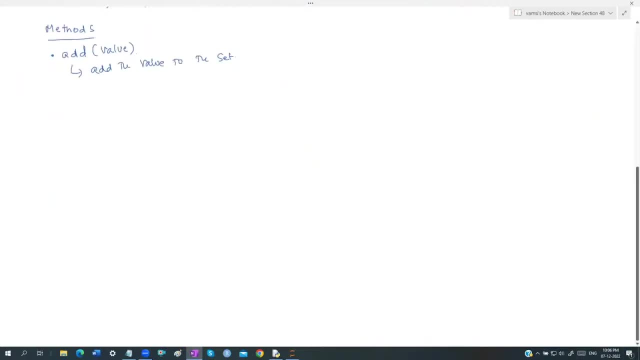 just now i told you the point. actually, guys, they are going to be immutable objects. sets are going to be mutable objects. actually, yes, okay, fine, add the value to the set, but i can't say that where it is going to be appended. actually, yes, and i think so. i need not to tell. 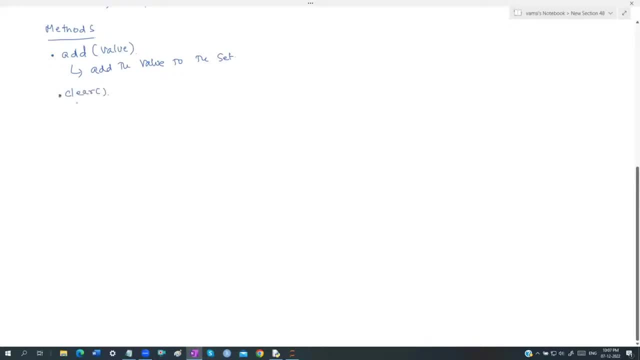 you about what is clear? actually guys. same clear is going to be common. actually, some methods are common actually, yes, but they will work with respect to that object only. it will works actually clear. you know what is a clear? actually guys. clears all the elements from the set. 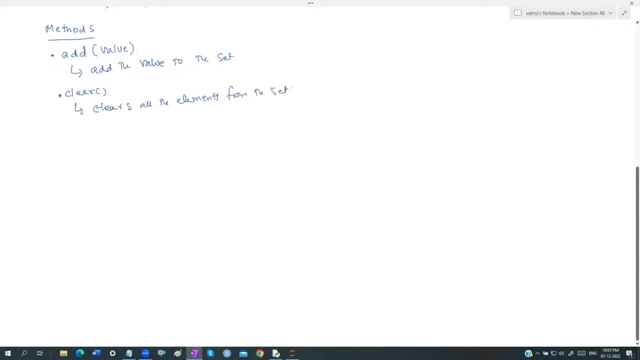 all the elements from the set. it is going to remove. actually, guys, same as it is. we are having some option called as and remove. actually guess, think a little bit carefully. guess: remove is going to be based on value based. actually, guess, right, it is going to be value based actually. 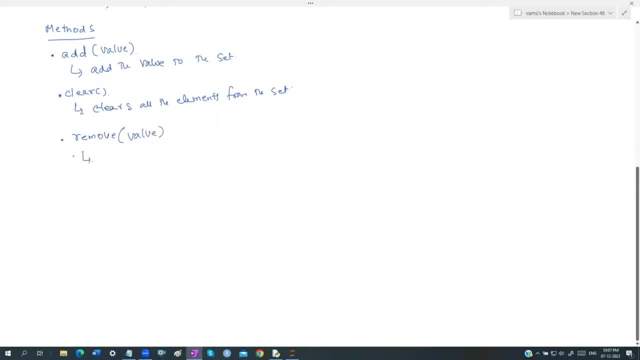 while i'm discussing about the list, i told you what is the remove method is going to do is best: in list object, same element may be there for multiple times. that's why it will remove only the first occurrence. but in set object it is only one time available. the value is not duplicated. 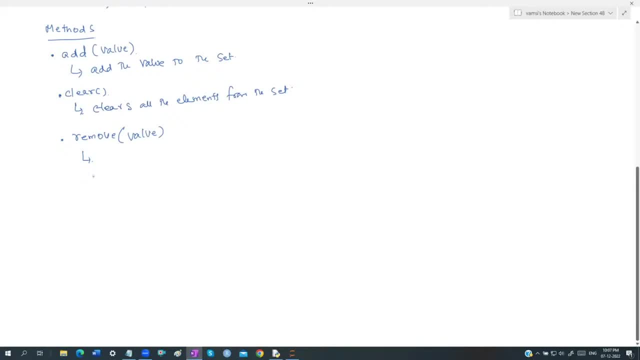 it is going to be only unique values only. so i cannot say that. first occurrence, second occurrence, i cannot say this: actually, guys remove, you know this. actually, guys remove is going to. it does not returns anything, guys, and you can see here, i will never able to transfer value to that إن. 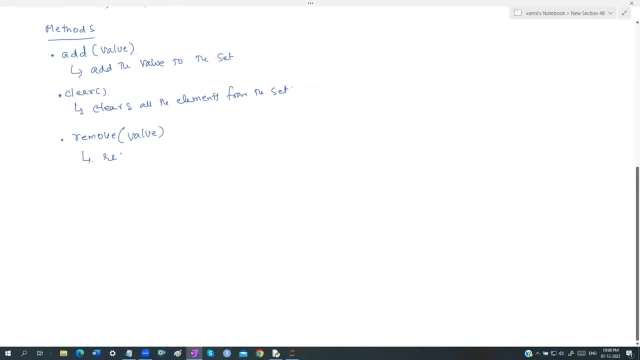 Add won't return anything. Clear won't return anything. Remove also won't return anything. guys, What it is going to do is, guys remove the given values or removes the given value from the list, Given value from the list, And we know this from the set. actually, guys, 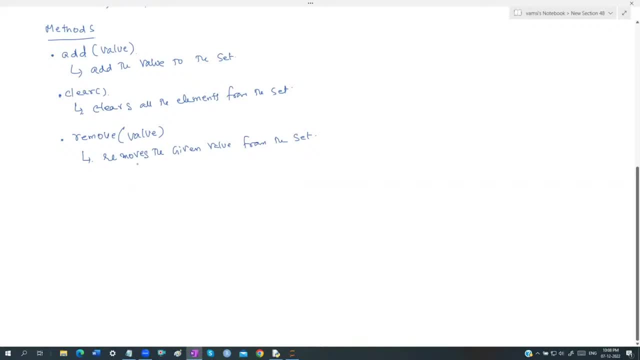 But you know one point: This value must and should. it must be there. actually, guys, If the value is not there, it will raise us an error. actually, The value must and should it must be there If the value is not existing. 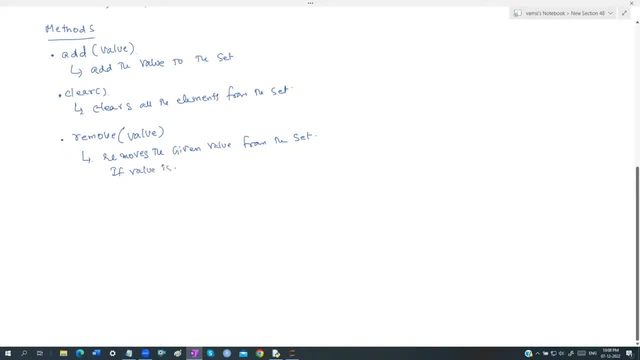 if value does not exist or if value is not in the list. if the value is not in the list, then it is going to be raised as an error. actually, guys, An error will be raised Here. there is one small method, which is speciality here. actually, guys. 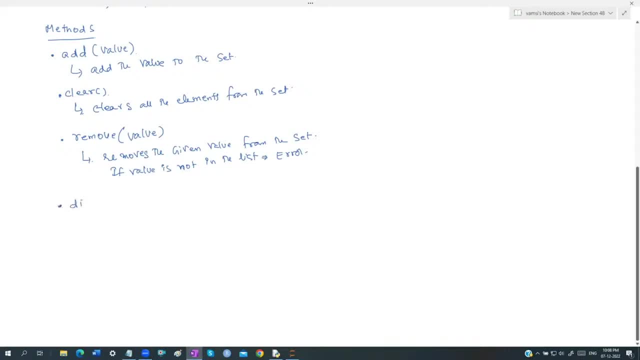 That is, we have a method, what we are going to call it as discard. It is going to be discard. actually, guys. What is a discard is going to do, guys? Discard is going to be nothing but same as a remove. actually guys. 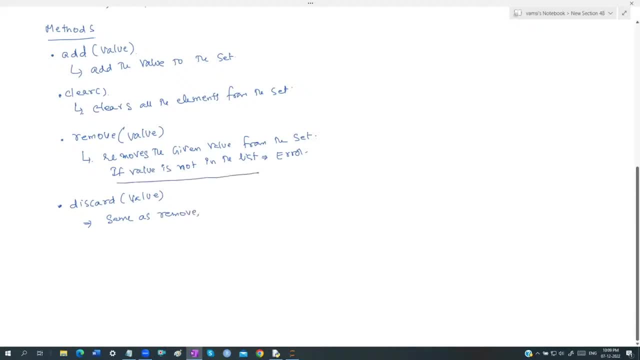 But difference is, if the value is not existing in the list- sorry guys, not in the list, it is not in the set- It is going to be not an error. So it is going to be no error if value is not in the list. 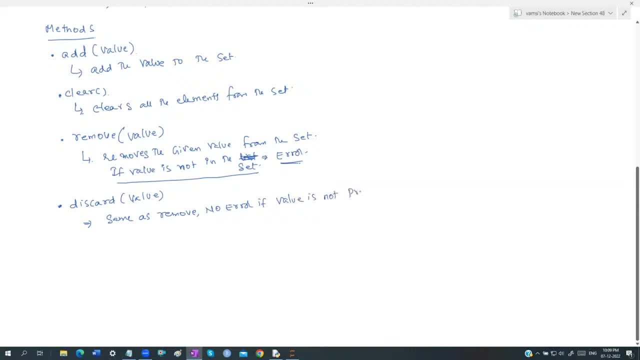 or value is not present, That means it does not make any noise at all. What is remove is going to do? If remove value, if the value is there, it does not make any noise. That means noise means generally. I am talking about that. 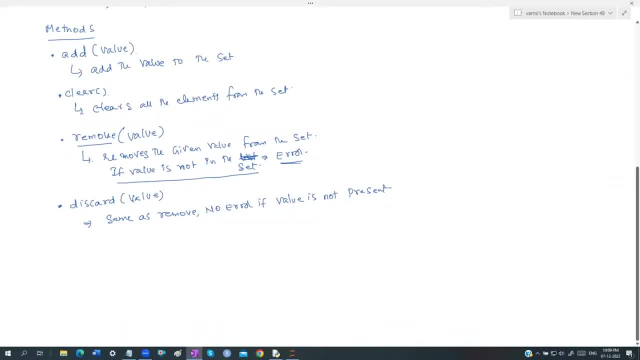 it does not raise us any error, But whenever the value is not there, immediately it throws an error. actually, guys, Error is a noise in our normally. error is always a noise, actually for us guys, Whenever we talk about a discard. 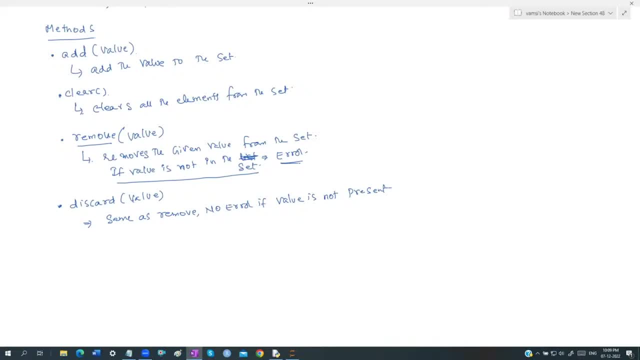 discard says that if the value is present, I will remove. If the value is not present, I do not do anything. actually, guys, If the value is there, it will remove, If the value is not there, it does not do anything. 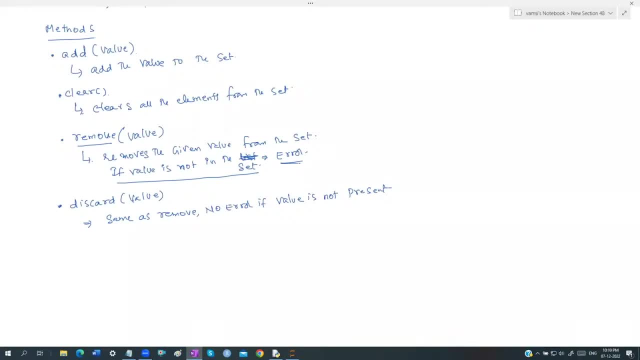 Discard is not like this, actually, guys. So remove is not there. It is not like that, actually. If the value is present, it will remove it. If the value is not present, it will raise us an exception. actually, guys. 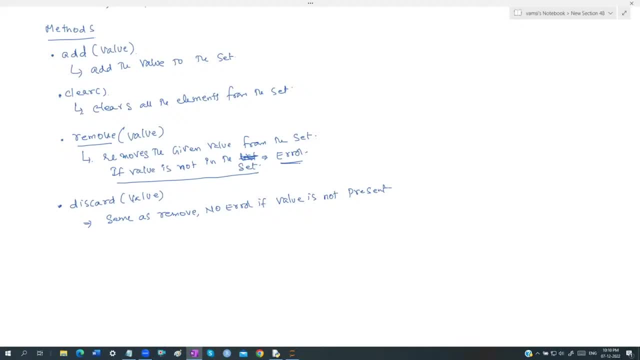 One error will come, actually, guys. So similarly the same way, guys, but with the small small changes. what we can do For adding only one, add method, guys, but for removing, we have clear, we have remove, we have a discard. 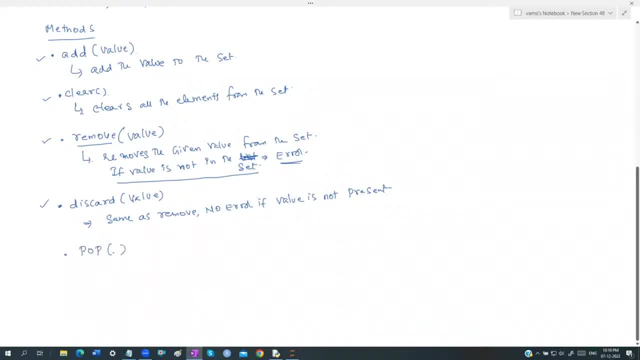 we have a pop also, actually, guys, But pop does not takes any index, guys. Pop does not takes any index because in set objects we can't remove any based on the index. actually, because we cannot point to the index, actually, guys. 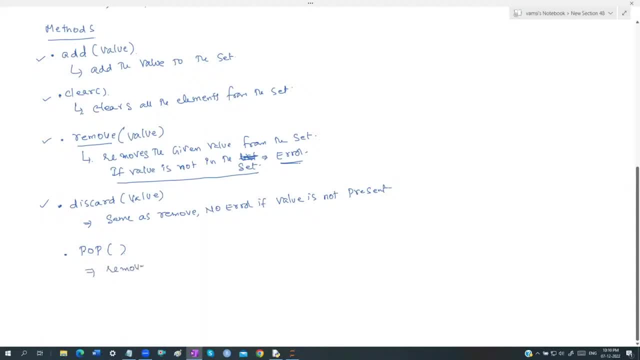 What is pop is going to do is, actually, guys, remove and return. You know this. actually, guys, It will remove as well as it will return. actually, guys, And arbitrary number. It's going to be arbitrary. actually, guys, It is going to be some arbitrary. 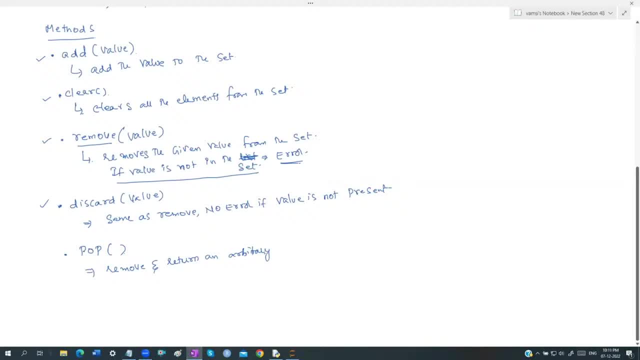 So it is going to be something like left to right, right to left. It is going to remove the values, So we don't say that That means it will all normally. list will always remove only the last element minus one. 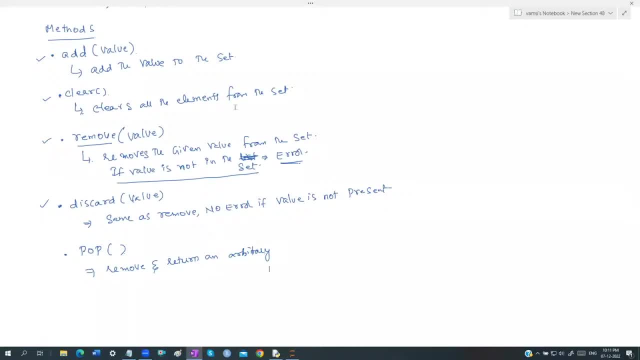 But here it is not like this, actually, guys, From left to right, it will remove the elements actually. So that kind of an exception, that kind of an application is what we are going to be using as of the pop method, actually, guys. 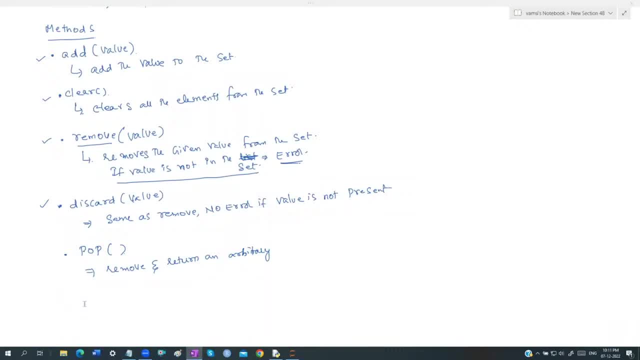 So add, clear, remove, discard, pop. These are the some of the common methods, guys. Only pop is going to returns a value. actually, guys Remaining: add won't return, clear won't return, remove won't return, discard won't return. 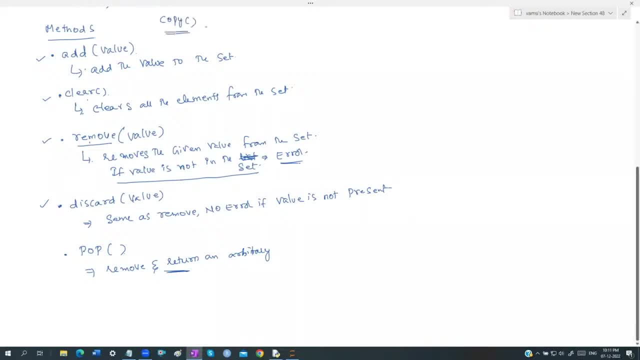 Even there is a copy method. That is there actually, guys. But I'm not discussing about copy. I told you Even in list. also, I didn't discuss the copy In tuple anyhow, we don't have a copy method, guys. 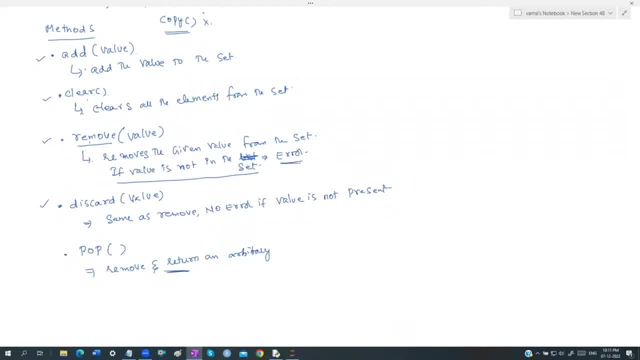 But in set objects also copy method. I'm not discussing Almost nothing, is there, guys, Some concepts which you already studied? Some concepts are going to be mathematical techniques. actually, guys, There are the mathematical techniques: Add, clear, remove, discard, pop, guys. 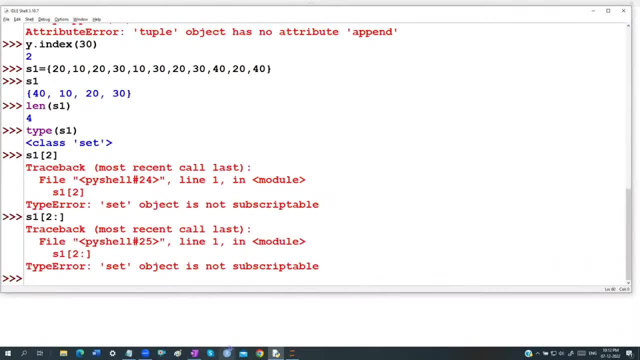 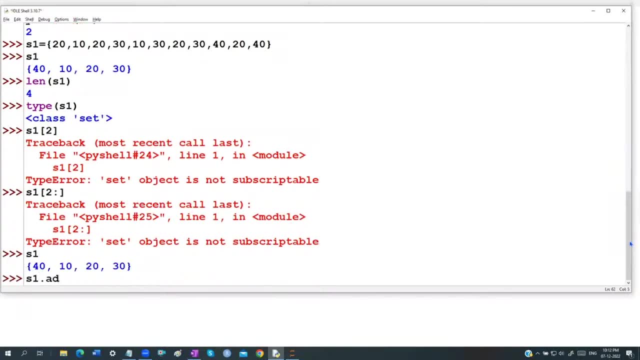 These are the some of the methods. First, let me finish off this, guys, And then we'll go to the next methods. actually, guys, These are your S1. actually, guys, I can say S1 dot, which is going to be. 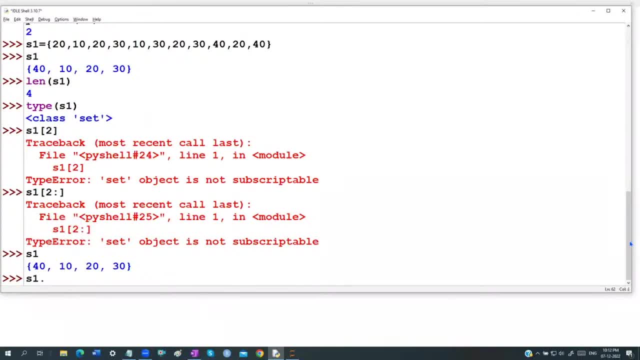 the first method itself is going to be nothing. But, guys, it is add actually guys, It is add, actually Add of 15.. We cannot say that very clearly, guys, Add an element to the list. See the documentation. guys, 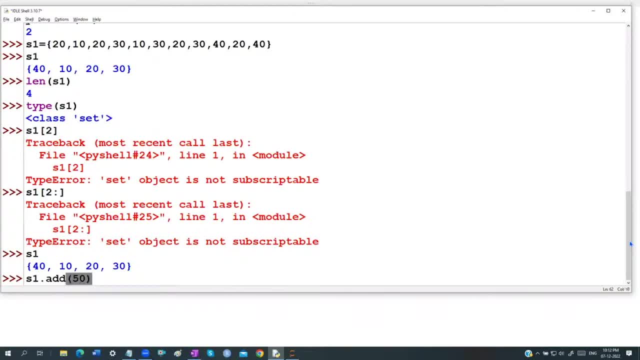 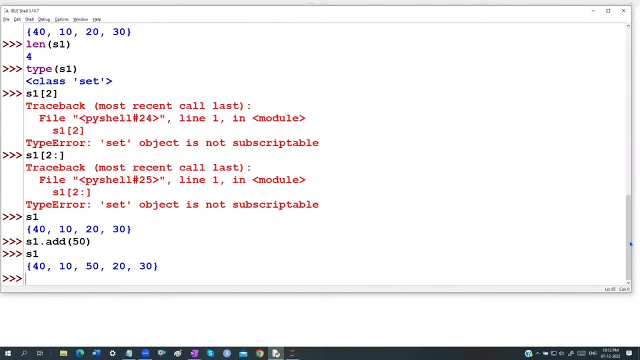 Add and sorry, not a list. It is going to be set, actually guys, Generally in a flow, we are getting it actually, But, sir, where it is added, actually guys, I can't say that 15 will be added only at the end, actually guys. 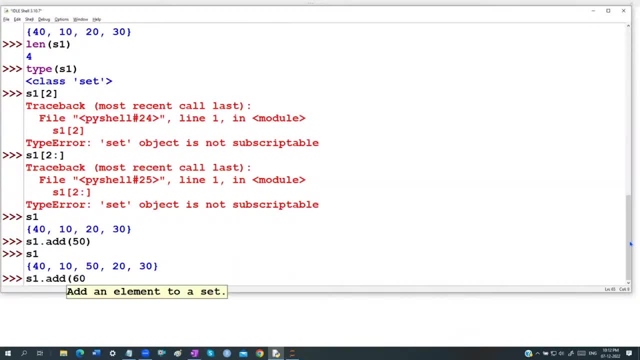 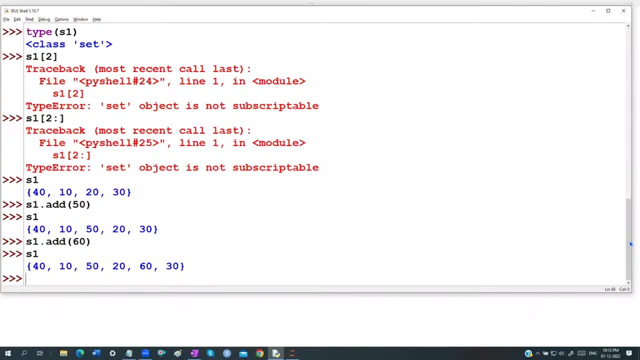 S1 dot which is going to be add, of 60, guys. I cannot say that beside the 50, only the 60 is also going to be added. actually, guys, 60 is going to be added somewhere. actually, guys, S1 dot- it is again an add. 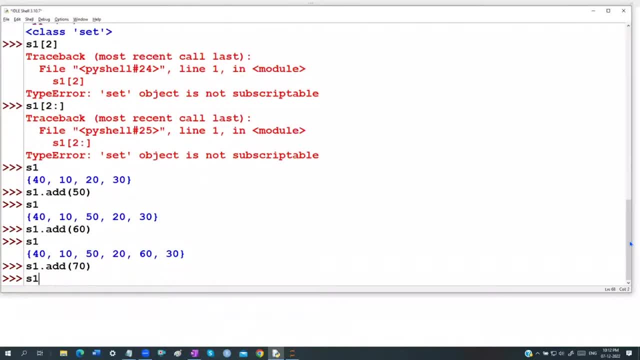 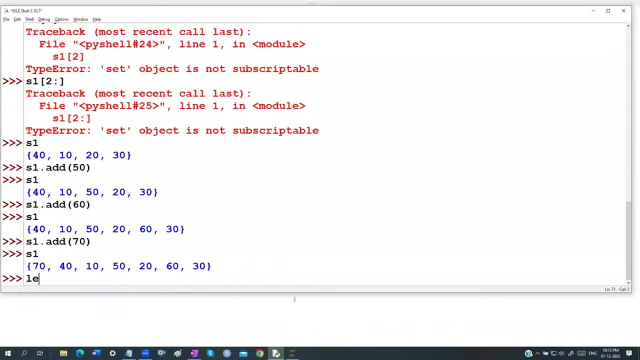 which is going to be nothing, but it's a 70 actually, Where it is going to be. gets added actually guys. 50 here, 60 here, 70 here, actually guys. What is the length of the S1 actually? 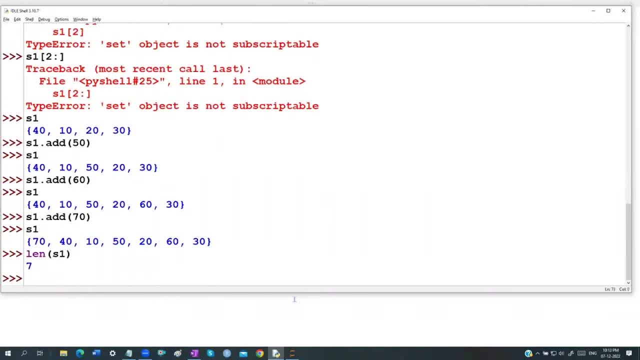 It is going to be. right now it is 7.. That's it actually, guys. So we can add up the elements as you require. If you want to clear guys, you can. simply you can do the clear, actually. 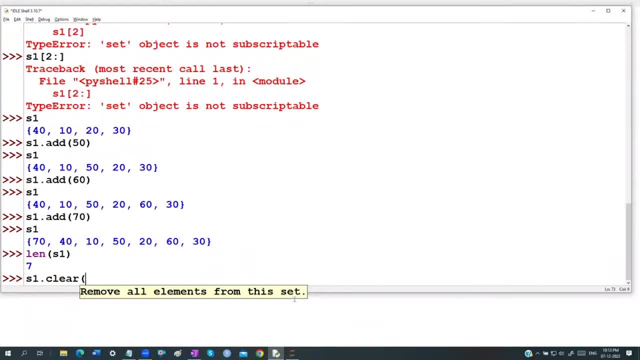 You know what is clear? actually guys, Remove all the elements from this set. I want to remove it. actually, guys. I can say: remove, actually guys. What is going to be? remove? actually guys. Very clearly: Remove an element from a set. 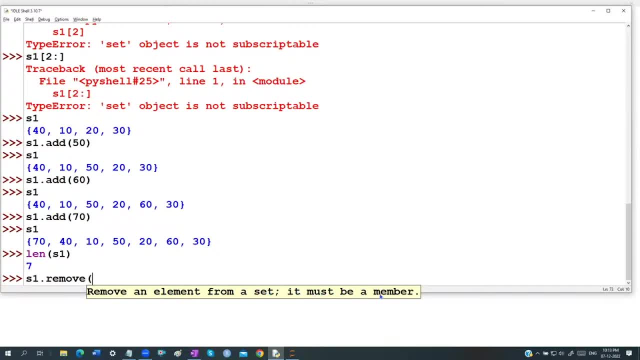 It must be a member. It is clearly saying that it must be a member. You know what is meaning of it must be a member. Must ensure it must be a member. actually, Okay, S1.remove of 70.. I can't say that. first occurrence, second occurrence, actually, guys. 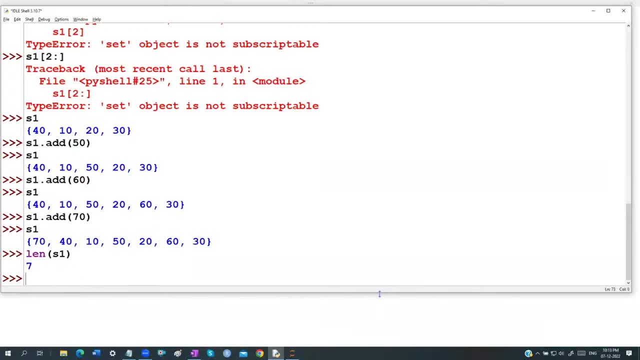 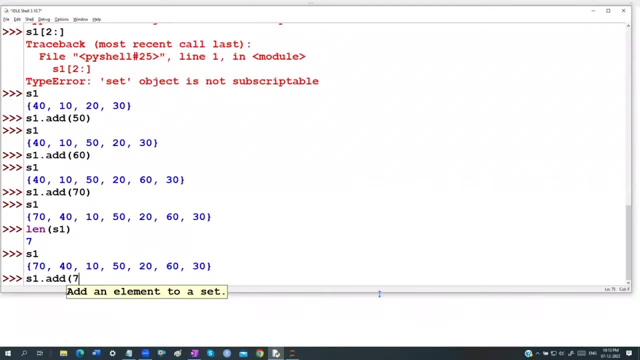 Why? Because this 70 is available only for one time. Okay, Before going to that, I didn't execute it, guys. 70 is already there. S1.which is going to be add of 70.. One more time: if I add up 70, nothing it will do, guys. 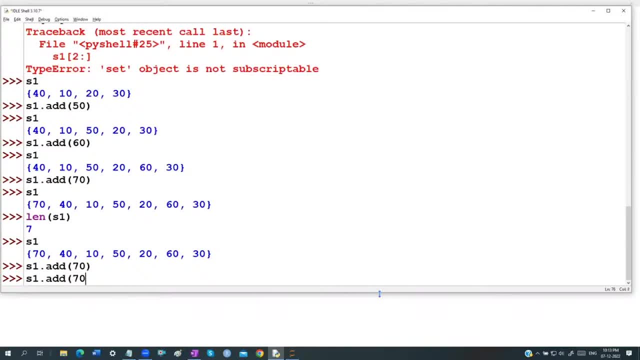 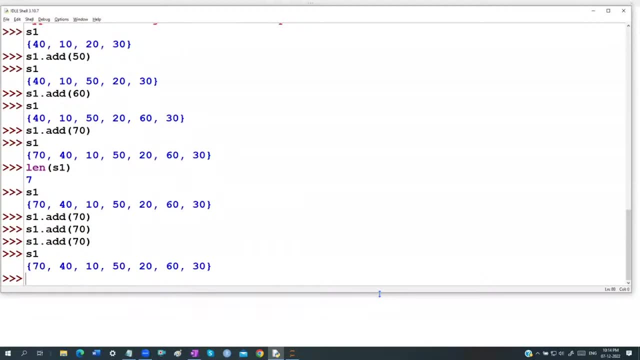 It does not throws any error. also, How many times you do it? also? it does not throws any error at all, actually, guys, But don't think that it has been adding the 70 for multiple times. Okay, It is there only for one time only. 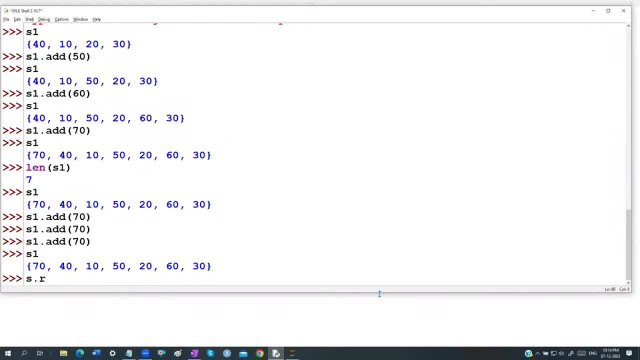 It won't add it for multiple times. Now I can say S1.which is going to be remove of, which is going to be 70.. 70 was removed, actually, guys, But it didn't return any value back Whenever I said S1.which is remove of again 70, this time 70 was not there. 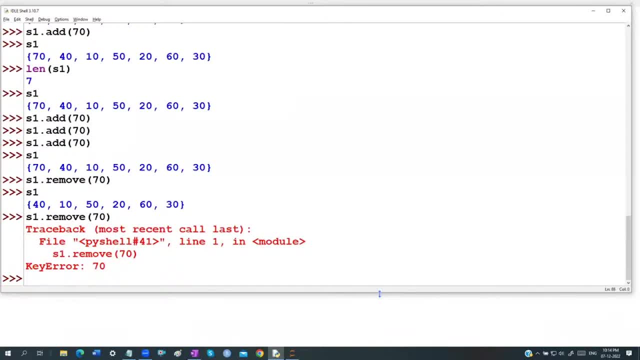 But remove will make a noise. if the value is not there, It's a key error. So I can say that the key was not found, which is 70, actually guys. Same example if I said S1.. If I said discard, actually guys. 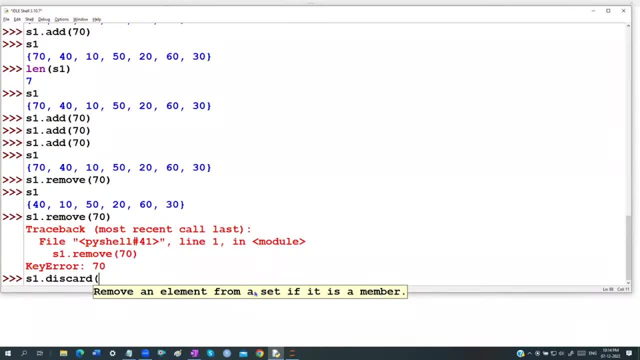 See the different. actually, guys Remove an element from a set If it is a member. it is not saying that it must be a member. In the earlier case, when I said remove, it is saying that it must be a member. 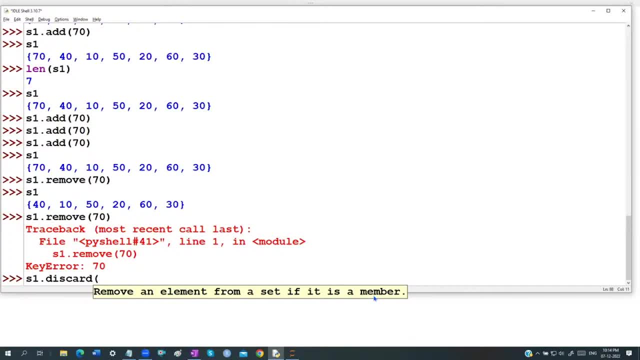 But it is saying that if it is a member I will remove, If it is not a member, I don't do anything. actually, guys, Try to say 70 once again. guys, Don't think that it has been got removed. 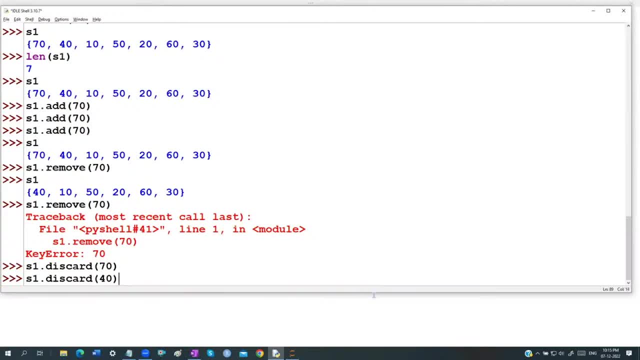 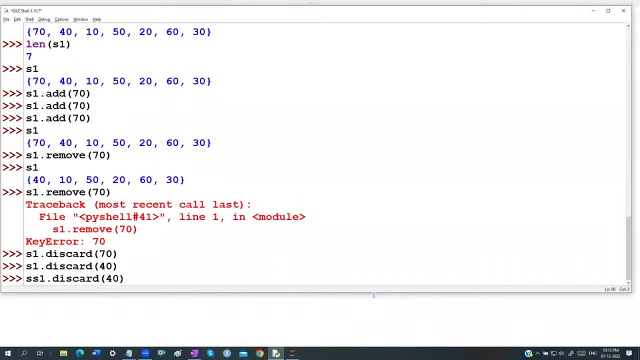 It may be removed. It may not be removed. Okay, I said 40. actually, guys, 40 was removed Again. if I said S1.again discard of 40, it does not throws any error. actually It does not throws any error. 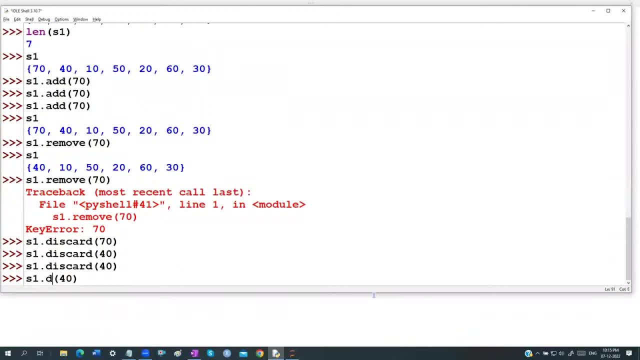 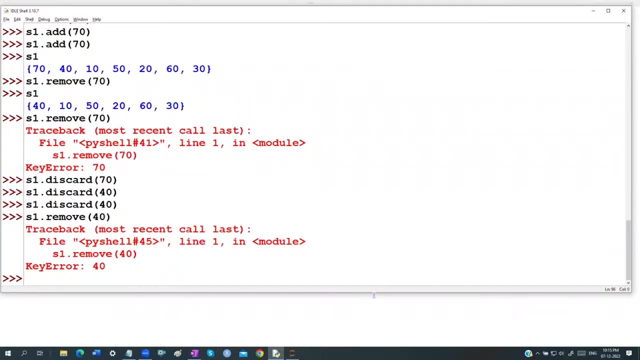 But if you say, if I say, sorry guys, If I said S1.remove of 40, actually, guys, 40 was already removed. We are getting an error, actually, guys. So it must be a member. It may be a member. 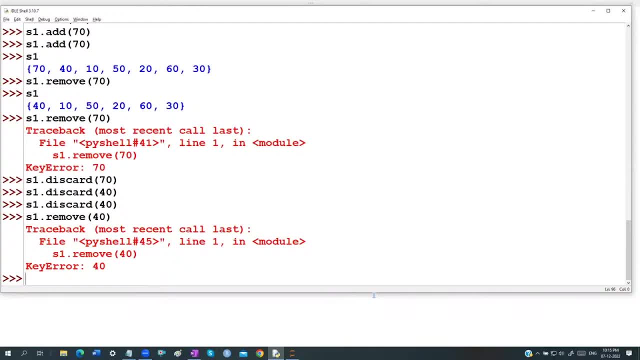 If it is there, I will remove. If it is not there, I am not going to do anything. actually, guys, This is going to be nothing, but this one. actually, guys, And you know what is pop? actually guys, Can you observe carefully, guys? 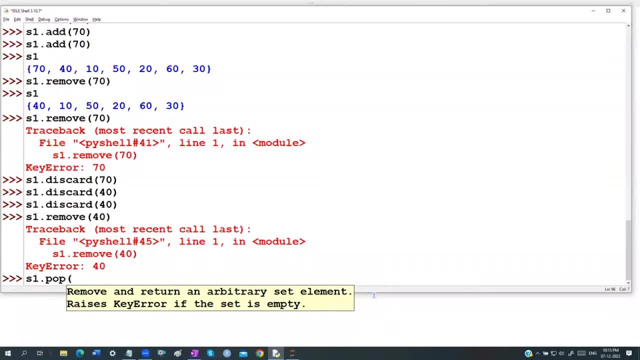 Removes and returns an arbitrary set element Raises a key error. if the set is empty, Don't give any input. actually, guys. We remembered when I said X dot X is a list, actually, guys. If I said X dot X is a list, actually guys. 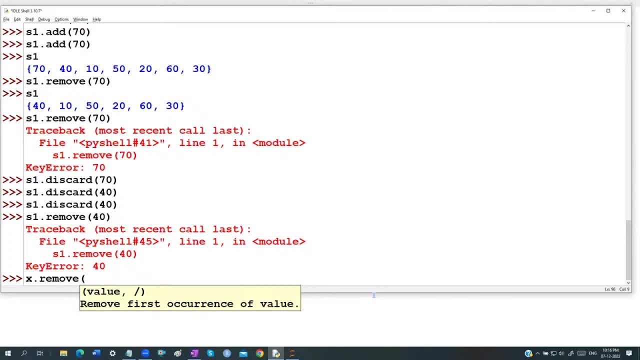 If I said X dot remove, you are getting a value. actually, Even whenever I said Which is going to be X dot, What I am talking about? Pop. actually guys. If I don't give any value, default value is going to be minus 1, actually, guys. 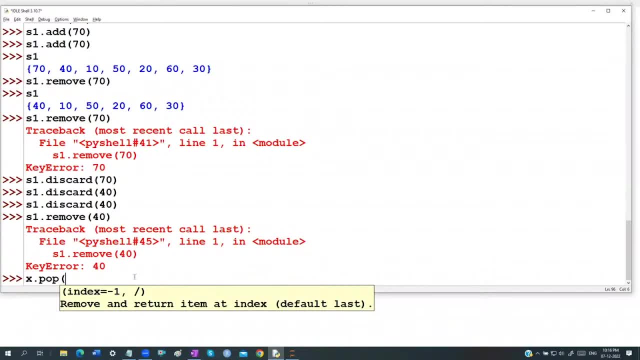 Index will be minus 1.. That means if I don't give it, default is last element actually, guys. But here it is not like that. If I said S1.pop, it is not taking any arguments, guys. Don't give any minus 1.. 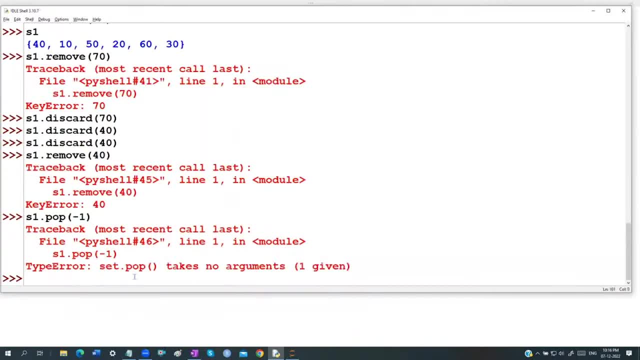 We will get an error. Pop takes no arguments, But you have been given one, So it is an error. actually, guys, If I said X dot pop, actually guys. Now you can see once. Let me show you S1 here. 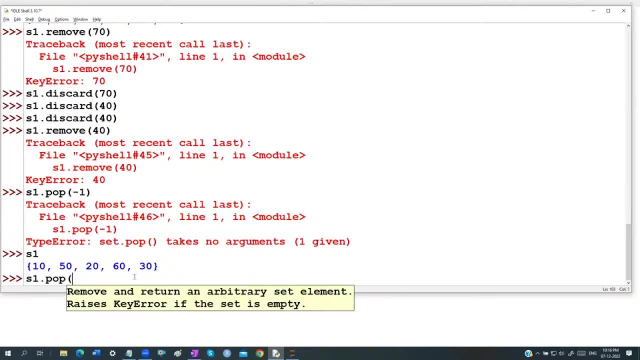 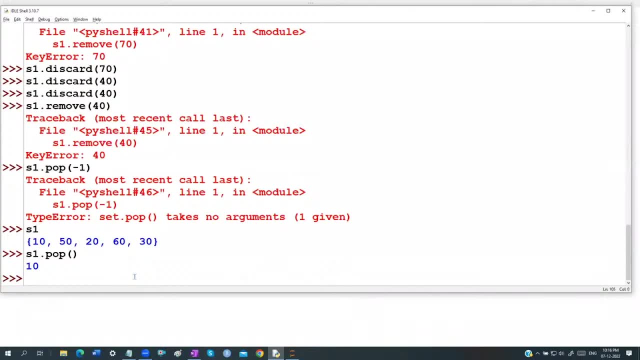 Now you say S1.pop, actually guys. So it is going to be removed basically from first element. That means from as of now, left to right, Again S1.pop. You know, pop will return some output, actually guys. 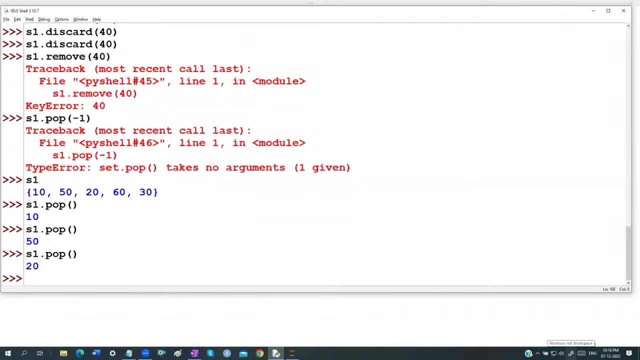 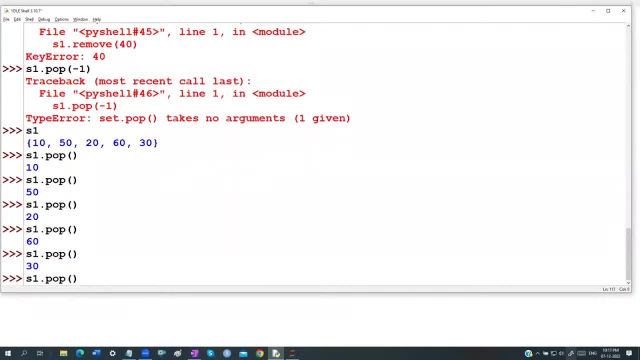 50 was removed And then 20 was removed, Then 60 was removed And then it is going to be 30 was removed. actually, guys, Now again, if we said S1.pop, it will throw an error Because there are no more elements from the list. actually. 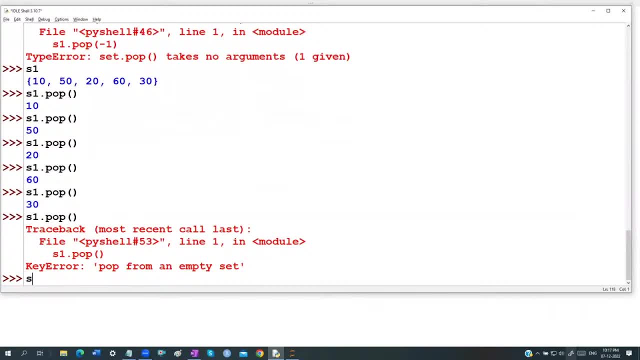 So it is saying that pop from an empty list, actually S1.. So what is the length of the S1 actually? Right now it is 0 actually. What is type of S1?? There is no change, It is still a set only. 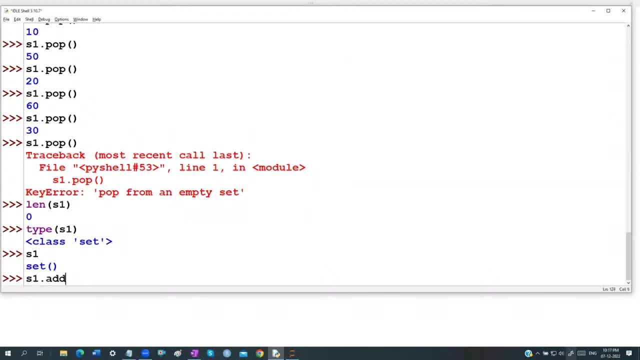 This is your S1, actually, guys. Again, if you want S1.add At any time, you cannot add multiple elements, guys 10. S1.which is add of 20.. For list, we can add up them, guys. 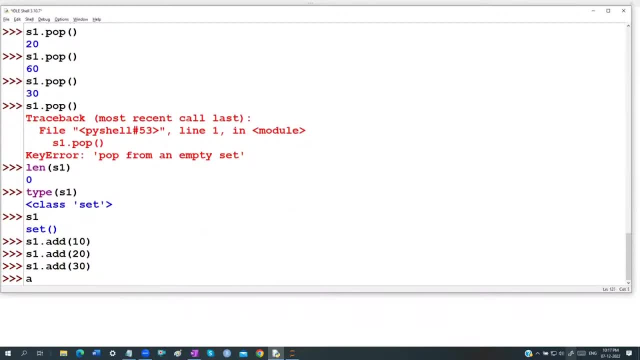 But for set, we can't add it actually S1.30.. S1.which is add of, which is going to be nothing, but it is a 40 actually, guys. So this is the data, what we can see with the data, guys. 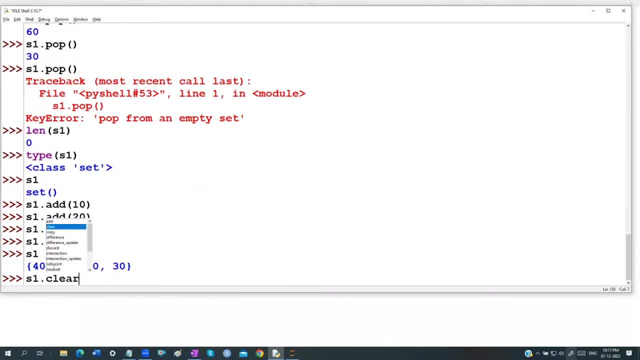 So these are the some of the methods, which are basically no's actually. guys, Once again, add Clear Copy. I told you guys I am not discussing, as of now, Discard. I told you guys, Discard. 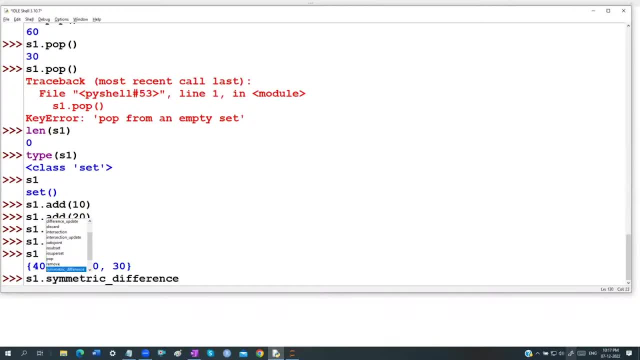 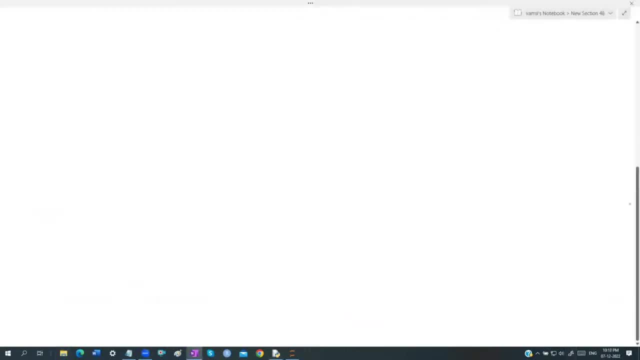 Discard is, I told you, Apart from that, pop. I told you Remove. I told you, actually, guys, Remaining are different methods. It is very easy, very simple, actually, guys. There are very easy and very simple methods, actually, guys. 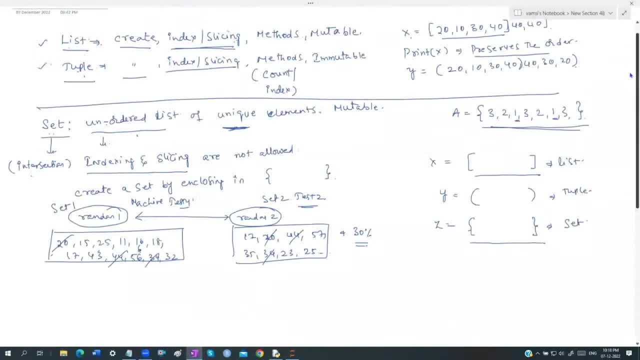 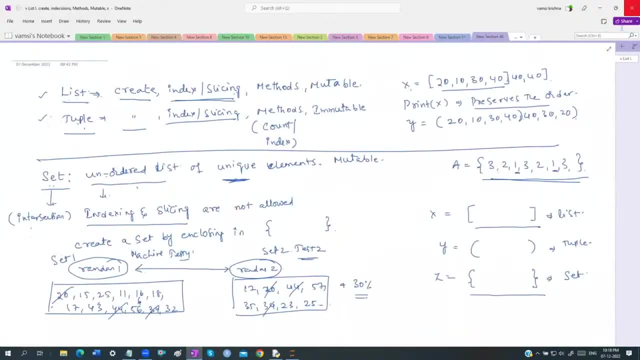 Okay, So once again, I have been got discussed about the methods associated with the list, So the methods associated with the set objects. I have been got discussed about that Just a second. Yeah, So these are the methods, what we have, it actually guys. 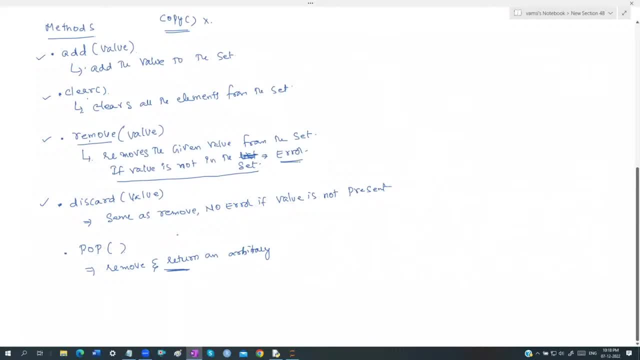 These are common things: Add, Clear, Remove, Discard Pop. These are common methods, actually, guys. Now, the methods which are special, which are going to be speciality in the list set. actually, guys, You can't see the methods in any other. 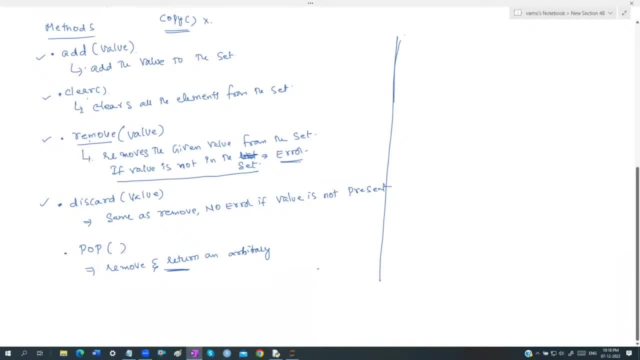 That means you don't find it in any other objects. We cannot find it actually, guys. What are those? What are going to be those objects? actually? guys Here, ascending, Okay, Actually ascending, descending orders. Generally, we have a method. is there actually, guys? 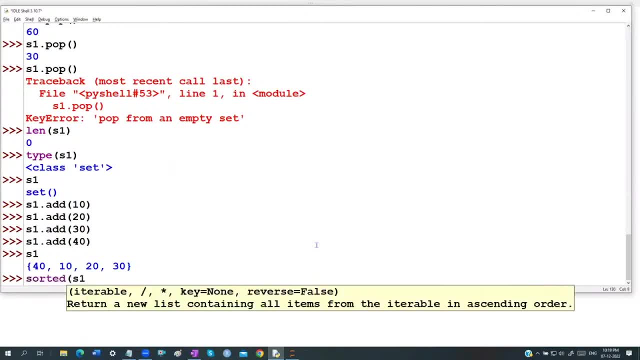 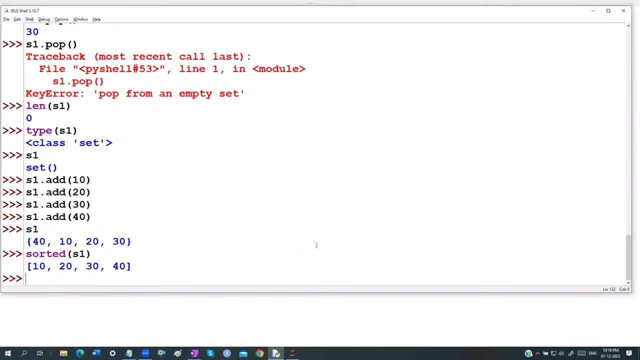 That means we have a function. is there Not ascending, descending? It is going to be nothing, but it is going to be the S1, what we can see with the data: There is a method. is there is a function? is there actually, guys? 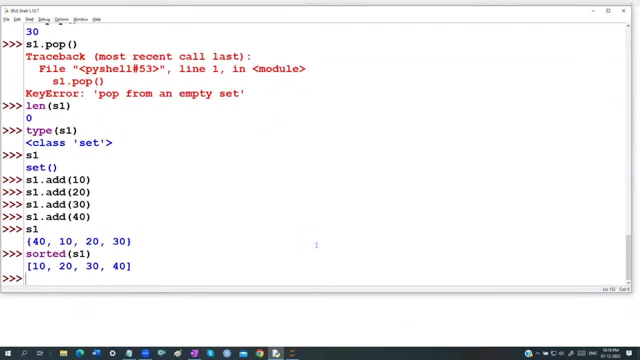 Sorted of S1.. You can see, Sorted can be used on list tuple sets, anywhere. you can use it actually It is working. But see the output, what we can observe carefully, guys. You see the output, what we can see it actually, guys. 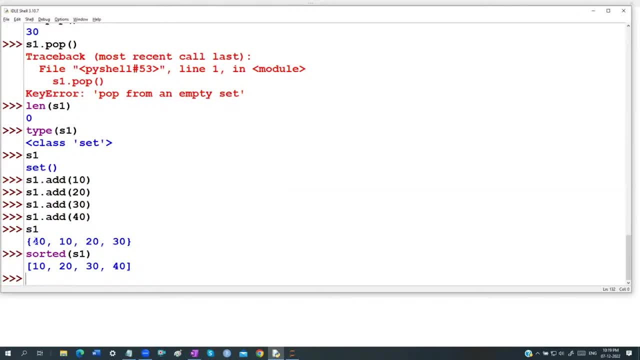 S1, I have given as an input, as a set, But sorry as a set, But outcome is coming like n, which is going to be nothing, But it's a list object, It is coming actually. So this is going to be sorted actually, guys. 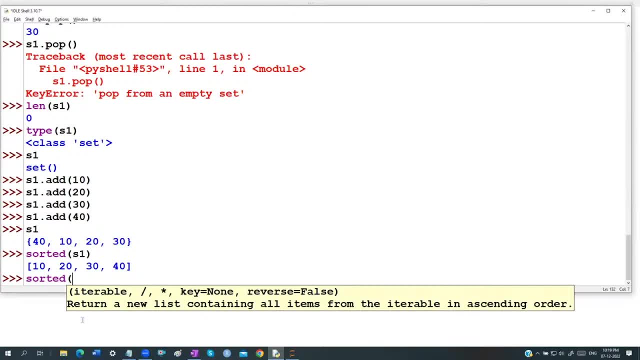 One point I didn't discuss, guys: What is iterable? I have been noted, discussed, But see the output. actually, guys, Returns a new list. That means the set is getting converted into list containing all the elements from the iterable in an ascending object. 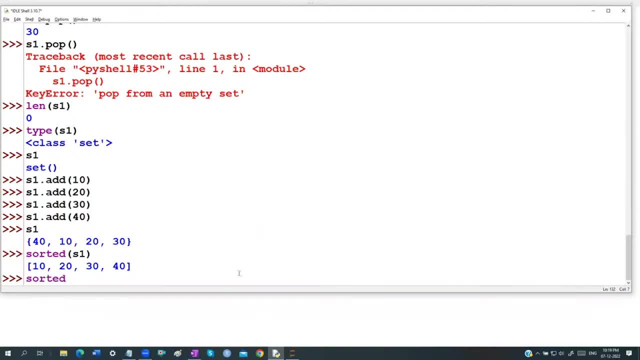 It is going to be returning. actually, We can do it, But it is no more a set, It is going to be converting into list. Sir, can I convert again into set? Absolutely, you can Convert it actually, guys. 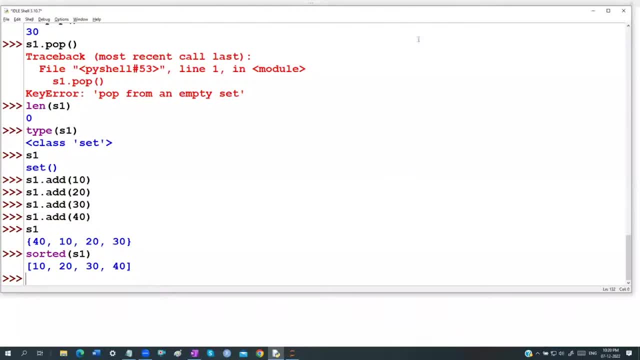 Okay, We'll see them. We'll see them in application. How to convert a set into list, list into set. How to convert them. we'll see them in applications. Okay, Fine guys. Okay, And I forgot to set the option actually guys to everyone. 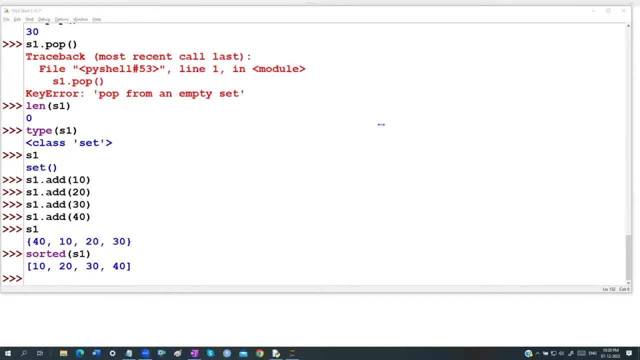 So, guys, if you have any doubts, please, when you're posting, when you're testing anything, please send it to everyone, guys, so that everybody can see what I'm discussing about. that, Right, guys? So this is going to be about 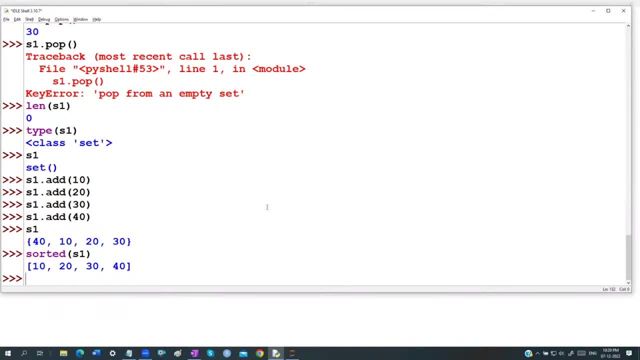 This is going to be about the basic methods, actually, guys. Now, whatever the methods I'm going to be discussing, they are going to be completely. They are going to be completely, Which is going to be special for the set objects, actually, guys. 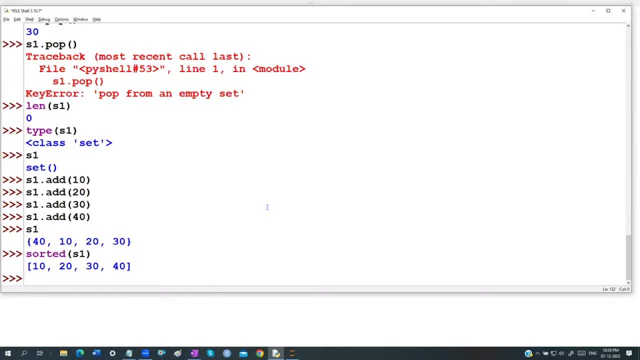 It is going to be nothing but a kind of a speciality, a special functionality for your set objects. actually, guys, Which is nothing, but we do it in our mathematics. no, guys, It is going to be nothing, but in mathematics, we know that. 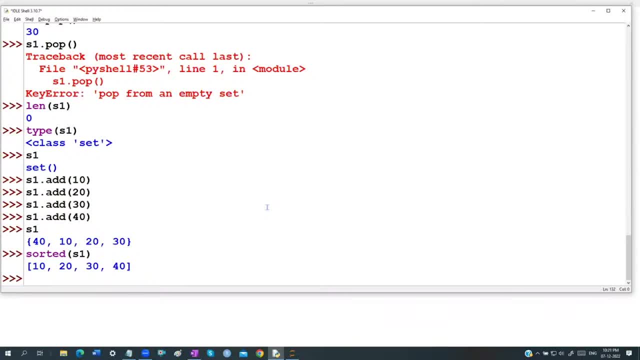 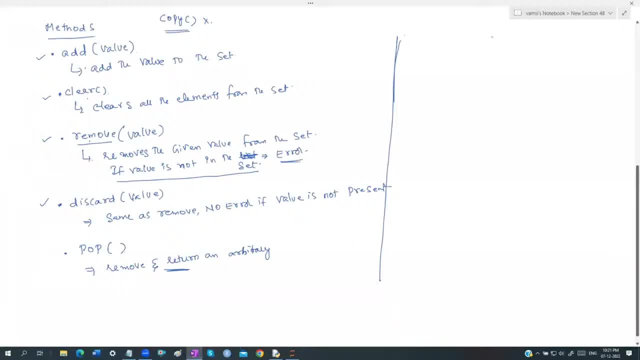 Actually set, objects, sets. we are going to be gets talking about that. So what are going to be that kind of an options actually, guys? One of the common methods? common methods are going to be nothing, but Let us imagine that there are two sets. are there actually guys, S1 and S2.. 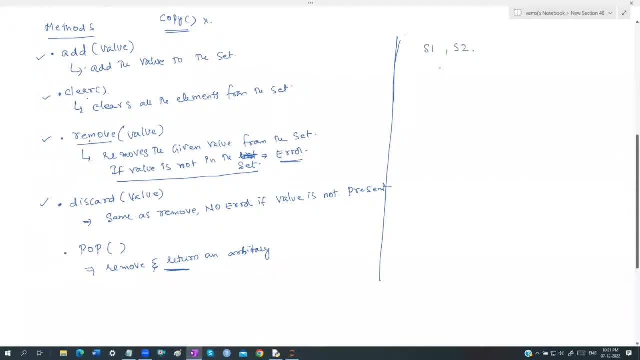 I want to find the intersection. You know what is going to be intersection between the two values? actually, guys, It is S1.. How do you do it? actually, guys, S1 dot, It is intersection of S2.. So we know what is meaning of intersection. 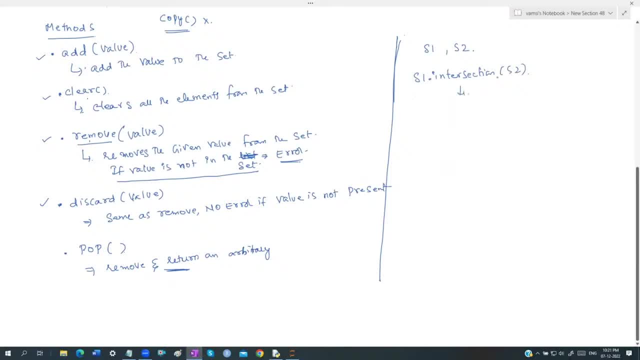 Between two elements. actually, guys. S1, dot, intersection with S2.. What it is going to returns, we know this. actually, guys, It is going to returns the common elements. actually, What are the elements which are commonly available in S1, dot, S2?? 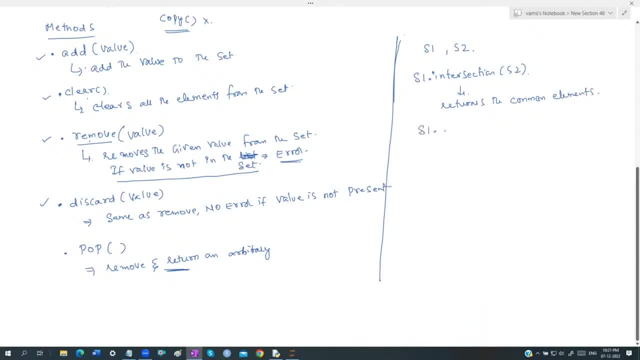 S1 and S2, it is going to returns And hope you remember it is union actually, guys, Union of S2, actually Same technique, guys, Intersection, and it is union, guys. You know what is going to be. 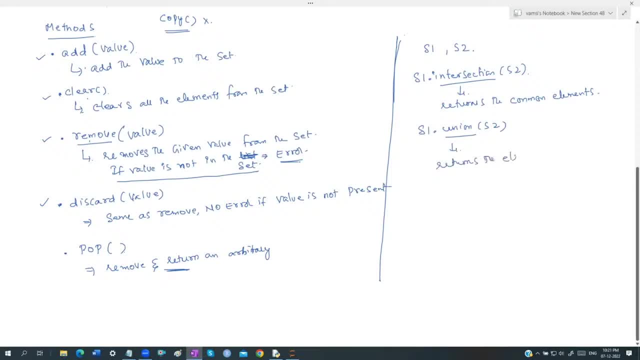 Union is going to returns. actually, guys, It is going to be returns the elements of both elements, from both S1 and the S2, actually, It is not common values, actually, guys. I will show you some examples what I can show you actually. 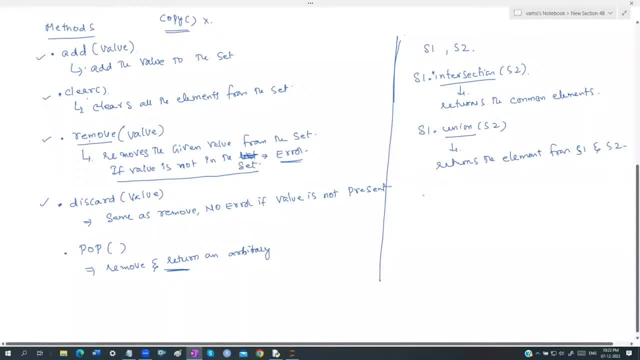 And what exactly we are having, if you remember, minus. actually, guys, We will call it as minus In mathematics, you call it as minus. Here, we are going to call it as a difference. actually, guys, It is what we are going to call it as a difference. actually, guys. 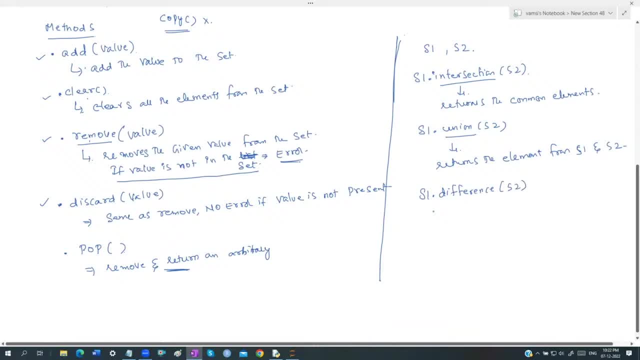 You know what is a difference. After, After removing the S2 element from S1, whatever that is left over, those values are going to be gets coming. I will show you once. Have a look at this one, For example. S1 is having some elements like, let us say this guys: 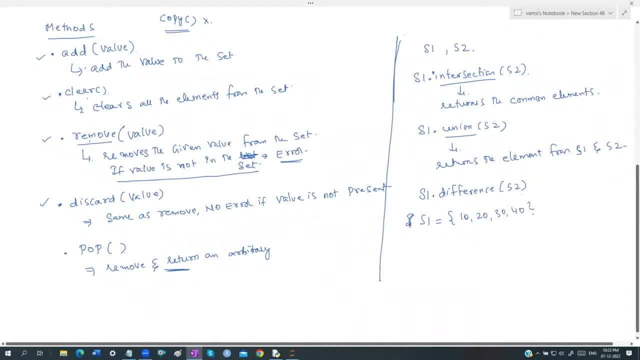 I am writing in a sequential order, But internally what order it will take, it does not matter. with that, S2 is equals to nothing, but we have some values like 10,, 20,, 30, 50, actually, guys. 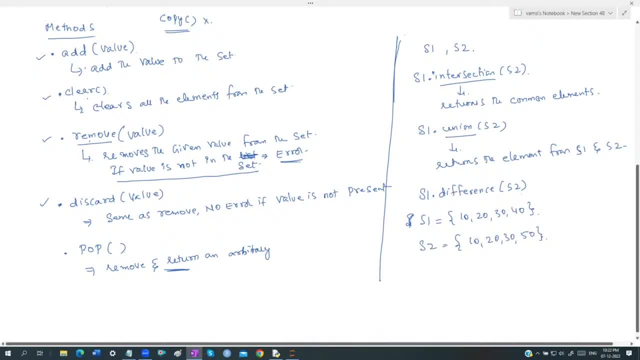 Just an example: S1 is having 10,, 20,, 30, 40. Whereas S2 is going to be having 10,, 20,, 30, 50, we have it actually, guys. Now, if I do S1 intersection S2, the result is going to be nothing but the common elements, actually, guys. 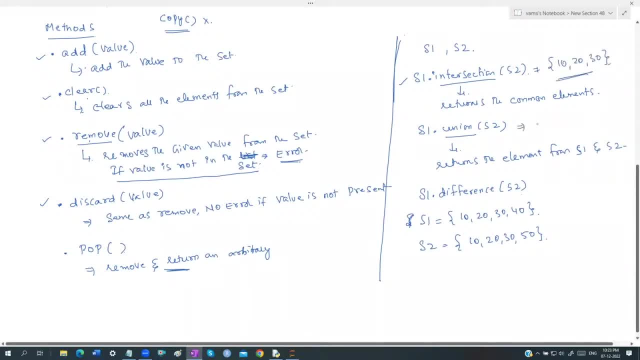 Order may not be the same. actually, guys, I cannot say that same order Union. we know it. actually, guys, It is going to be 10,, 20,, 30,, 40,, 50 will come. actually. 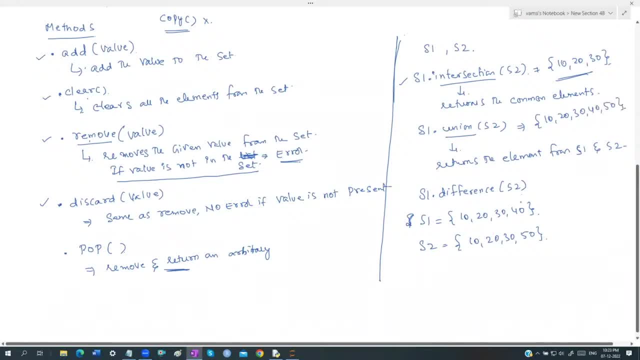 But we know this guys: What is S1 difference, S2, S2 difference, S1? If I say S1 minus S2, it is 20, 20, 30.. Sorry, 10, 20, 30 is eliminated. 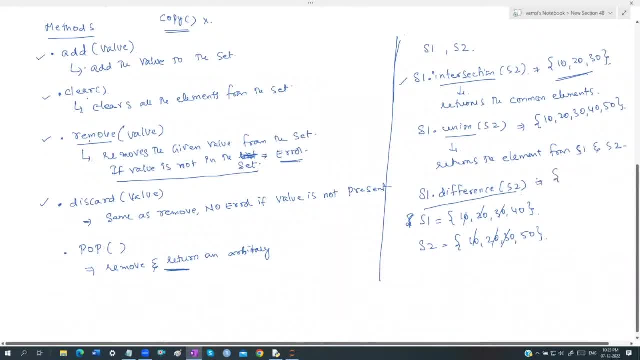 If I said S1 difference, S2,, the result is going to be nothing but what is left over in S1, which is going to be nothing but 40, actually, guys. But whenever I said S2, difference of which is going to be S1,. 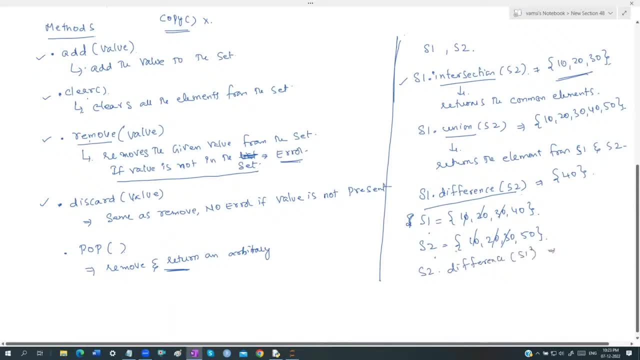 then the result is going to be nothing but what is left over in S2 after removing the element from the S1.. Then the result? we know that it is 50,. actually, guys What the point is. So it is going to be nothing but the intersection union. 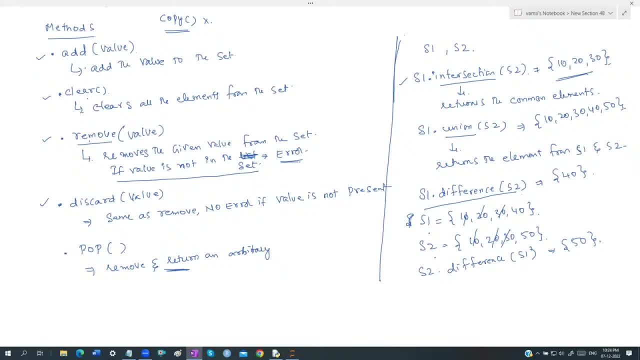 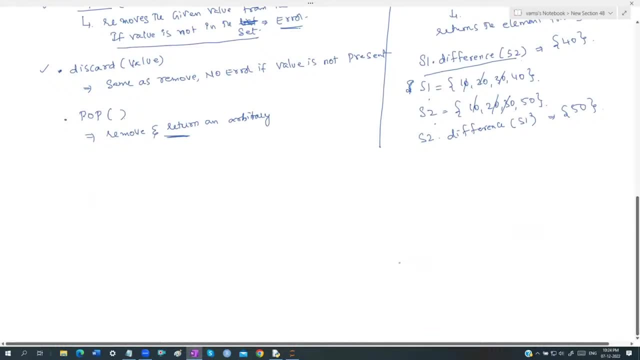 and it is going to be difference. actually guys. And if you remember the concept of like, which is going to be something like N, I hope you remember actually guys, subset and supersets. actually You know what is meaning of subset and supersets, actually guys. 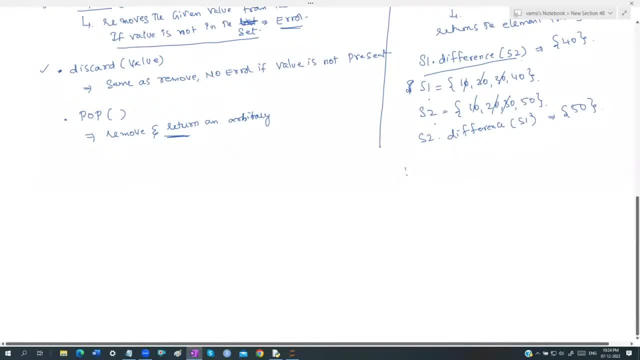 If one set is also a part of another set, like, for example, we know that S1 is having some elements like 10, 20, 30. Let us say that we have a 40 is there. S2 is having some elements like we have 10, 20.. 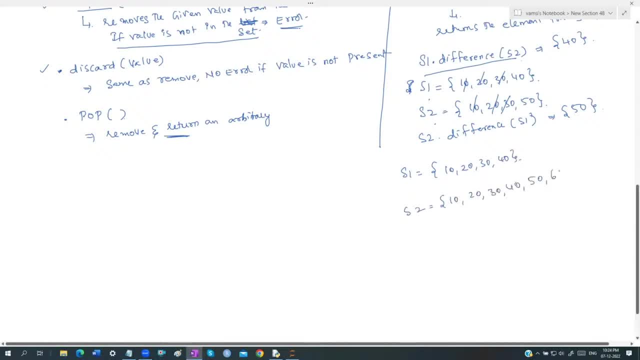 We have a 30,, 40, and 50 is there or 60 is there. Now, if we can see, S2 is containing the S1.. So S1 is nothing but a subset of S2.. And S2 is going to be nothing but a superset of S1. 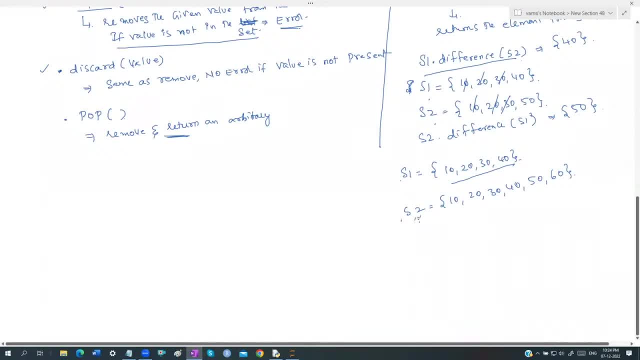 What is S2?? S2 is a superset of S1. S2 contains all the elements of S1. So if you want to check whether S1 is a subset, S2 is a subset, we have a method. is there actually, guys? 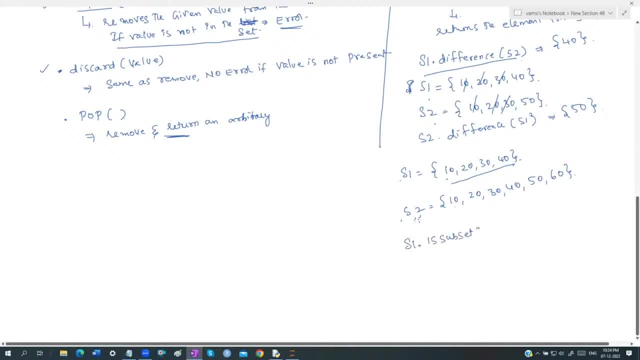 S1 dot. We have a method. There's an E subset of S2.. We are asking: S1 is a subset of S2.. It is going to return true or a false, actually, guys. So you know that E subset and E superset you are asking, you are checking. 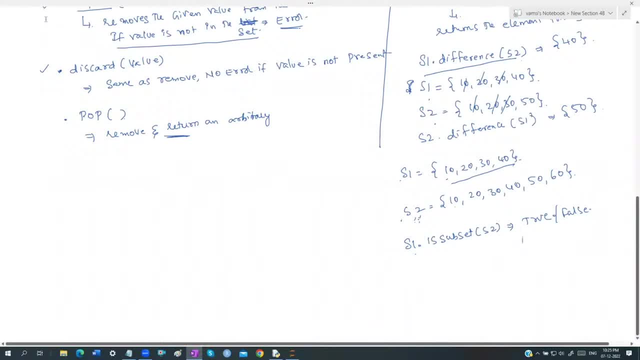 whether this set is a subset of S2, whether the S2 is a subset of S1, it is returning something like a true or false. In this case, S1 is a subset of S2 now, so it returns true, actually, guys. 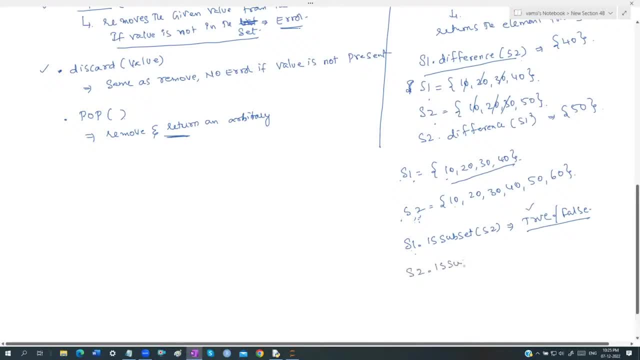 Now reverse order. I want to check whether S2 is a superset, actually, guys. So it is E superset of S1. Then also, it is going to return true or a false case. S1 is not a superset of S2, and S2 is not the subset of S1,, actually, guys. 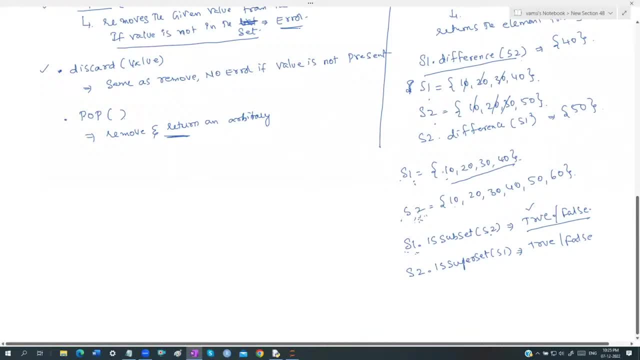 Because S2 contains all the elements of S1, but S1 does not contain all the elements of S2, actually. So a little bit mathematics, guys. Don't think that, sir? we learned a long back ago. It's just like a reference. 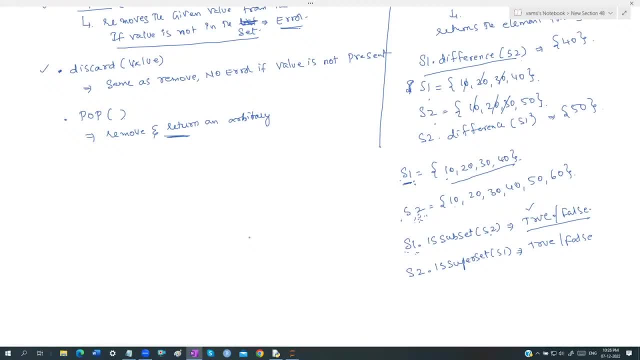 Freshman class. you maybe learned a long back ago Intersection union. it's a difference. actually, guys, In mathematics we call it as a minus, Here we are going to call it as an. a difference is there? 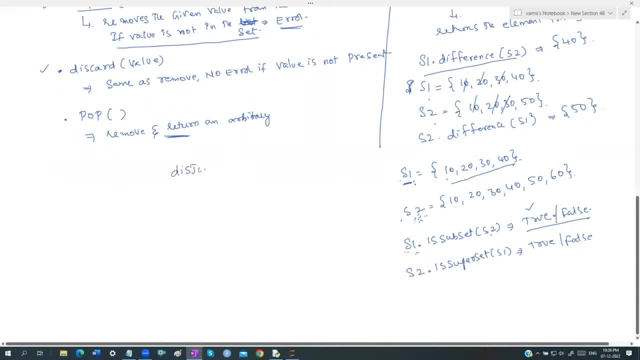 Do you remember, guys, anybody, what is meaning of a disjoint? Anybody, guys? Do you remember guys, what is meaning of a disjoint? actually, guys, No, Vamsi. Disjoint is nothing but whenever two sets don't have any common values. 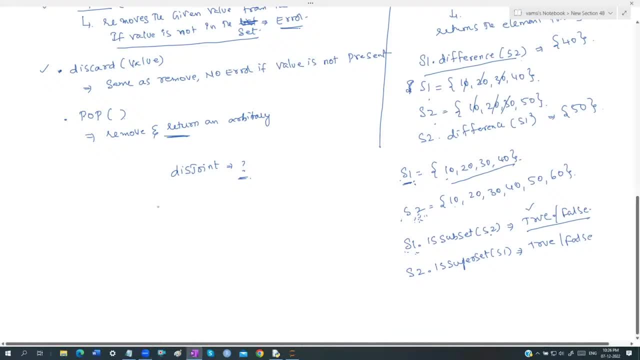 Then the two sets are nothing but what we call it as a disjoint sets, actually Like, for example, A is having some elements like 10, 20,, 30, 40. And whenever we are having, B is having an element like 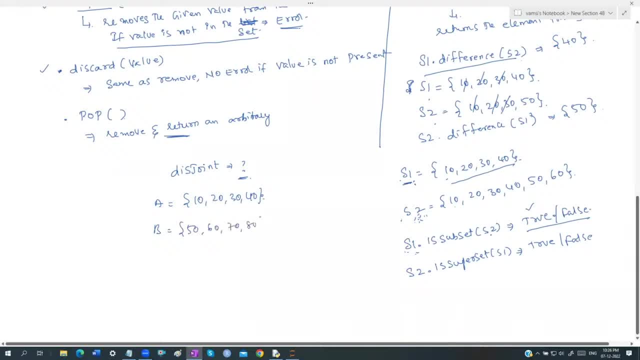 which is going to be 50,, 60,, 70,, 80.. Now, what about the A intersection B? actually, guys, In mathematics- I'm writing it actually- A intersection B is going to be nothing, but it's an empty, actually, guys. 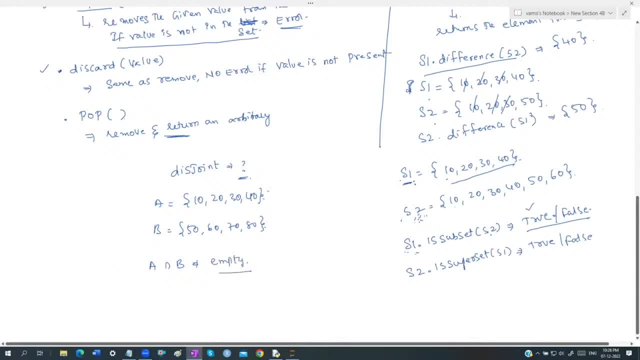 That means there is no common values, are there? So if you want, then the A and B is nothing but what we call it as a disjoint sets- actually Disjoint sets, actually. Okay. So if you want to test, we can test it. actually, guys. 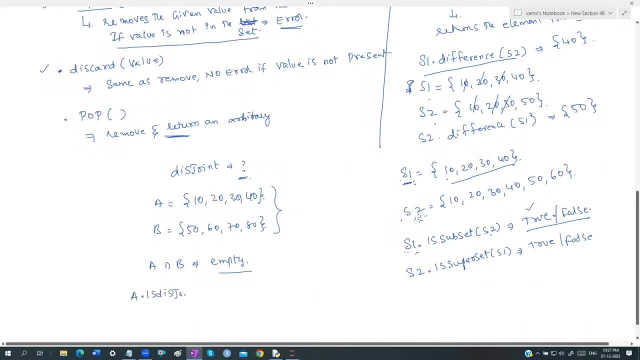 It is A dot is disjoint of, which is going to be nothing, but it's a B actually. So it is going to tell you whether it is true or whether it is false actually. So see, guys, Is disjoint is subset, is superset. 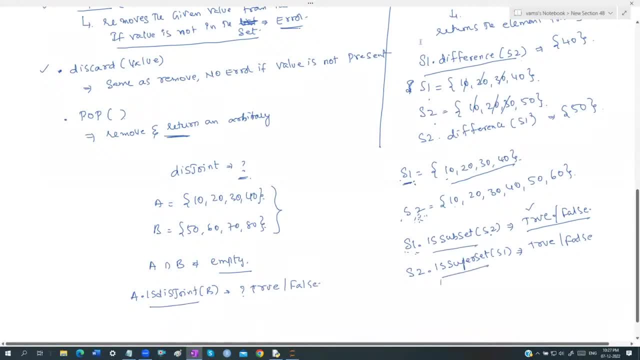 They will only check out whether it is a subset and superset or whether it is going to be a kind of a disjoint. Actually, it's a negation. actually, guys, It's an okay opposite. It's a negation. 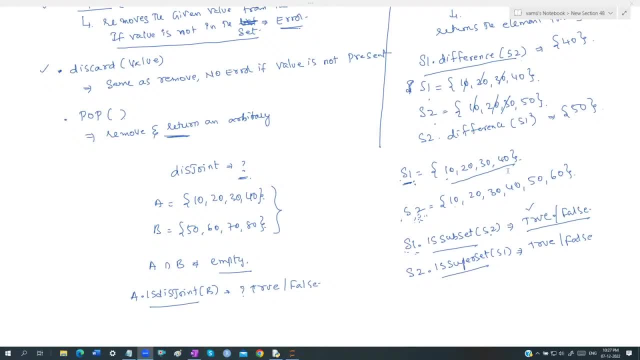 It's a negation. actually, Intersection is nothing but which is a common values will be there. Disjoint means nothing but which do not have any common values, Which have common values, which do not have the common values. That's it actually, guys. 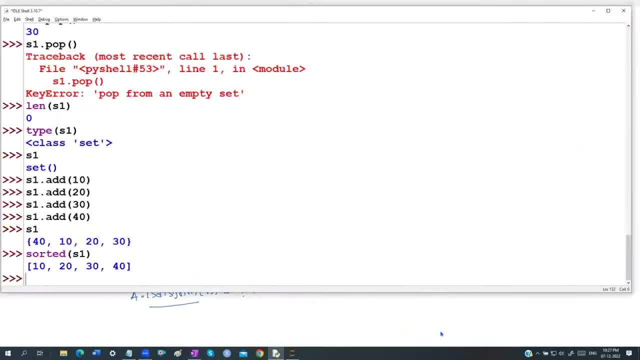 Okay, So just we can play with the things. We can just play with the things actually. Just you can also do by yourself. actually, guys, I think one or two days back, maybe you may be having a little bit confusion to understand them actually- 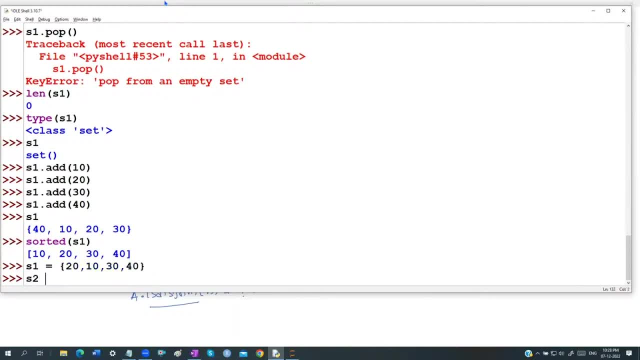 But now you got a little bit control on this. all these topics, actually It is going to be 10, 20, which is going to be 30 and 50, actually, guys, If you want, I can show you once again. 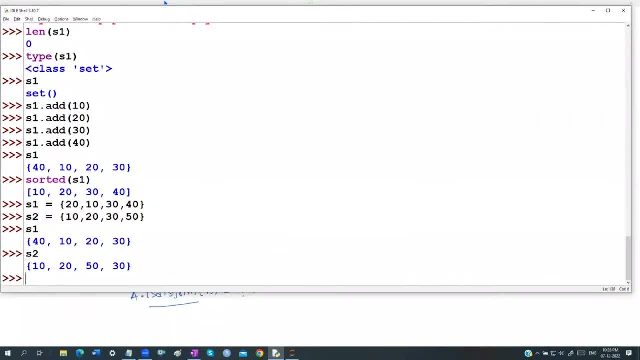 S1, S2, actually guys. S1 is having 10,, 20,, 30, 40.. S2 is having 10,, 20,, 30, 50.. So how do you do it, actually, guys? 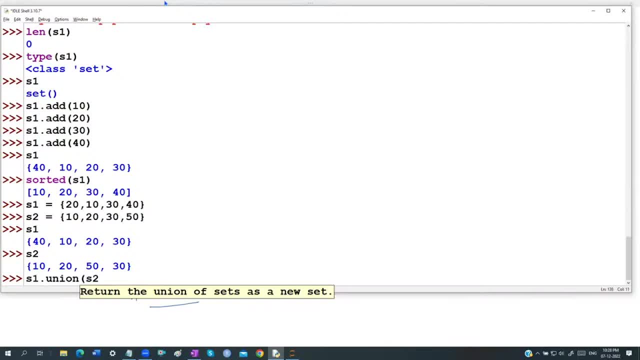 S1 union, S2.. Very simple guys. Returns the union of the sets as a new set, So 10,, 20,, 30,, 40,, 50. And you know that. S1 union, S2, S2 union, S1,. 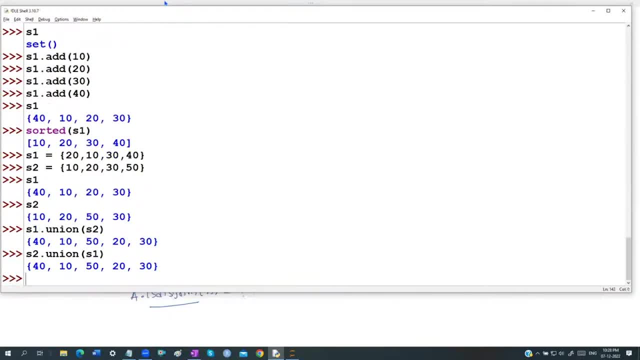 both of them are going to be same, only guys. There is no change in the output, Same as it is. what is intersection actually, guys? Intersection of S2.. Returns the intersection of two sets as a new set actually. 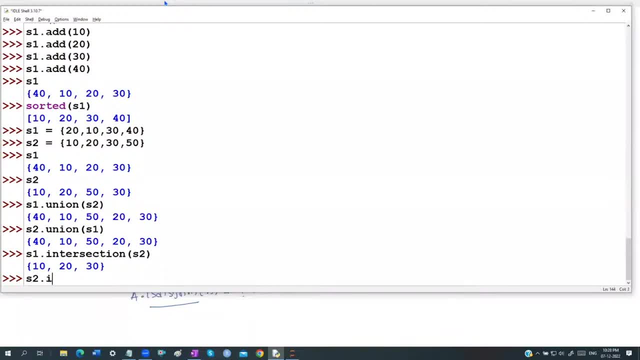 S1 intersection S2 is going to be 10,, 20,, 30. Even S2 intersection S1 is also going to be same result, only No change in the output. But what about the difference? Actually, guys, difference is nothing but minus. 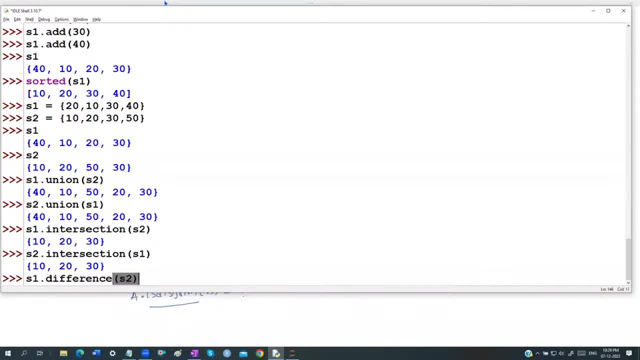 We have a function. is there Method? is there actually, guys? Difference of S2.. You can see very clearly, guys, What is difference will return. Return the difference of two or more sets. as a new set, It is going to be S2, actually, guys. 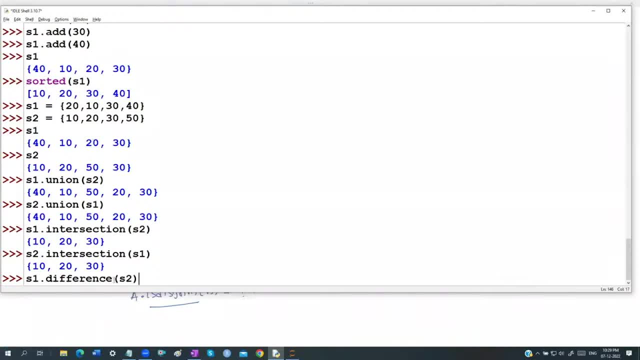 That means what we have to do, guys: S1 minus S2.. So S2 should be eliminated from S1.. What is there in the S1? After removing the S2 from S1,, what is left over in S1, guys? 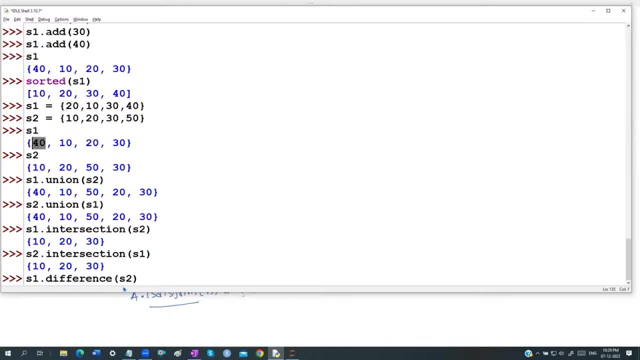 Don't think that S1 difference S2 means it is S1 is removed from S2.. No, It's S2 removed from S1.. So what is left over in S1, which is going to be 40, is the result actually. 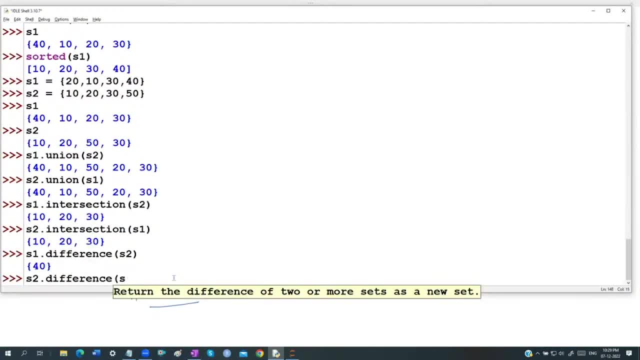 But when you do S2 difference, S1, then the reference is going to be nothing but difference output S. So we know that A union, B and B union is the same associative property. A intersection, B and B intersection is the same, But A minus B, B minus A is not the same case actually. 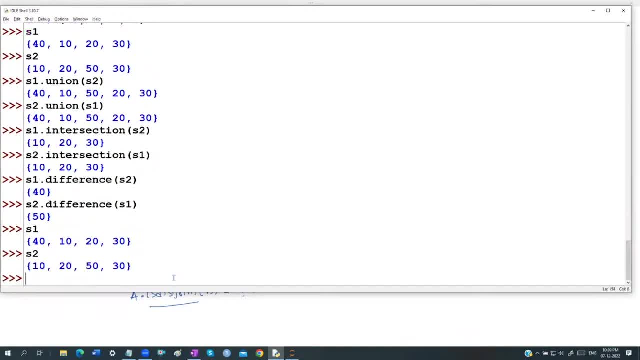 Same as it is. we have S1 and S2, actually, guys, Here, S1 is not a subset of S2.. S1 is not the subset of S2,, guys, What is meaning of subset? All elements must be there. 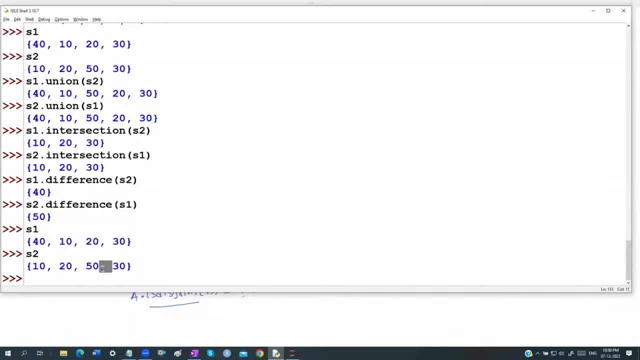 So all elements of S1 is not there in S2.. All the elements of S2 is not there in the S1, actually. So S1 is not a subset, S2 is not a subset. None of them is a superset, actually, guys. 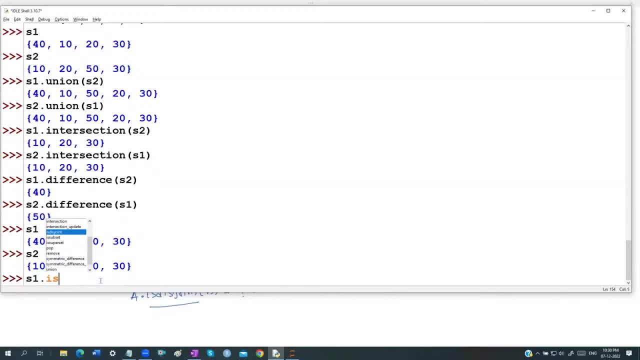 S1 dot which is going to be. I'm asking guys, is You can see there guys- Is disjoint, Is subset, Is superset? Is S1 is a superset of S2.. Returns whether this set contains another set. 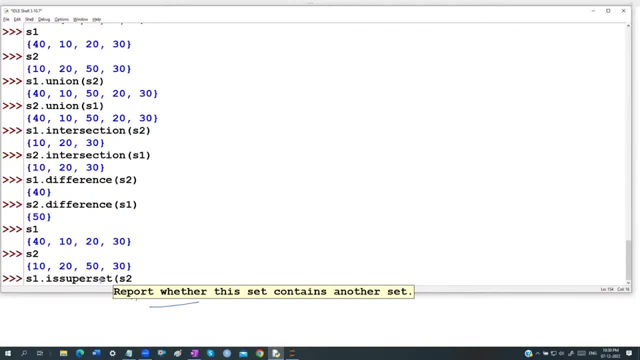 You know, superset means It contains another set. It is subset means this set is part of another set actually. So S1 is a subset of superset of S2.. It's a false Is: S1 is a subset of which is S2.. 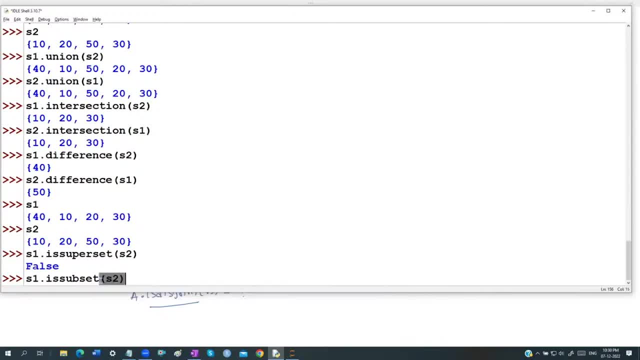 Returns whether other set contains this set. actually, guys, It is going to be. none of them is going to be true, guys, Even S1, intersection S2.. Is it is a disjoint? actually, guys, They are not disjoints, actually. 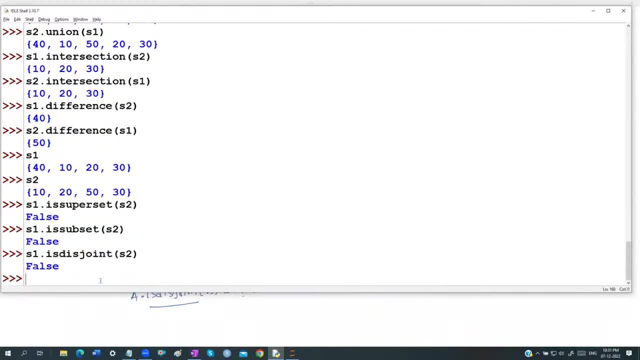 Because there are some intersection common values. are there, guys? All of them are returning false. actually, guys. But if you want to return true, you know what we have to do. it, actually guys. S1 equals to 10,, 20,, 30,, 40.. 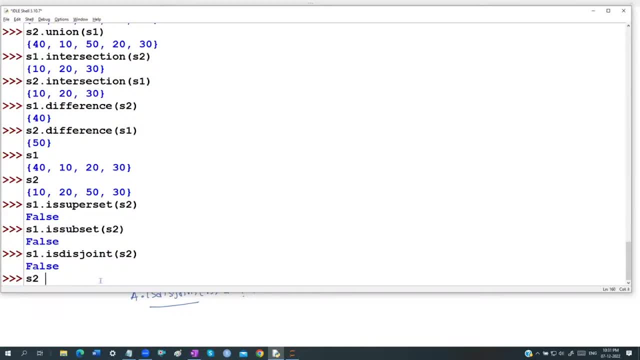 It's already there, S2 is equal to nothing. but Otherwise I'll do one thing, guys. S2 is equivalent to: Let us say it is Sorry. S2 is equal to 10,, 20,, 30.. 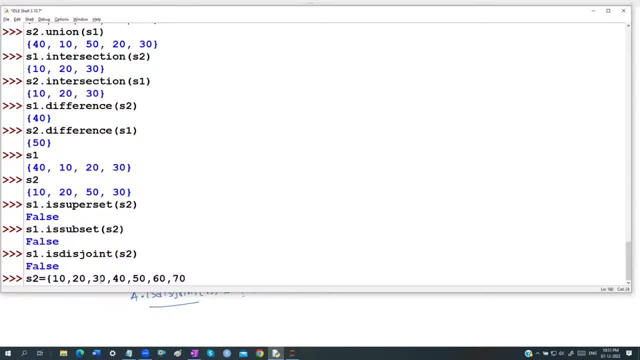 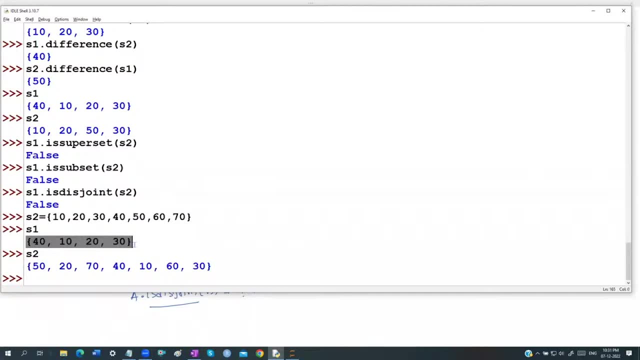 Which is a 40,, 50,, 60,, 70, actually, guys, Just an idea about that: S1 is this one, guys. S2 is this one. Now, whatever the elements of S1 is there, all elements are there here, guys. 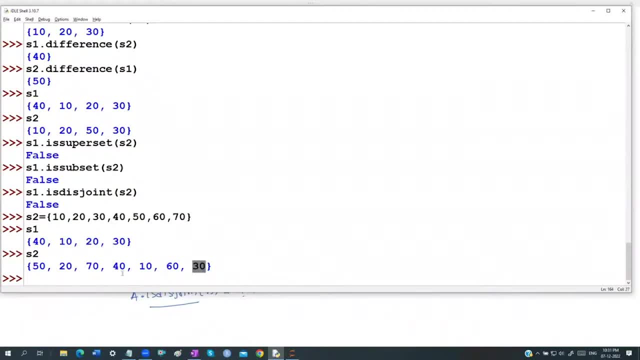 That is 10.. It is 20.. It is 30. And it is 40. So here S1 is called as an subset of S2.. Now you can ask: Is S1 is a subset of? Is it is a subset of S2.. 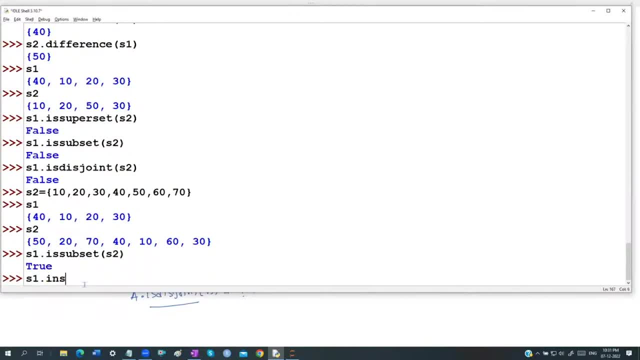 Yes, it is a subset of S2.. Is S1 is a subset of S2.. Is it a super set? No, it is not a super set. actually, guys, It is not a super set of S2, actually. 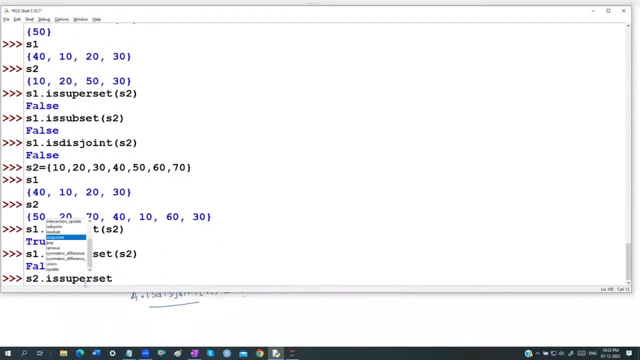 But S2 is a super set of Which is going to be nothing, but It's a super set of S1, actually, guys, That is the idea of how we are working with And how to say that it's a disjoint. actually, guys. 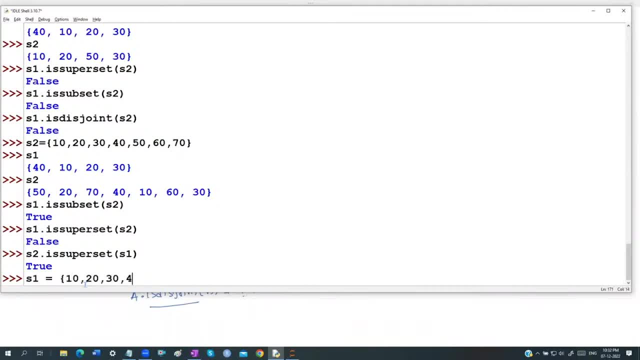 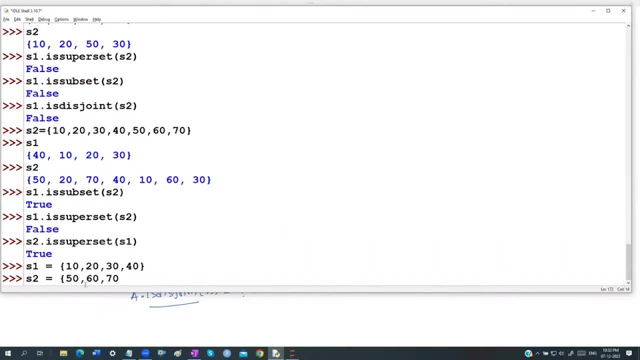 S1 is equals to, I said, 10,, 20,, 30,, 40. Whereas S2 is equals to, Let us say, 50,, 60,, 70, and 80, actually, If we can observe carefully, there is no common values guys. 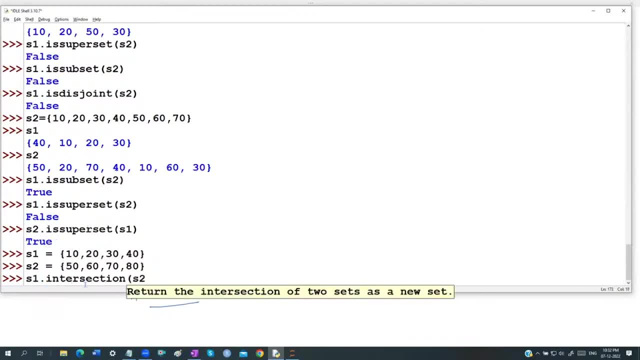 S1 intersection with S2 is going to be nothing. but There are empty list. actually, guys, You can see empty list is coming Then whenever there is no common values between S1 and S2.. There is no intersection values, guys. 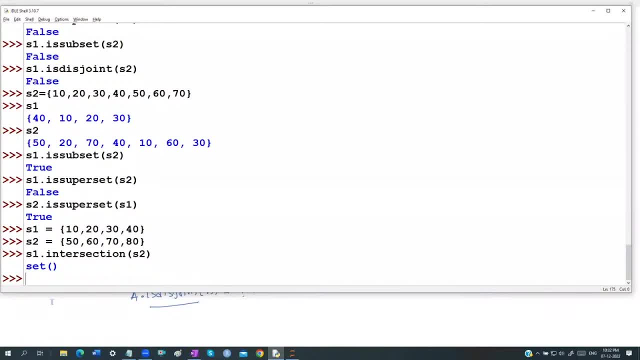 Union I can do, guys, But intersection I can't do. Intersection is empty. So, whenever there is no common values, Then S1 and S2 are basically what we are going to call it as an. A disjoint functions What the disjoint sets. what we are going to call it as actually guys. 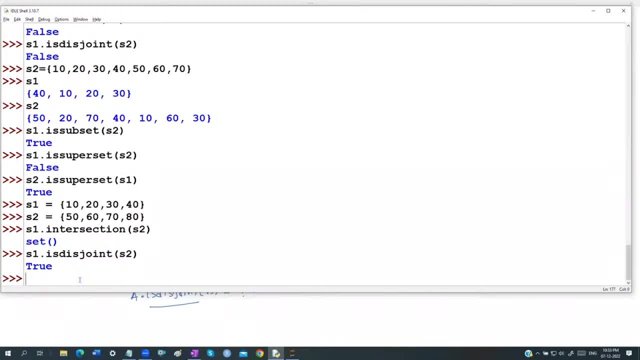 We have a number of methods actually, guys, If you remember, in list concepts, first day I taught you three methods. Second day I taught you another three methods. After that I have discussed about the remaining one or two methods. 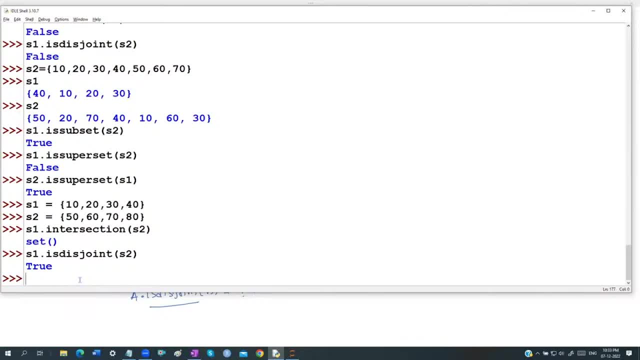 I have been discussed about the three or four, I think. first class it is four, Second class it is three And next class it is three. I have been more discussed, But today how many methods you discussed actually, guys. 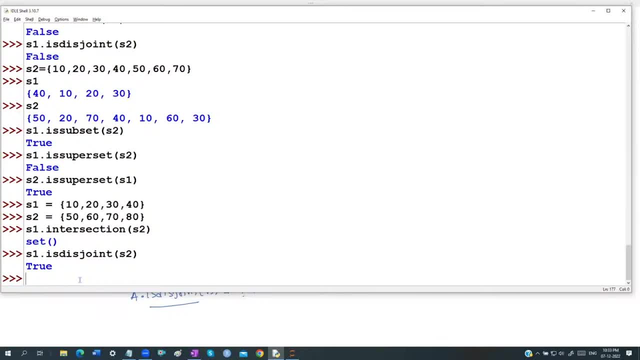 Add: Uh, we have. I have been seen about a clear. These are common methods. Actually, guys, remove discard Bob. No intersection union at this. uh, minus, which is going to be the difference. Actually, I guess he subset is, superset is disjoint. 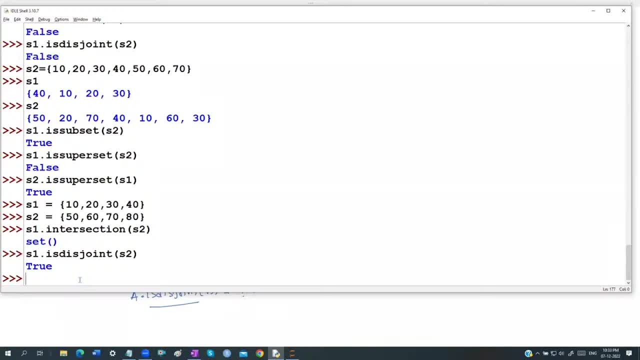 So almost all we are having somewhere around 11 or 12 methods. We have been got this Like that. we are going to be the same methods, only Guess if you see them. I told you, no, I don't have anything to hide from you. 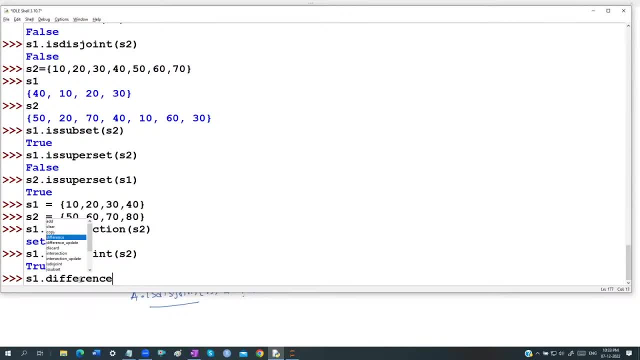 Add clear Copy. I told you guys I don't discuss about that difference. I already explained guys different underscore update. I'll explain difference: difference underscore updates. Like the difference is there: Discard intersection, intersection Underscore update is there.